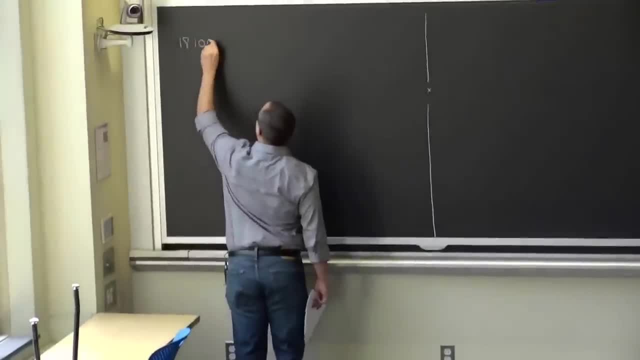 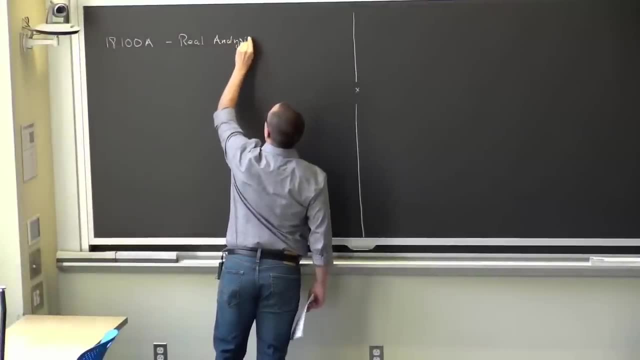 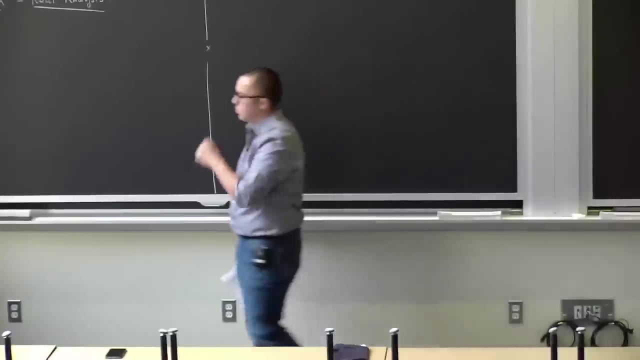 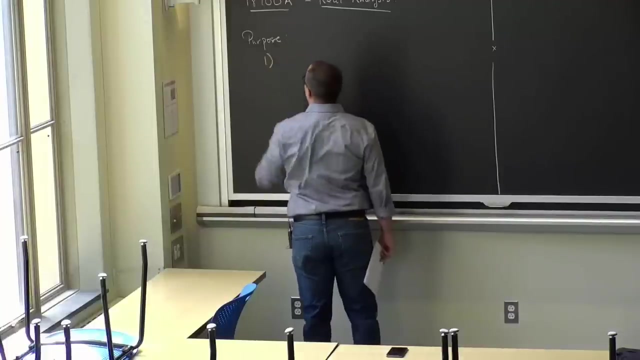 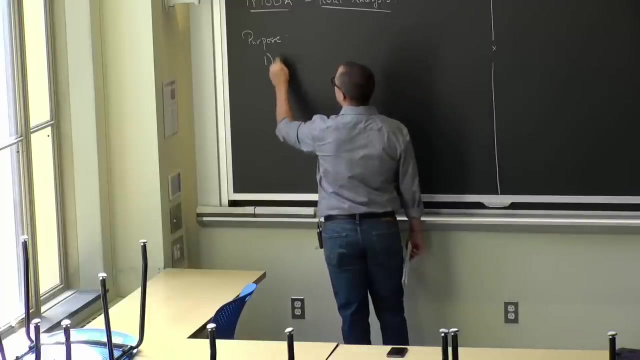 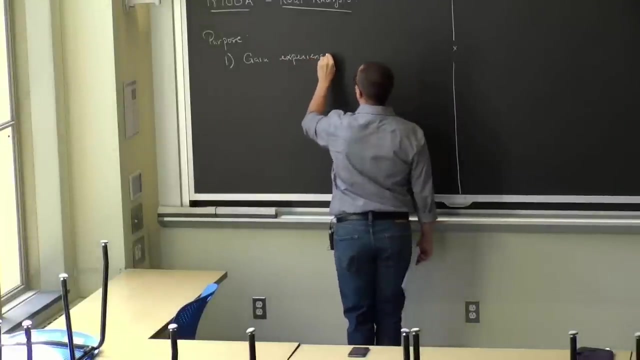 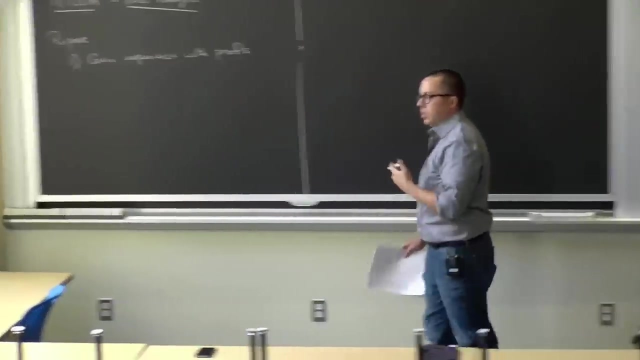 the purpose of this course. So this is for 18100A- real analysis. So the purpose of this course is twofold, Really, I think the first primary purpose of this course is to gain experience with proofs. So that means being able to read the proofs. So that means being able to read: 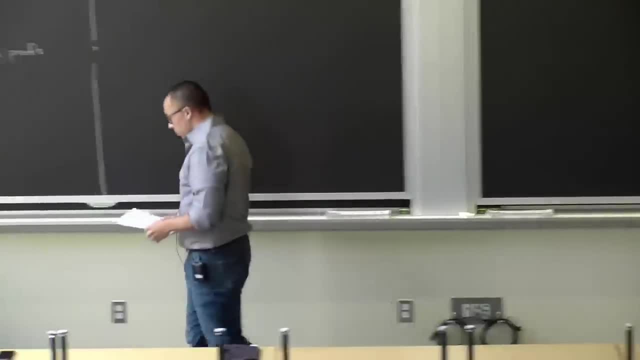 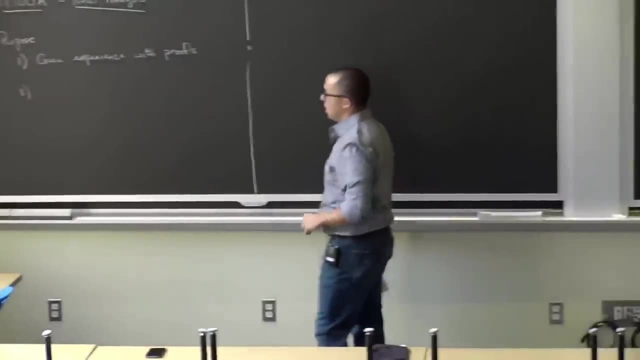 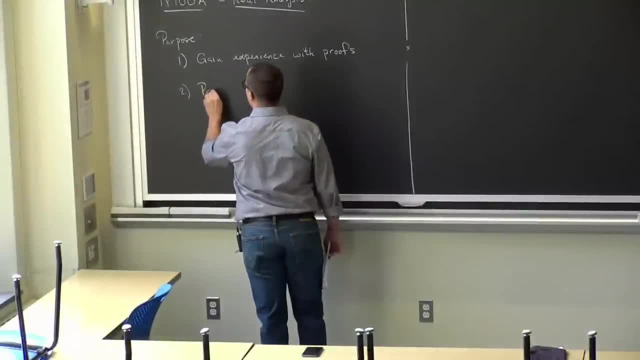 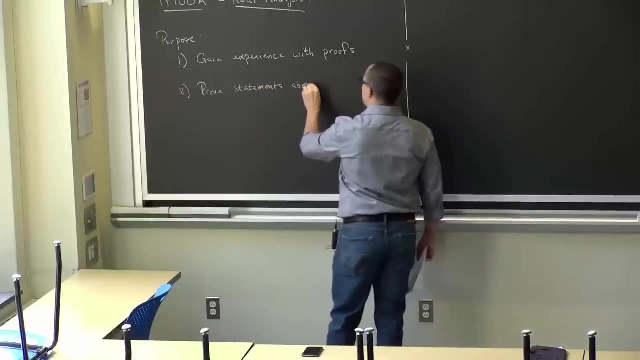 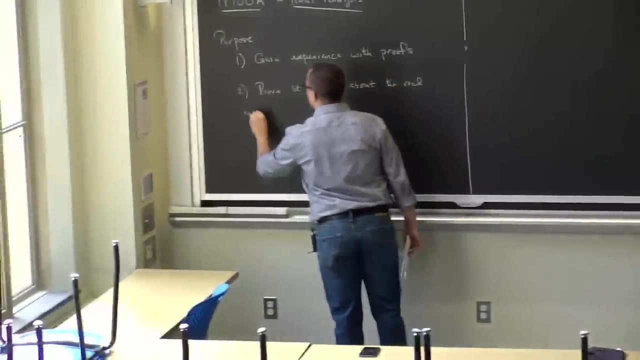 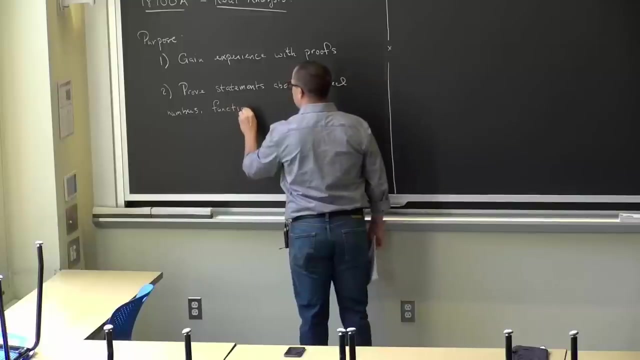 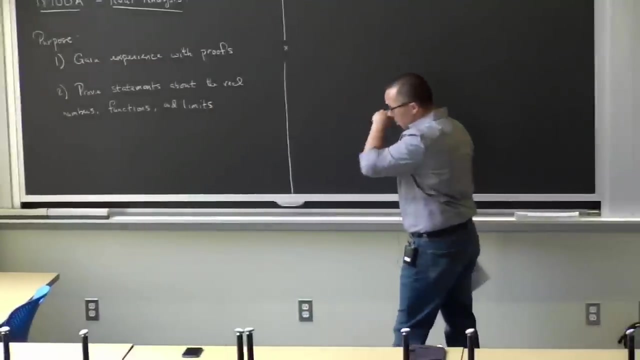 the first purpose is to prove statements about real numbers, And the second statement, which is supposed to be kind of a way to obtain the first purpose, is to prove statements about functions and limits, call text. Okay, so the second part. this is the. I'm missing one here. I don't want to do the 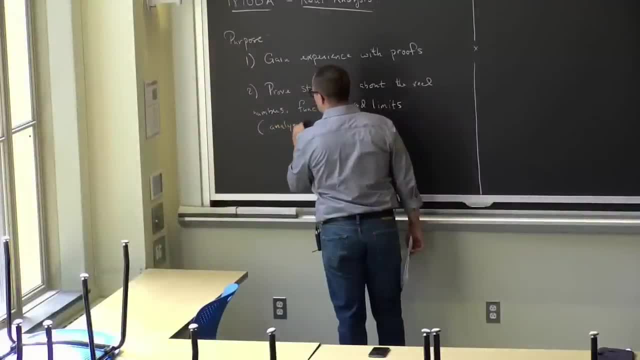 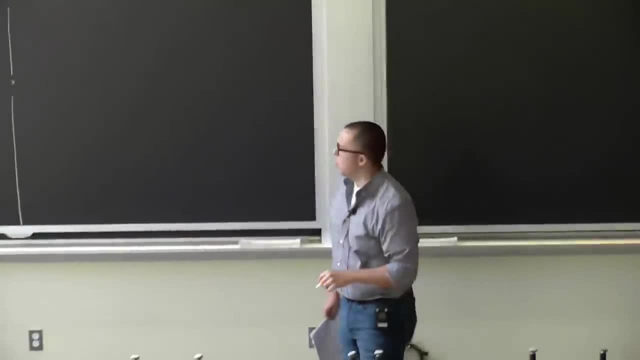 third part here. Tell it again. exercise 96. analysis part. Okay, So for the first few lines I thought I had already discussed this, because it's all a good piece of lithography I'm not giving up on because I don't think it should be Not only. 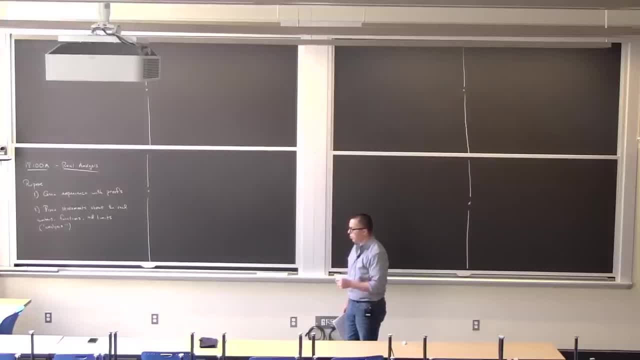 lectures. we're going to do what maybe to some will be kind of review And for most of you a lot of this material in the first few lectures will be review. But it's a nice way to ease into the material and things will most definitely pick up after a few lectures. 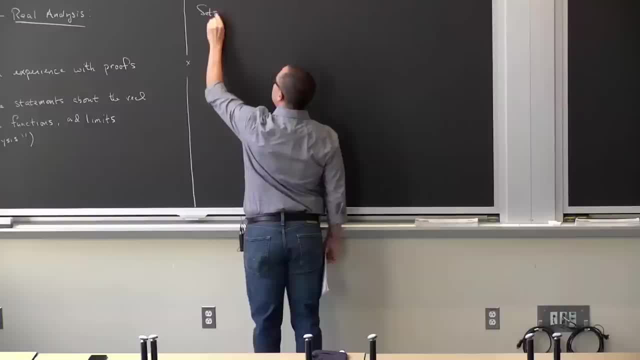 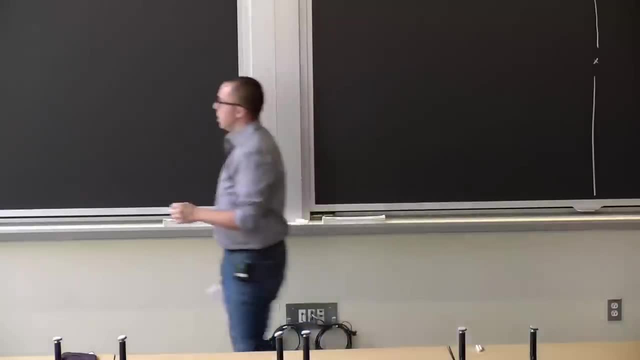 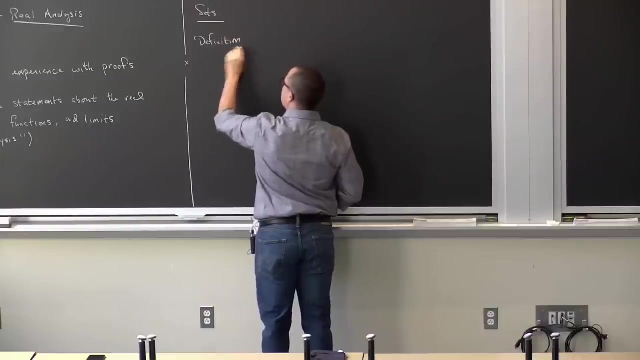 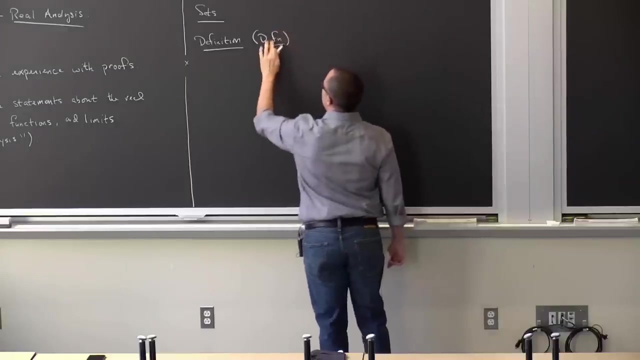 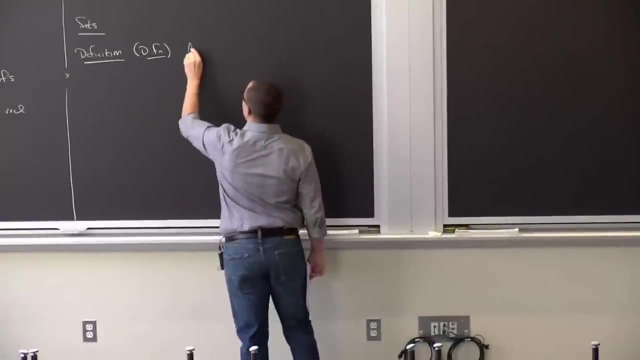 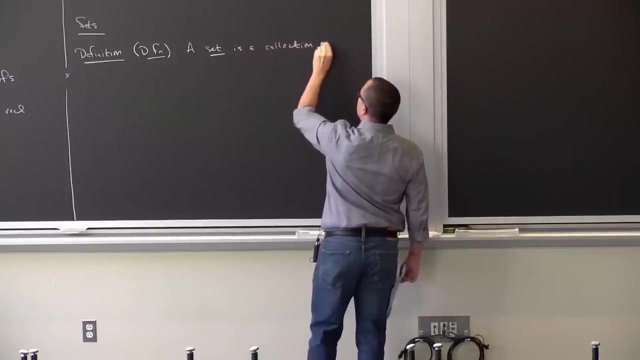 So the first set of objects we're going to define and try to prove some statements about are sets. So definition- and because I use a lot of shorthand, I will mostly write DFN from now on instead of the entire word definition. So a set is 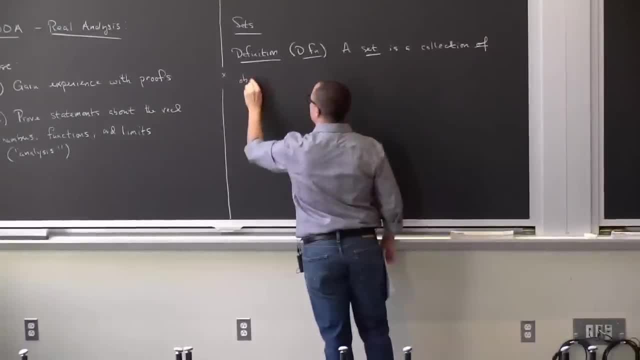 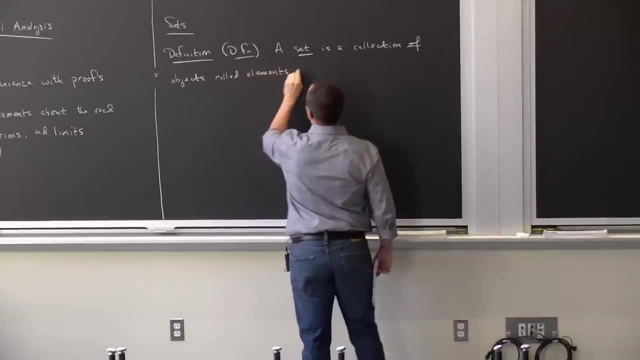 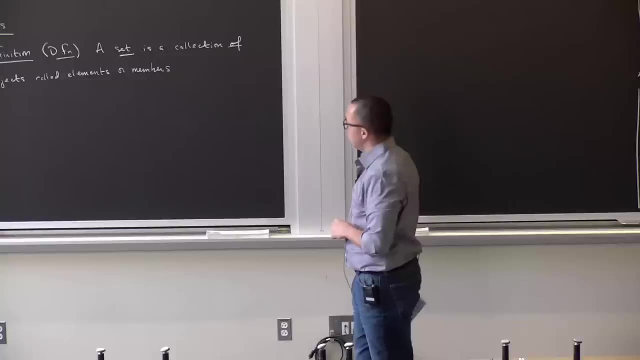 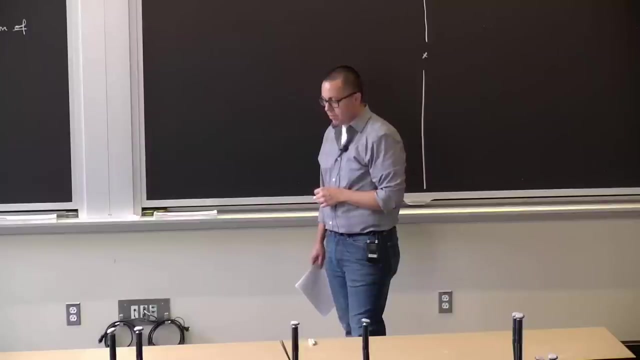 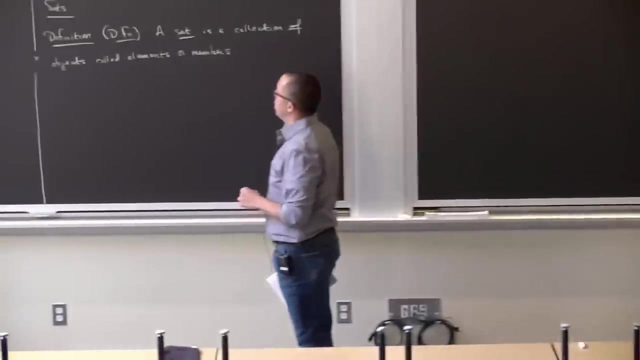 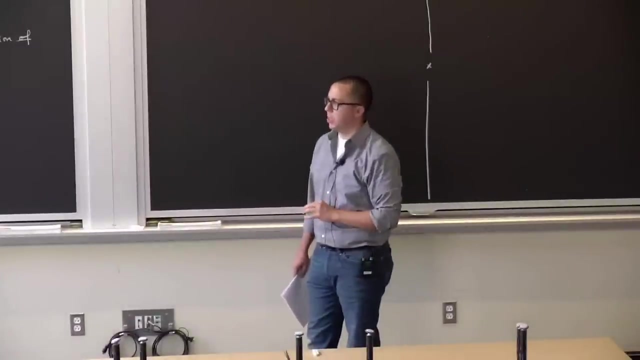 a collection of objects called elements Or members. Now, this course is supposed to be probably the first really rigorous course in math that many of you will deal with, So essentially everything that we talk about will be rigorously and unambiguously defined. but we do have to start somewhere. 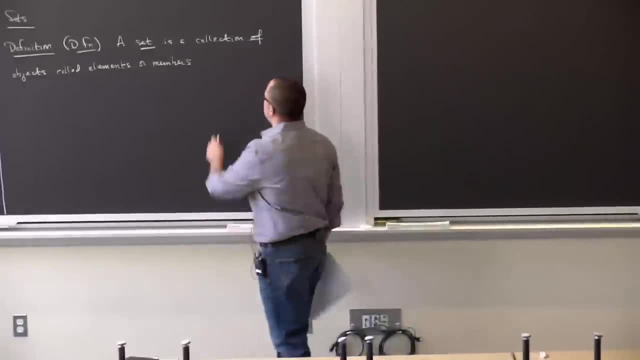 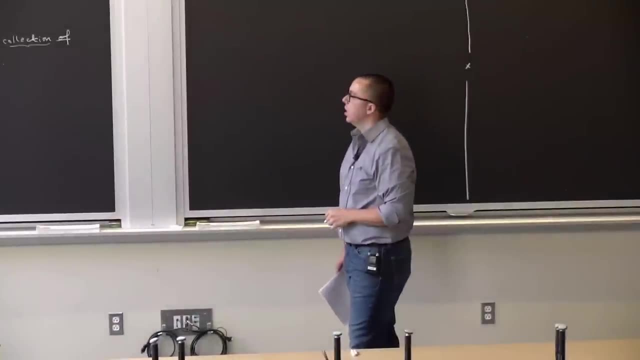 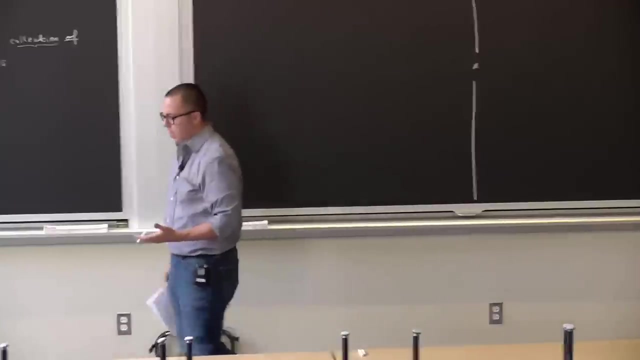 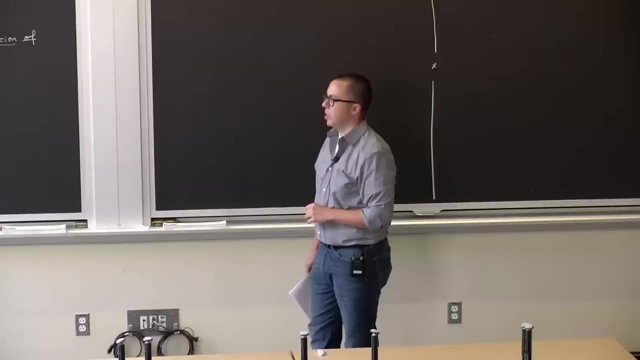 And so maybe you think this word collection is a little ambiguous, and perhaps you should. But to actually build up set theory from the ground up would take us quite beyond the scope of this class and too far afield of the things that we want to do, Or at least what I want. 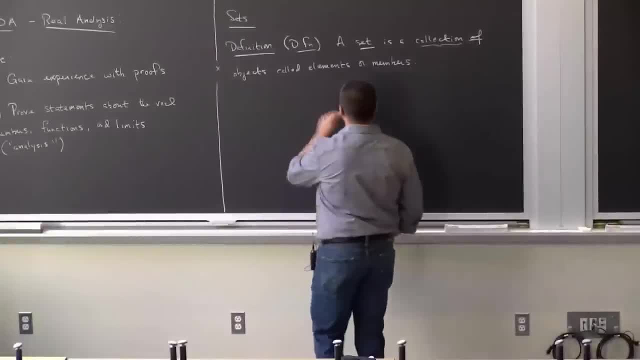 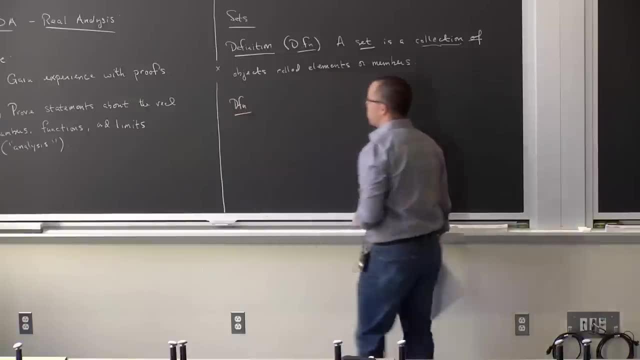 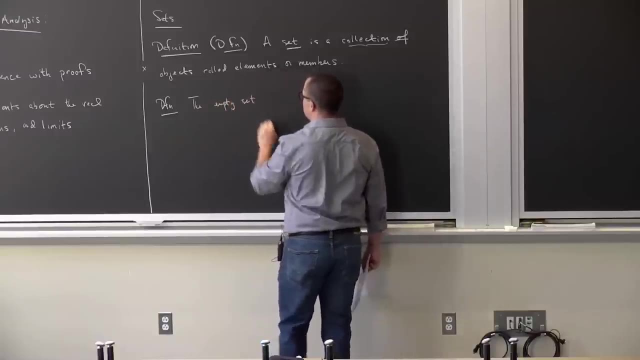 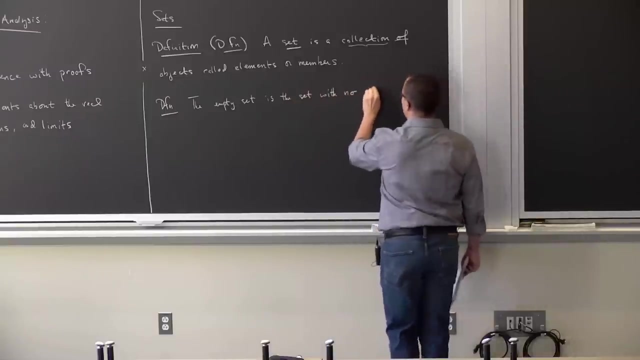 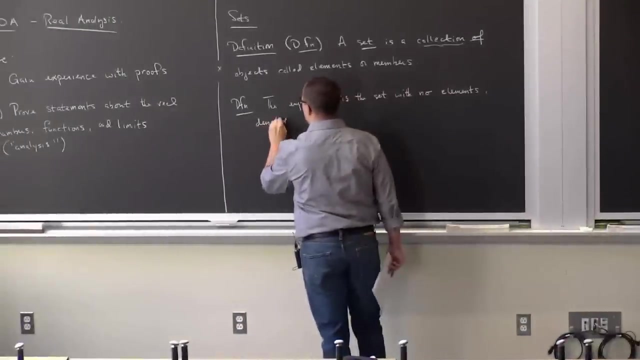 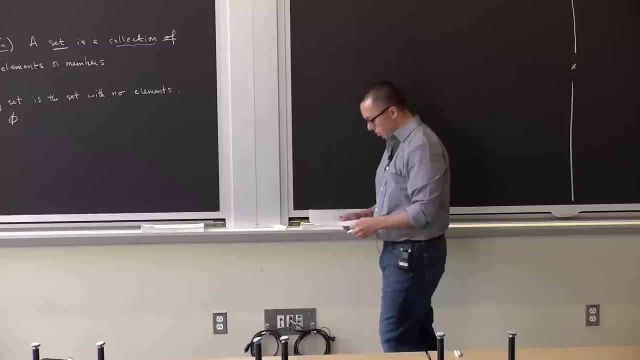 to do OK. so a set is just a collection of objects called elements or members. There is the simplest set to define: The empty set is a set with no elements, and we denote it by this symbol here, a circle with a dash through it. 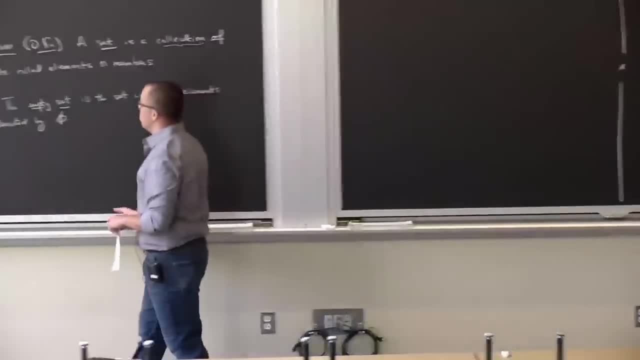 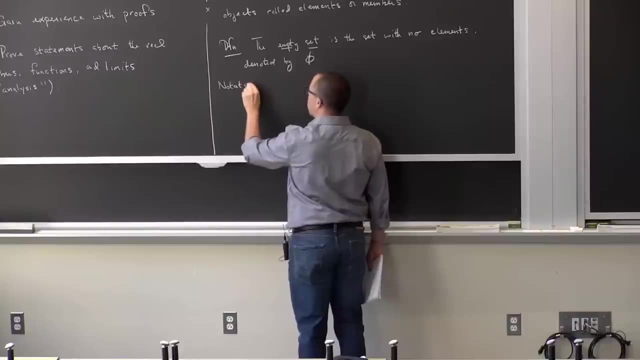 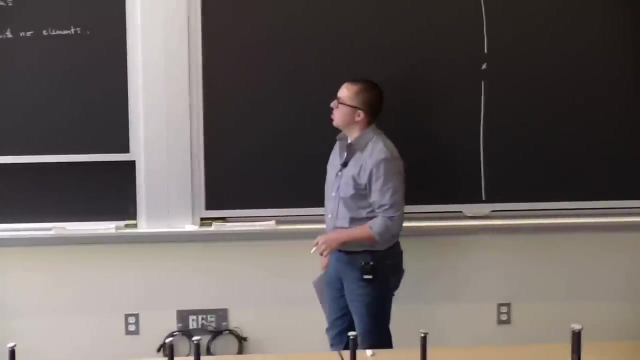 OK, So with new math typically comes new notation, new symbols that you use. so let me introduce a few shorthand notations we'll use throughout the course. I mean, quite honestly, this is, You know, quite honestly, this is a little bit of the fun of doing higher math. 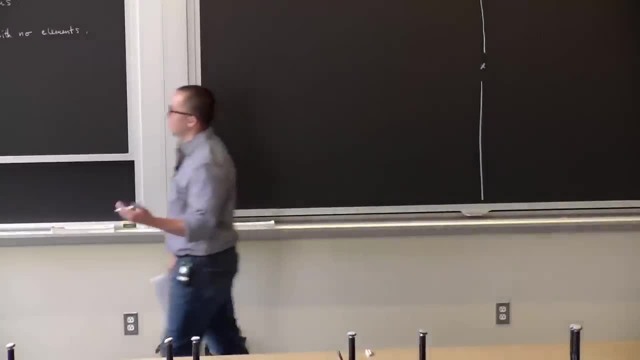 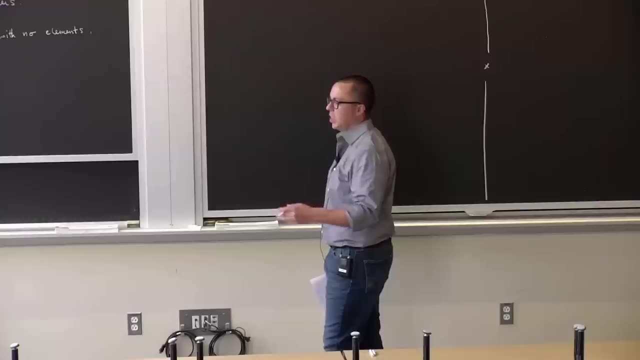 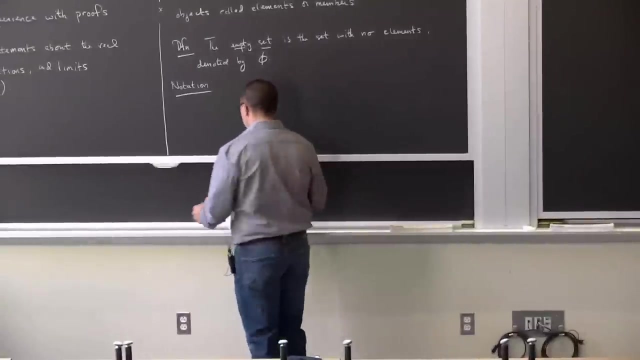 You get all these funny symbols, And a very accomplished mathematician at the University of Chicago one time said: you're really only interested in the math where that has the symbols you like to write over and over again. So some notation A and 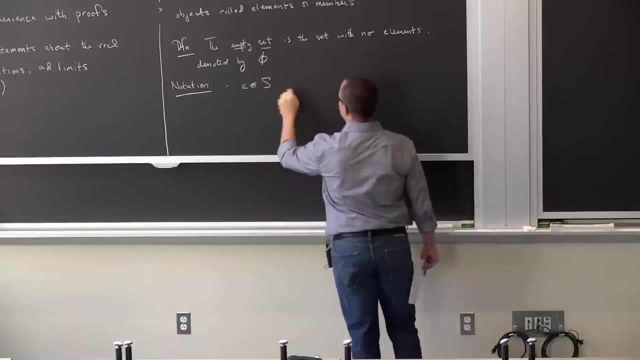 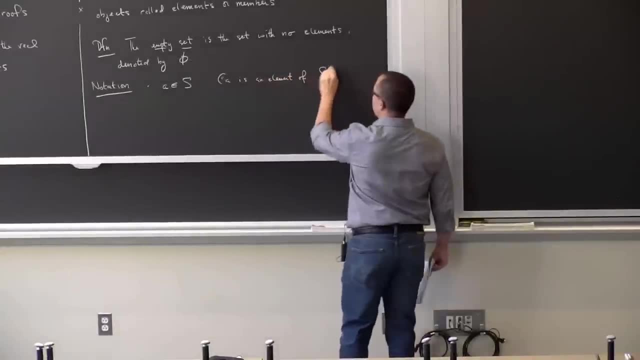 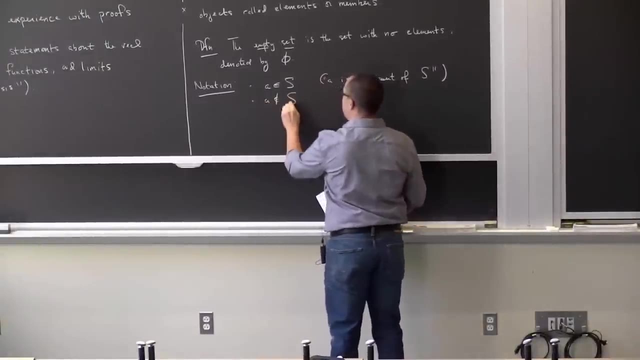 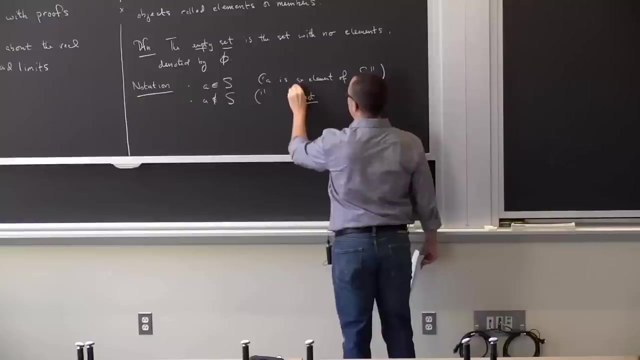 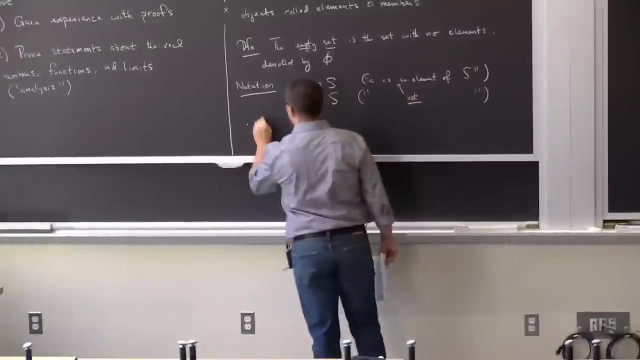 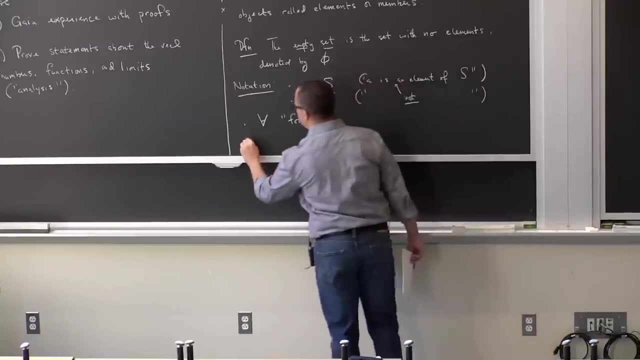 this symbol, which looks like a ES, means A is an element of S. A, with dash through this little E means everything here, but So A is not an element of S. Upside down, A means for all, the short hand, for all stayed for. 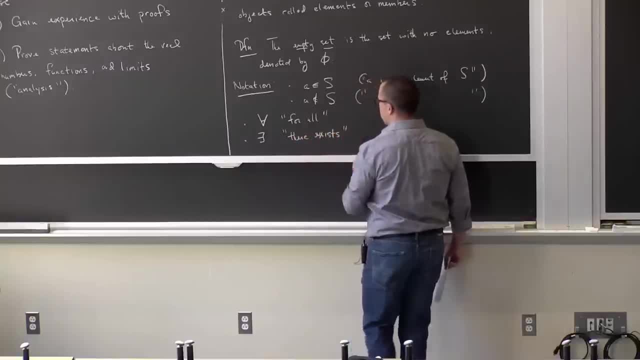 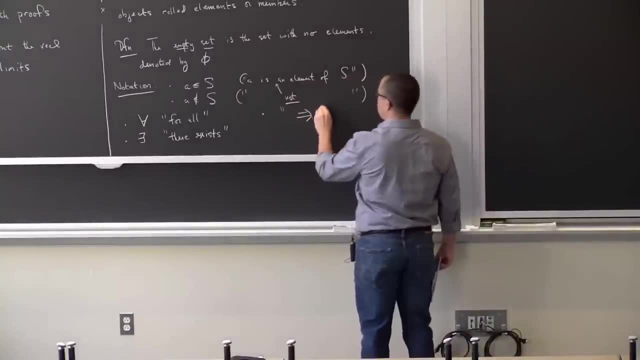 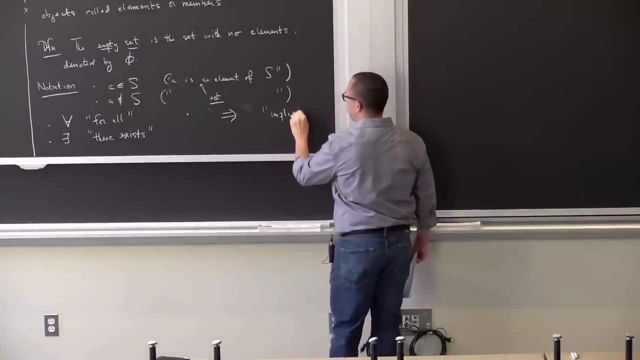 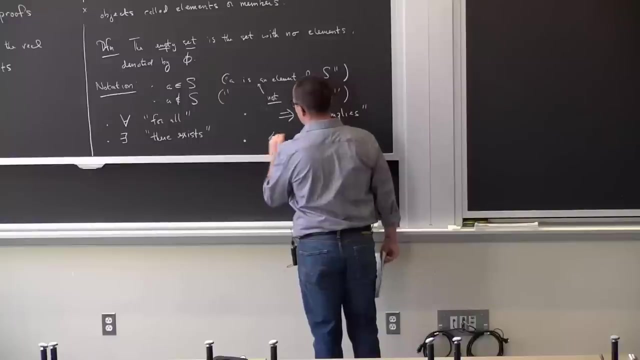 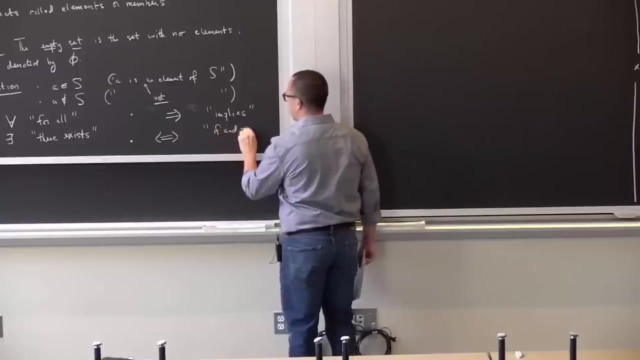 all backwards. E means there exists and a couple more. You seen arrow like this. this mean, this means Now, implies: so I've written down one thing. This implies the next statement: Put an arrow between them And an arrow going both ways means if, and only if. 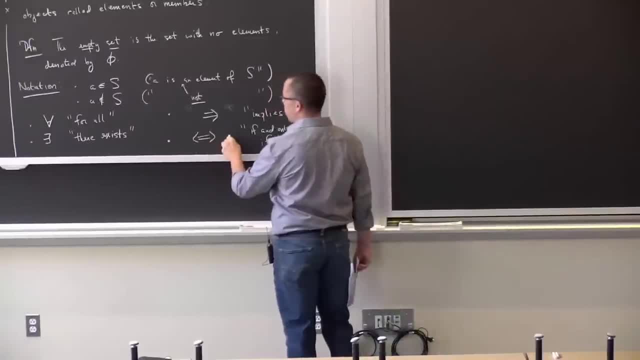 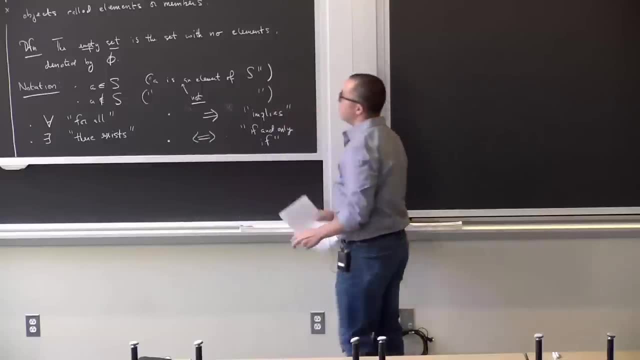 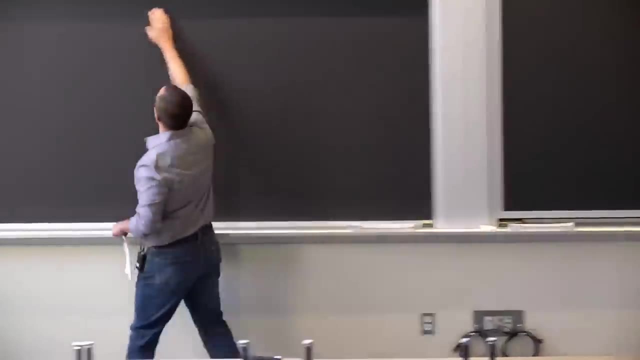 meaning, if I have a statement P, if, and only if- Q, that means statement P implies Q and statement Q implies P. All right, And if you need a quick refresher on kind of basic logic, you can find that in the appendix of the textbook. 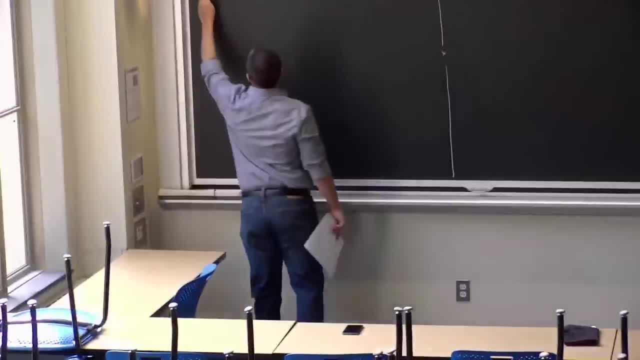 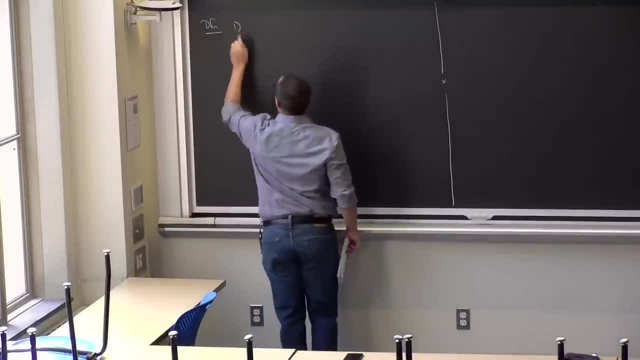 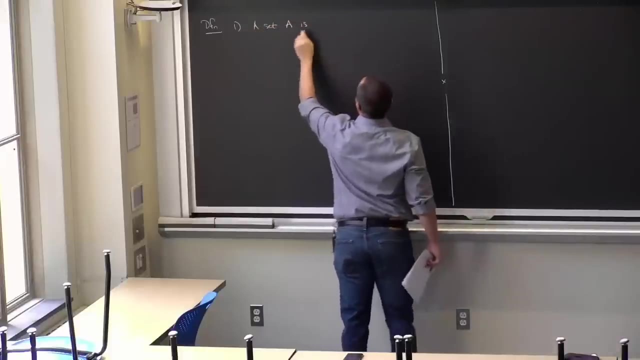 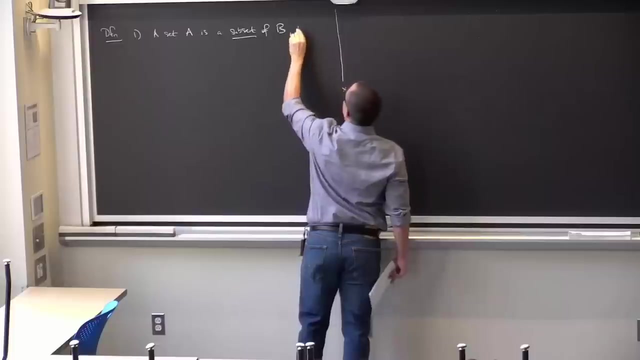 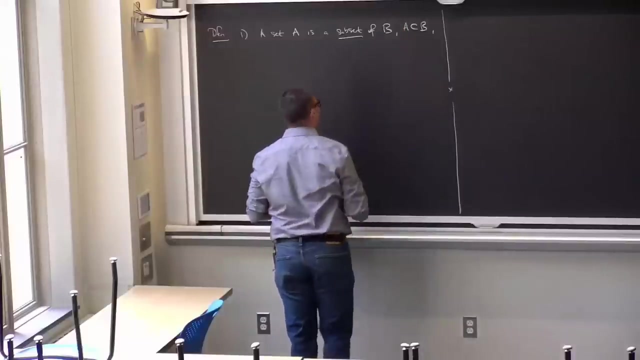 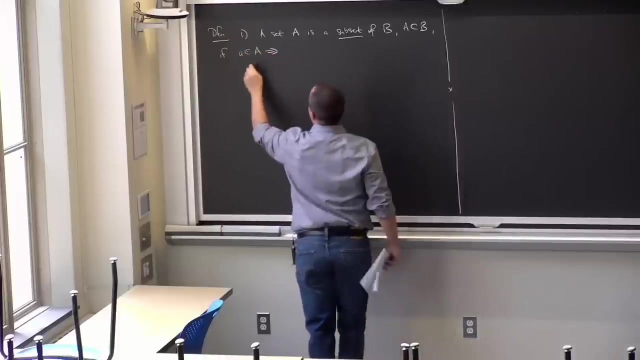 OK, So that's the basic definition of set, empty set. So it's set A. Another definition of set A is subset of B, which we write A, this little symbol that looks like a, C, B. if every element in A is an element in B, A little a's. 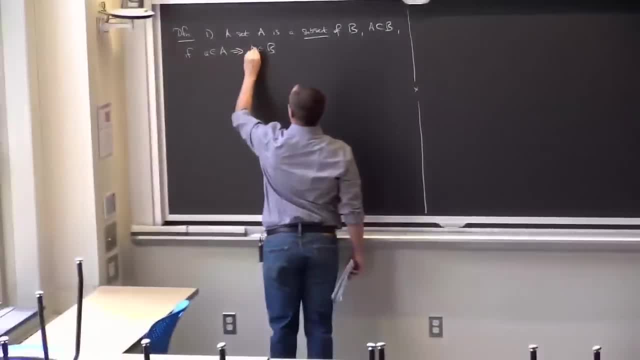 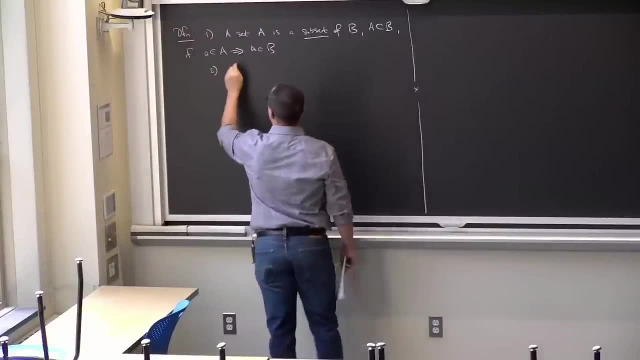 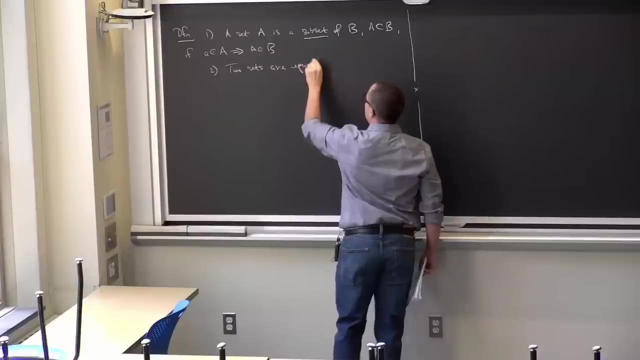 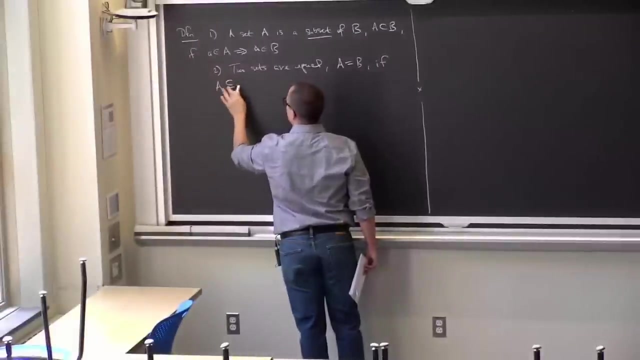 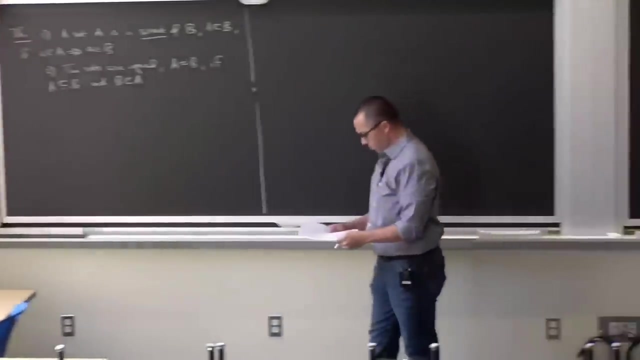 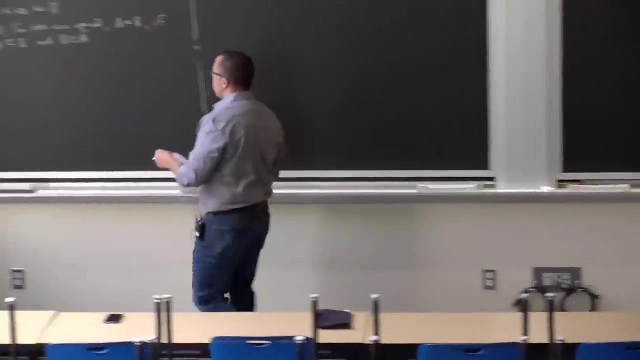 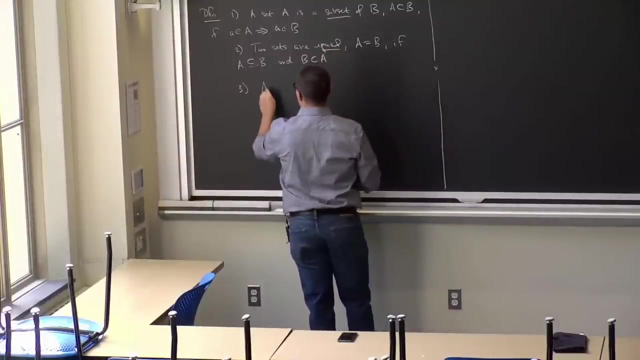 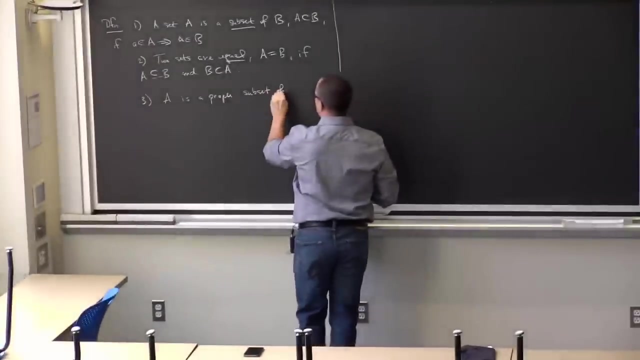 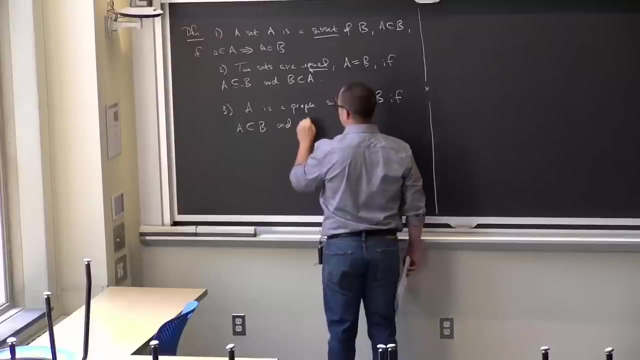 and capital A means little a. OK, OK, So A is in capital B. So two sets are equal. We write: A equals B if A is a subset of B and B is a subset of A And A is a proper subset of B. if A is a subset of B and A does not equal B. 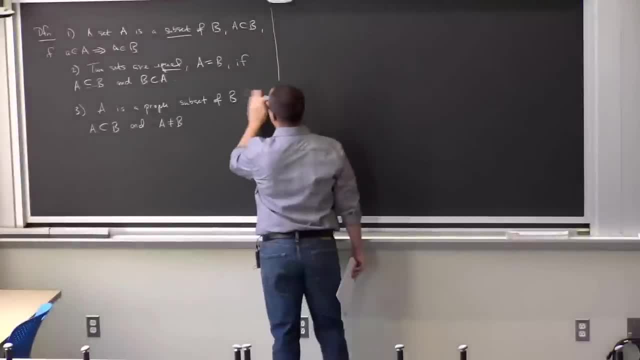 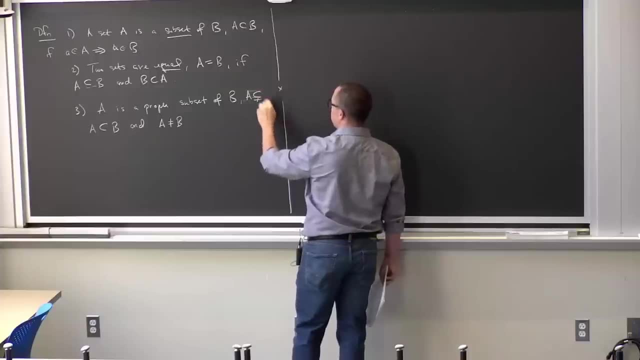 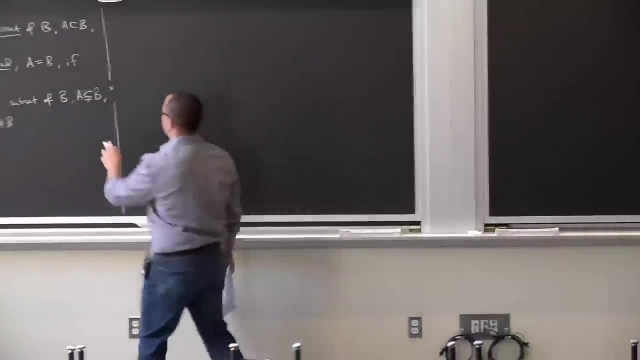 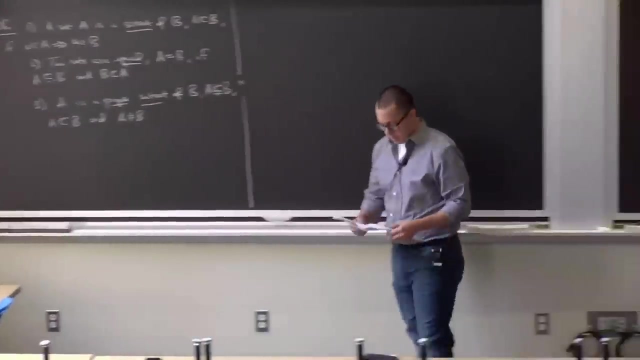 And A is a proper subset of B. if A is a subset of B and B does not equal B, OK, And we typically write that by A and with a dash going through a line underneath the C to signify that it's not equal. So think of it as not so less than or equal to, but not equal to is one way to think about it. 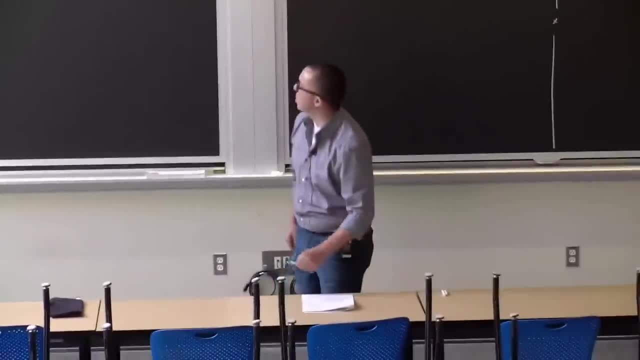 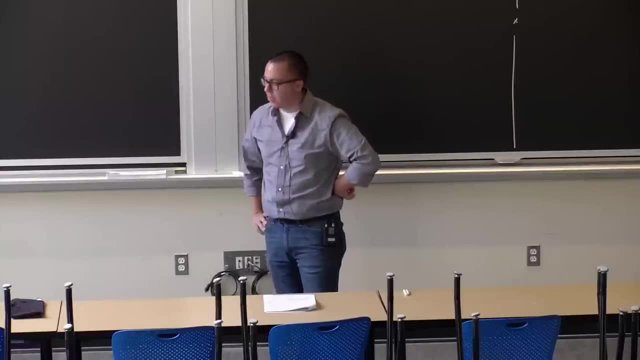 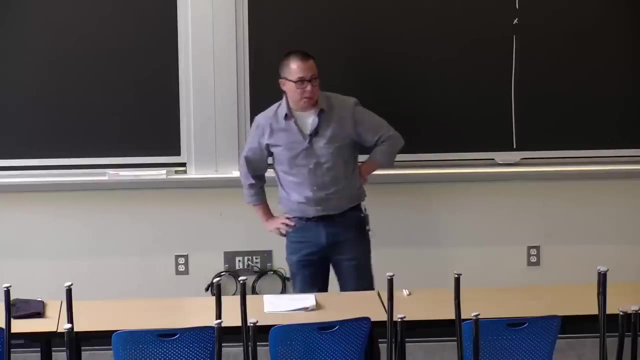 OK, So let me say something, since I'm now one, two, three definitions in. So definitions are a fact of life when it comes to math, In the beginning of any subject there's going to be a lot of definitions, because we have to have objects we want to talk about. 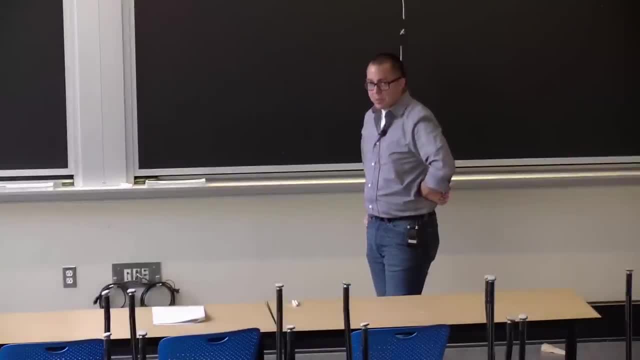 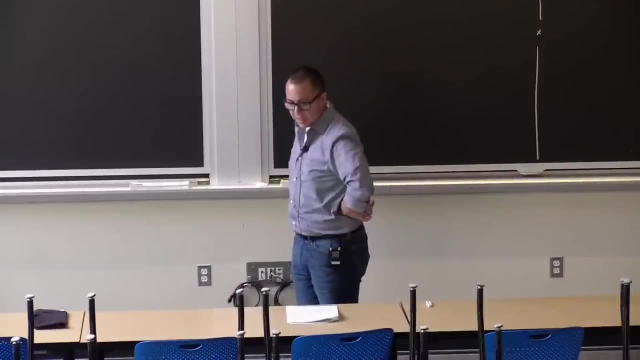 And we have to have these unambiguously defined objects. So it may seem like there's going to be a lot of definitions now, but this will last. We'll let up and we will start proving some theorems which are facts about these objects. 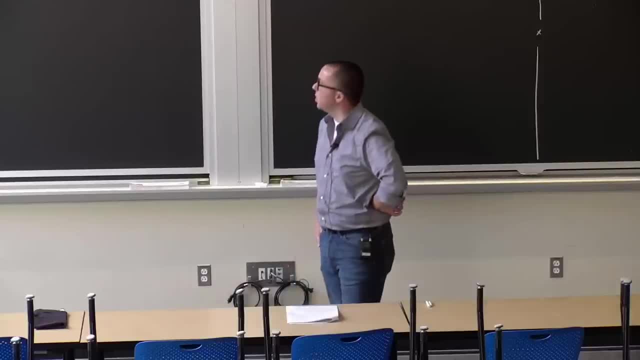 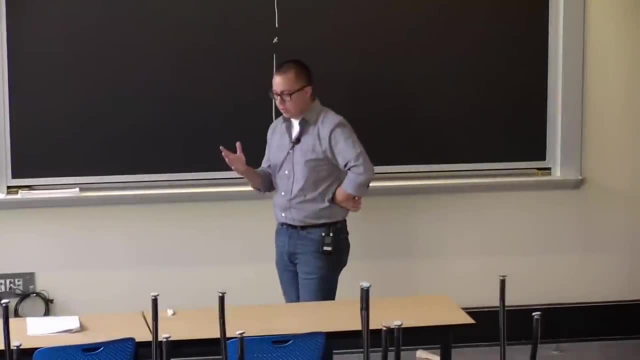 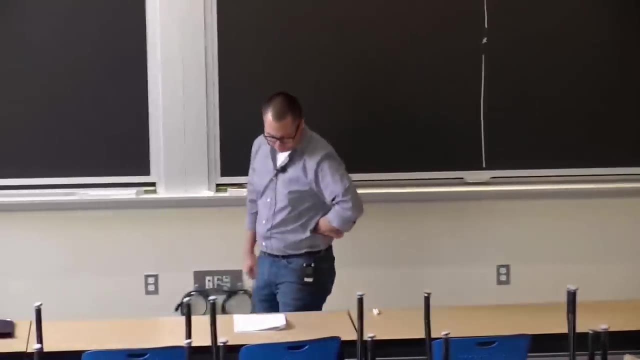 These are the things that we're really after. We're not really after just making up definitions. Definitions are meant to be a rigorous way of defining an object. we're interested in studying. We're interested in proving theorems facts about. OK. 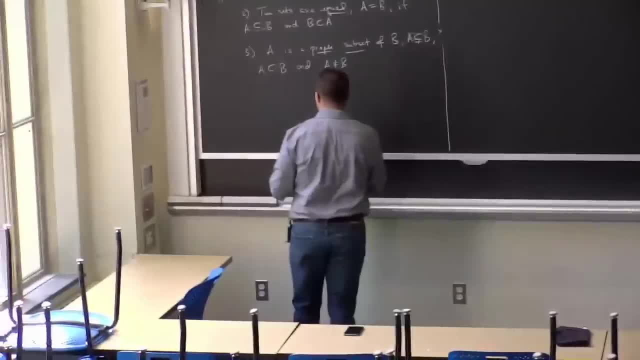 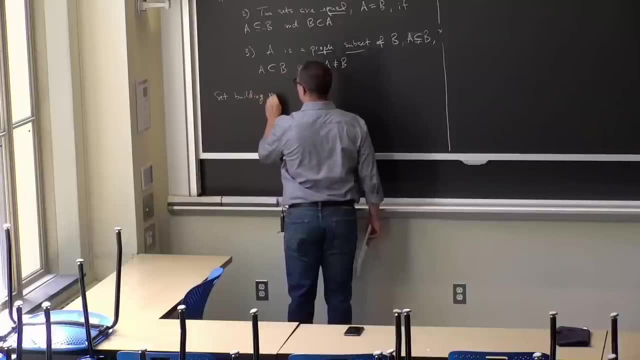 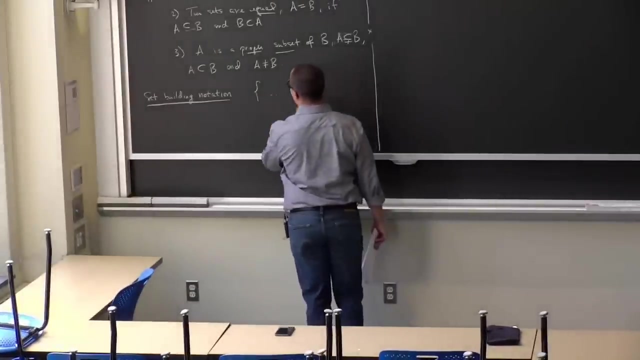 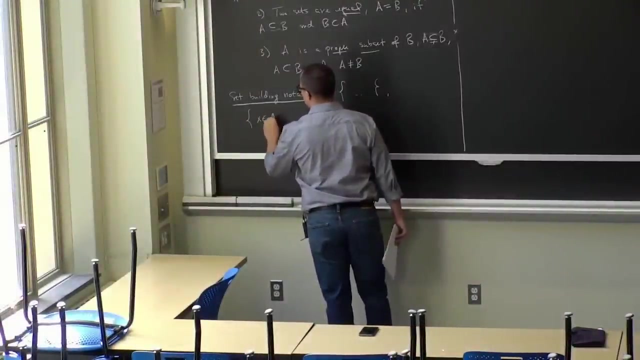 So OK. So again, a lot of this is just probably review. When we describe sets, we will use these braces and maybe list the elements in here, Or we will describe it as x in some set. OK, OK, OK. 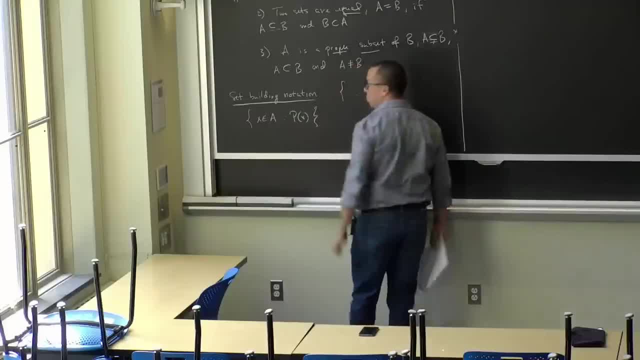 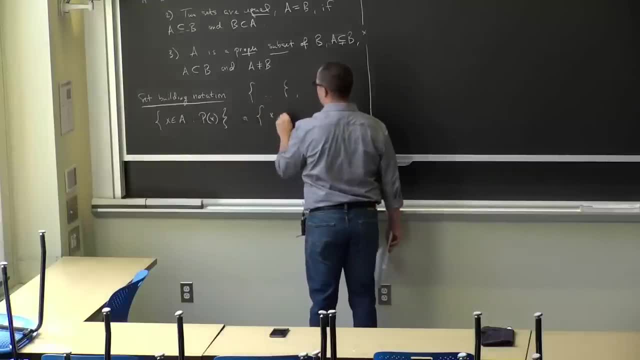 At set a satisfying some property p of x, Or we won't write this x in a part, We'll just write all objects x satisfying x as being an element of whatever universe we're in That satisfied property p of x. OK, 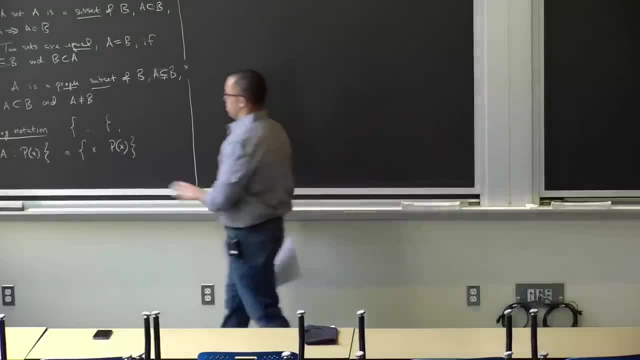 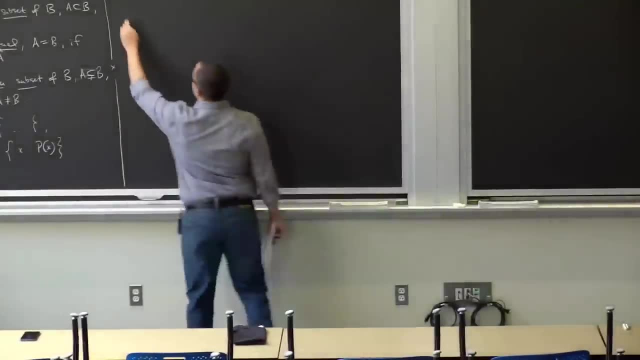 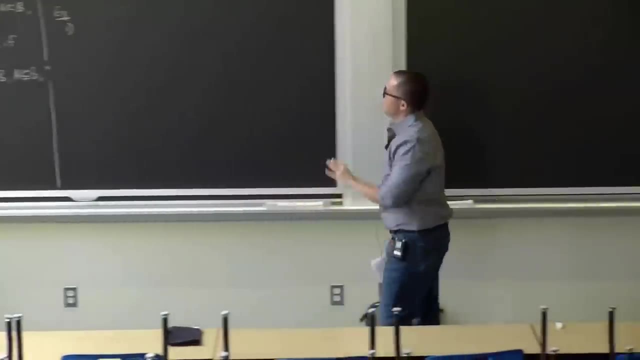 So Again this, you should read this as all x satisfying, satisfying property P of X. So the basic examples, and this is you should expect this, after kind of seeing any kind of non-trivial definition. If you were here I would ask. 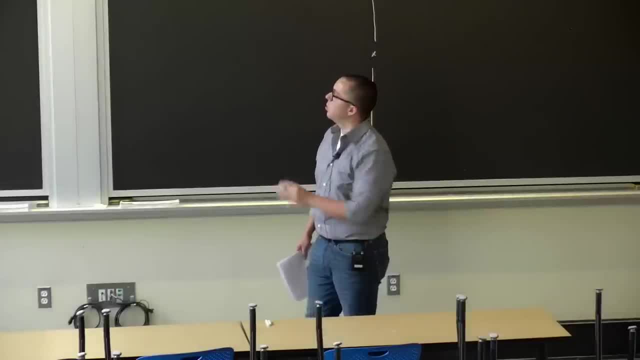 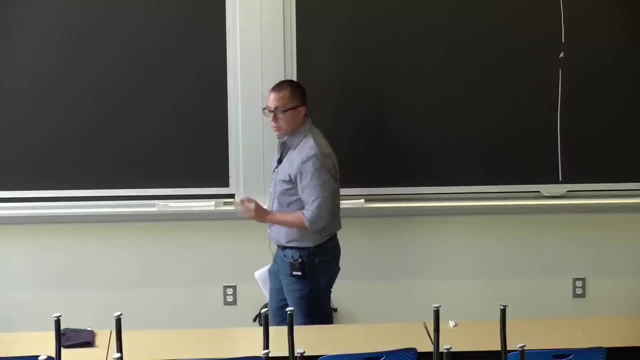 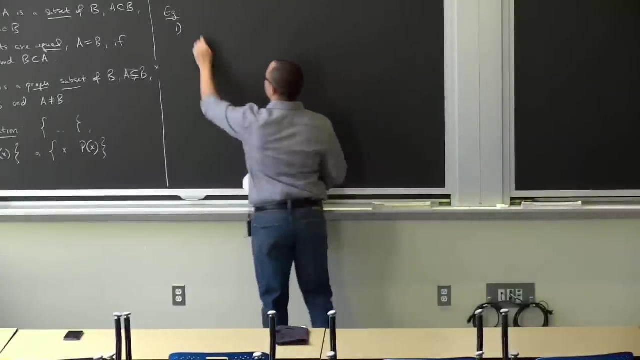 you to call me out, so I'll have to police myself. But after every kind of semi-interesting definition, you should see examples. okay, This is how you actually learn about these things, or at least digest what these things are. So we have the natural numbers, which. 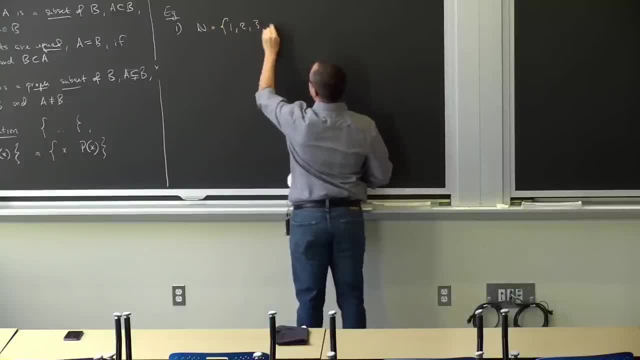 everyone's familiar with, since they started to count 1,, 2,, 3,, 4, and so on, We have the integers, which is 0, 1, minus 1,, 2, minus 2.. So all the natural numbers, along with their 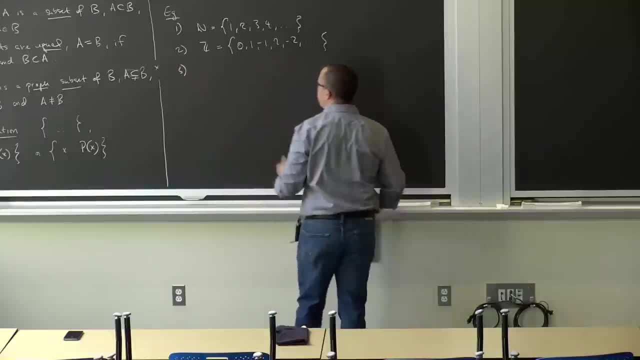 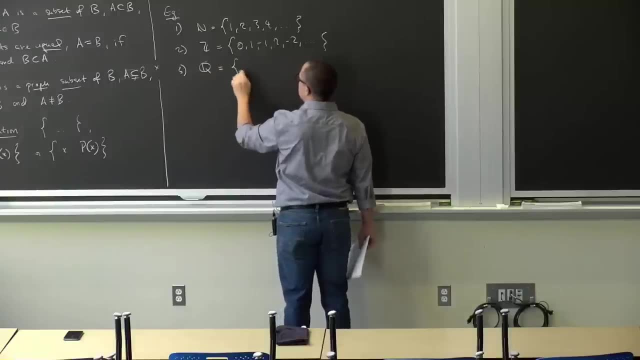 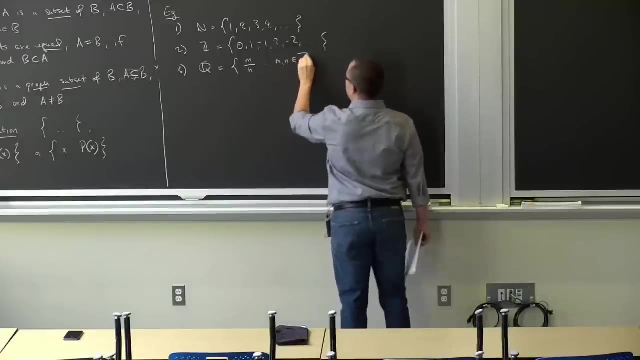 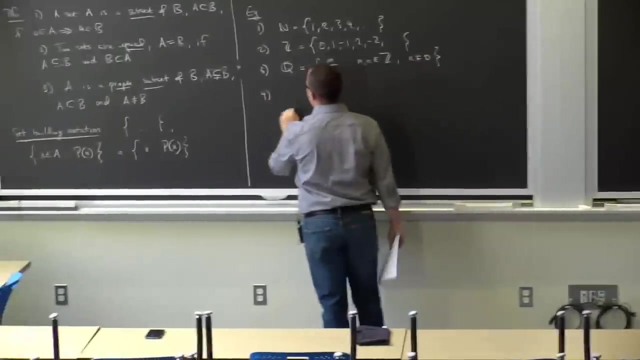 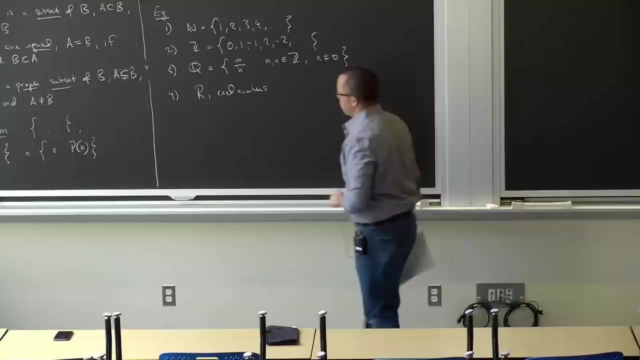 additive inverses. along with the zero element, An additive identity, We have the rational numbers, So this is written as M over N, such that M and N are integers and N does not equal to zero, And we have R, the real numbers. 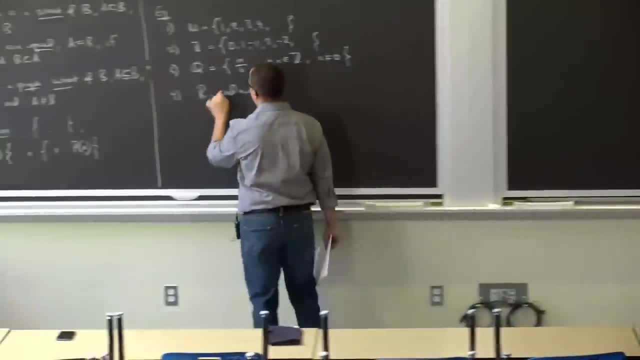 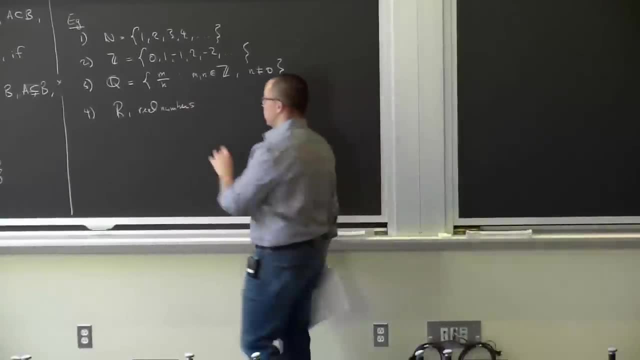 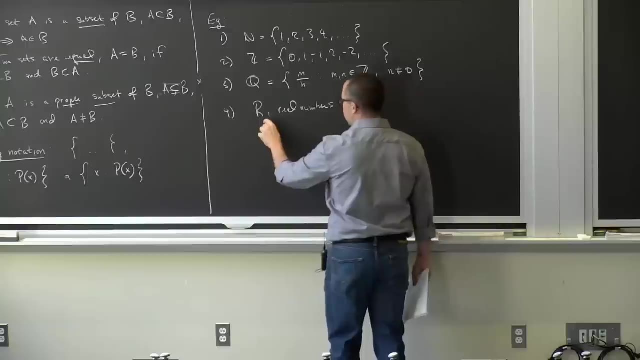 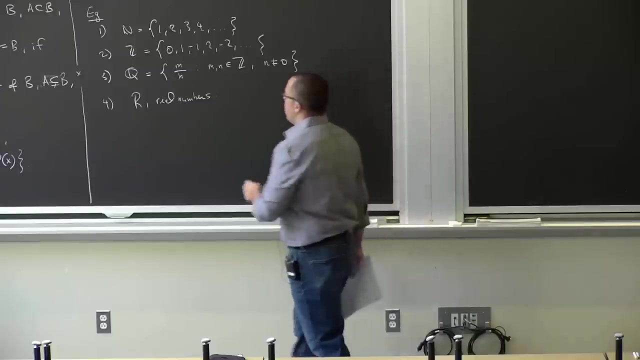 Okay, Okay, Okay. So we have a set building which I, as of right now, cannot actually write down what they are in terms of set building notation. In fact, this will be our first. goal of the course is to give a proper description or definition of what R actually is. But you 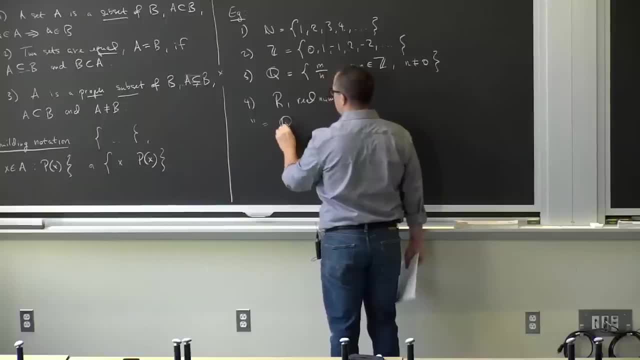 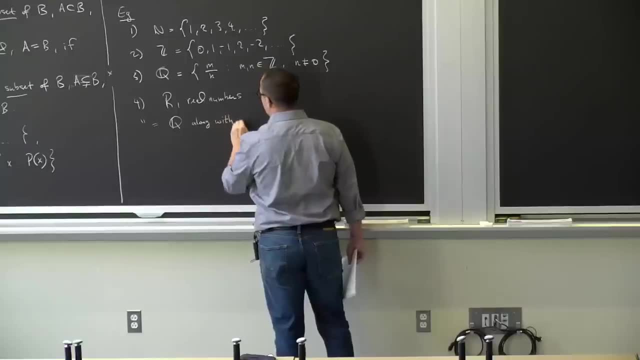 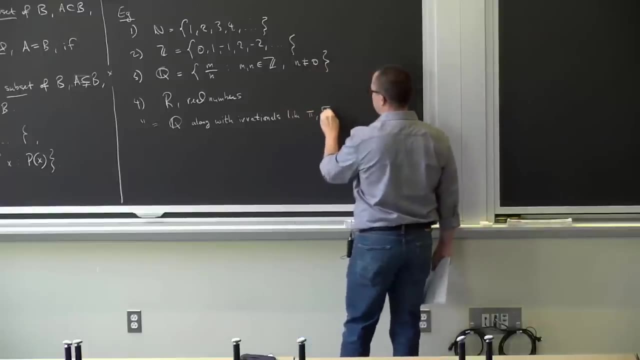 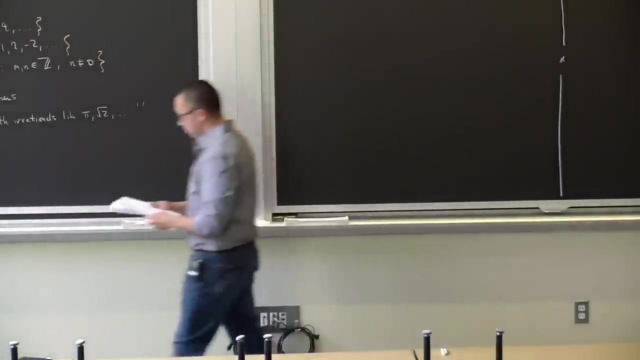 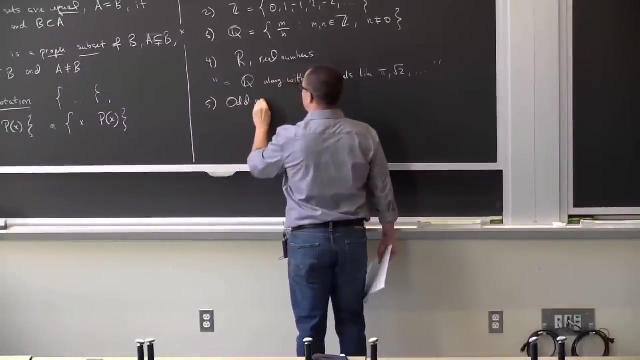 can think of this as so, So, as you did in calculus, as Q, along with so rationals and irrationals like pi 2 and these things. So this is fine to think about for now. So of course I didn't have to use these. 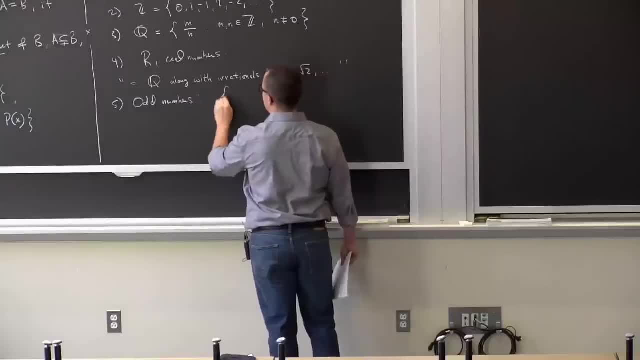 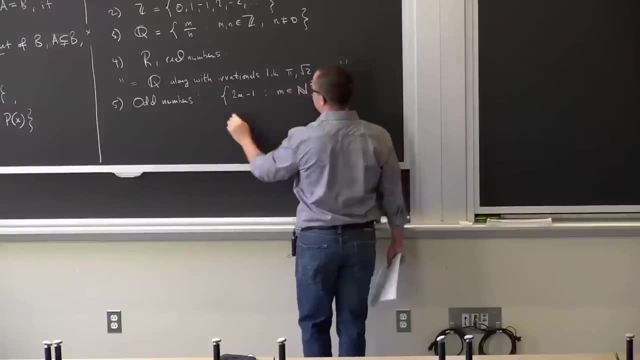 I could have maybe I'm interested in odd numbers- That's the set of numbers of the form 2m minus 1, where m is a natural number. So this is just 1,, 3,, 5, and so on. 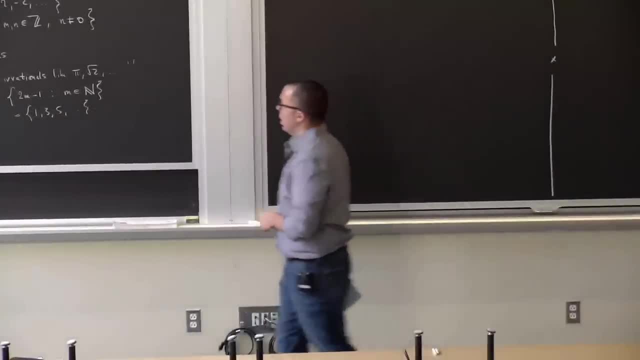 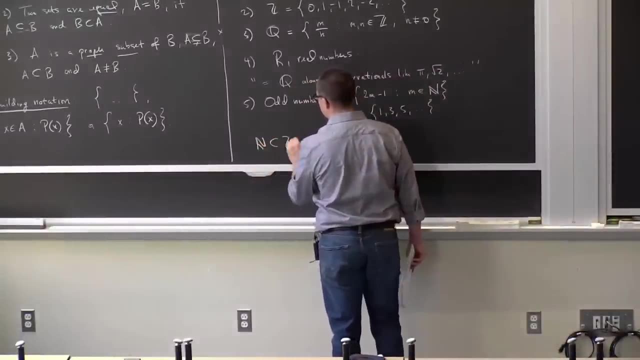 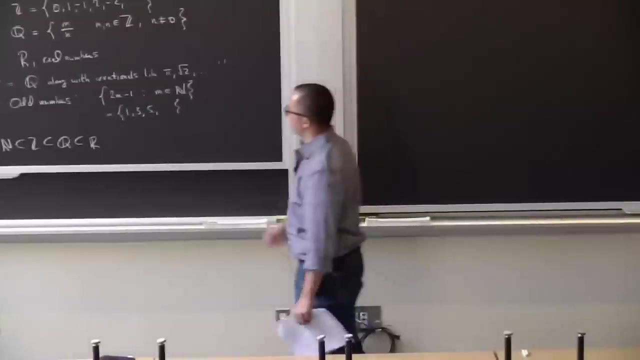 And so note that we have the inclusions- Natural numbers are contained in the integers, which are contained in the rational numbers, which are contained in the real numbers. And if you kind of look at the history of why these things were thought up in the first, 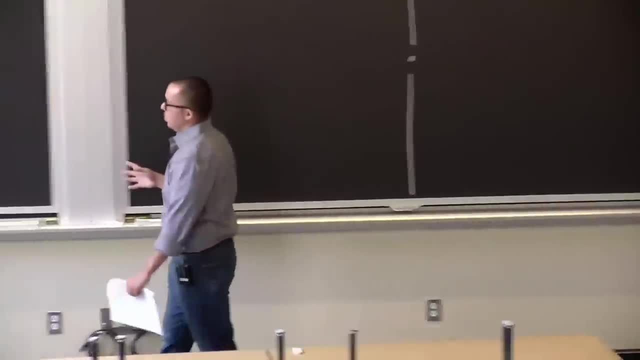 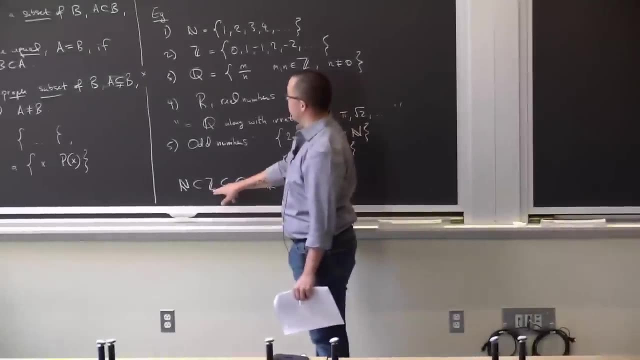 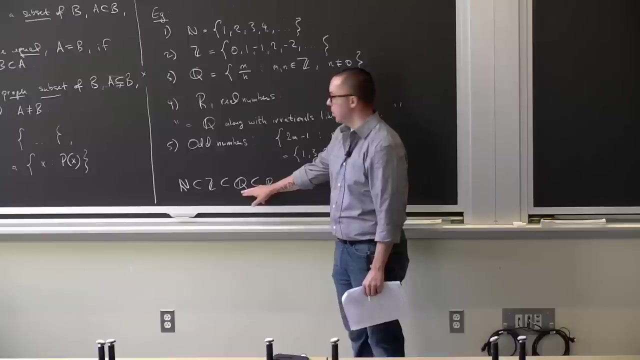 place. I mean they were thought up to solve kind of polynomial equations that you couldn't solve in the number system. before Integers were created because I could not solve the equation x plus 1 equals 0. in the natural numbers, Rationals were thought of because I could not solve the equation 2x plus 1 equals 0. 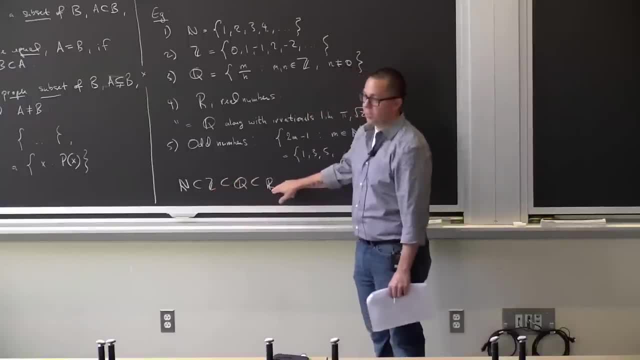 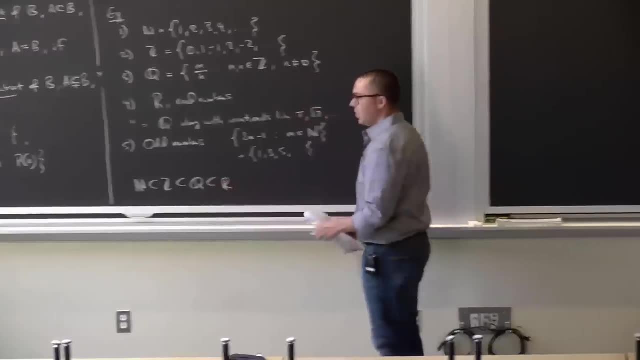 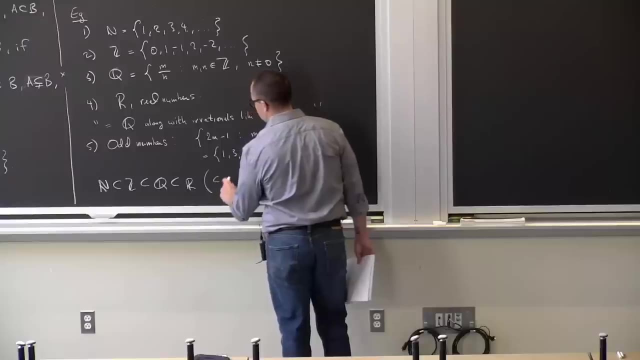 in the integers And the real numbers were thought of because I could not solve the equation x squared minus 2 equals 0 in the rational numbers. Now solve the equation x squared plus 1 equals 0 in the real numbers, which led to the creation. 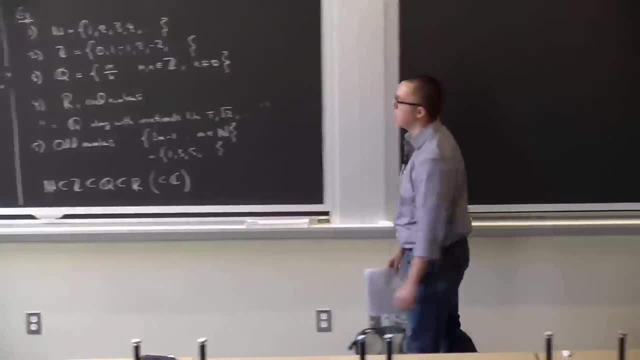 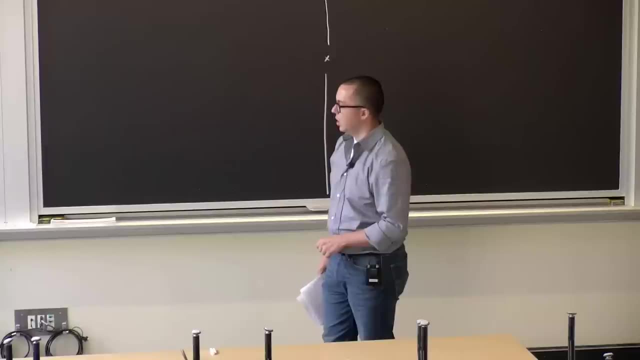 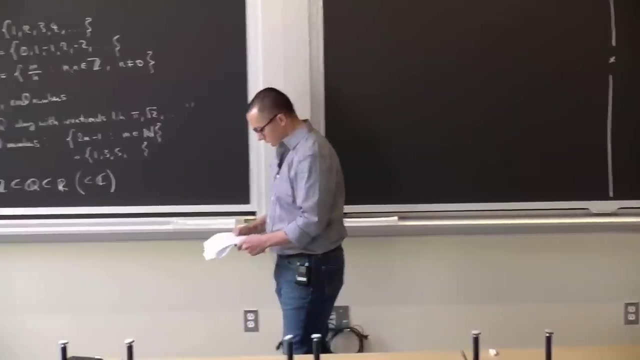 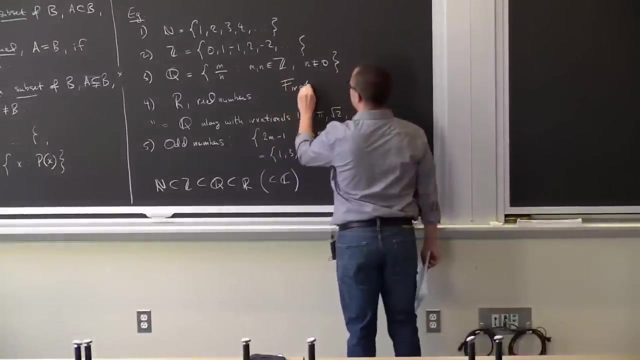 of complex numbers, but we will not deal with complex numbers in this class, although, hopefully, if you keep studying analysis, you go on to complex analysis, which is really a beautiful subject of study to this day. so, as I said, let me write this here: our first goal: real. 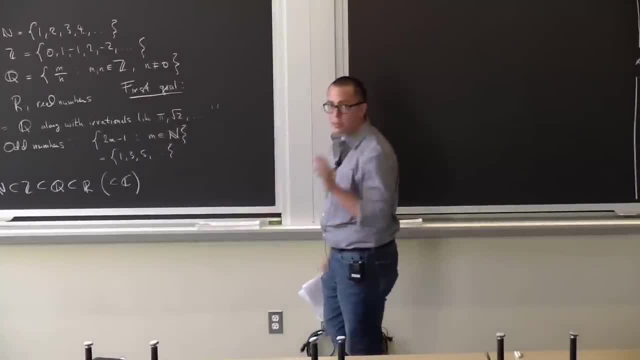 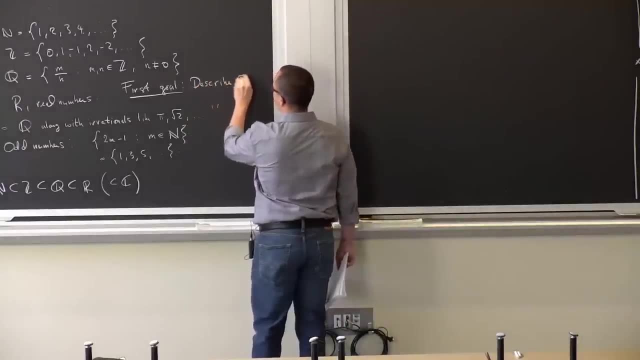 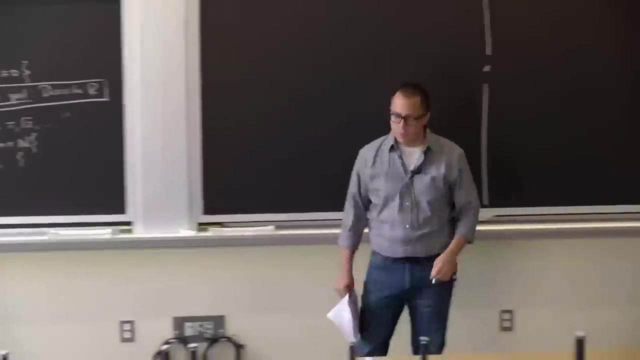 goal of the class, and this is something to keep in mind. we're not going to do it right now. our first real goal is to describe what r is. I mean if we're going to be proving statements about the real numbers, functions of real 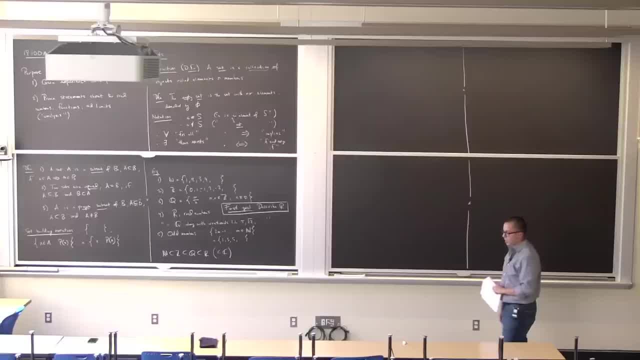 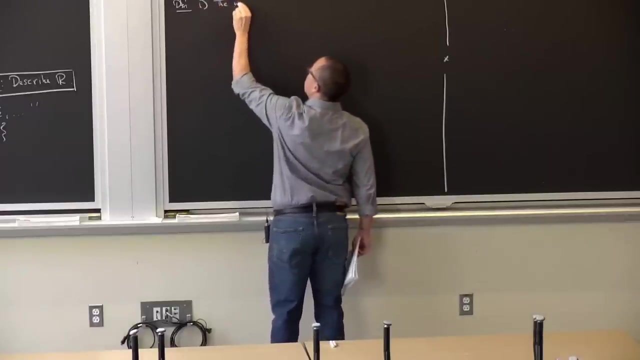 numbers and limits, those limits that you learned in calculus, then we have to be able to really describe what we're starting with the real numbers. Okay, so let's get back to sets, to our review of sets. Okay, So there were some examples. we have a few more definitions: the union of two sets A. 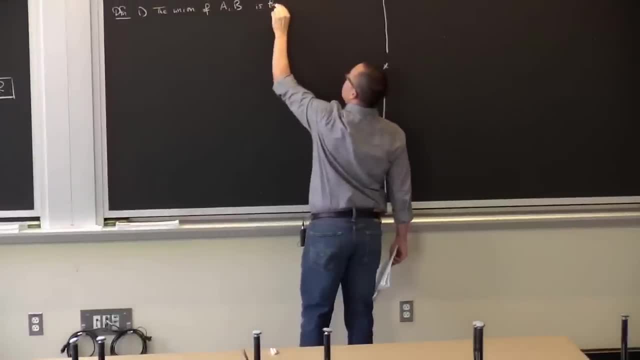 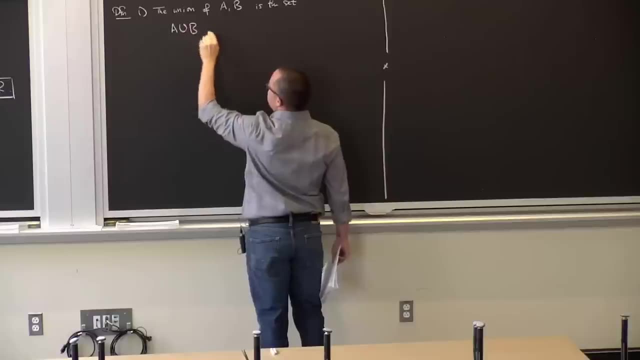 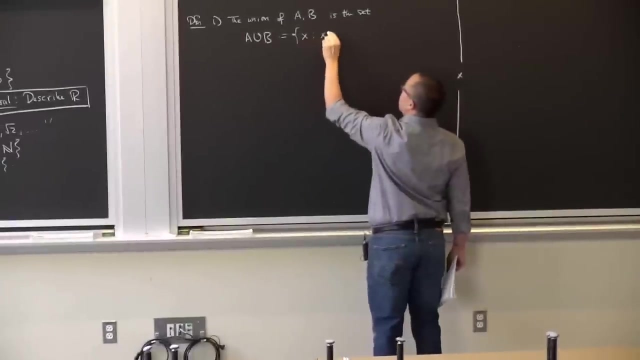 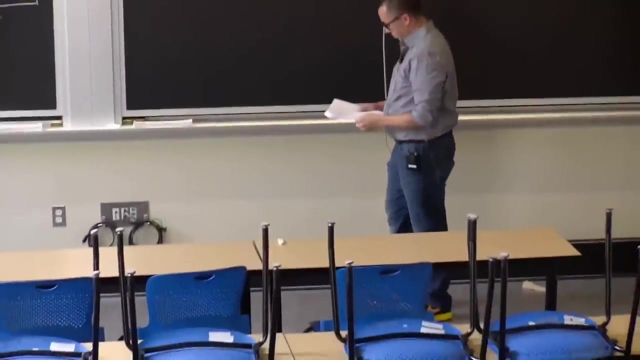 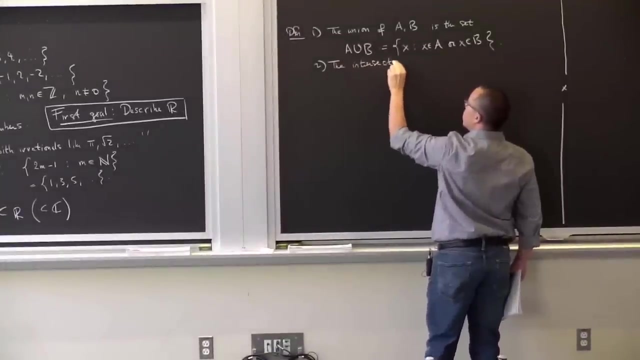 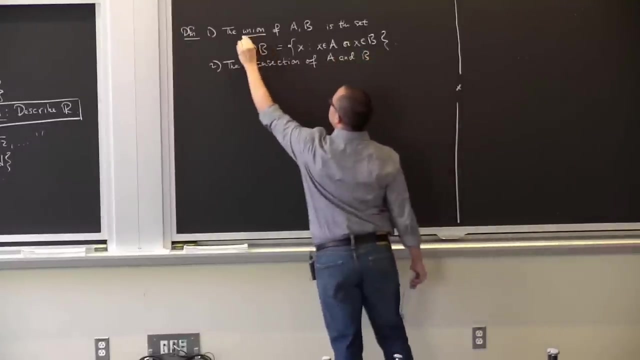 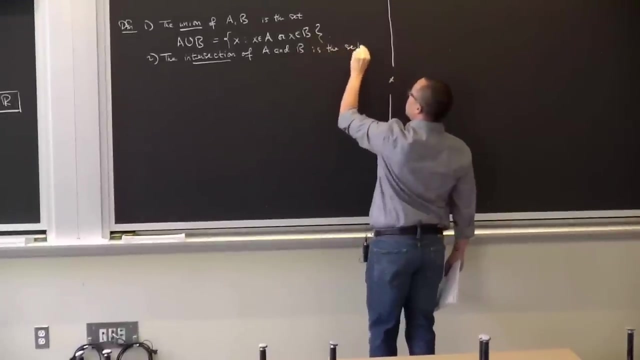 and B is the set which we write, so this is how we denote it: A, U, B. this is the set of all elements: x, X is in A or x is in B, The intersection of A and B. so this was defining the union, this was defining the intersection. 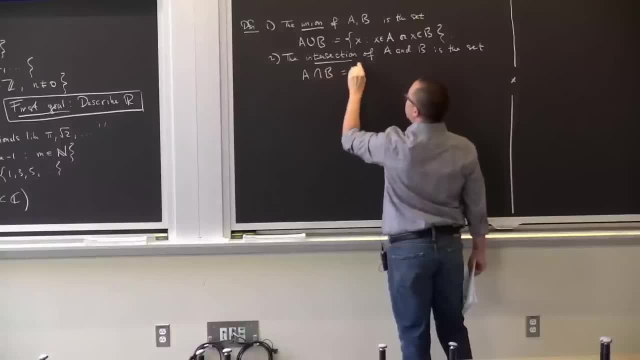 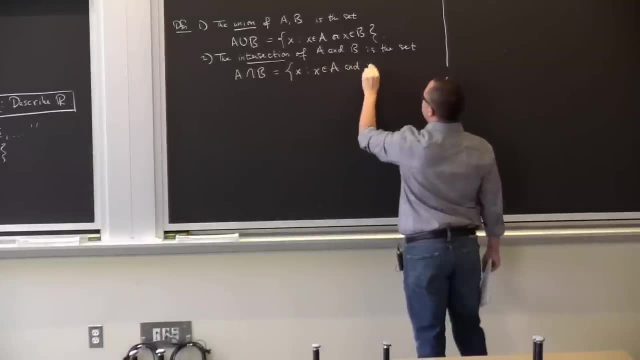 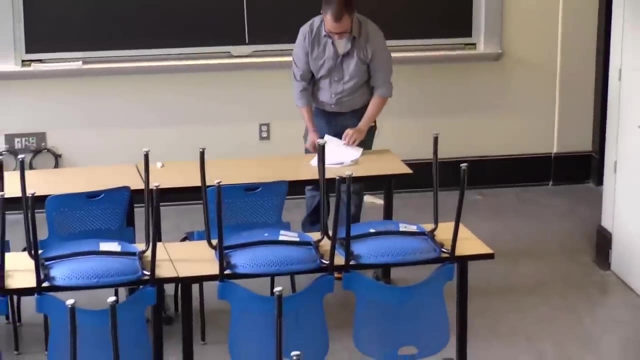 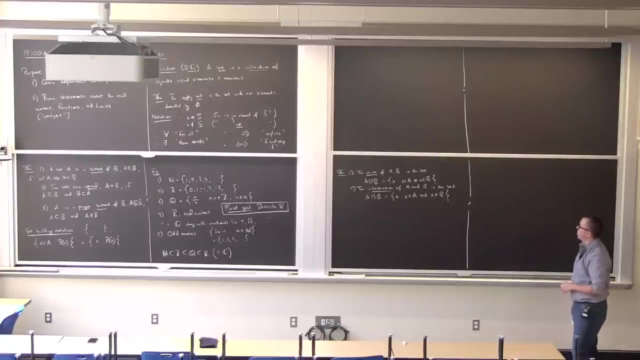 is the set, Okay, And this is the set of all x's, so that x is in A and x is in B. So the union is: take all the things from A, take all the things from B and put them together. 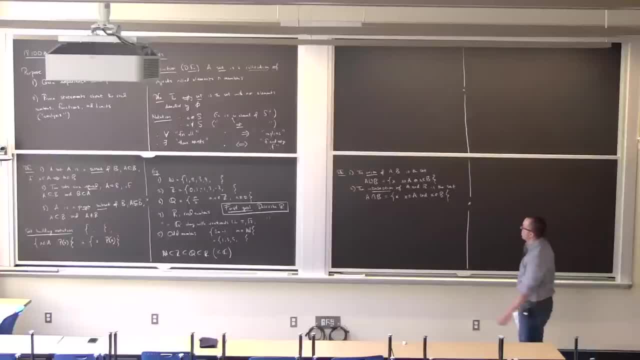 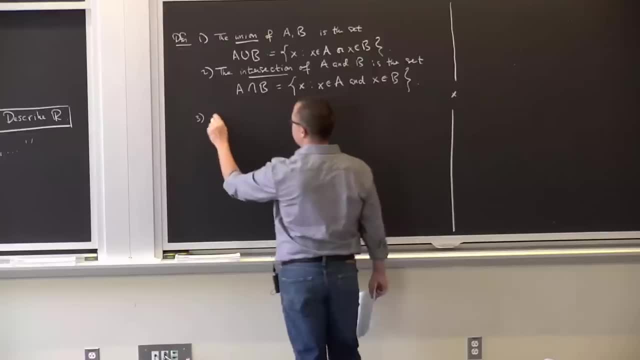 in one big basket. The intersection is just take the things from A, take all the things from B and put them together in one big basket. Okay, So these are the things that A and B have in common. Okay, So the thing, the set difference of A with respect to B is the set. 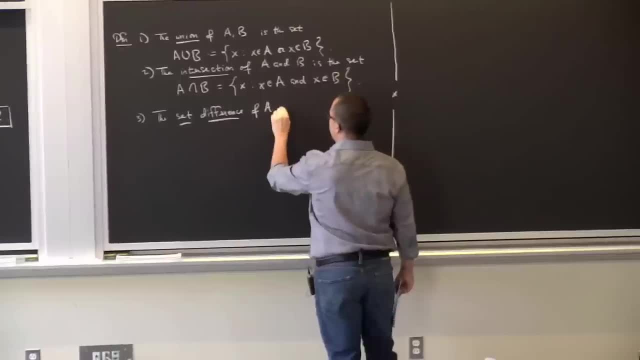 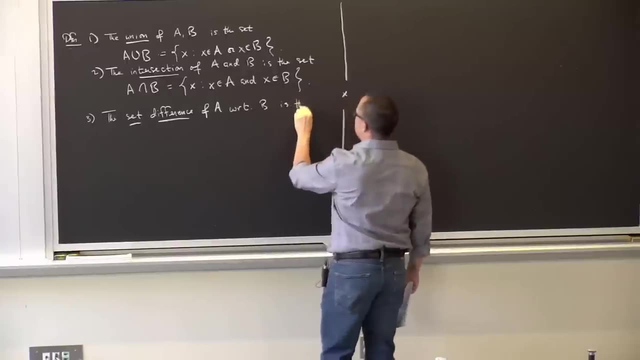 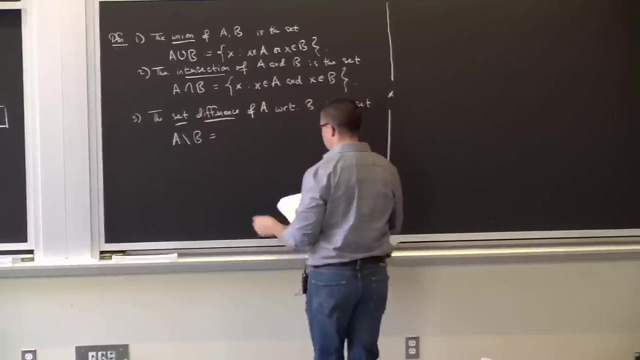 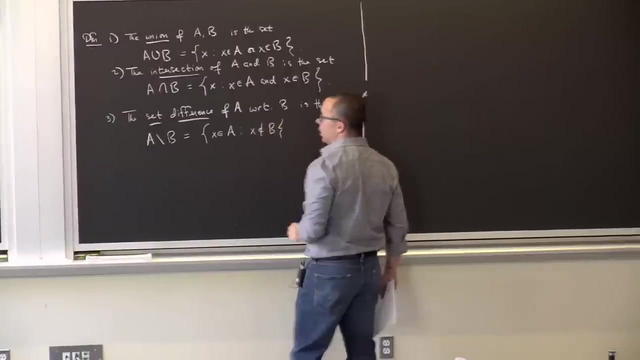 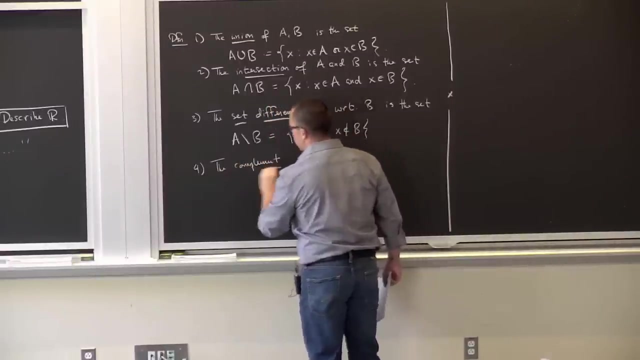 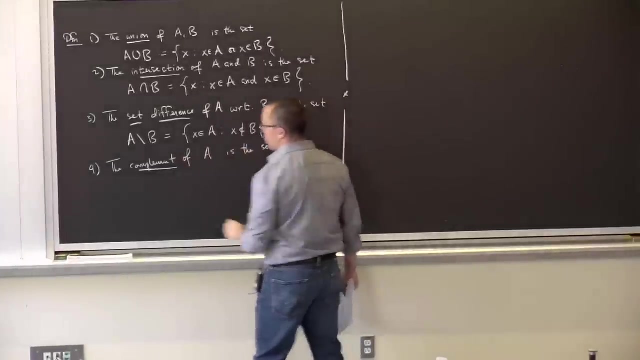 the set. the thing is different, but we will do it together, Okay So, Okay. Okay, A backslash B: this is the set of all elements in A, such that X is not in B. The complement of A is the set A. 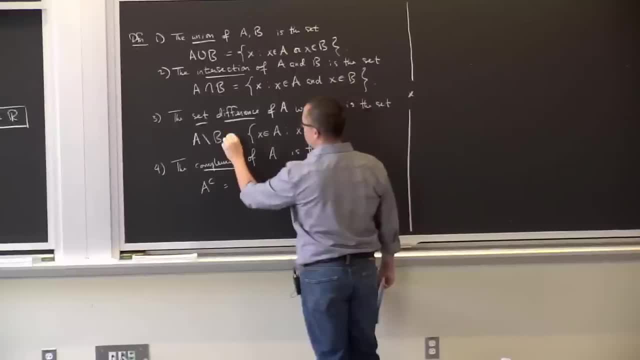 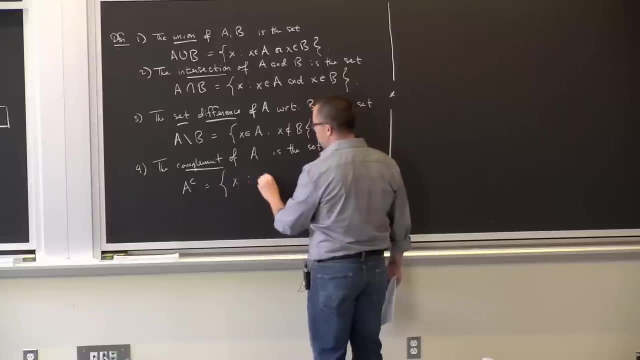 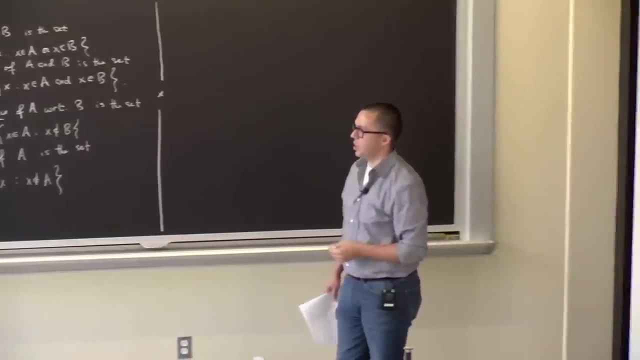 So this is how I'm denoting the set Kind of. the next part is how I'm defining this set. This is a set of all elements in our universe that is not in A, And when I say universe I don't mean this universe necessarily. 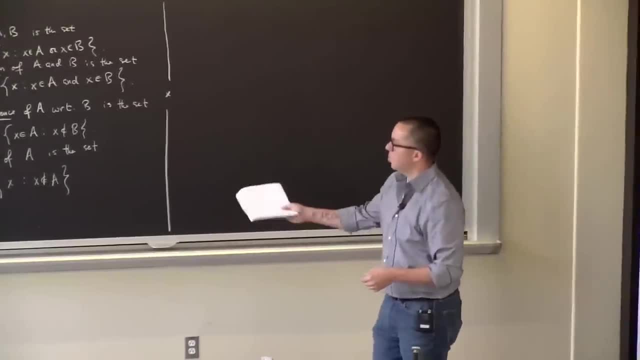 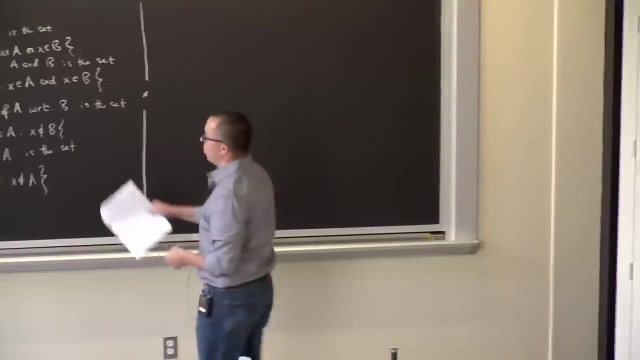 I mean, if we're looking at subsets of R, the complement is generally with respect to R, Or if all of our sets are subsets of Q, then our universe would be Q- the rationals- And we're taking the complement in there. 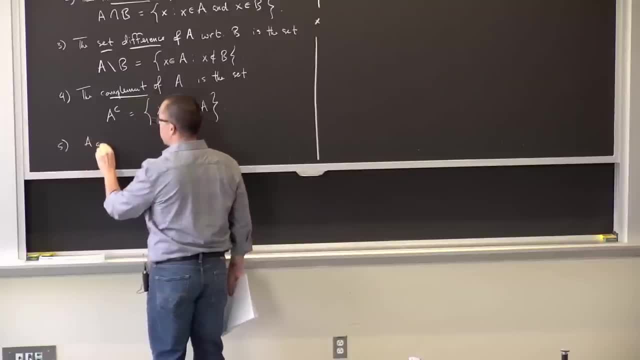 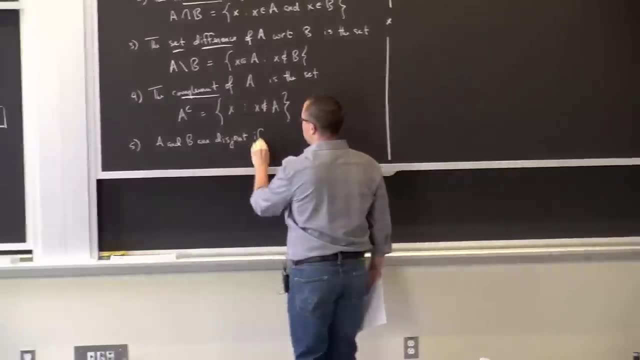 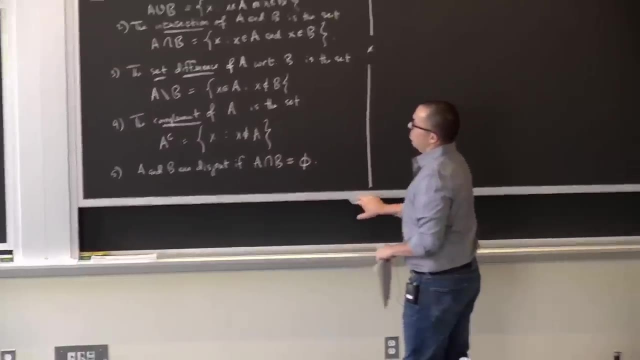 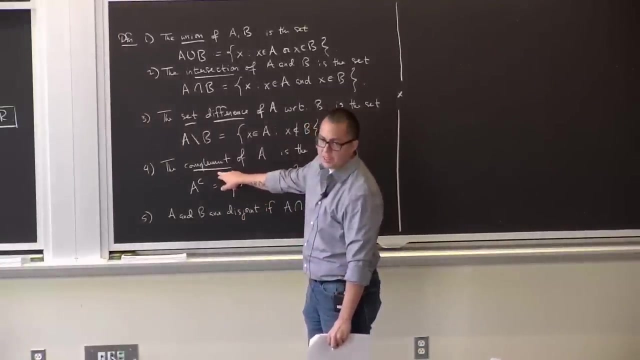 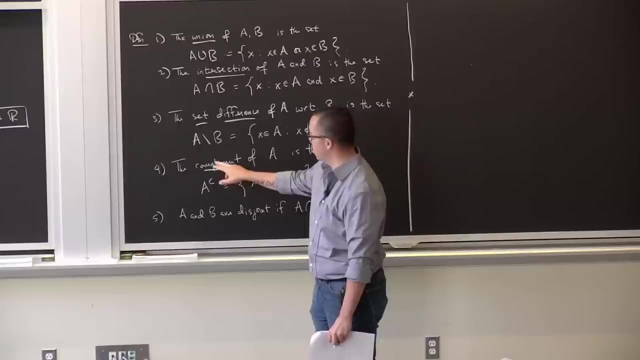 Two sets are disjoint- Disjoint If their intersection is empty. So it took me quite a long time to figure out. this complement has an E in the middle as opposed to an I as in the complement you would give a friend. I had to do a lot of spell checking in my thesis when my advisor pointed that out. 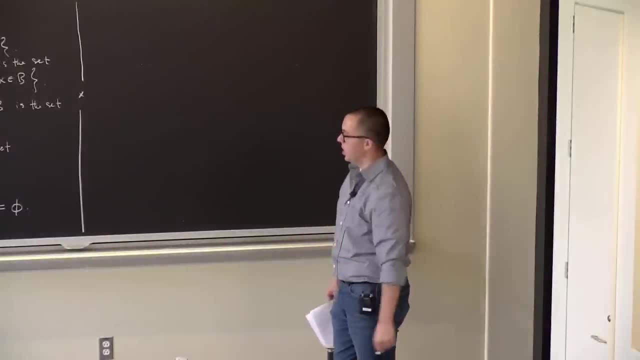 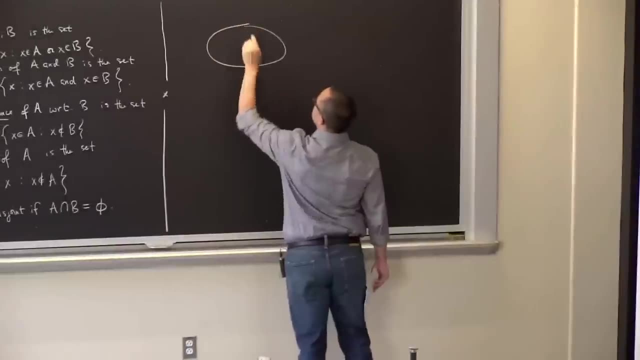 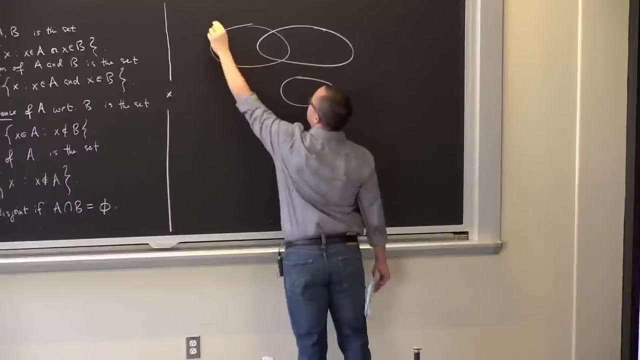 So this is just something to keep in mind. This complement has an E in the middle of it. Okay, So Let me just kind of draw a quick picture. So this blob over here is A. This is a set B. This is a set C. 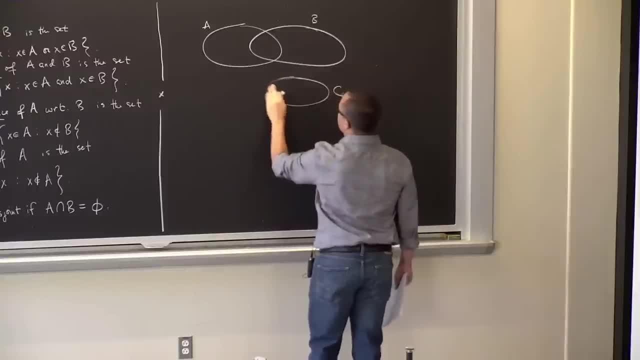 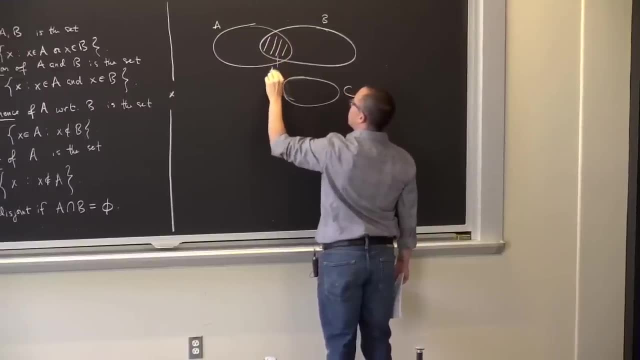 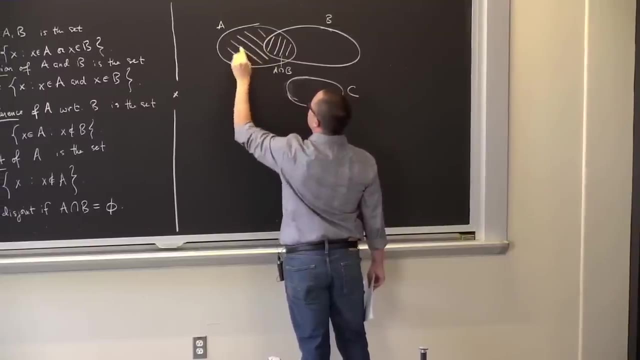 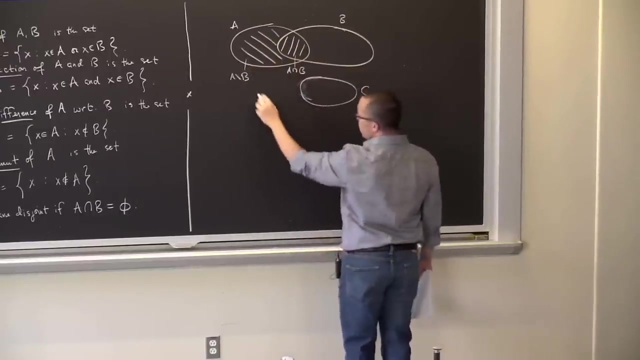 In fact, let's make this a little more. Okay, Let's keep C there. Then what I have here, that's a intersect B. This bit over here with the intersection is B. Okay, lines going this way, but not including this. This is a takeaway B, a backslash B, and 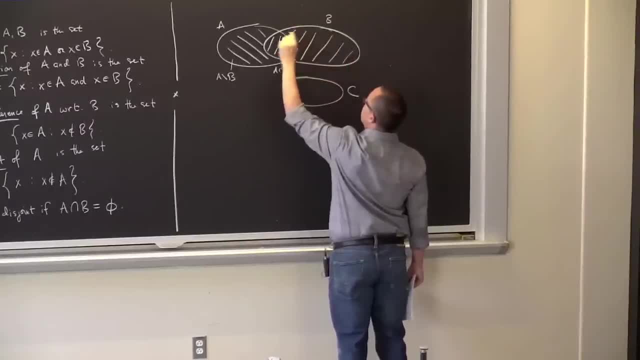 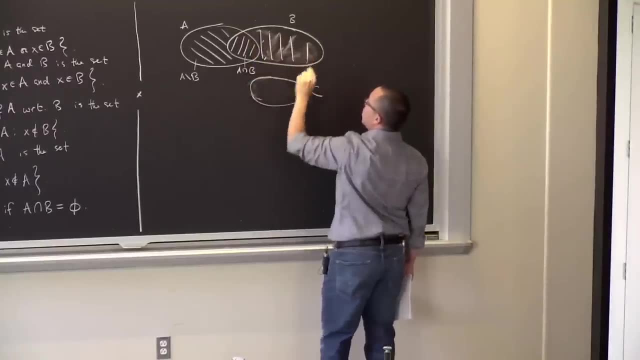 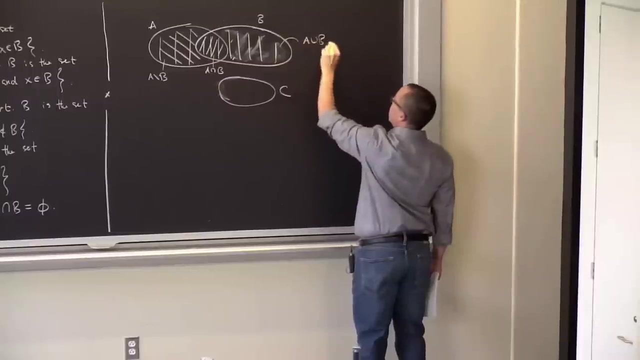 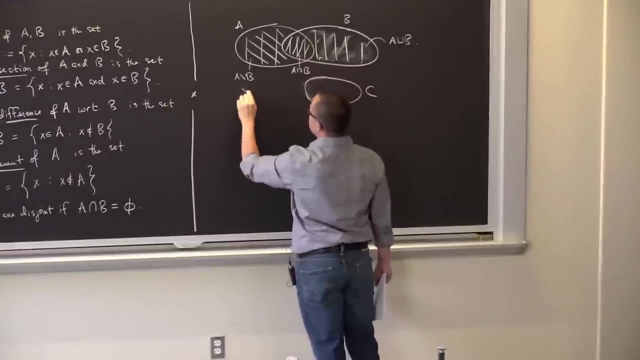 okay, so that was not meant to be along the same direction as this one. so let's go vertical and everything with a vertical line is a intersect B. okay, So a backslash has the lines going this direction. a intersect has the lines going this direction. 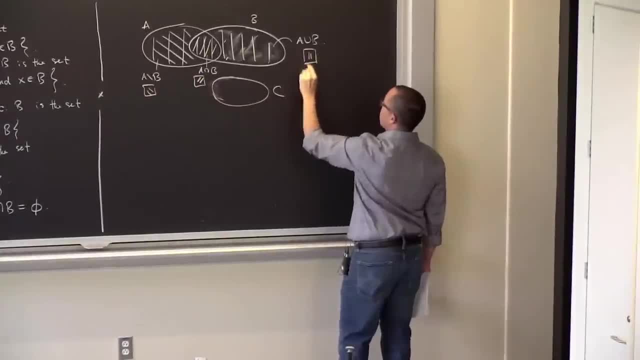 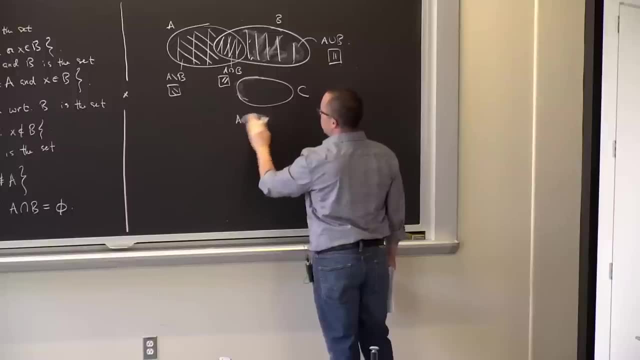 a union. B has the lines going vertical and C is way over here, not touching any of A and B. so A is going to be on the other side and A is going to be on the other side and B is going to be on the other side. 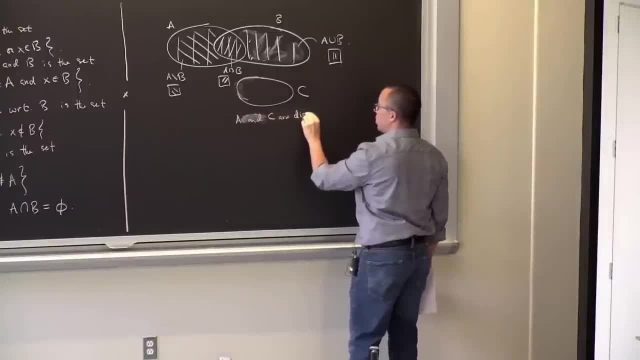 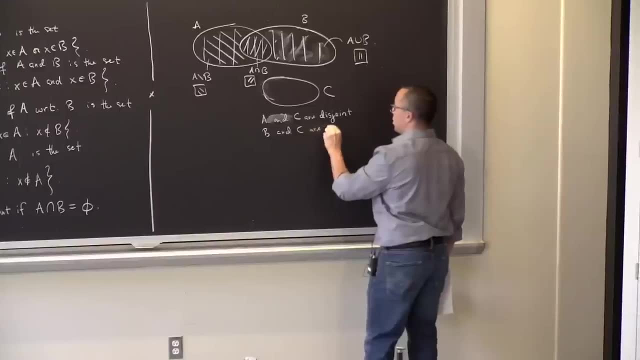 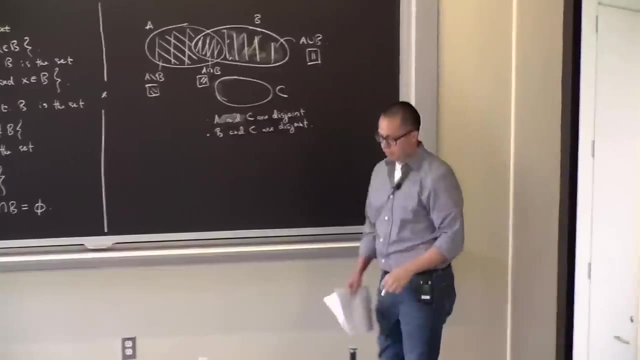 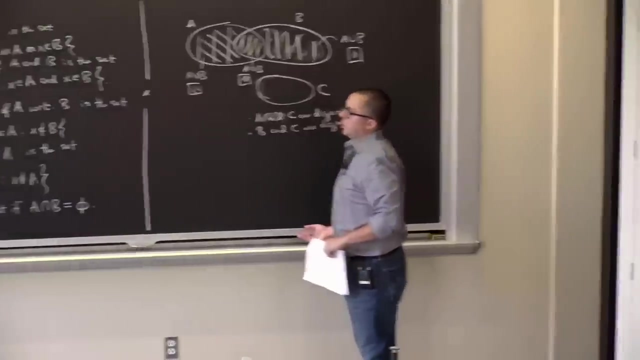 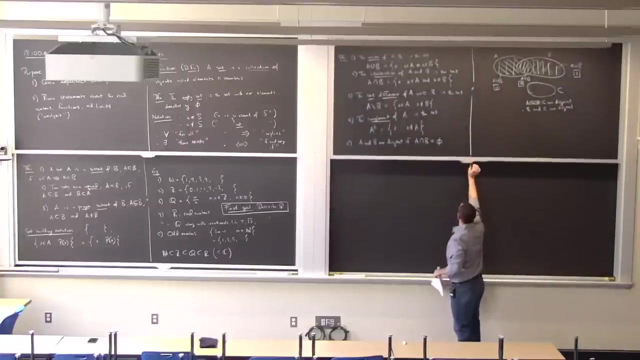 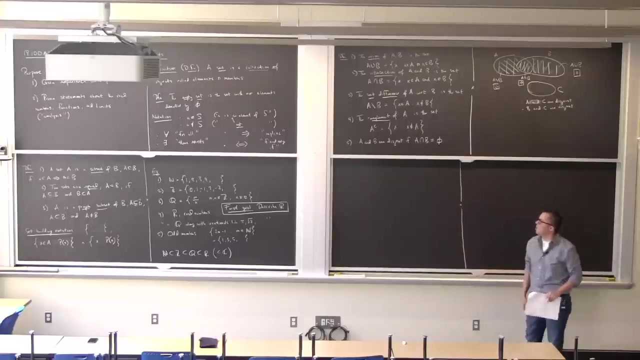 A and C are disjoint, and B and C are disjoint. okay, They have nothing in common. Okay, so this is a lot of definitions. We have not proven a single statement yet, so it's about time we do. This is probably one of the most basic. 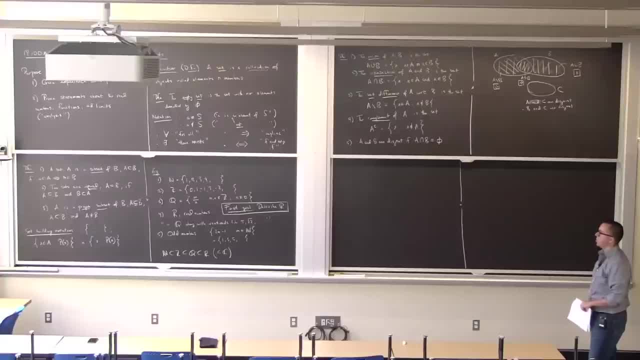 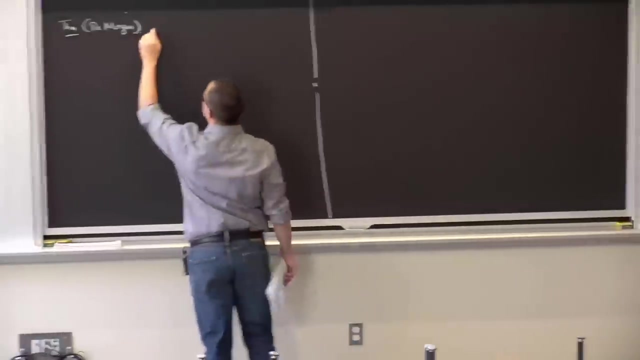 theorems one can prove at the start of a real analysis class or any class about proofs. This is, you know, analogous to when you write your first hello world program in a programming class. so let me state the theorem, which is De Morgan's laws, and the statement is the following: 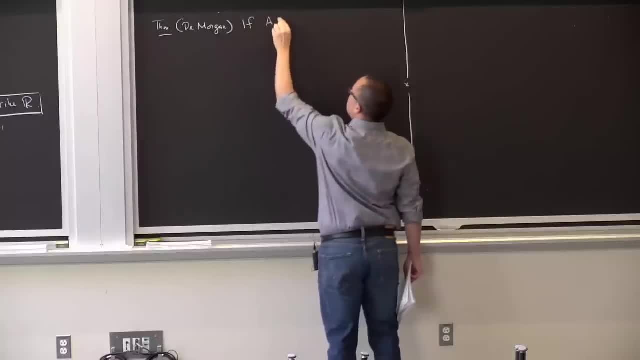 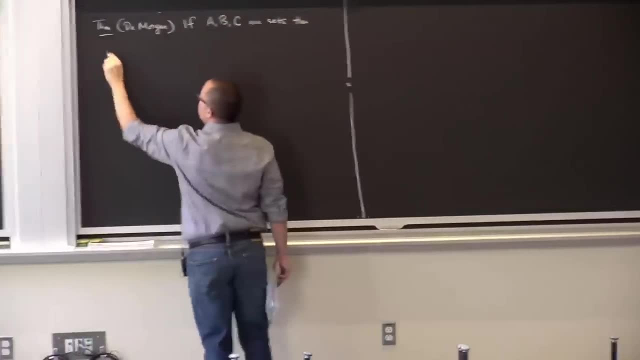 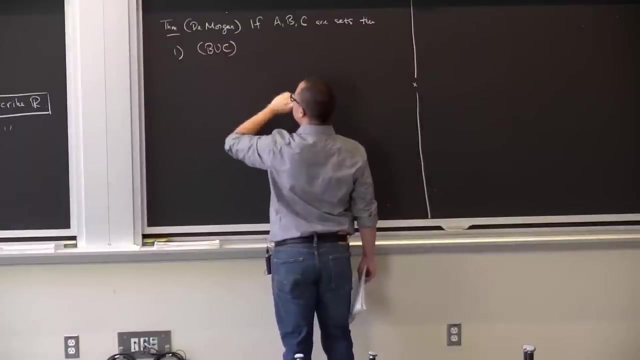 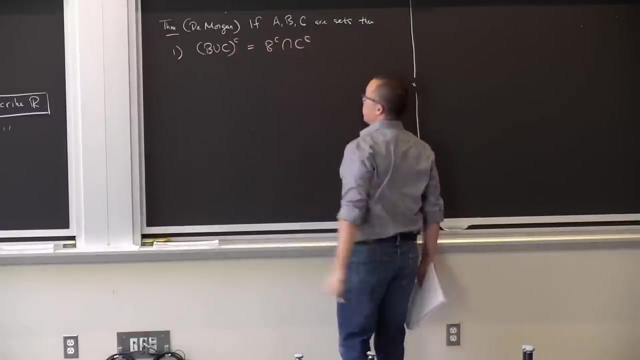 So if A, B, C are sets, then I have several things I can say: The union of B and C taking their complement, this is the intersection of the complements. so the complement of the union is the intersection of the complements. 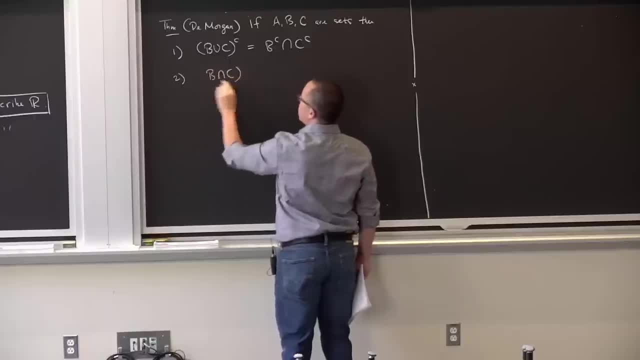 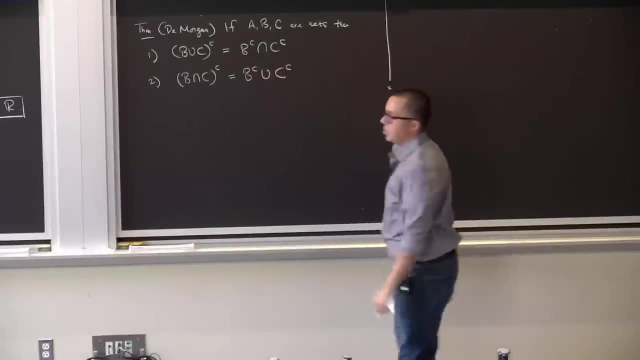 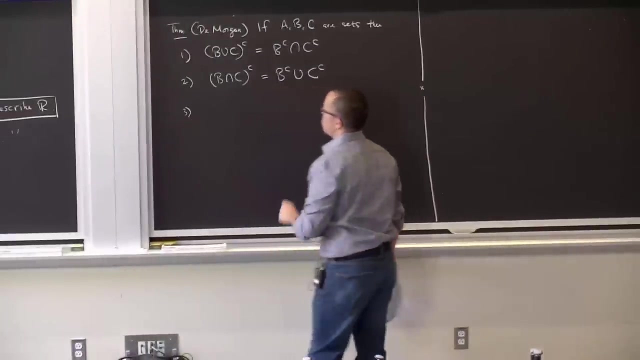 If I take their intersection and take the complement, this is the union of the complement. so the complement of the intersection is the union of the complements. Now, these are complements, meaning in some sense taking a set difference with respect to the entire universe. 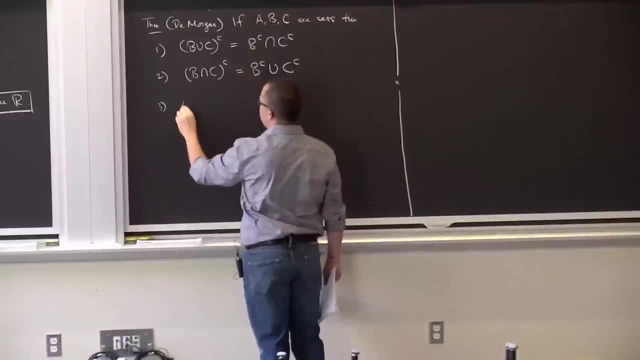 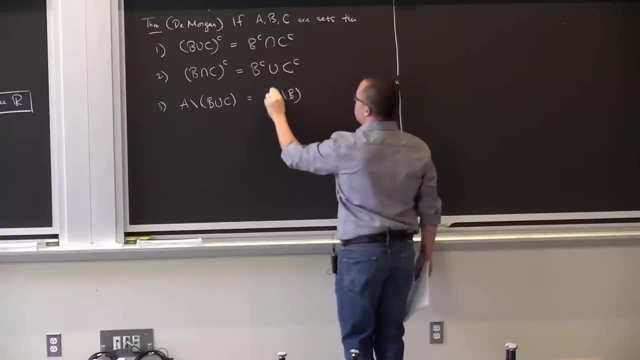 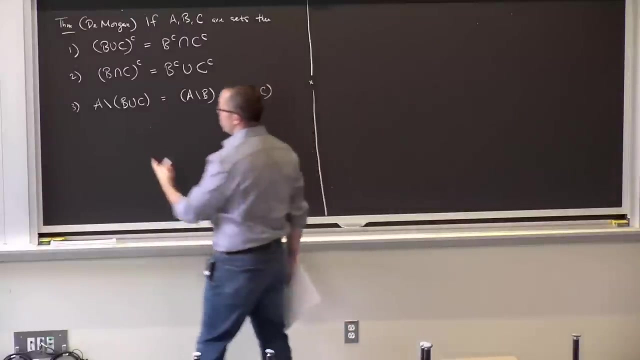 but I can make these things relative to some set A, So A take away B, union C. this is the same as A take away B intersect A take away C. Really again, this is- you should think of this as a special case of one. Really again, this is- you should think of this as a special case of one And again because of what the displacement tool has. JONATHAN KAVANAUGH also mentioned the Dienst regiment usually comes up to this solution. notice that the principle weirdness is esa. Here in the inverse denominator, you could basically have 1, 0 Jones. so there is no vision of 1, 0 Y, This little flappy 1, 0, 1, 1 Y, 0 Y, 1 O, 1 A, 0, 1 C. 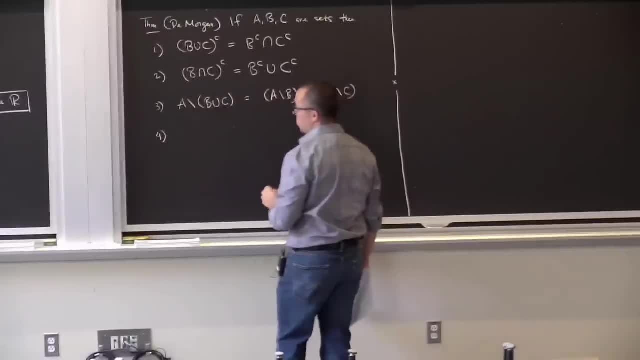 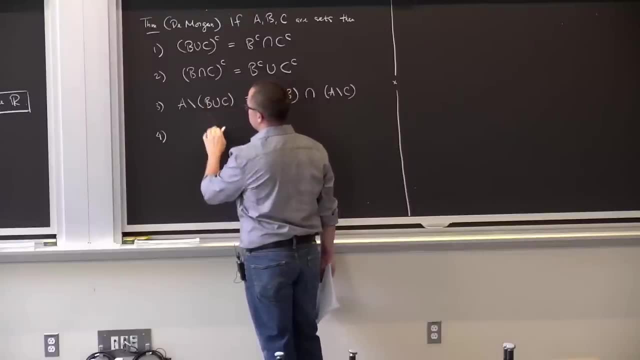 This little flappy: 1 0, 1, 1 2018 k, or at least, if you were to write the proof- I'm not going to because it's all going to be contained in the first two- then you would see it's really just a proof of this guy. 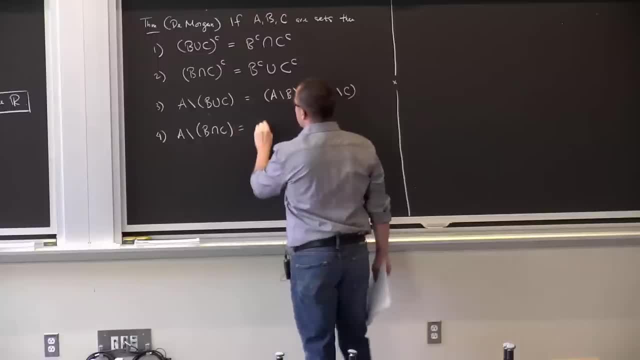 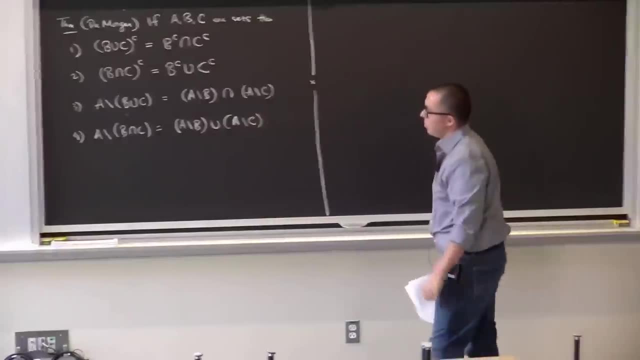 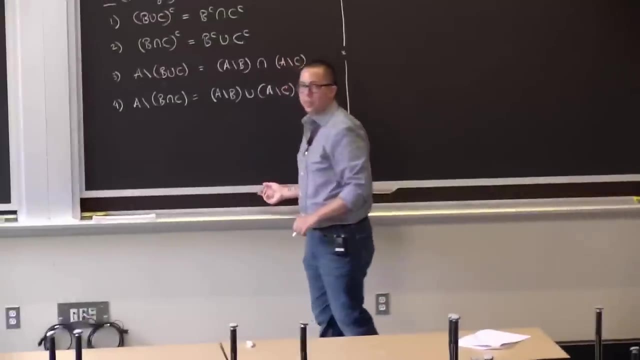 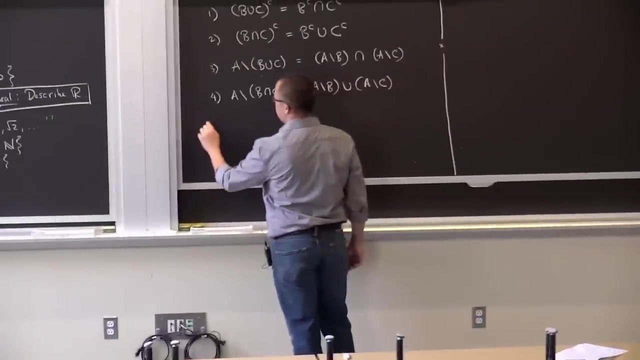 A take away B. intersects C equals A take away B, union A take away C. Okay, Okay, so again for a quick refresher about logic, I would look at the appendix of the textbook In general. so let me make a few remarks before we move on to the proof. 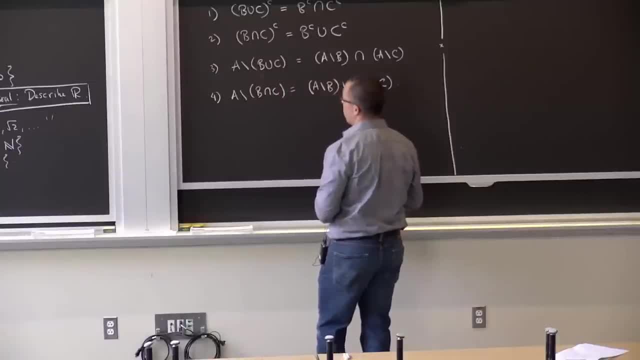 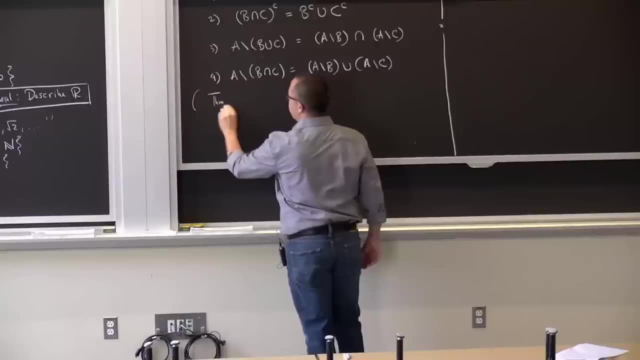 about typically how this is going to look. So this is some remarks. Typically, a theorem is a statement. It's a statement of the type P implies Q. Let me write this out in English: If some statement P holds, then Q. 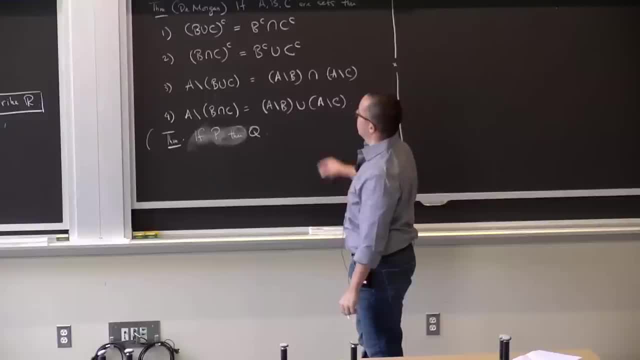 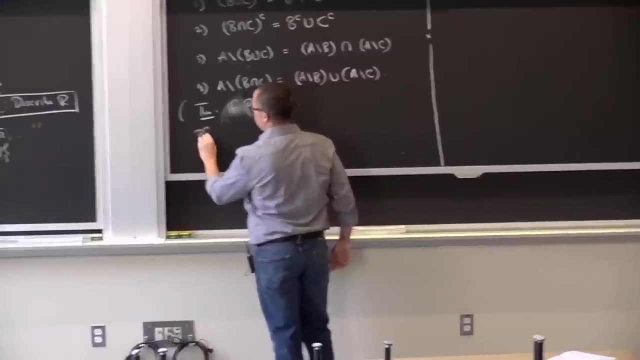 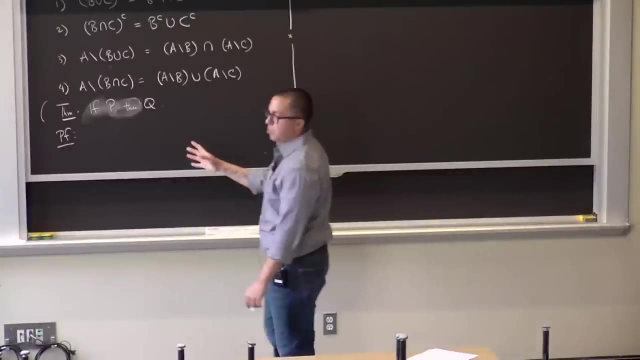 For us it's: if I have any three sets, then I have these equalities between these operations of sets. So the general structure, you'll see, of the class is: I have objects which I define unambiguously. I want to prove theorems. 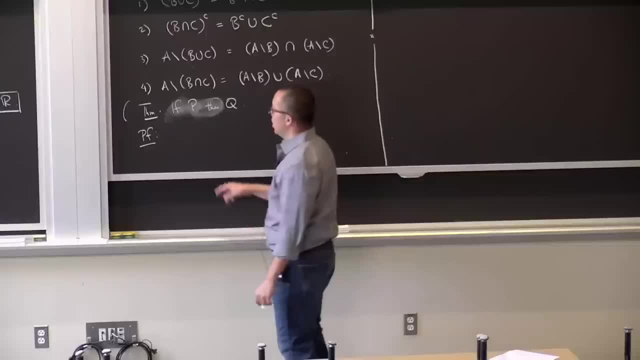 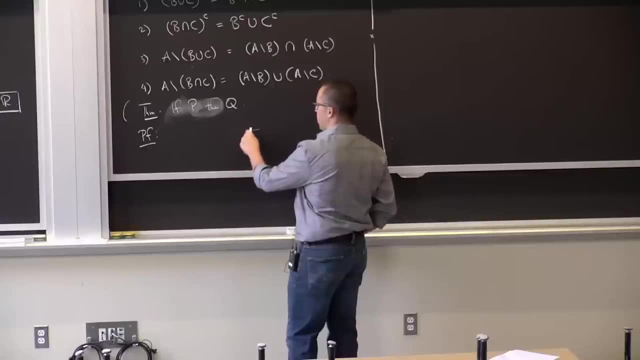 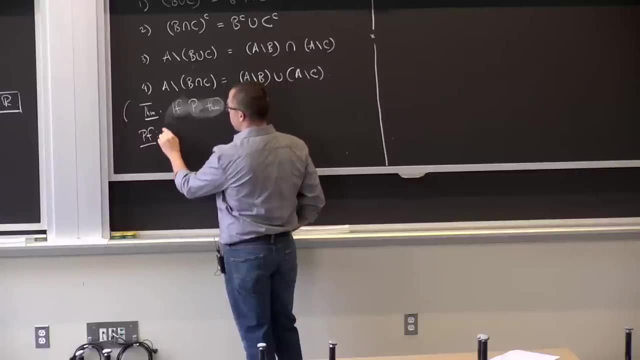 Now meaning true statements about these objects, And the real meat is the proof part. So what is in this mysterious guy the proof? It's quite simple. You start with, You assume P meaning what you're given the hypotheses. 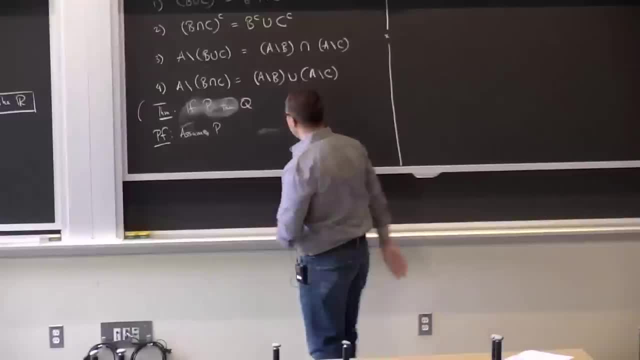 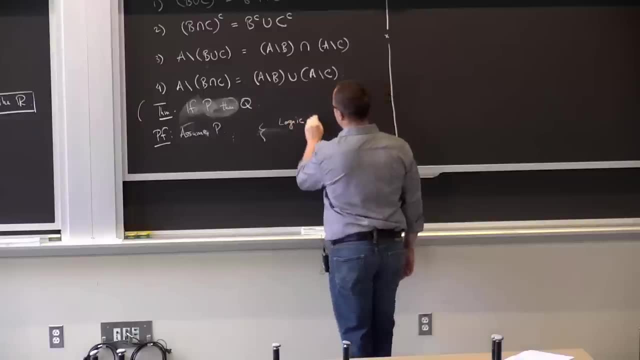 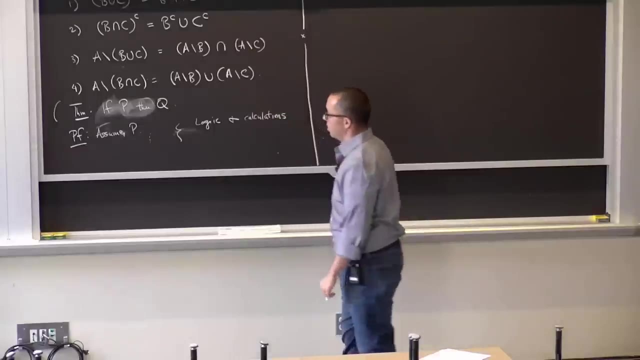 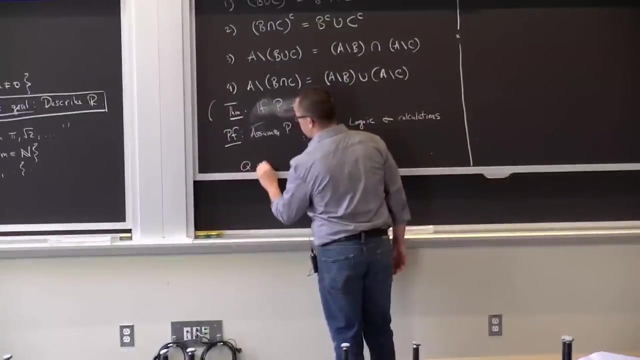 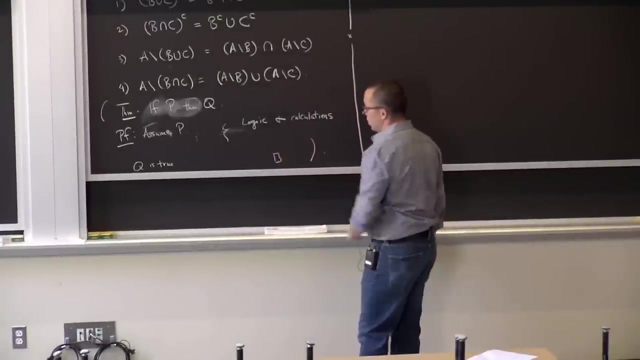 The hypothesis P, And I'm going to put dots here through logic And most definitely most of the time, some calculations you arrive at Q is true And most proofs are ended with This little box here. okay, So most proofs have this structure. 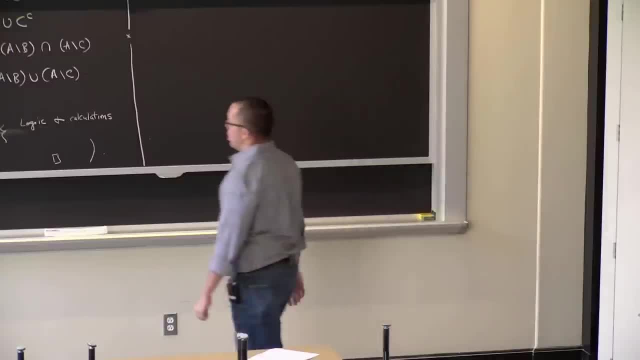 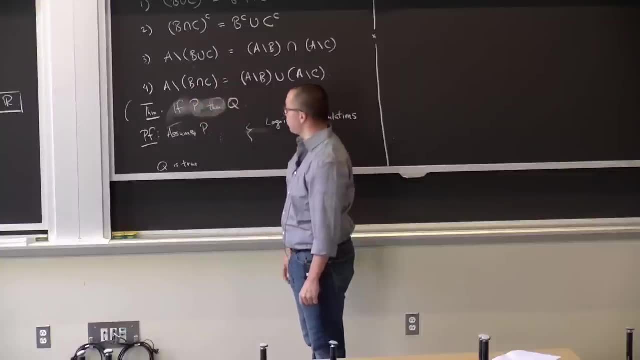 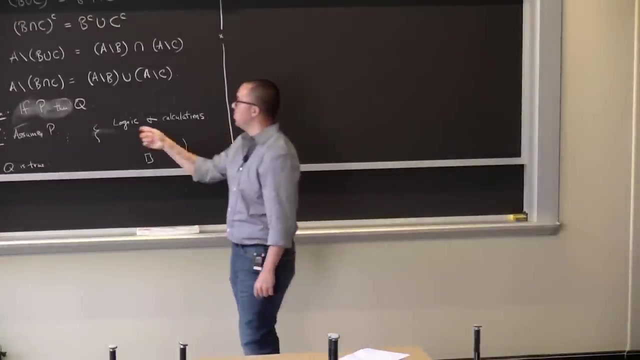 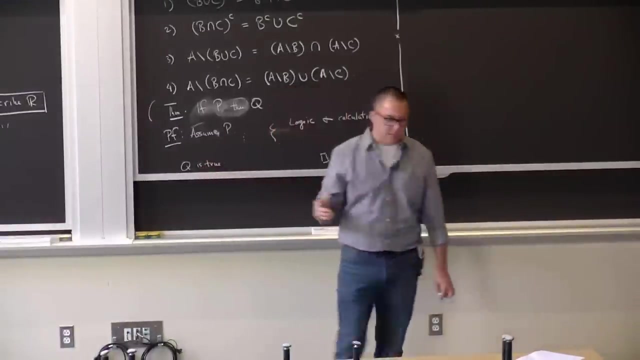 I take my hypotheses, and these hypotheses mean something in terms of the definitions I have given, And now I need to use these unambiguous definitions, along with logic and maybe some calculations, to conclude that statement Q is true. So, if I use the statement Q, 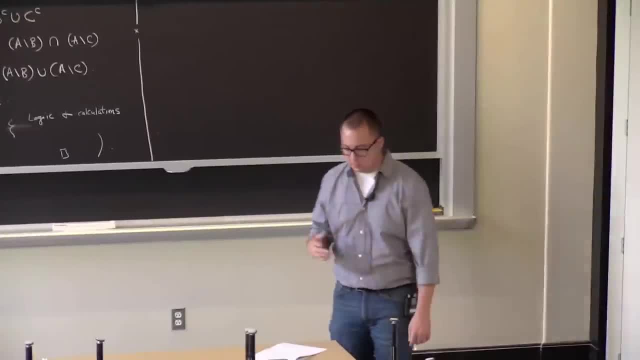 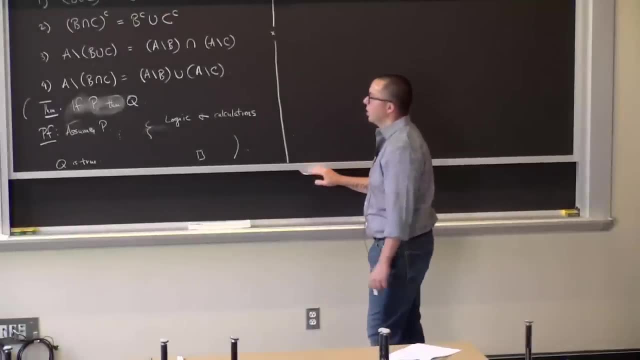 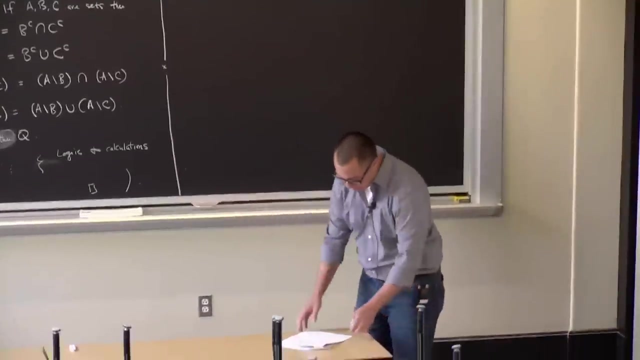 that is the essence of a proof. that is all there is to it. Now, that doesn't mean it's a simple thing to learn how to do. That's the point of this course. But, distilled down, that's what a proof is Okay. 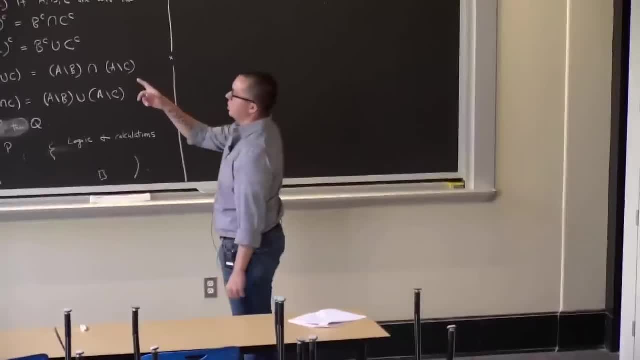 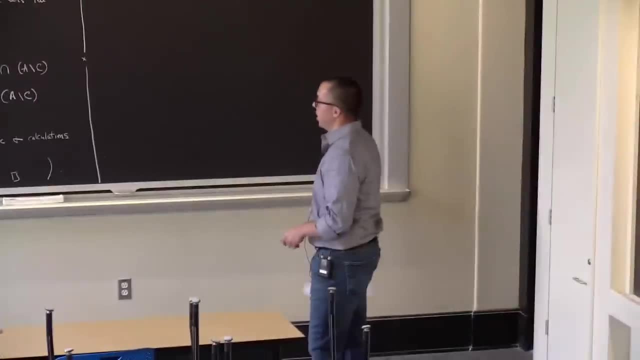 And Q. so I said P usually means something in terms of the definitions we have, But also Q. We'll use that one. Okay will usually mean something in the definitions that we've given, And so our job is to verify Q. 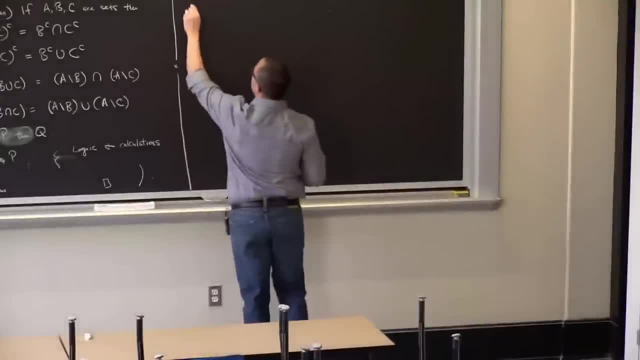 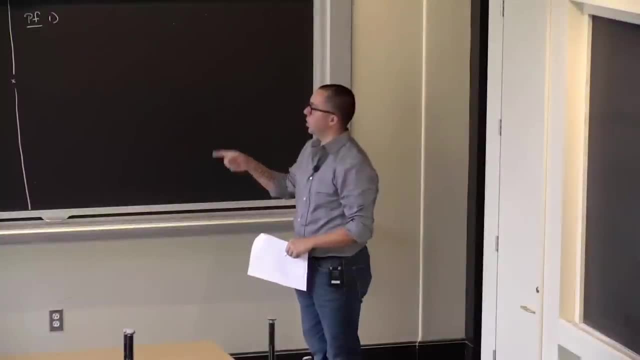 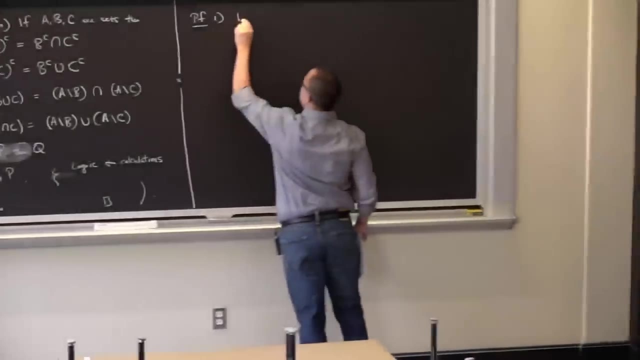 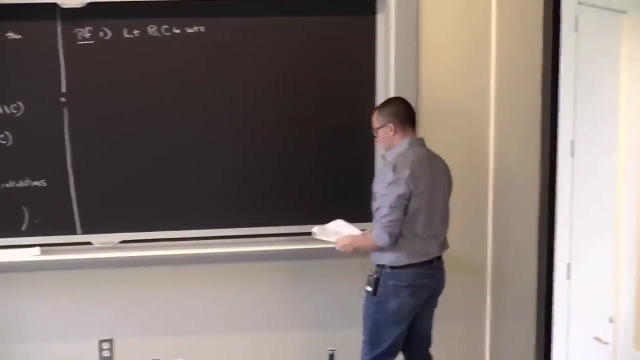 So let's go with proving this theorem, And in fact I'm only going to prove property 1.. Property 2, 3, and 4, I'll likely put on the homework, So B and C be set. So I mean, this is the only hypothesis I get. 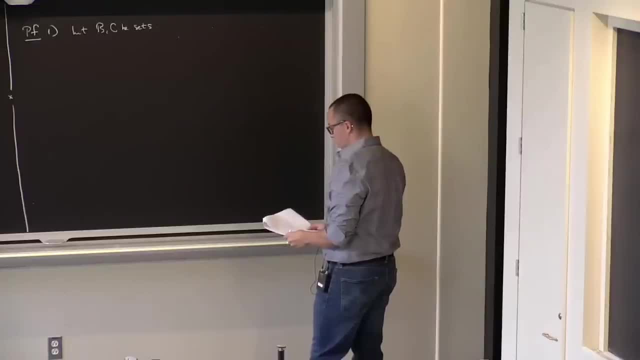 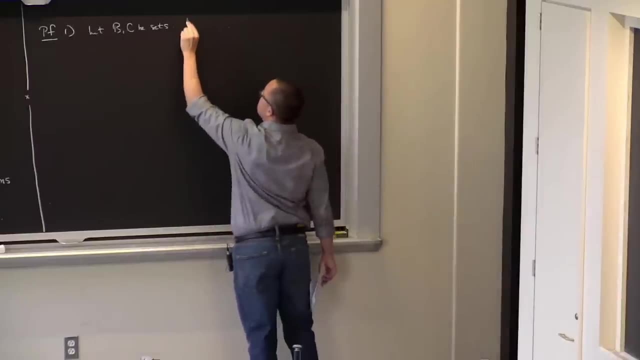 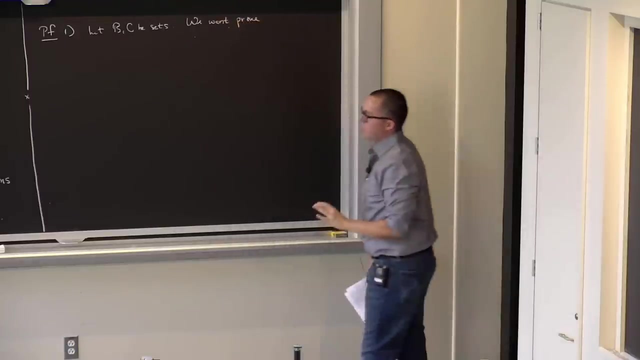 I'm trying to prove that B union, C complement equals the intersection of the complements. So what does that mean? So we want to prove. So this is quite helpful, especially when you're first starting to do proofs, to write down what you're actually trying to prove. 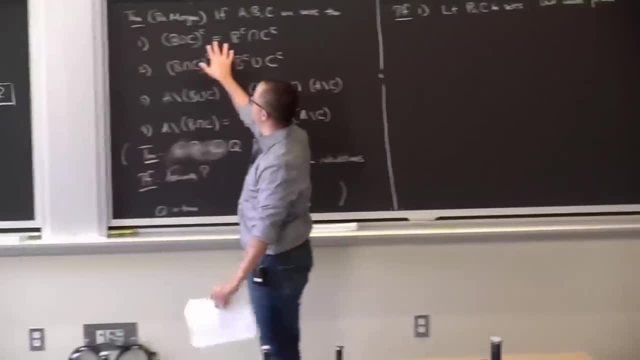 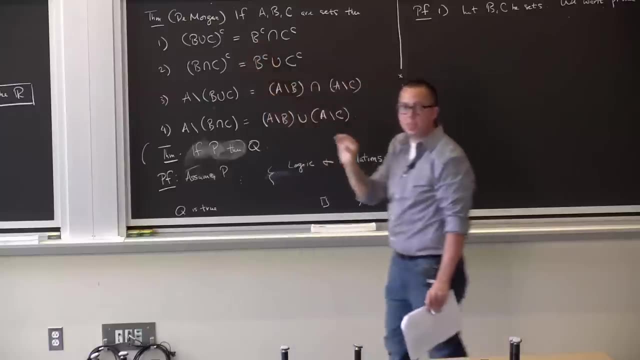 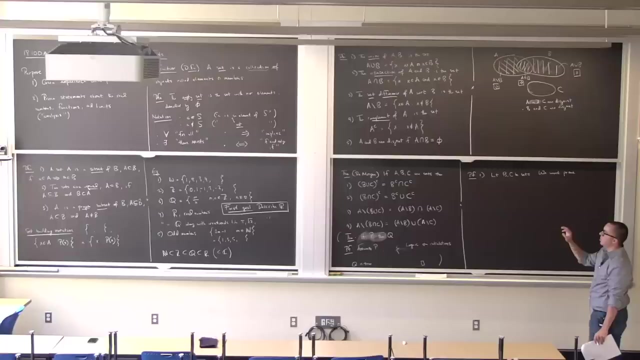 So, even though I have this statement here, it's an equality between two sets. Equality between two sets means something specifically right? We have that in our definition. Where is it Over there that two sets are equal if one is a subset of the other and vice versa? 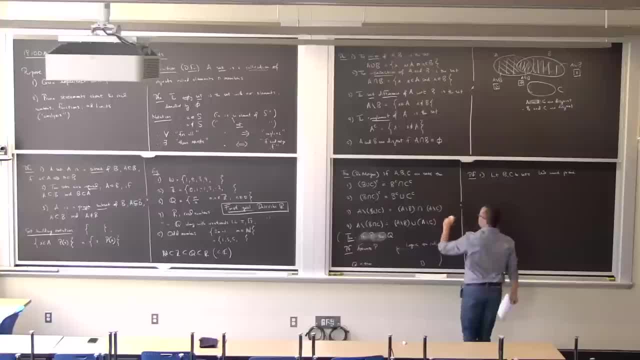 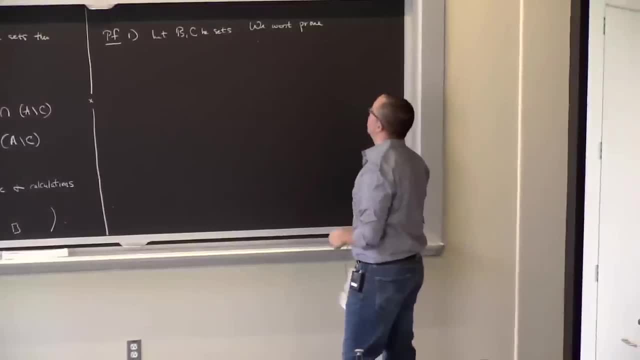 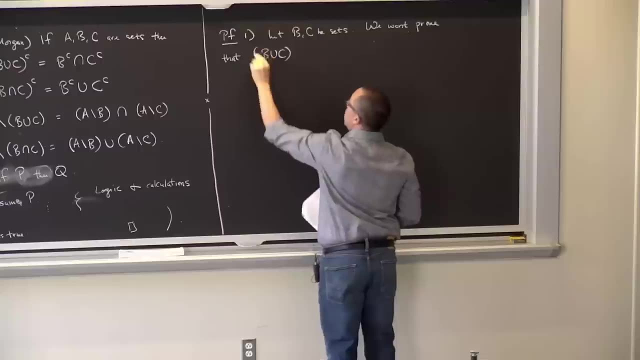 So that's what we have to prove. We have to prove, We have to prove that the left side, B union, C complement, is a subset of B complement, intersect C complement and vice versa. So we want to prove that it's a subset of B. 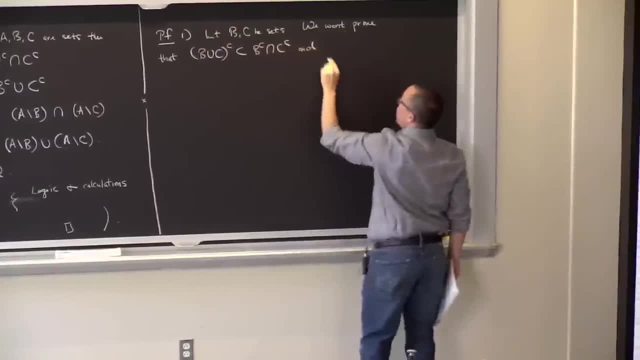 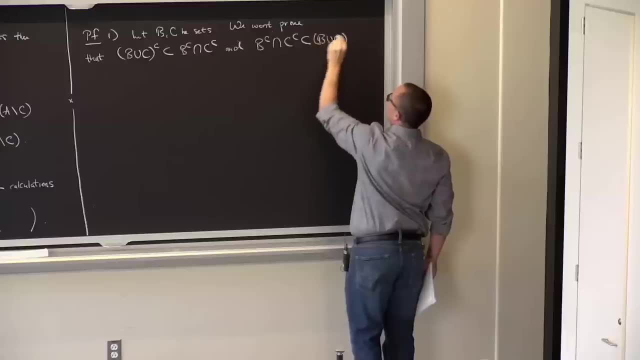 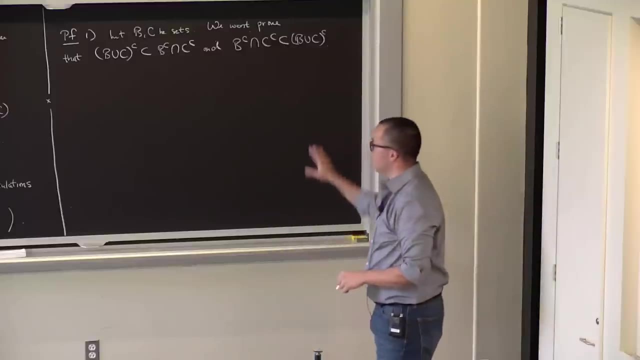 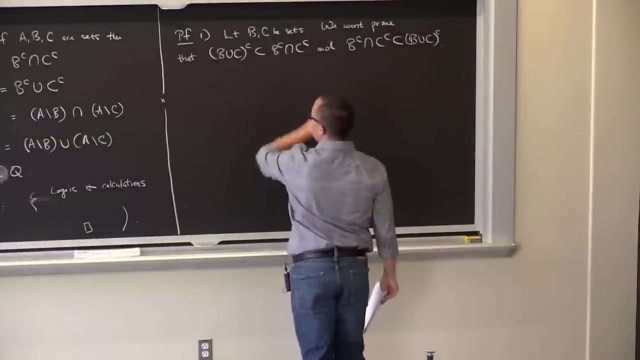 And, And, And. So that's what the equality means. That's what we have to prove. We have to prove those two statements now, And that's as distilled down as far as we can go. So let's prove this Now. we'll prove this using, again, logic. 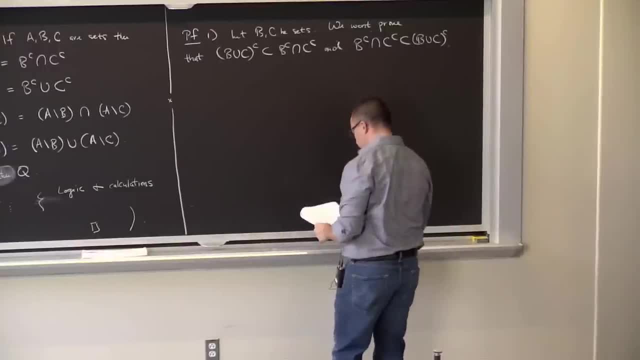 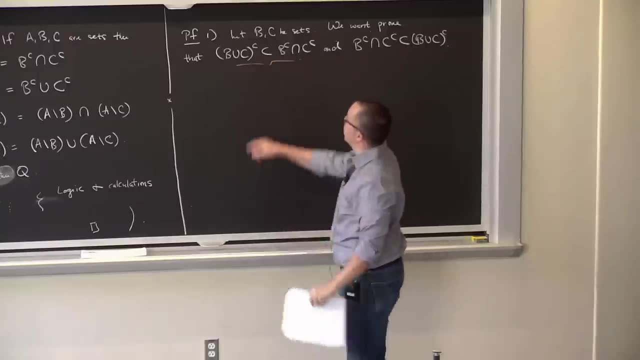 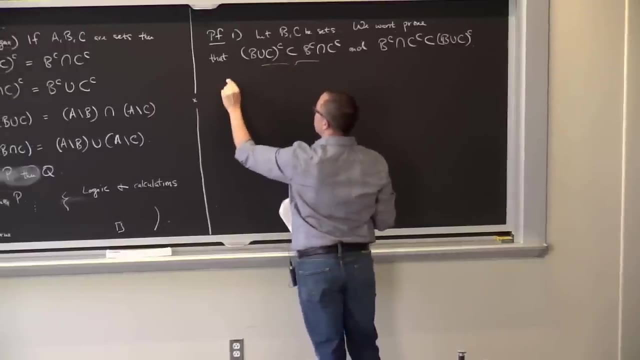 And what these things actually are. So let's prove this first statement here. So I have to show that every element in this set is an element of this set. So I'll even write this down As WTS. that means want to show. 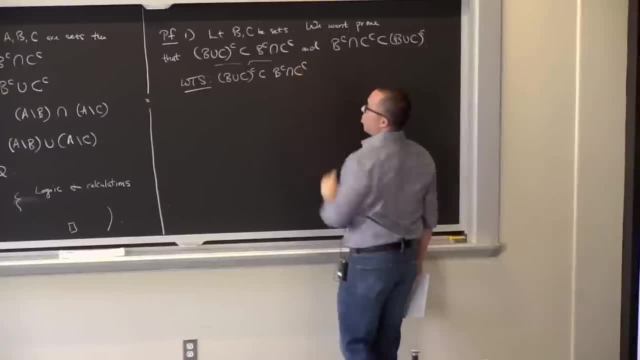 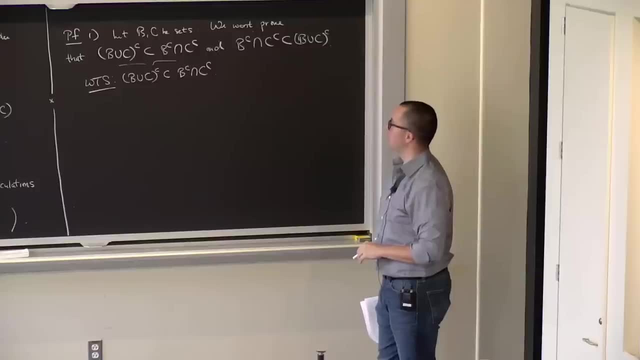 This is the first thing we'll show. So, as we go on, I'm not going to write as much as I'm doing right now, But this is the first theorem and proof you're seeing, So I should write down quite a bit. 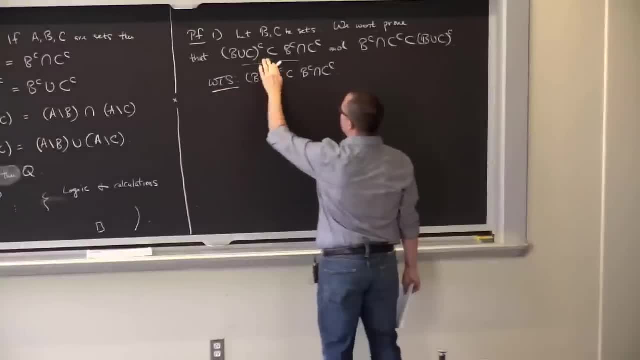 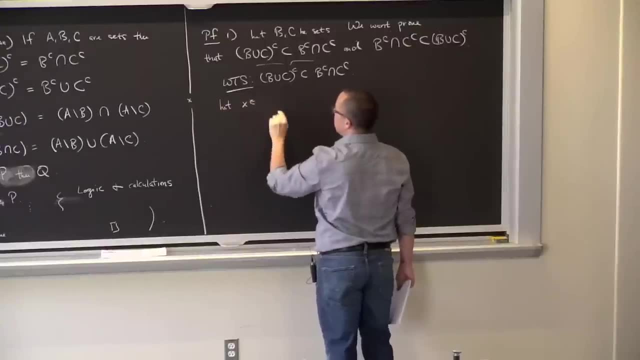 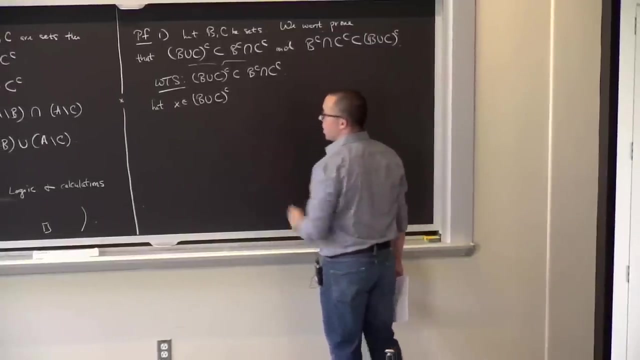 So the first thing we want to show is we have this inclusion. That means every element here is an element here. So let X be in B, union, C, complement, And now we're going to trace what this means And we'll eventually arrive at X is in this. 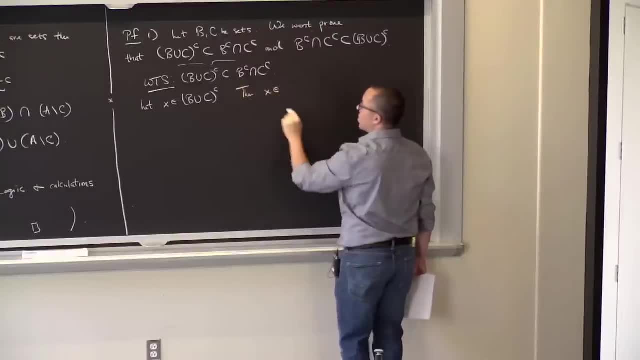 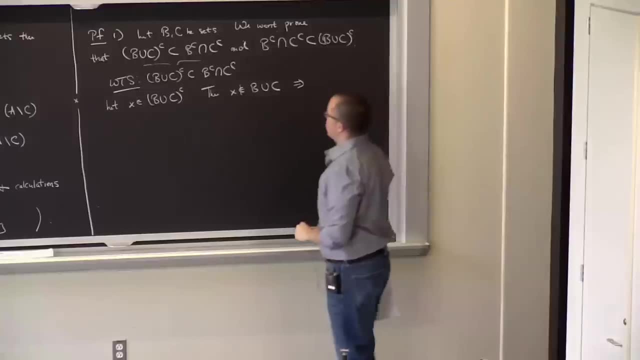 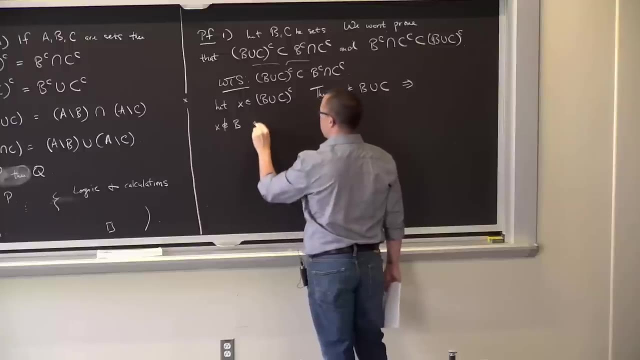 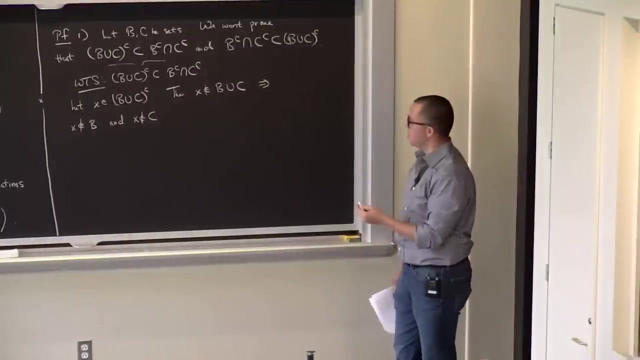 So then X is not in B, union C. That's just the definition of the complement. Now, X is not in B, union C means X is not in B and X is not in C, Because the union is something's in the union if it's in B. 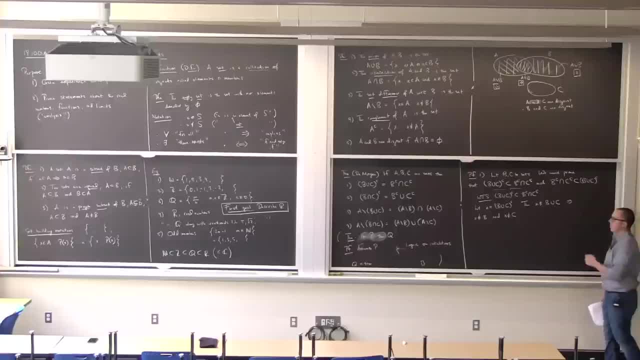 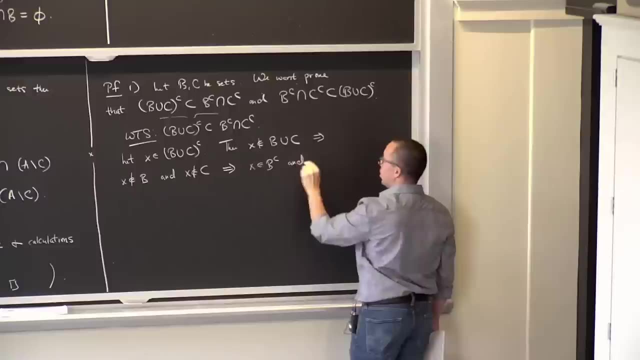 or C. So something's not in the union if it's not in B and not in C. Now this implies simply, again by the definition of what it means to be in the complement, X is in B complement and X is in C complement. 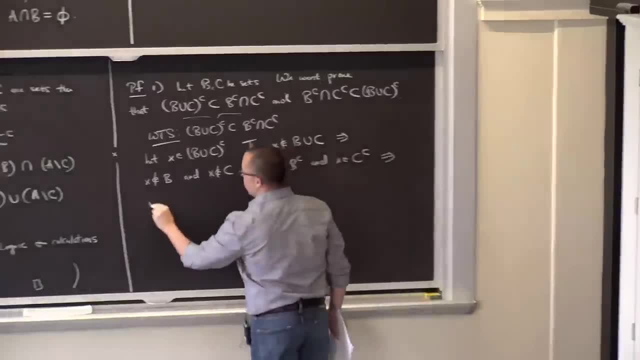 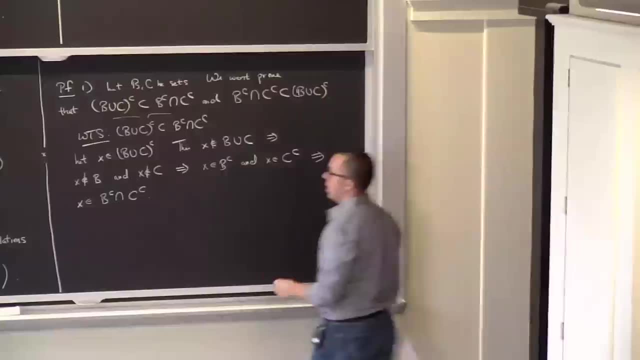 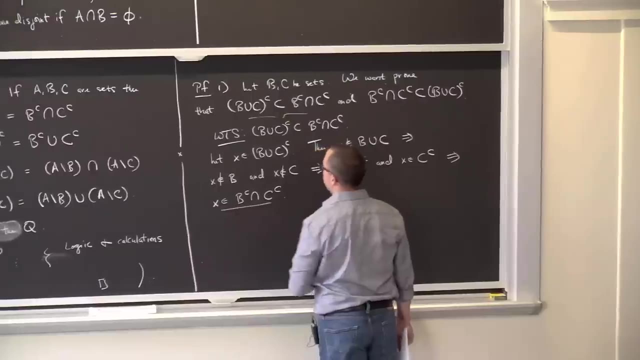 But this again is simply the definition of X being in C. So let X be in B, complement intersect, C, complement. So you see, we started off with an element in this guy And we showed that it's also an element of the right hand side. 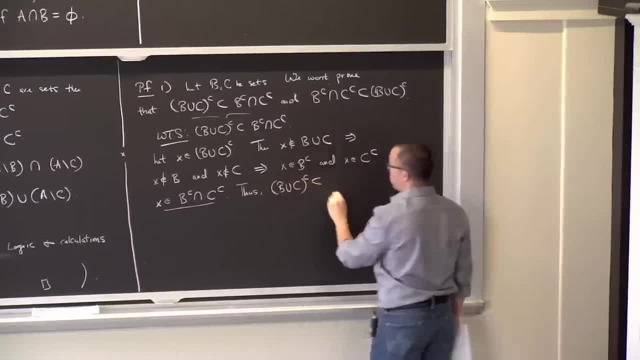 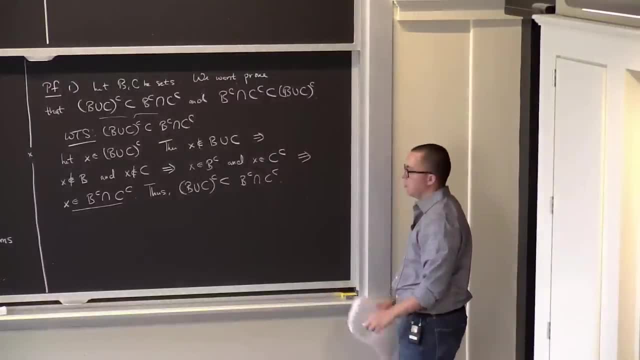 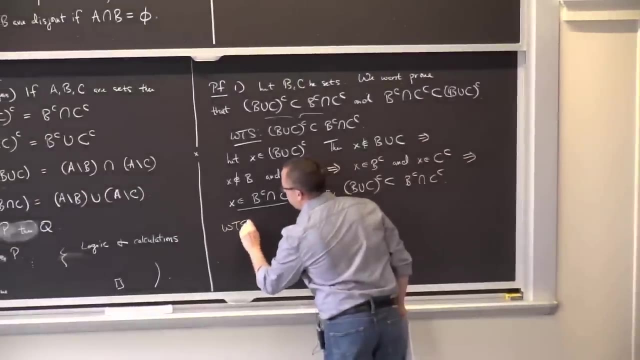 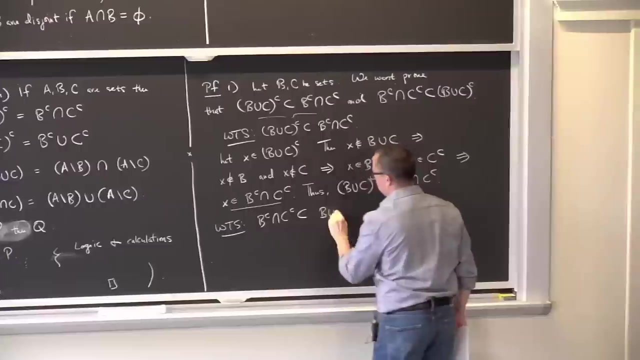 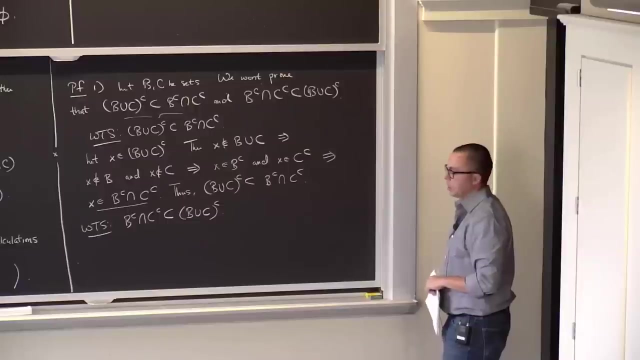 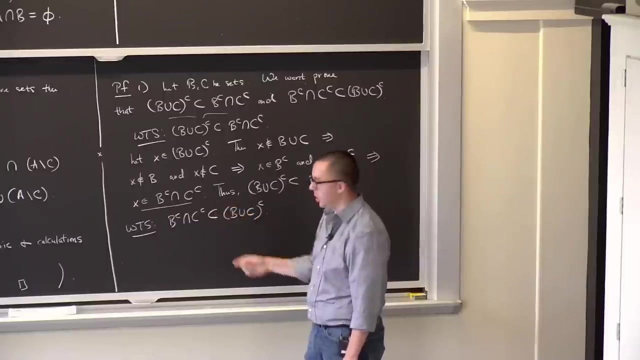 So thus B union C complement is contained in B complement, intersect C complement. Now we want to do this other inclusion here. Now, this is one of those kind of rare situations where you get to essentially reverse the entire argument and get what you want. 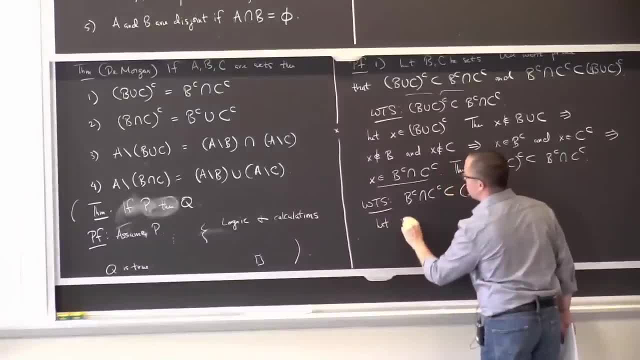 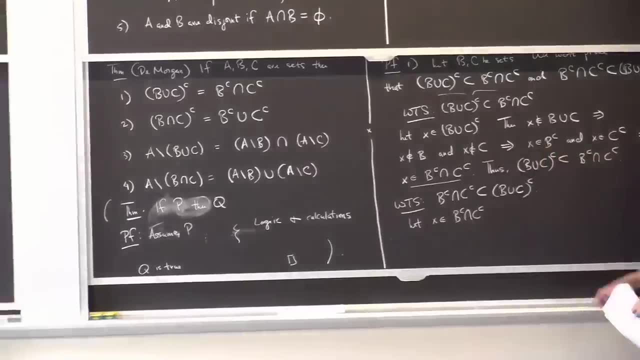 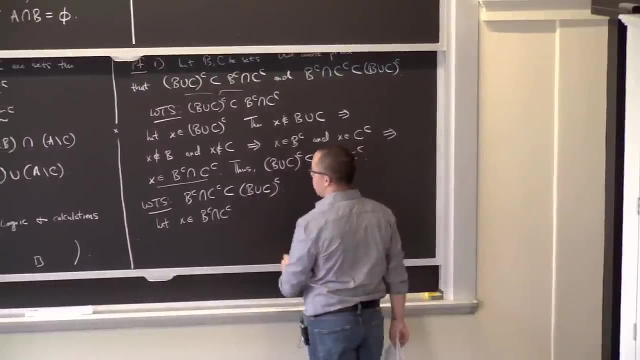 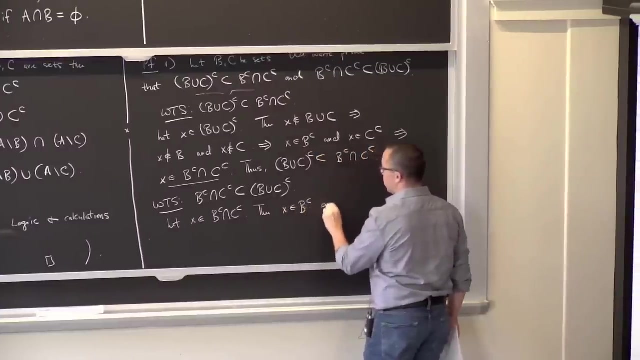 But let's just go through it in a linear fashion. Let's take something from here and show it's in here. So let X be in the intersection of the complements. Then that means X is in B complement and X is in C complement. 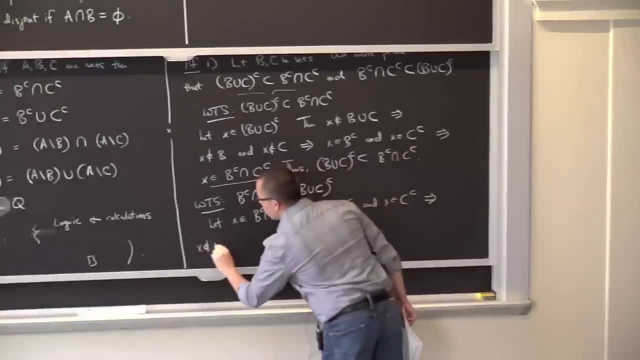 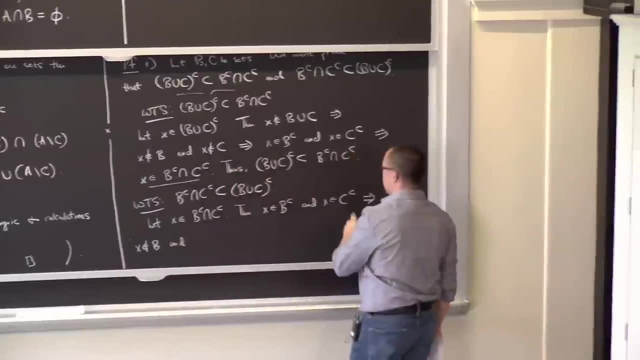 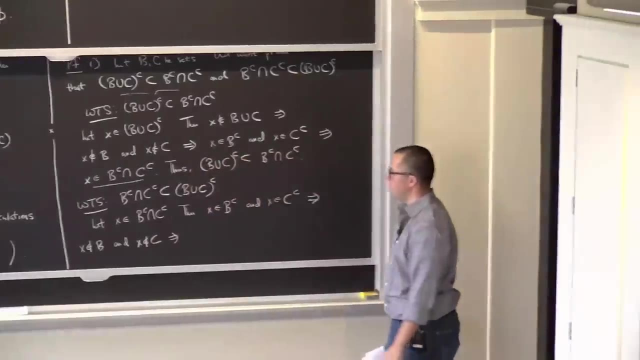 That means X is not in B. So that's this statement. That's the definition of being in the complement, And X is not in C. That's, again, the definition of being in the complement Now, just like we used here in this step. 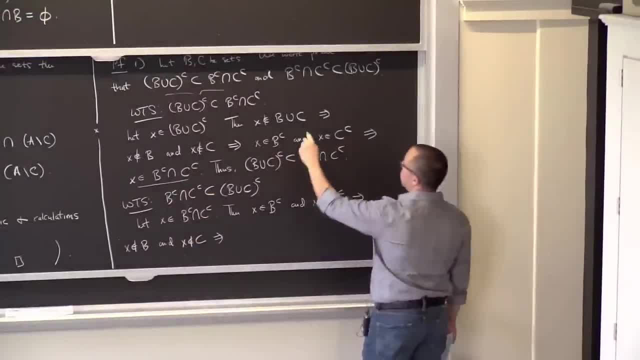 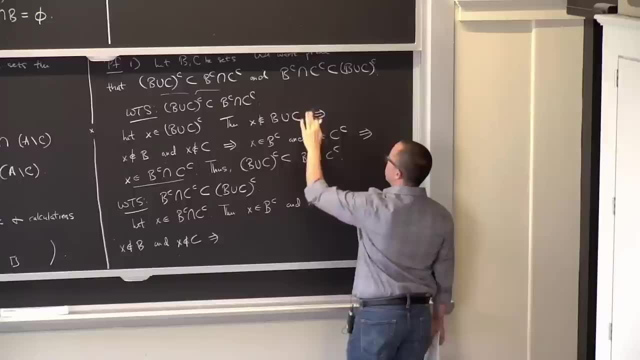 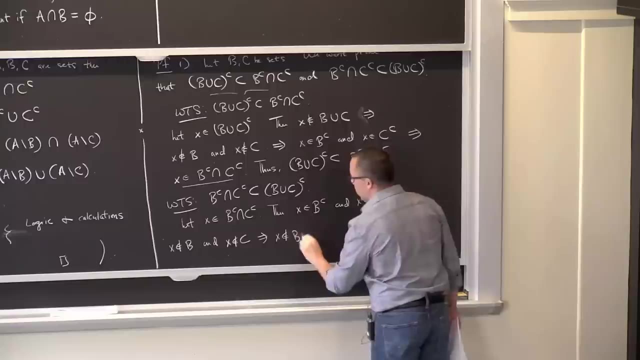 this is equivalent to. So really I should in this statement I should have written: this statement is equivalent to this statement, but we'll remove that. So X is not in B and X is not in C. This means X is not in their union. 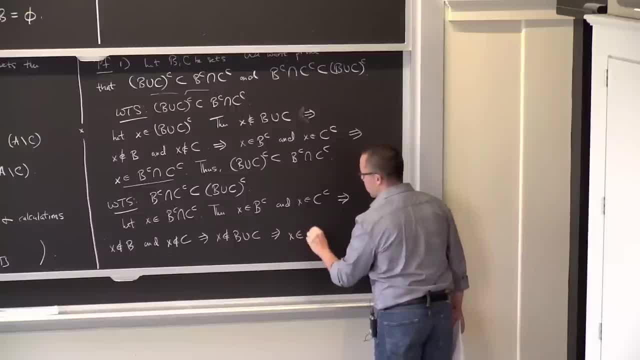 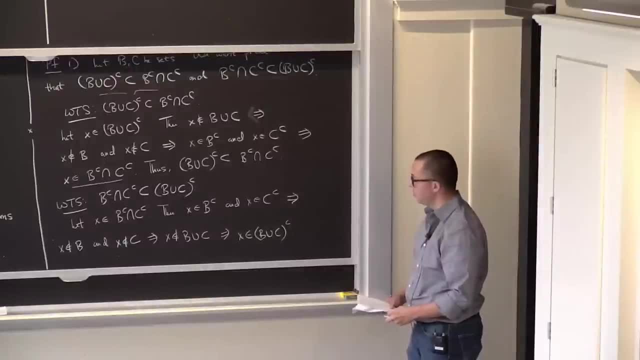 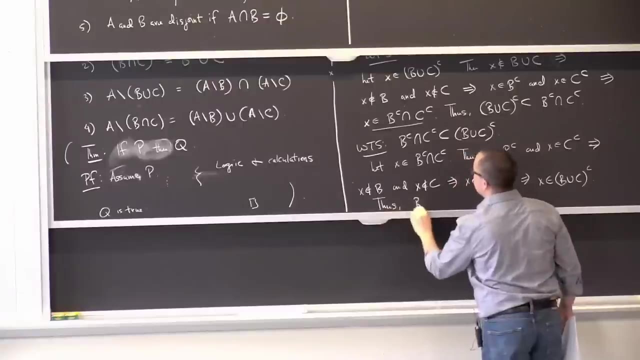 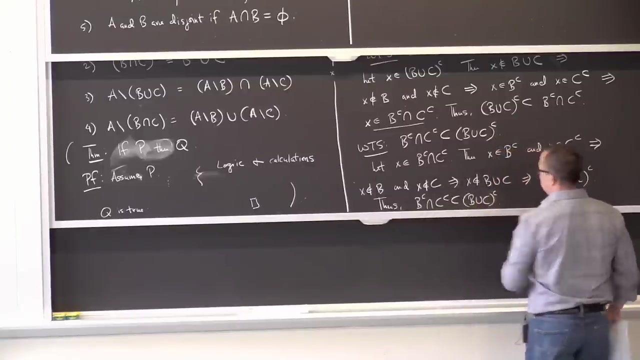 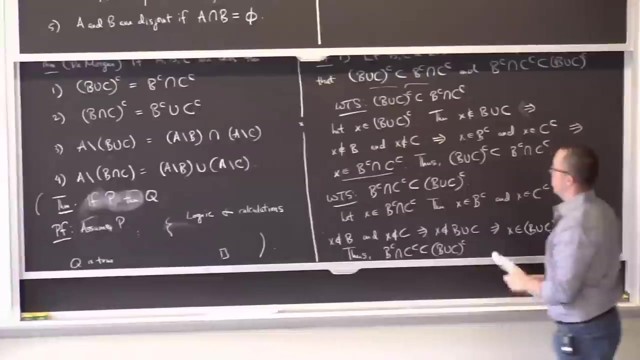 which implies that X is in the complement of the union. Okay, So Thus we've proven it's a subset of B And since we've shown both sets are a subset of each other, that means by the definition of two sets being equal. 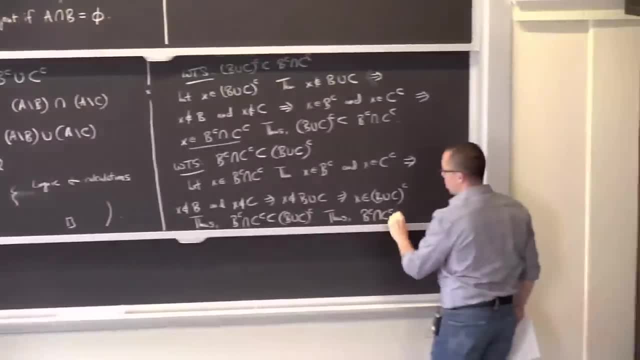 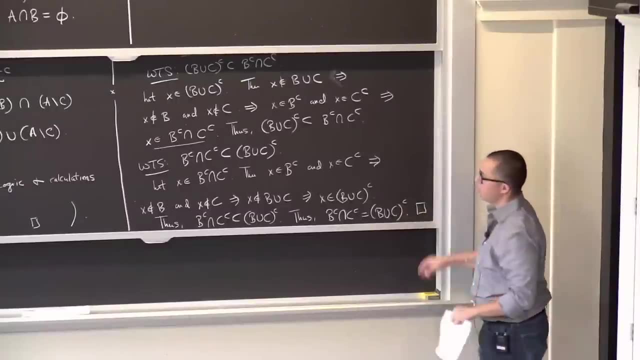 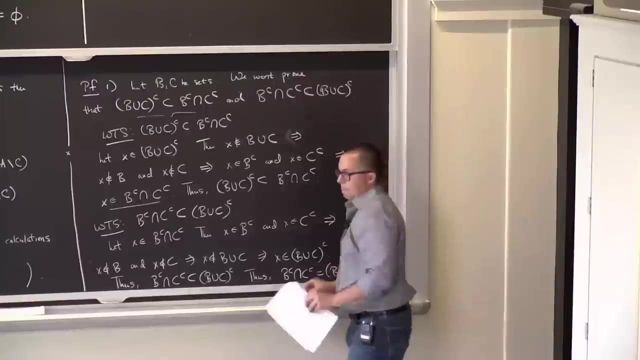 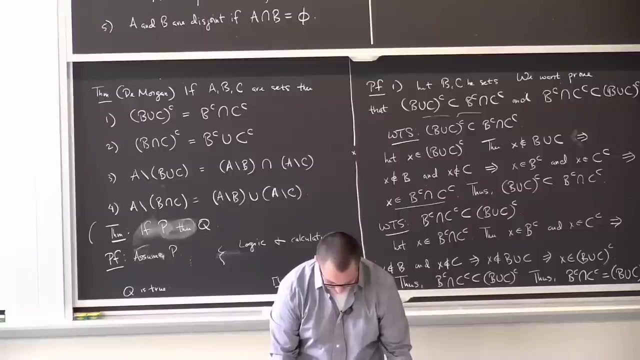 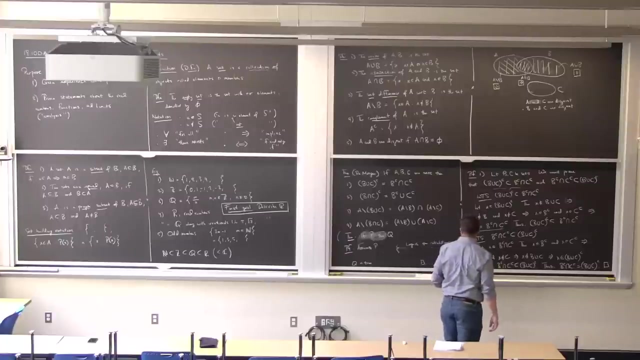 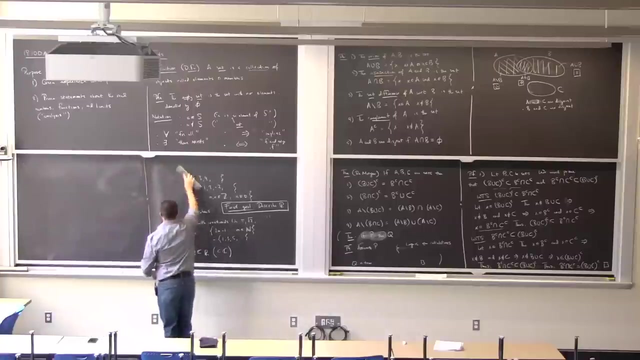 they are equal. And again, this box means really nothing. It just means that's the end of the proof. All right, Let's move over here. This is terrible, And not everybody uses that little box to finish a proof. Some people don't put anything. 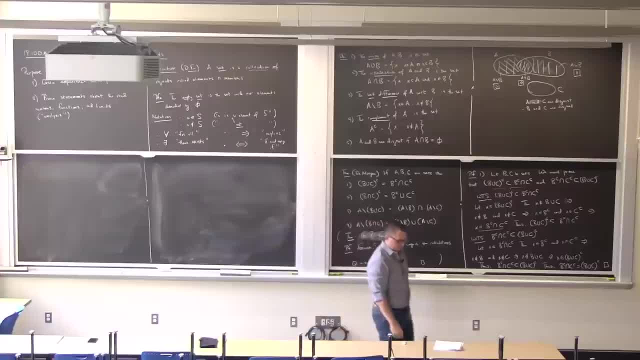 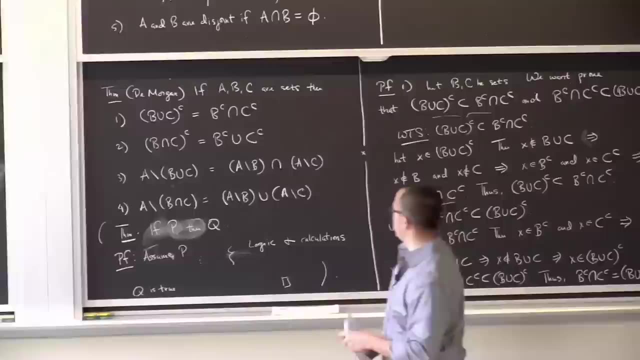 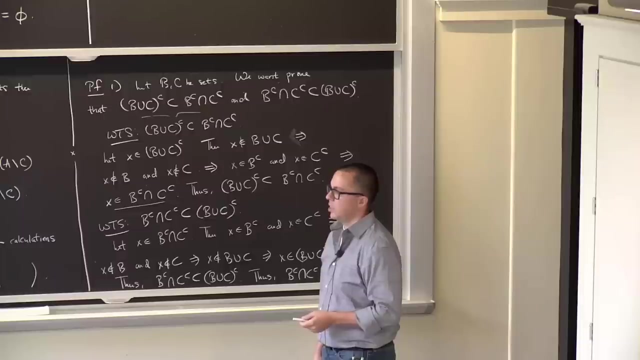 I was. When I was in graduate school, I was a TA for this guy named Paul Salley, who was a fantastic teacher and really loved math. who would end. So amazing story about this guy is, you know, when I was his TA he was in his 70s, I think. 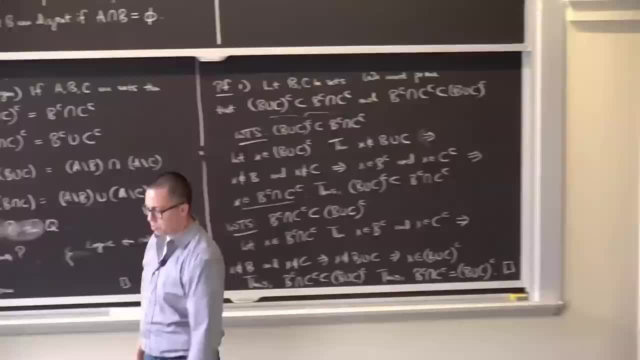 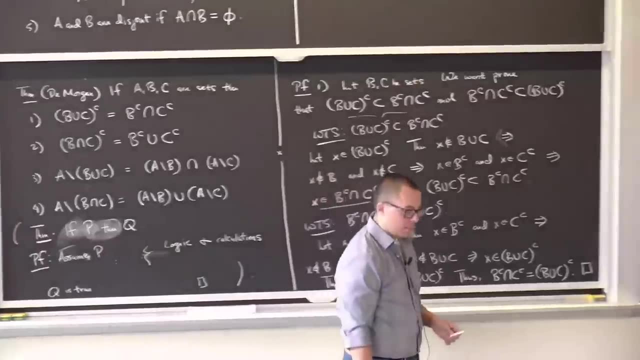 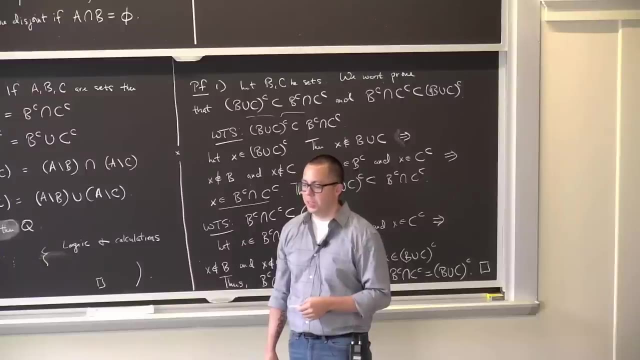 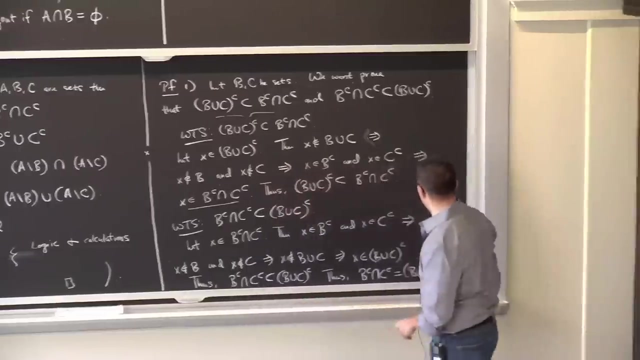 But he had also had diabetes, so he had lost both of his legs beneath his knees. He was also legally blind And he had a patch over one eye. So he himself often referred to himself as the pirate mathematician. But he would end his proofs with: 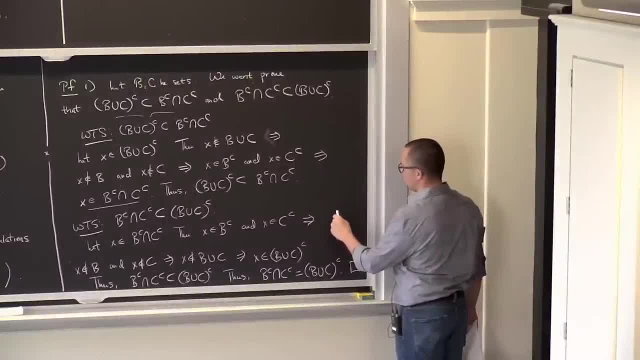 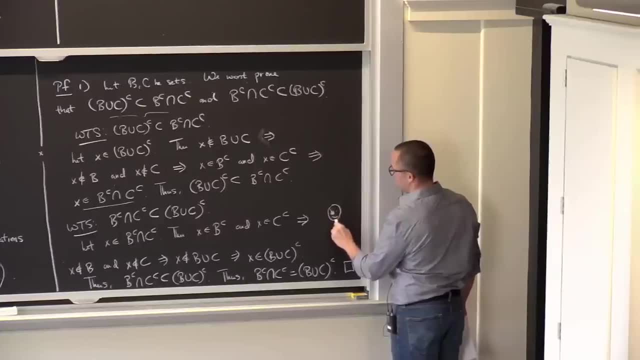 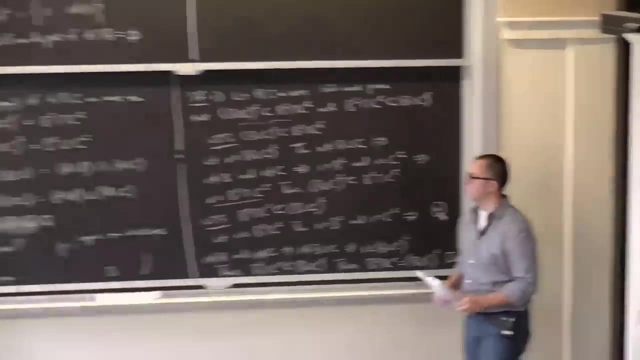 at least in his textbook. He didn't ask me to do this on the board. thankfully, He would end his proofs with a picture of himself with this cob pipe that he had. very much in the pirate fashion, Anyways. okay, moving on from things that end proofs. 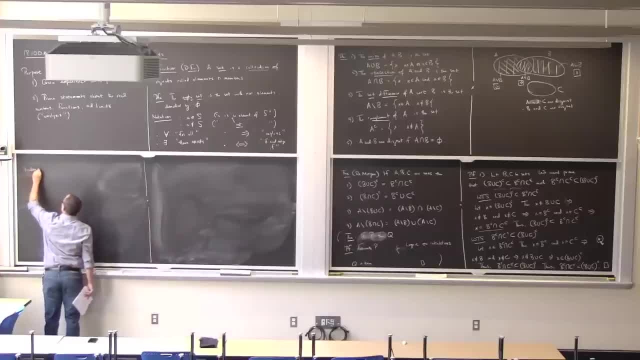 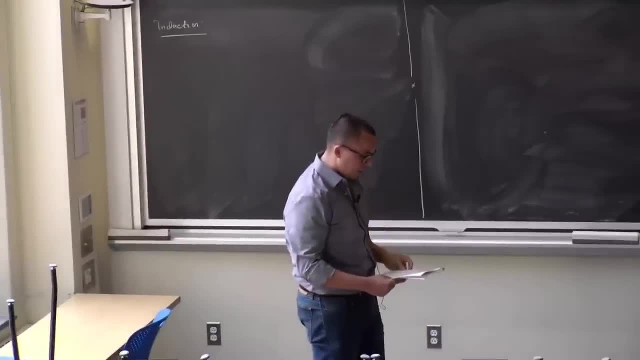 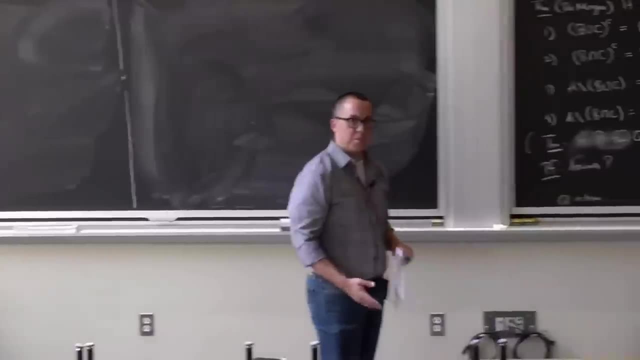 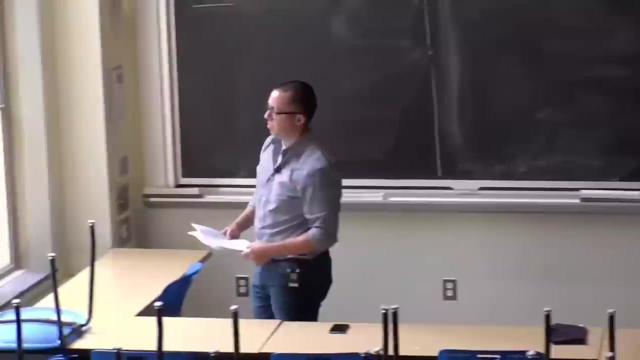 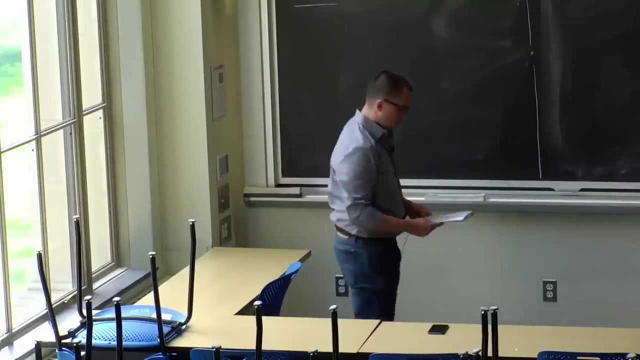 Let's go on to next subject: induction. So induction is a way to prove theorems about natural numbers, That's. you know, the theorem itself is more of a tool rather than an interesting fact on its own. So let me state the theorem. 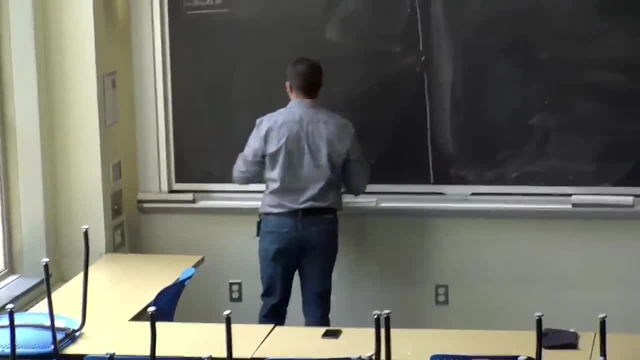 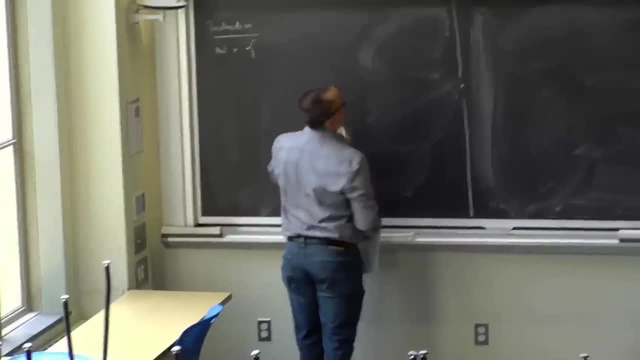 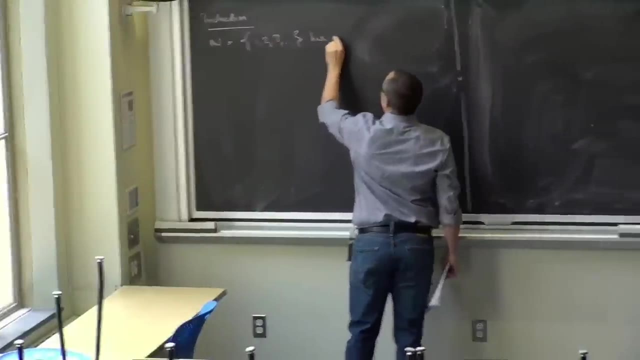 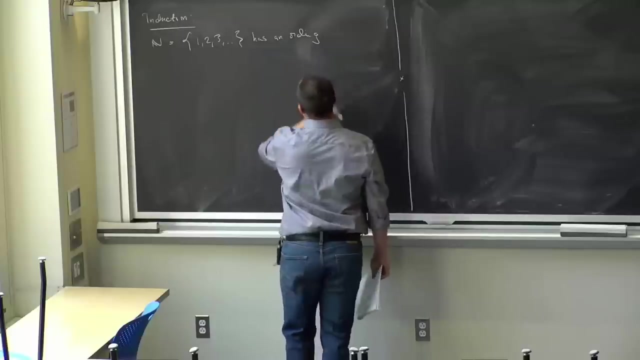 and then we'll go over a couple of examples on how to use induction. So Let me recall from- I think I just erased it- N is the natural numbers And it has an ordering meaning. So we'll precisely define what ordering means. 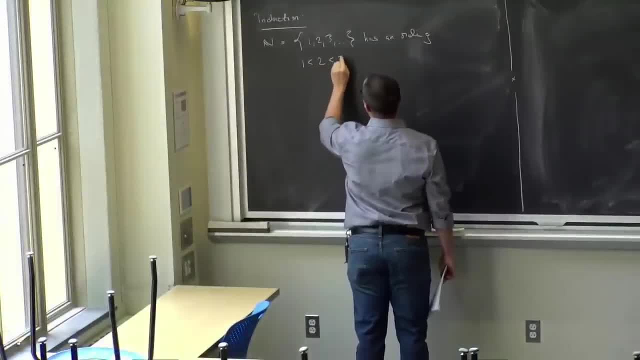 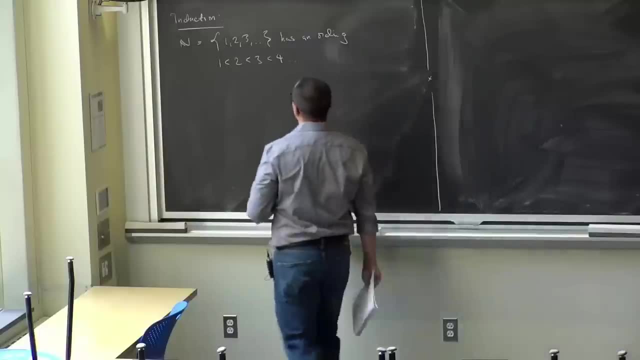 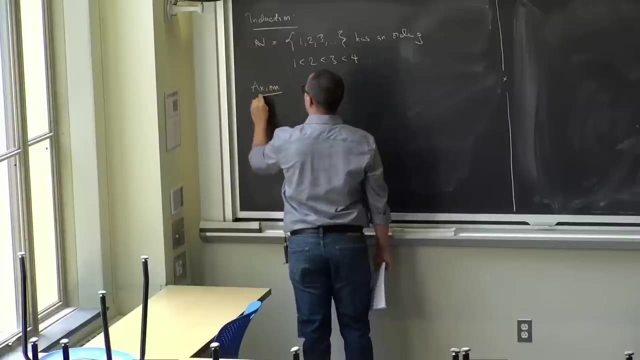 but just in your head, this means the usual thing: One is less than two, is less than three, is less than four, Um, So a property of the natural numbers which we'll take as an axiom. 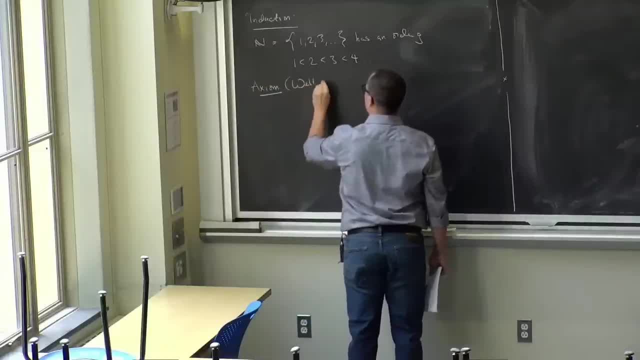 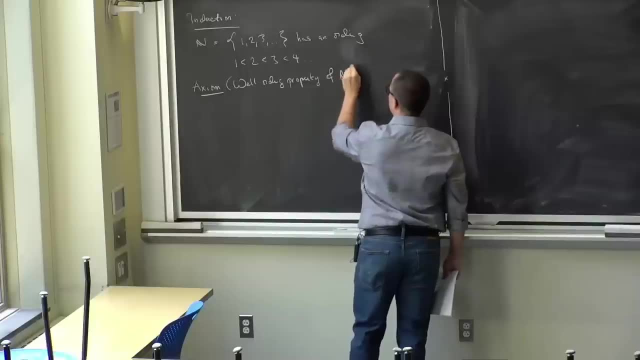 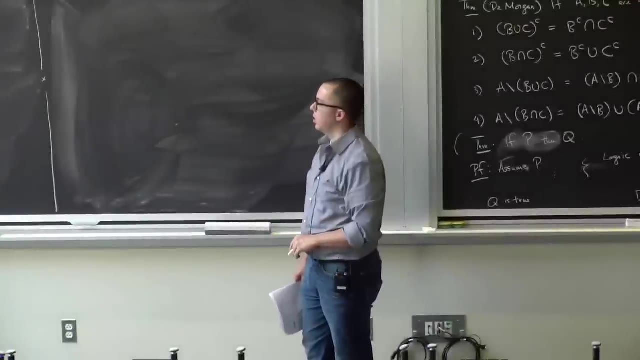 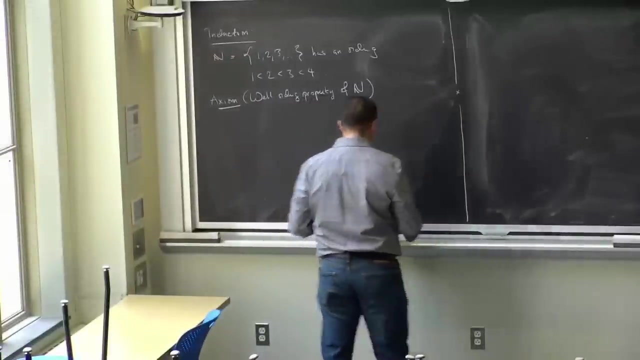 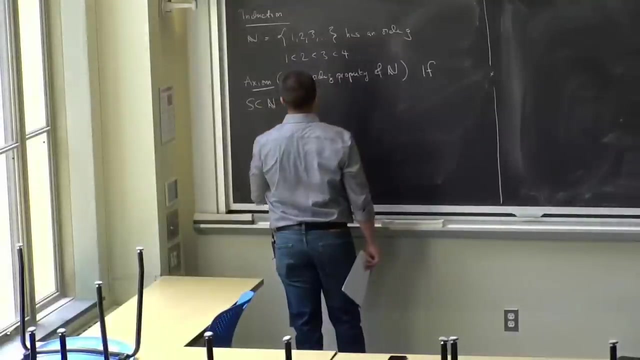 is the well-ordering property. So an axiom is not something you prove. You assume this about the objects that you've defined or are studying up to this point, And so the statement is: if I take a subset of natural numbers, 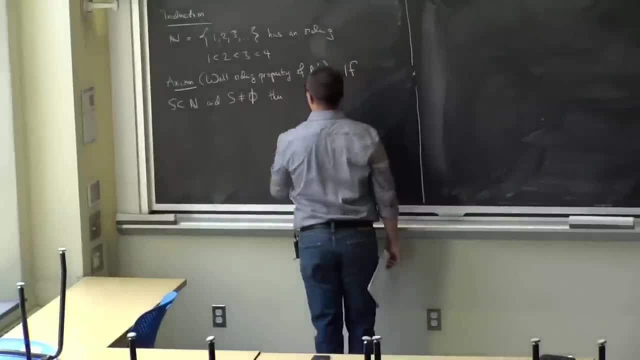 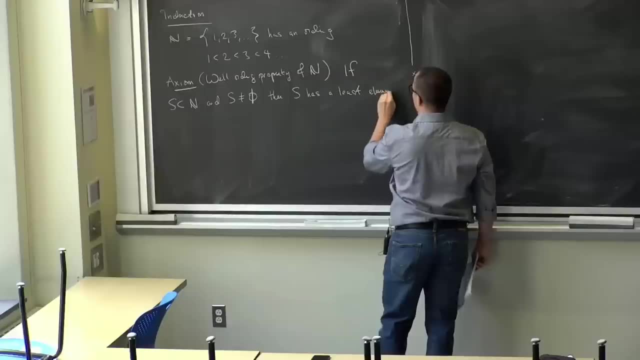 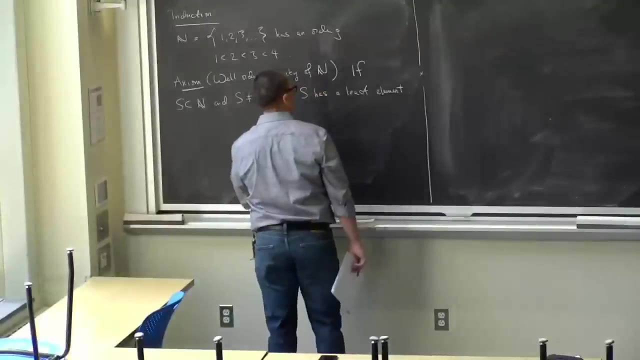 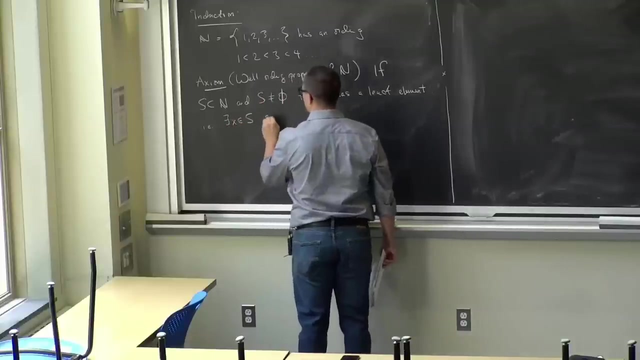 which is non-empty, then S has a least element or smallest element. Now, what does this mean? Let me write this last statement out, ie there exists an X and S, ST. I will often write meaning such that: 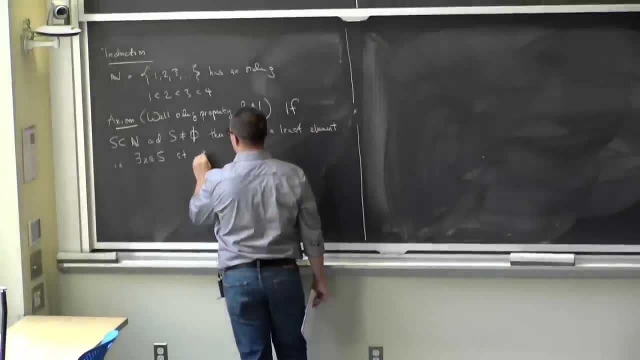 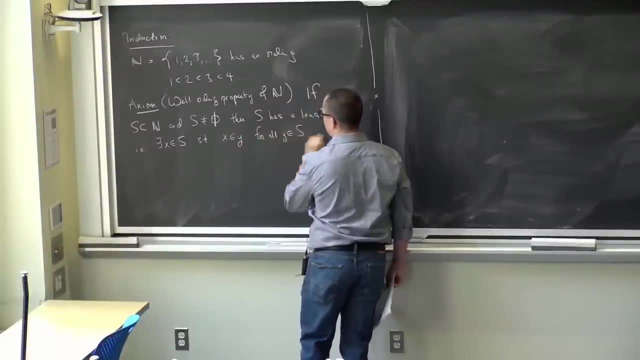 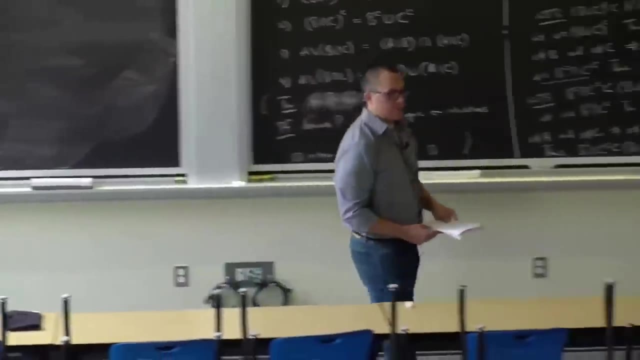 or so that such that X is less than or equal to Y For all Y and S. Okay, Every non-empty subset of the natural numbers has a smallest element. Okay, And we're going to take that as an axiom. 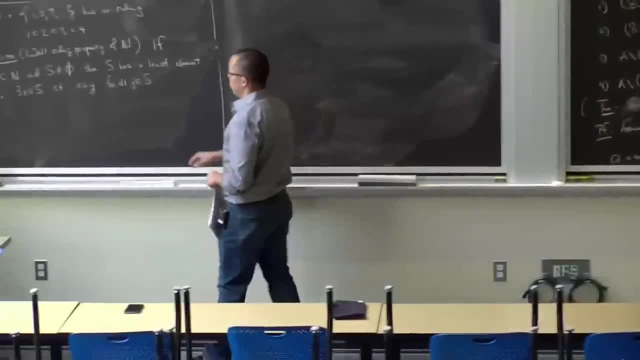 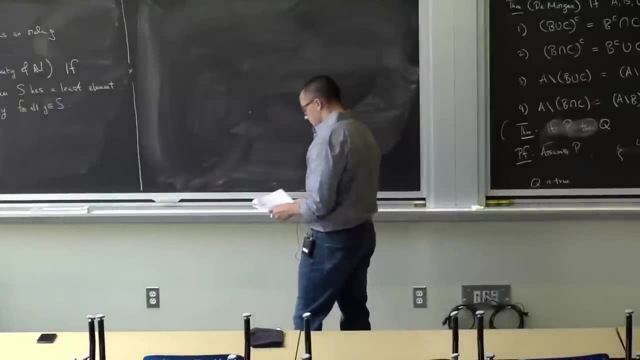 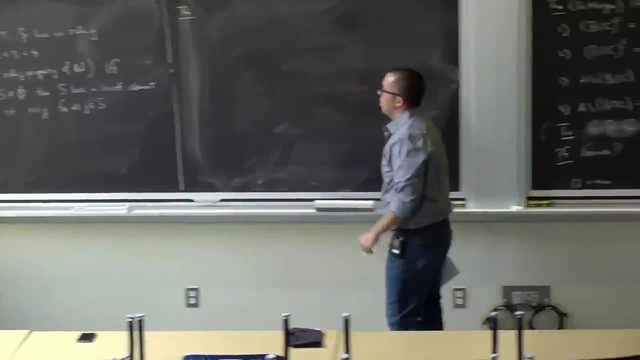 as just a property of the natural numbers, which we'll assume. Now, using this axiom, we're going to prove It's not really a. You'll often hear it called as the principle of mathematical induction, but this will state it as a theorem. 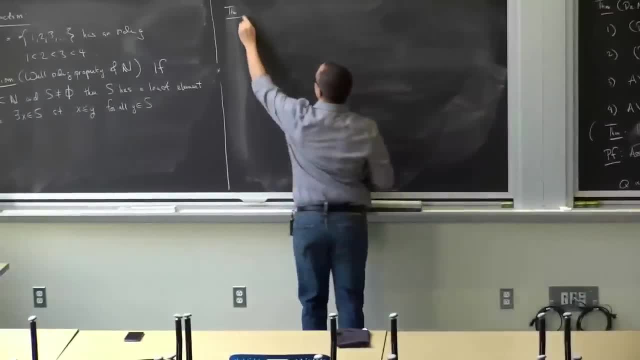 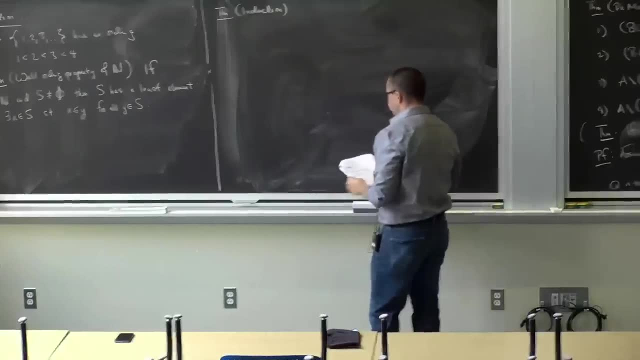 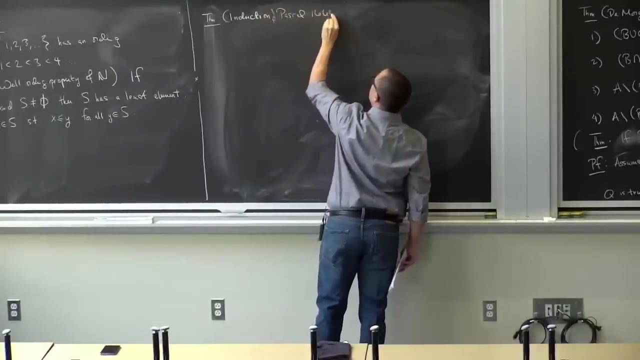 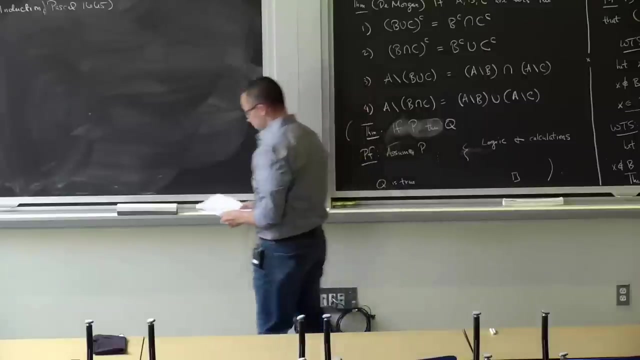 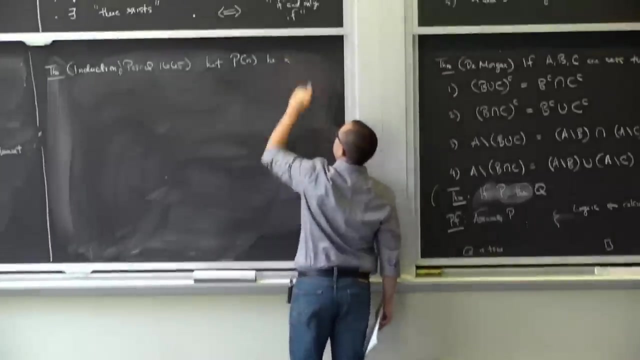 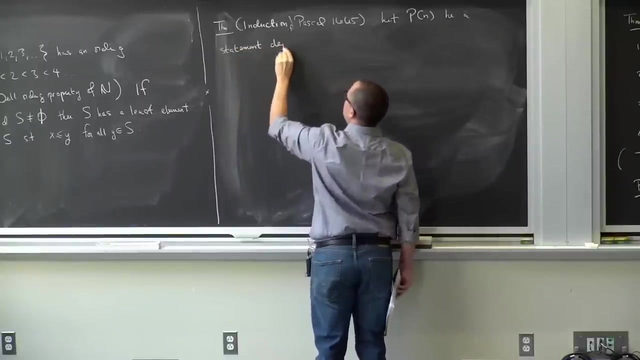 instead of a principle, Whatever a principle is supposed to be, So induction- So this is due to Pascal, or at least in its first rigorous formulation- is: let Pn be a statement. 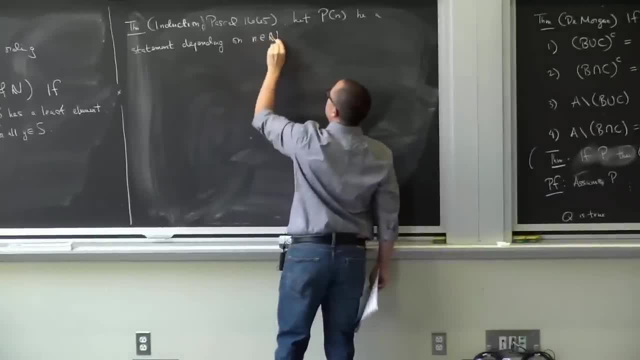 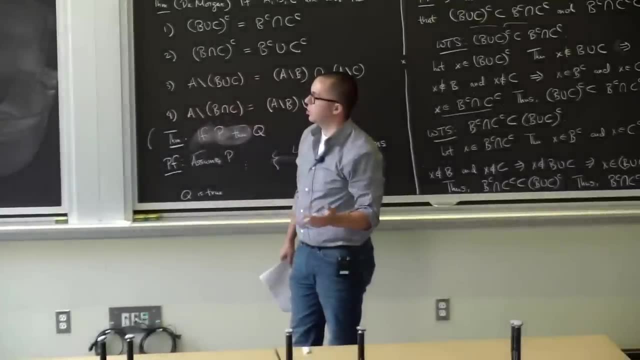 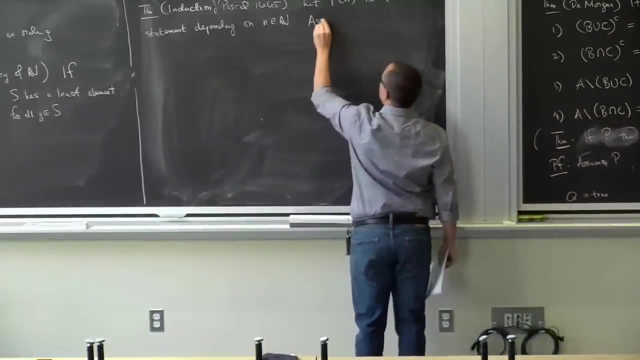 depending on the natural number n. Okay, So maybe we have some equality between two quantities that involves a natural number, n. Okay, That could be our statement. P of n. Now we're going to assume. So what are our hypotheses? 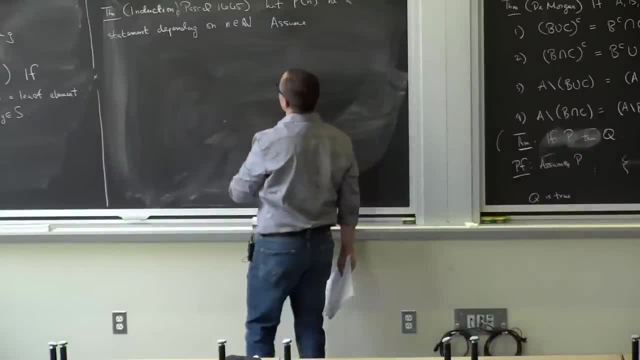 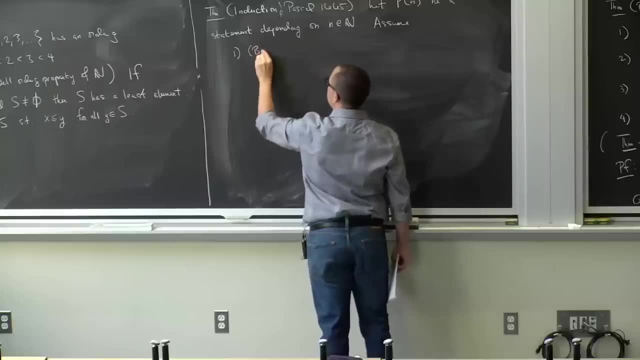 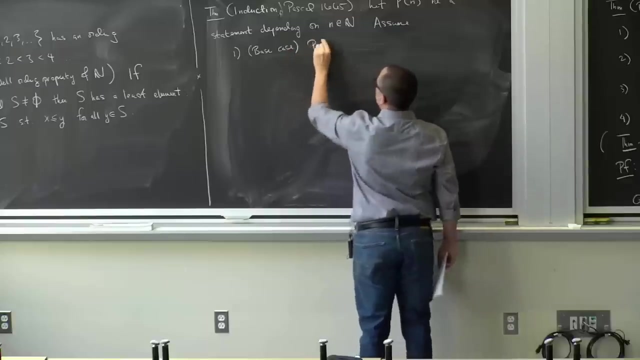 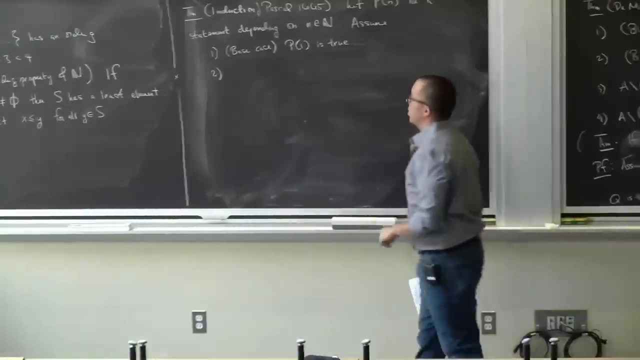 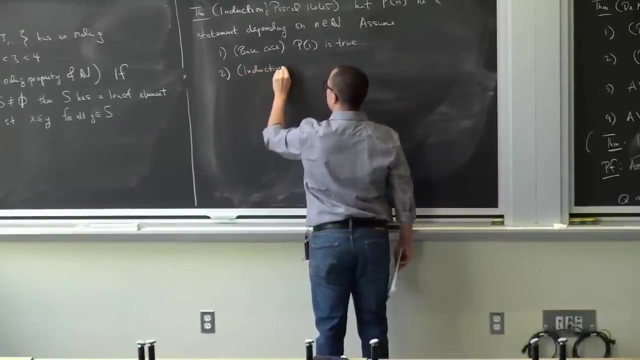 about this statement. What's our if? Assume that this statement satisfies two properties. This first property is usually referred to as a base case, That is, that P of 1 is true, And the second property is called the inductive step. So this statement satisfies. 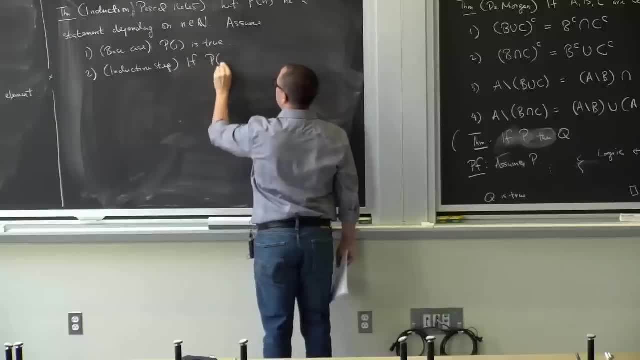 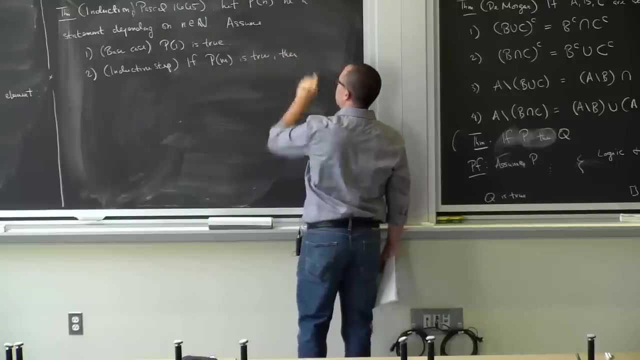 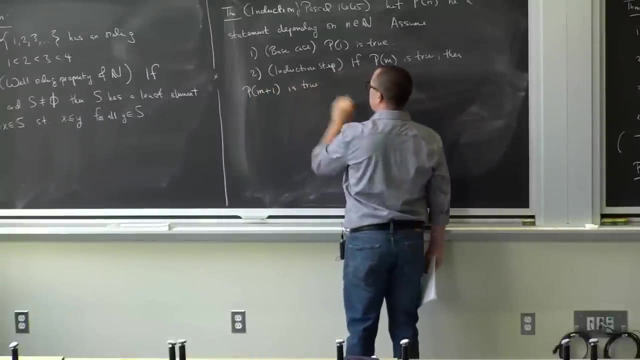 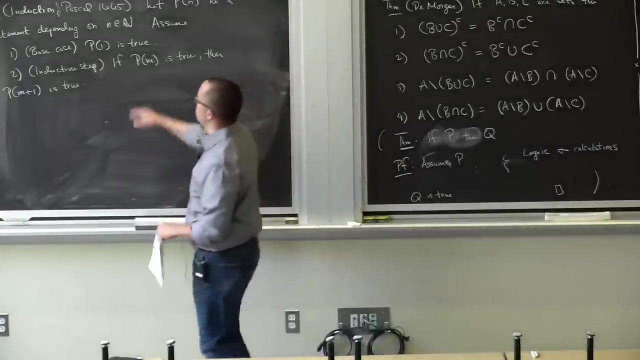 the following property, That if you assume P of m is true, then you can prove that P of m plus 1 is true. So I have a statement which satisfies both of these properties. Okay, In particular, since I'm assuming P of 1 is true, 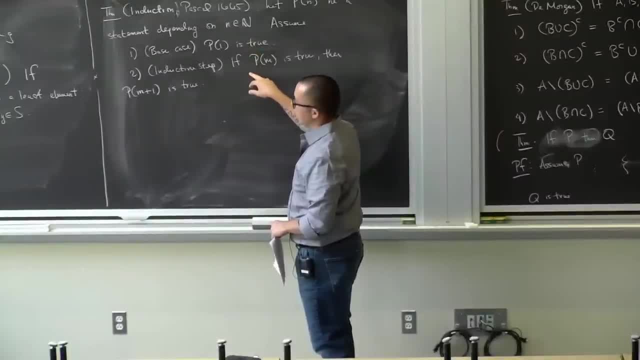 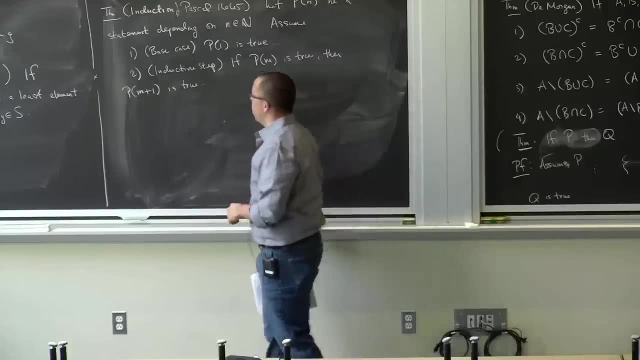 by the second property, P of 2 is true, And then again by the second property, P of 3 is true, And then P of 4.. And then P of 5.. And so, if you follow that last line of reasoning, 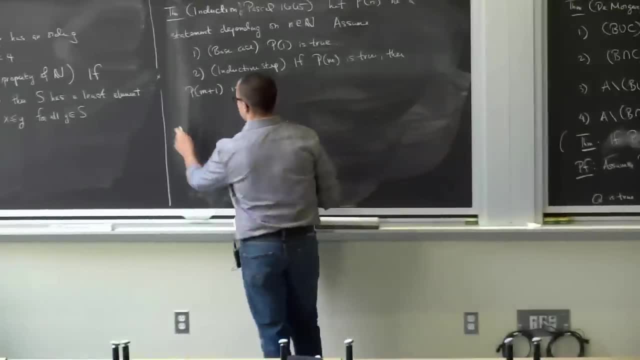 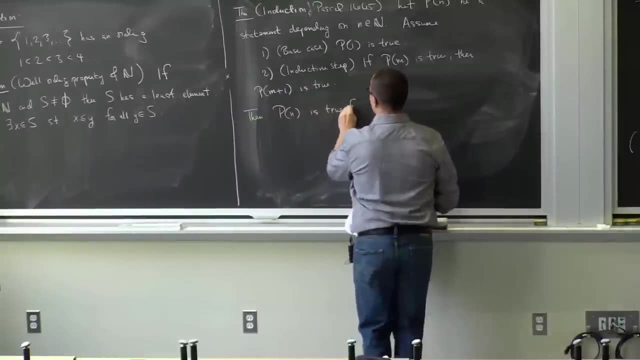 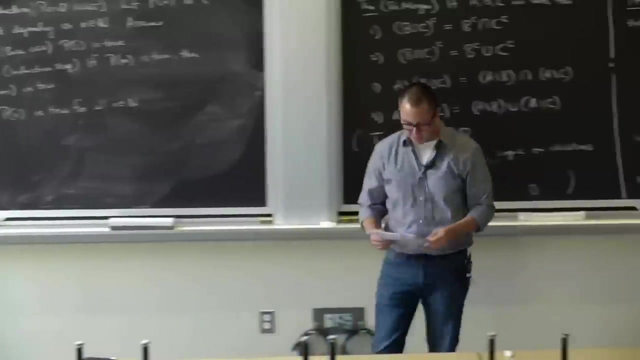 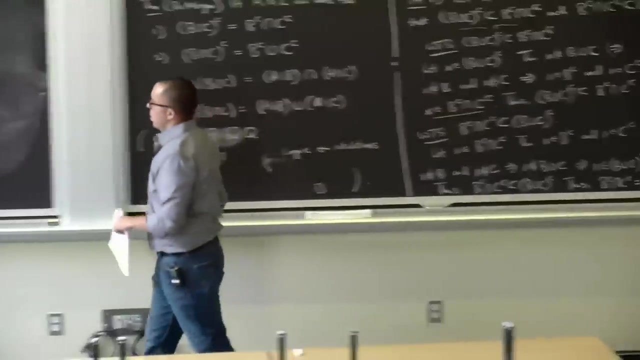 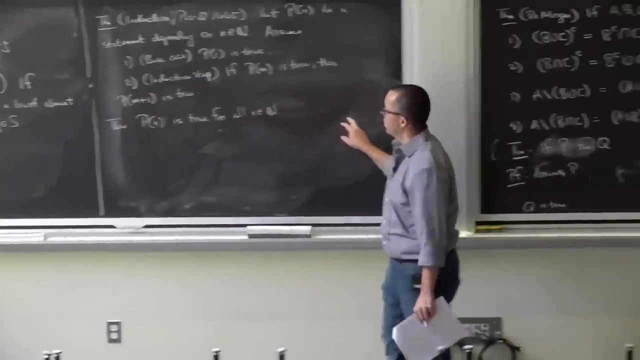 this means you should kind of be able to guess what the conclusion of this theorem is. Then Pn is true for all natural numbers. Okay, All right, So we're going to use the well-ordering property of the natural numbers to prove this theorem about induction. 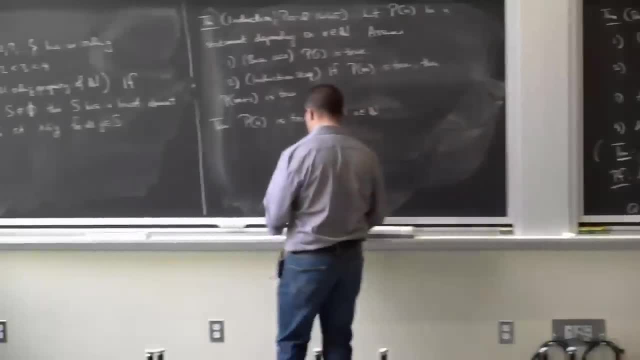 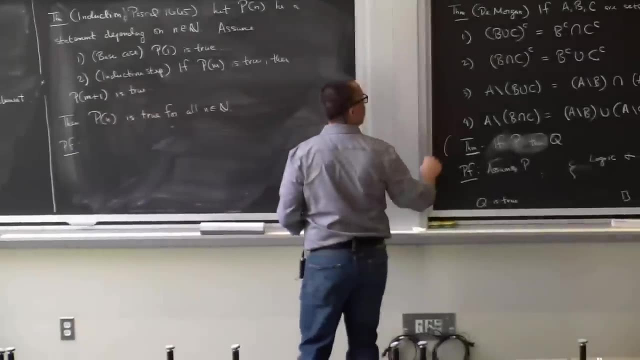 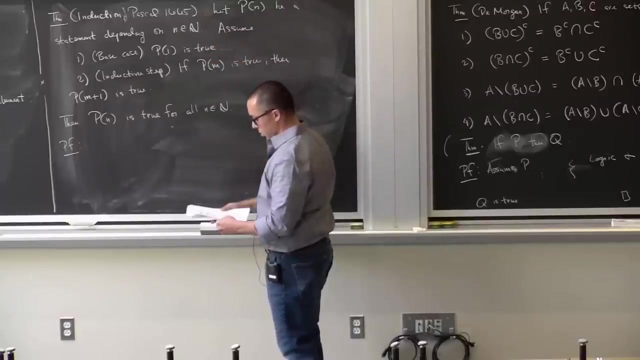 Okay, So we have our assumptions. I'm not going to- although I said, you know, over there, let B, C be sets. I'm not going- to rewrite the assumptions that we have about our statement P. We're just going to start trying to prove. 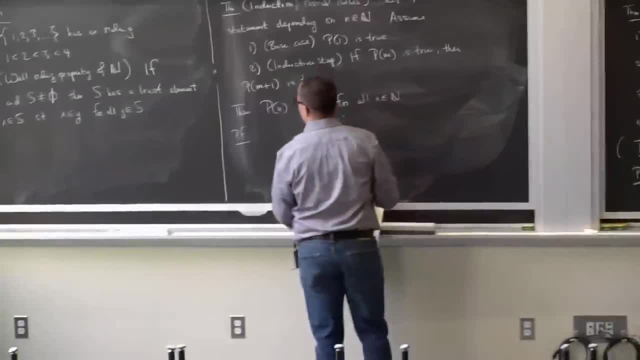 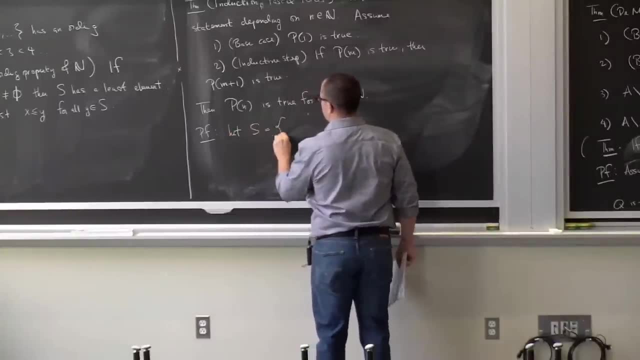 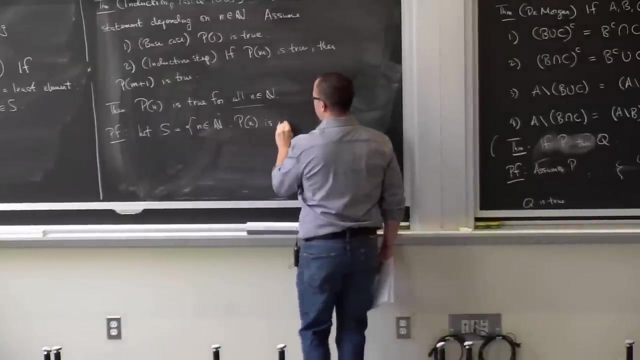 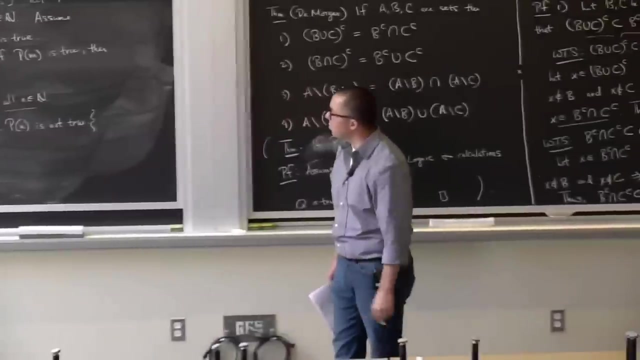 P of n is true for all n. So let me write our conclusion slightly differently. Let S be the set of all natural numbers, such that P of n is not true. So what I want to show is that P of n is true for all n. 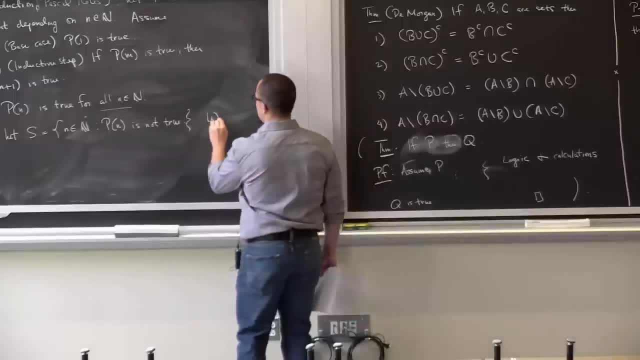 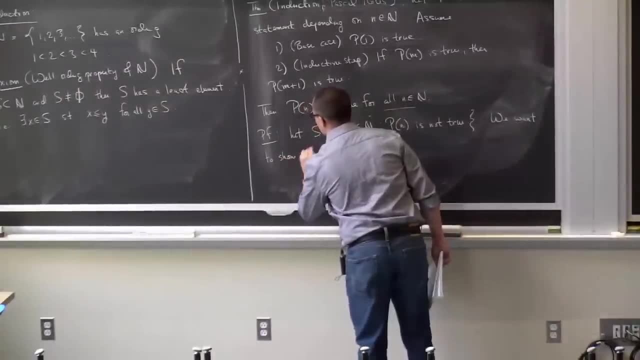 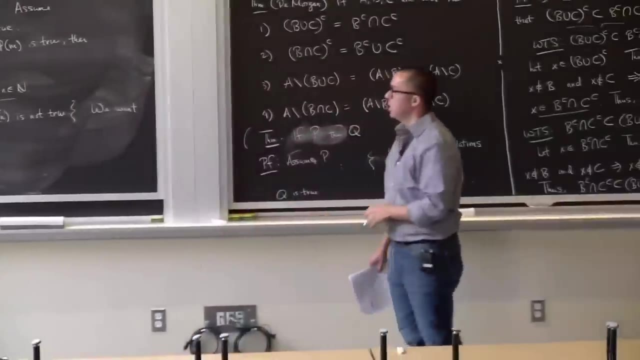 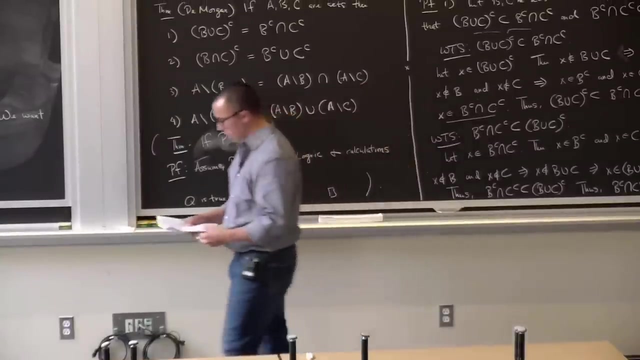 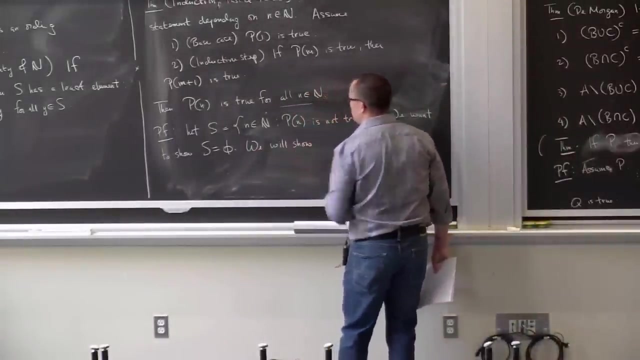 So that's equivalent to saying: we want to show that S is empty. Okay, Set of natural numbers where P of n is not true, this is empty. This is equivalent to saying P of n is true for all n, And the way we're going to do this is: 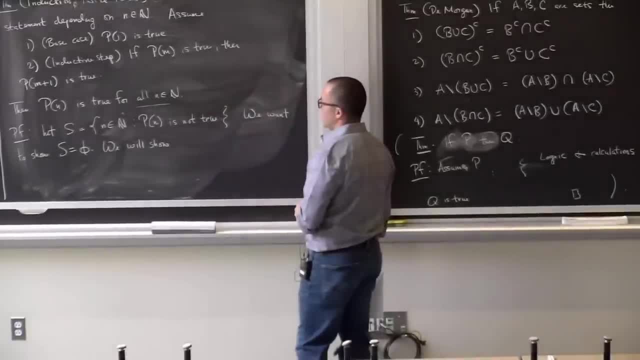 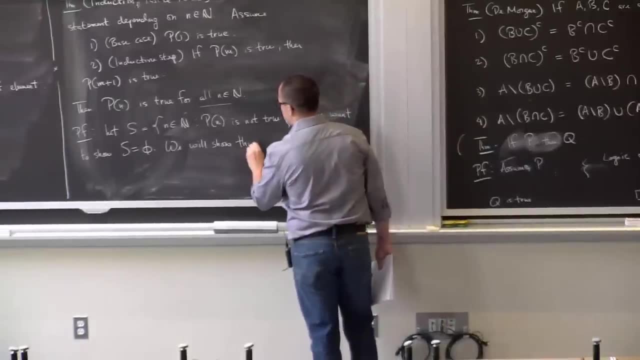 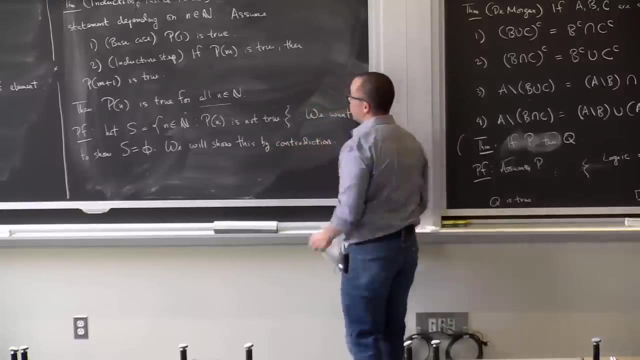 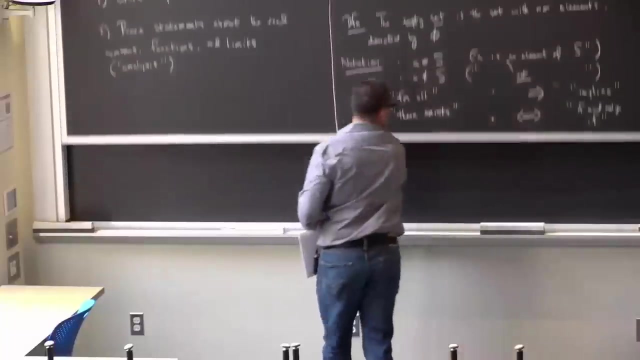 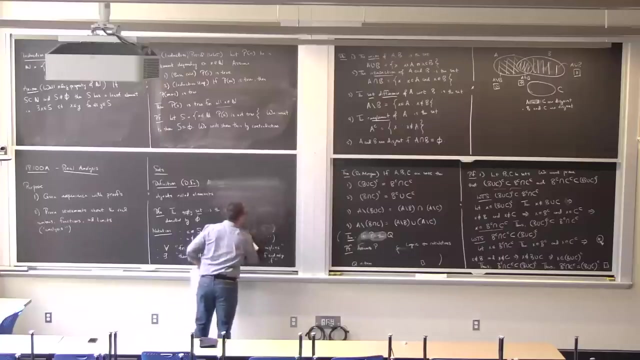 kind of another staple of mathematical proofs, is trying to prove this by contradiction. Okay, So what does that mean? Let me make a few comments about what that means. proof by contradiction. So this is the first argument You can go ahead and ask. 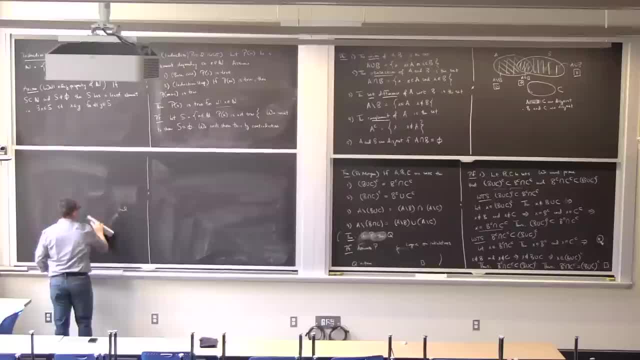 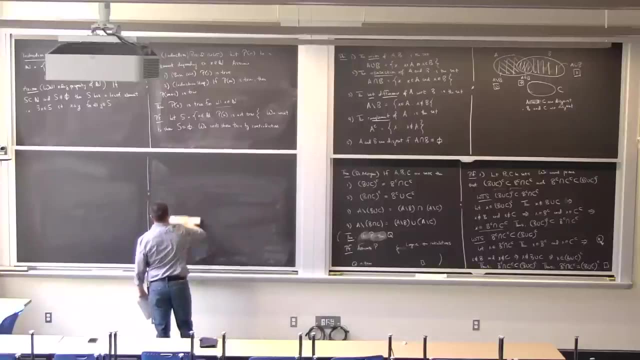 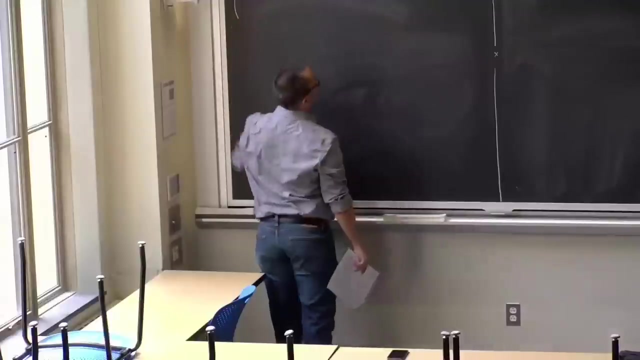 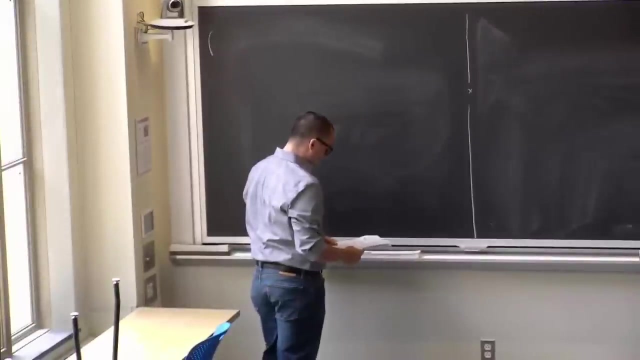 You can go ahead and ask: Okay, so in a proof, by contradiction. so this is what I'm about to write down- is not part of the proof. this is commentary not to be included in the proof. 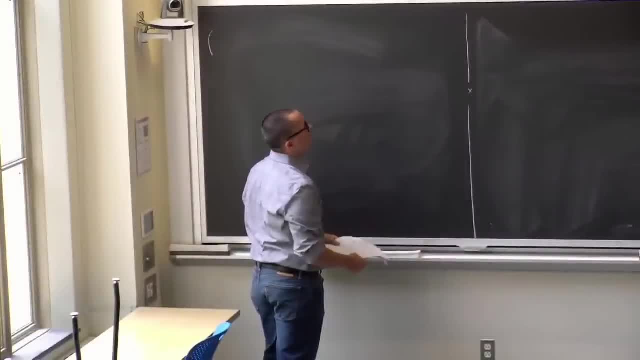 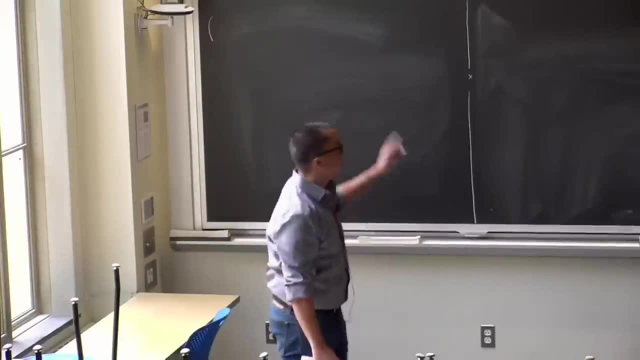 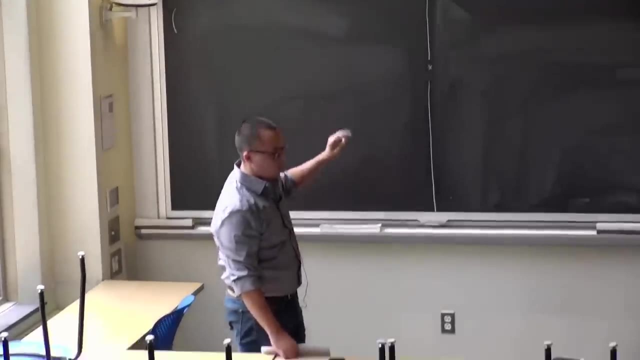 What does it mean to say we're going to prove S is equal to the empty, set by contradiction? We're going to assume that the statement we want to prove is false, not false, but we want to assume that the negation of the statement we want to prove is true, and then arrive at 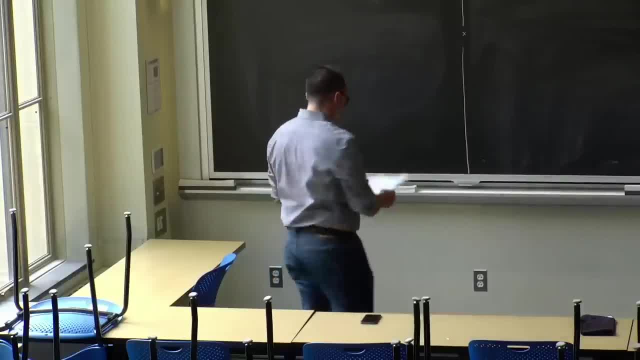 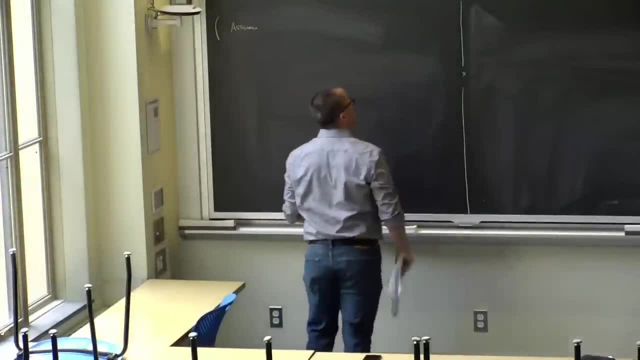 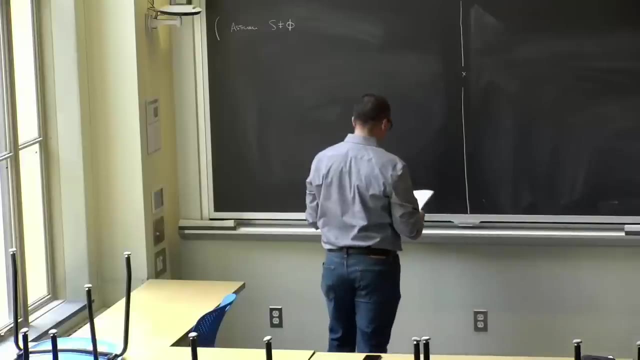 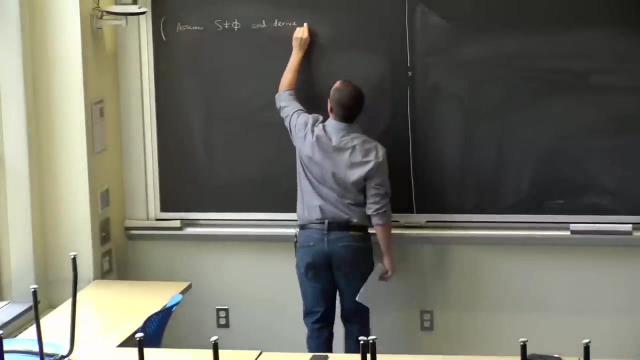 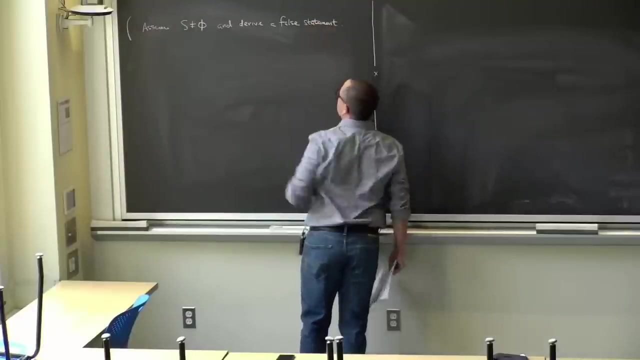 a false statement. So we want to assume this is what we're going to do. we're going to assume the negation of the statement we want to prove, namely S, is non-empty, And from this we want to derive a false statement. 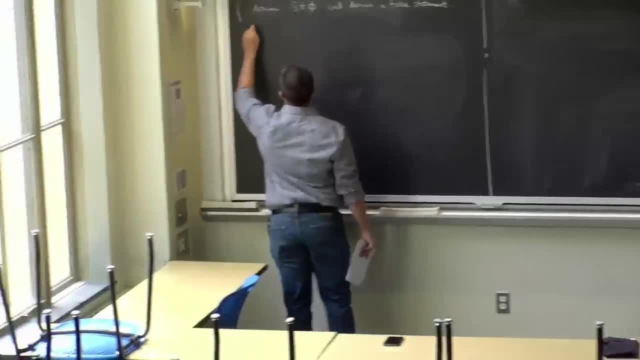 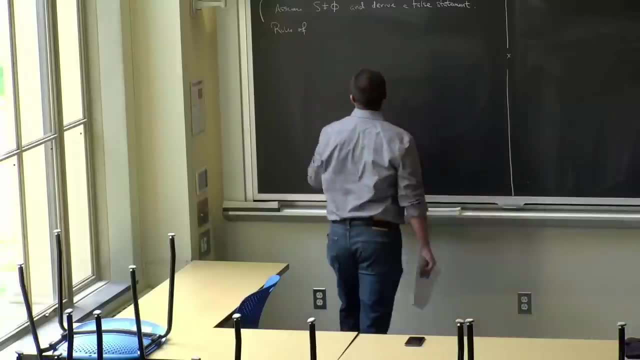 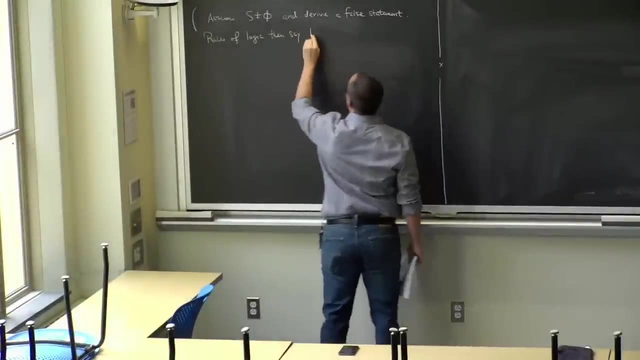 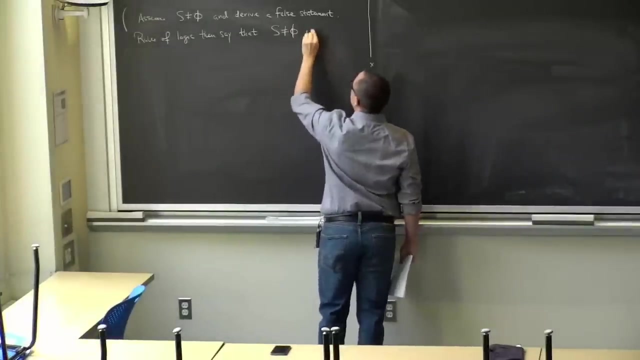 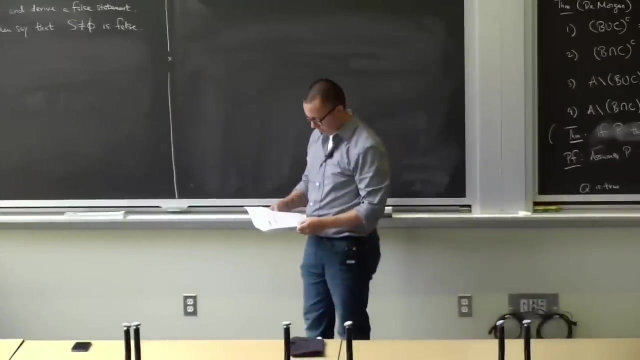 And so if we are to do, if we were able to do that, then let me just Say again- you can check in the appendix or you can just believe me- that the rules of logic then say that our initial assumption that S was non-empty is false to begin with. 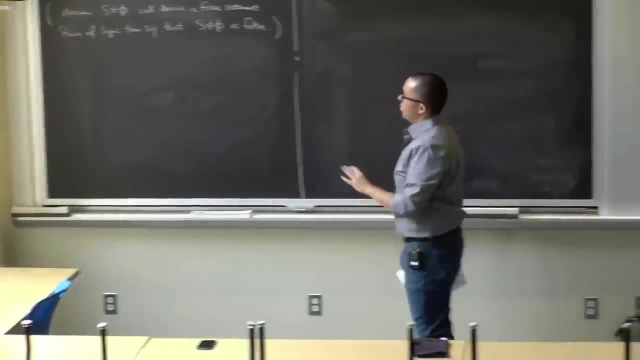 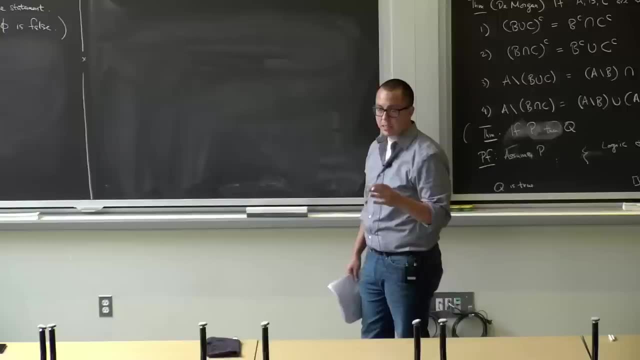 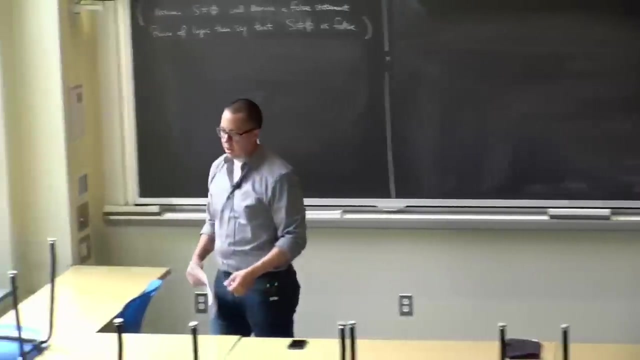 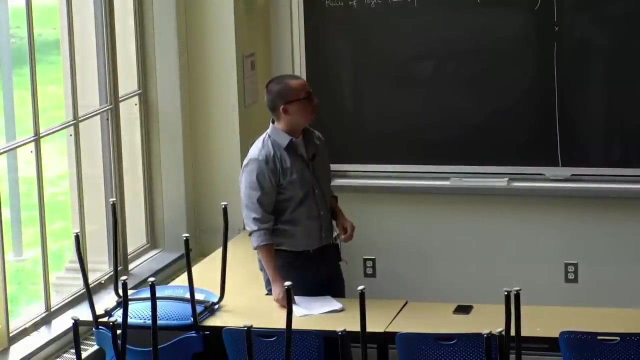 Okay, Rules of logic meaning I cannot start from a true assumption and derive in a logically consistent way a false statement. Okay, That is, if we believe that the rules of logic we're using are consistent, Which that's a little bit hairy to talk about. but you, for our purposes, of our class, you. 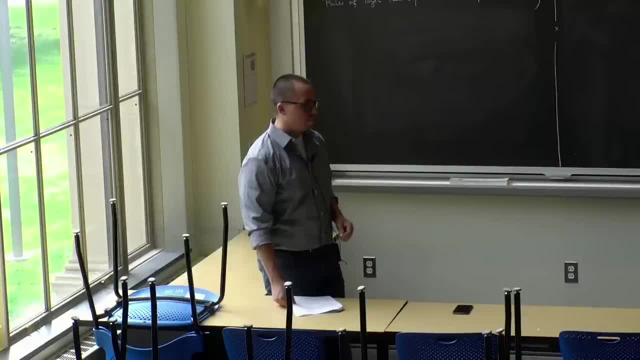 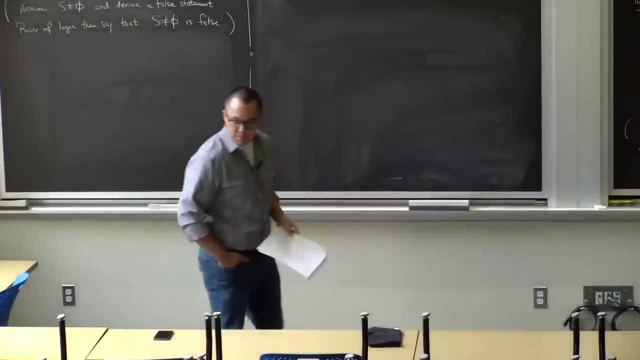 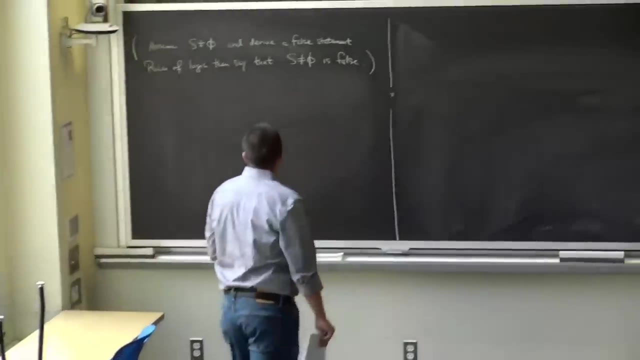 can do that, Okay. Okay, You can believe me that the rules of logic we use, or at least accept that the rules of logic we're going to use, are consistent and sound. Okay, So back to the proof. at hand, we had this set of natural numbers where the statement 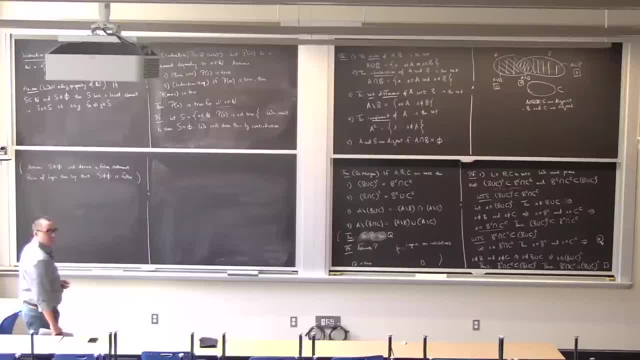 is not true. We want to show it is empty. We're going to do it by contradiction, meaning we're going to assume the negation of the statement we want to prove, Namely S is non-empty, And we're going to derive a false statement from that assumption. 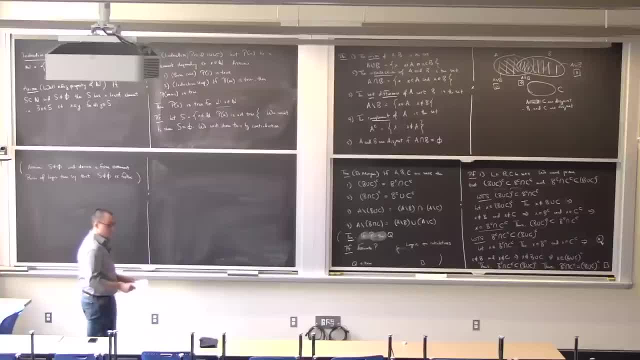 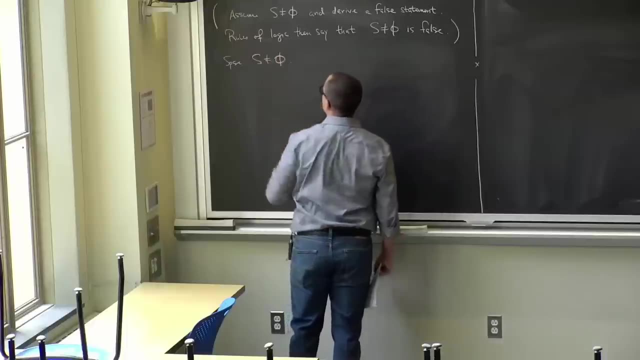 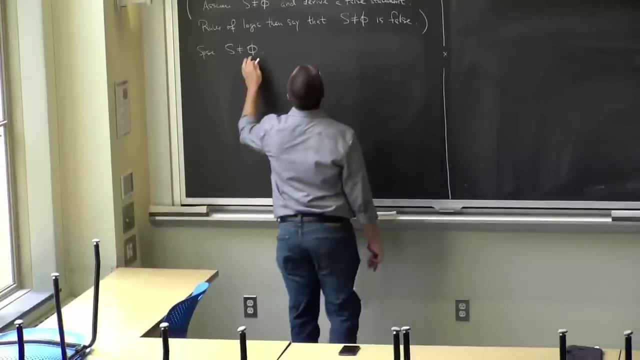 Okay, And by the rules of logic, that means that our initial assumption that S is non-empty is in fact false. Okay, All right. So towards a contradiction. suppose that S is non-empty. Okay, Now we're going to use the well-ordering property of the natural numbers. 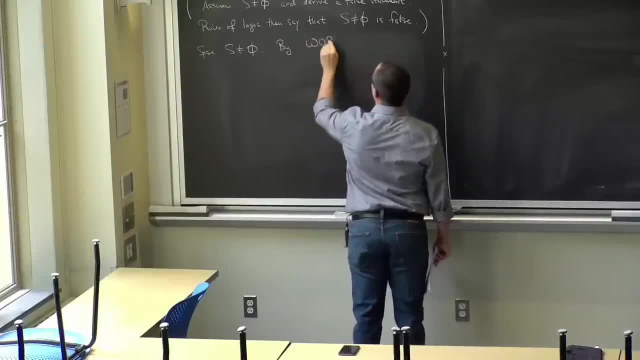 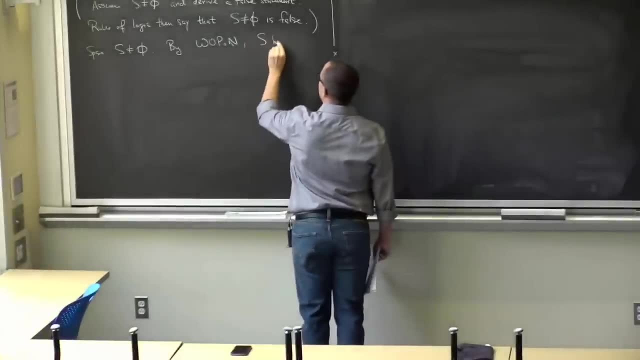 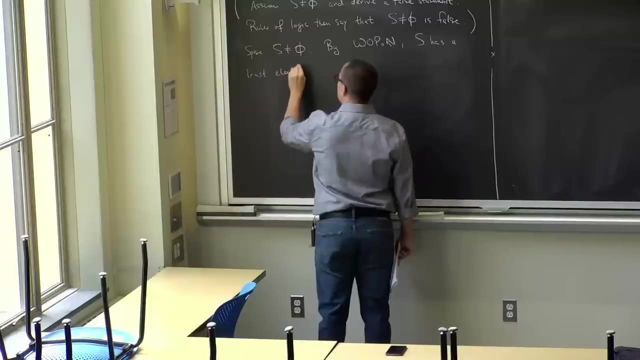 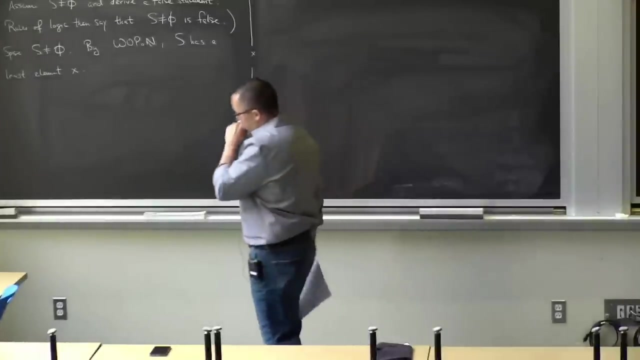 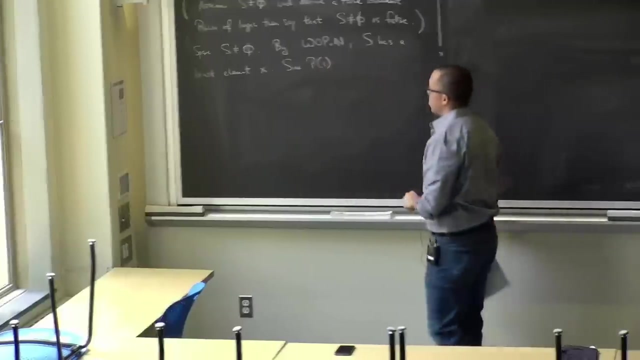 By the well-ordering property of the natural numbers, S has a least element: X. Okay, All right, All right, All right Now. what do we know about X? So, first off, X cannot be 1.. Okay, S is a set where this property does not hold. 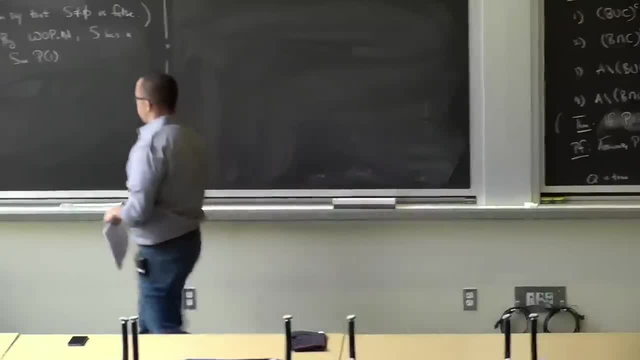 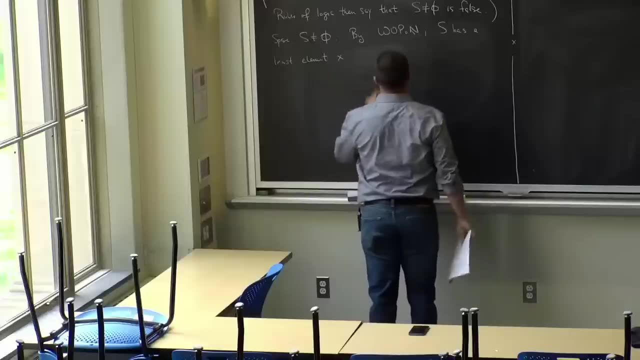 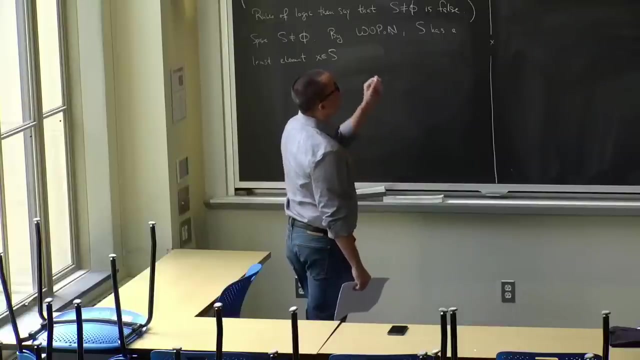 X cannot be 1 because let me again rewrite that this fact that S is a least element, Let me just reiterate that S has a least element in the set. Okay Now, X cannot be 1 because we're assuming the base case meaning P of 1 is true. 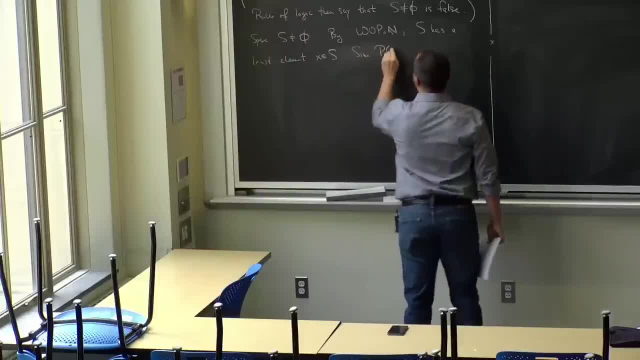 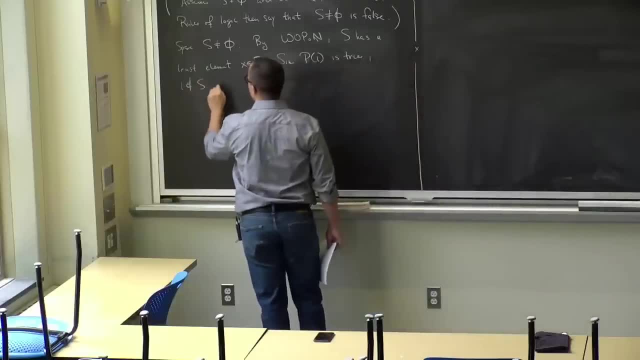 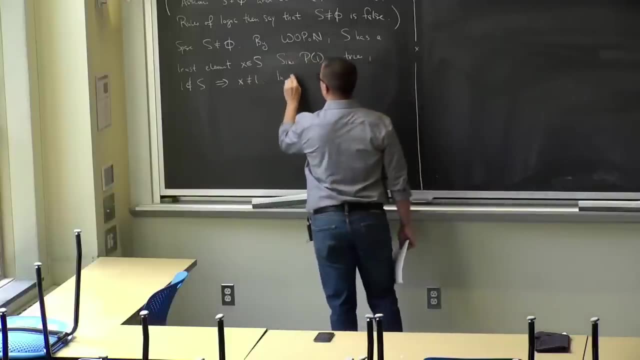 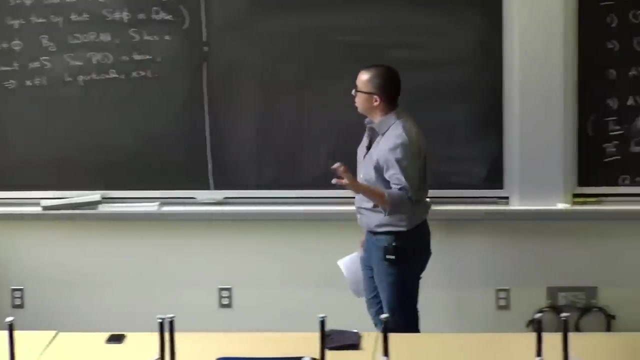 So since P of 1 is true, that means 1 is not in S, which means X is not 1.. In particular, X must be bigger than 1.. Okay, There's a magical natural number out there, bigger than 1. that's the least element of. 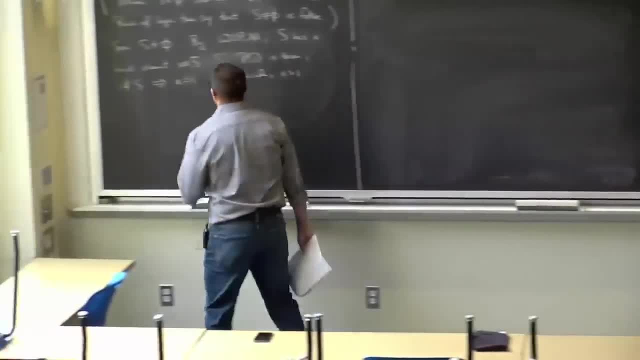 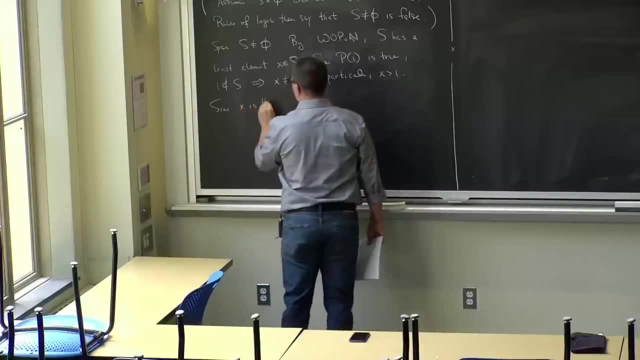 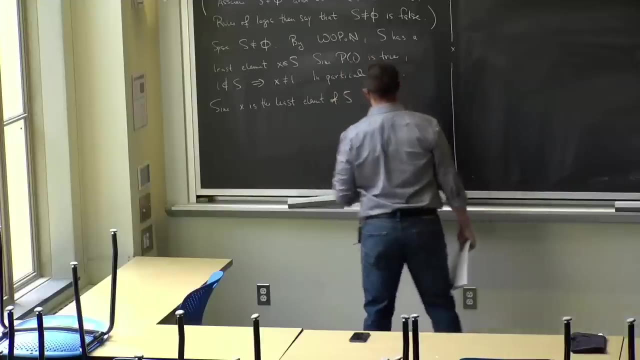 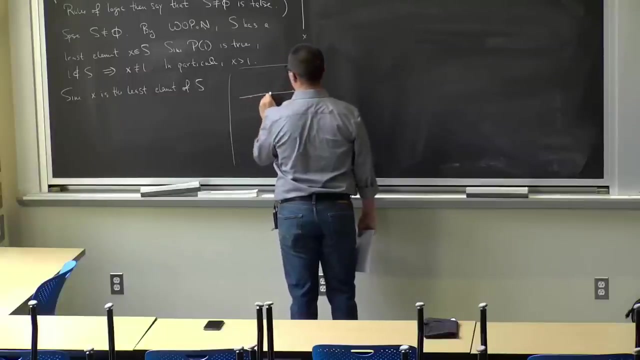 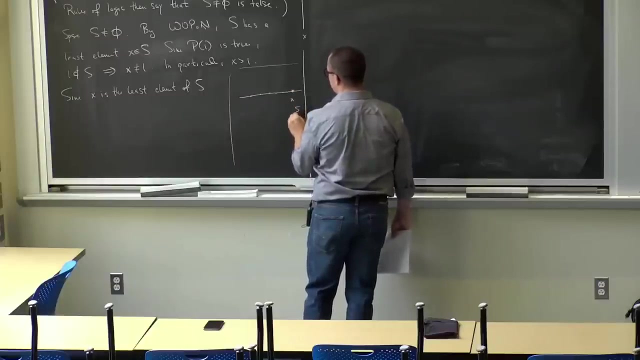 this set S. Okay, Since X is the least element of S, so let me draw along the number line. we have 1,, 2,, 3, 4.. Out, there is some magic point X, which is the least element of S, and the rest of the. 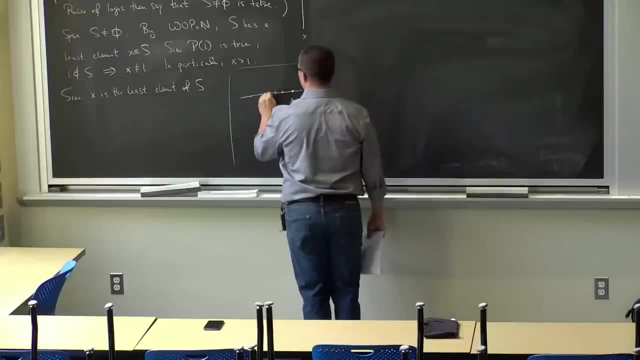 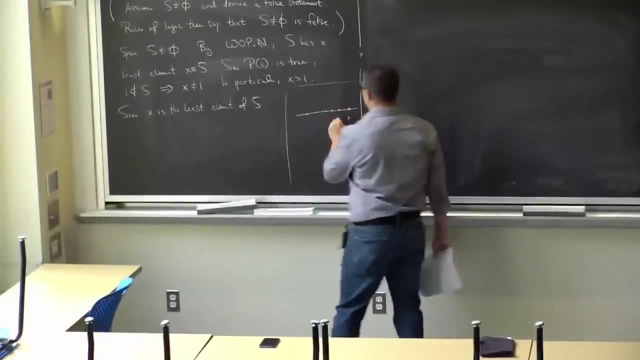 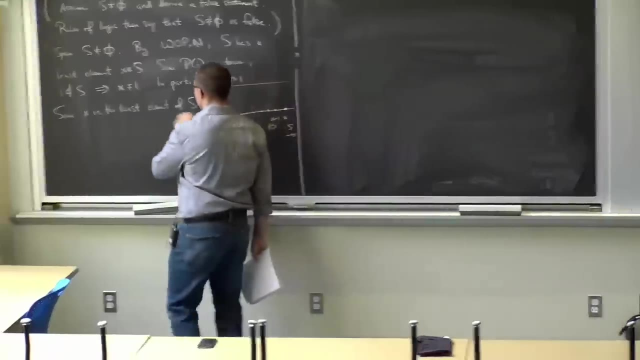 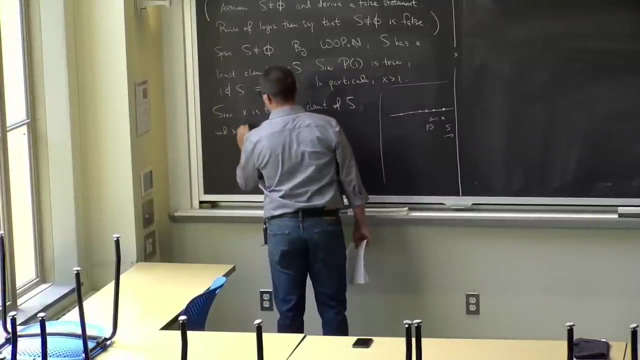 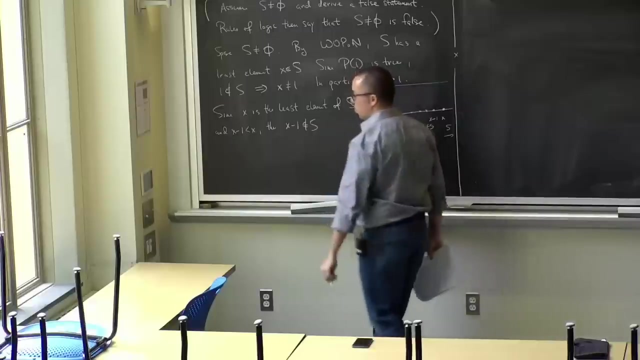 subset S lies to the right of this number, X. Right, Because it's the least element of S And therefore X minus 1 cannot be in S. So, since X is the least element of S, And Okay, All right. So if X minus 1 is less than X, this means that X minus 1 is not in S, Otherwise it. 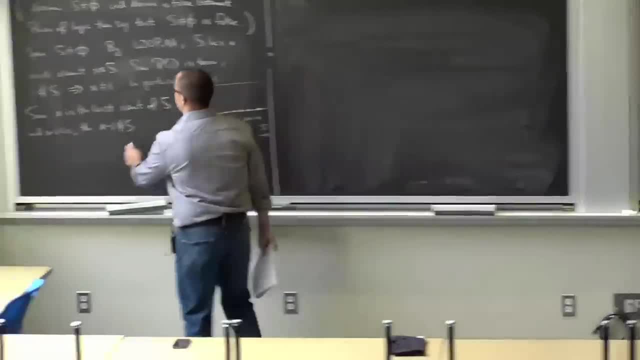 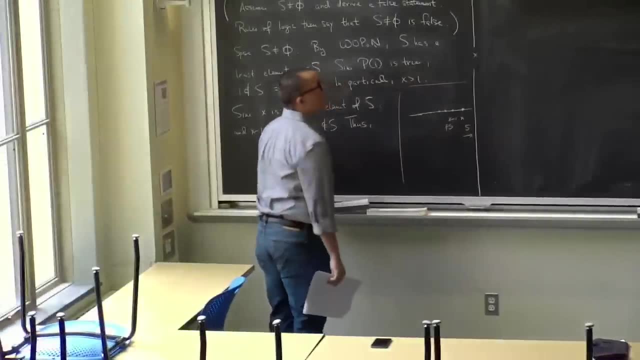 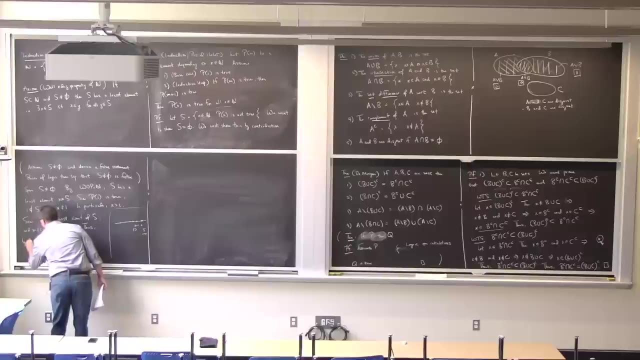 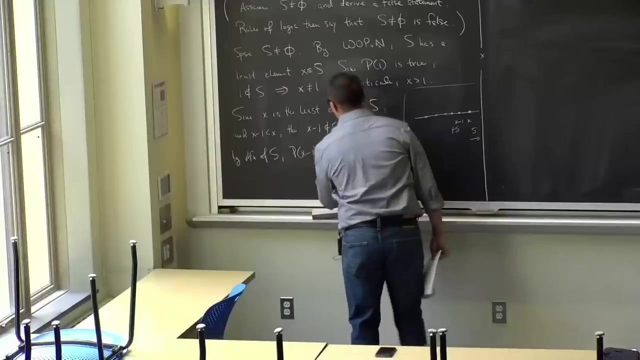 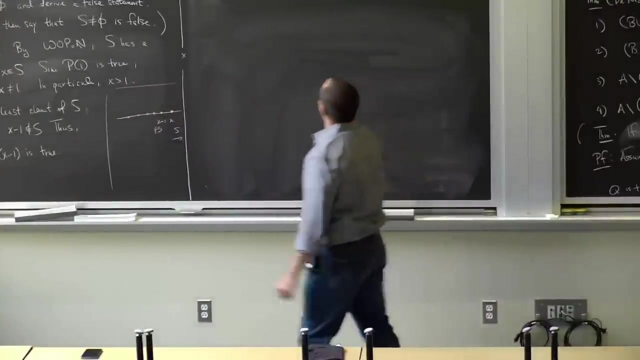 would be a smaller element than X in S. So thus, what does it mean to not be in S? It means that P of X minus 1 is true By the definition of S. Okay, This means P of X minus 1 is true, okay. 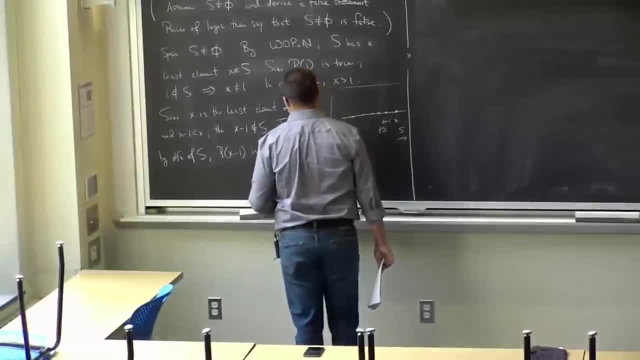 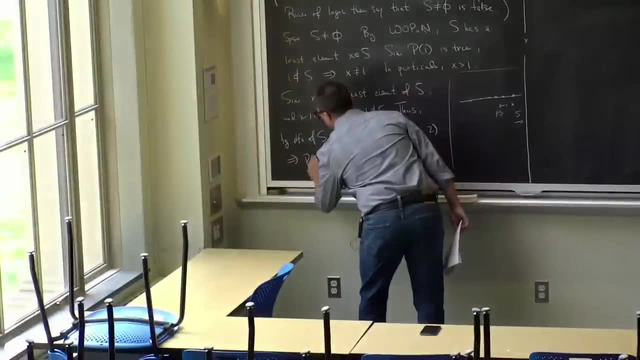 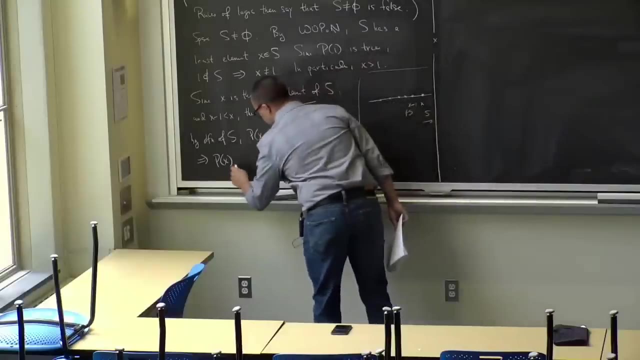 But by the second property we're assuming about our statement P. this means that the next guy in line, X minus 1 plus 1, is true, which is just X. Okay, All right. Next one comes in, Which means that X is not in S. 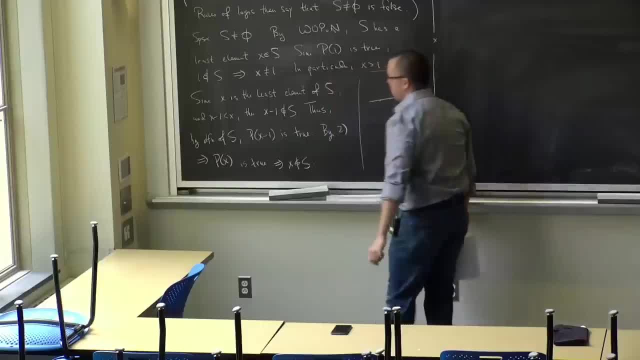 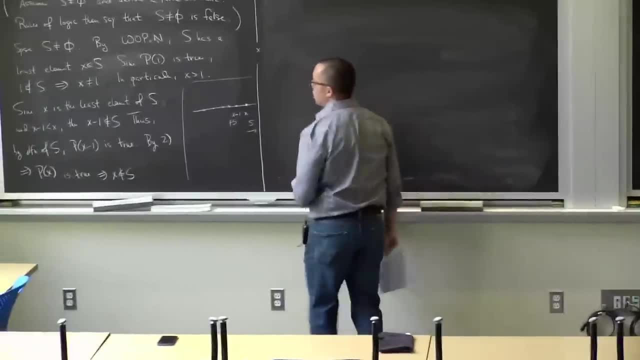 Okay, So let me just recap. From the assumption that S is nun empty, we've derived two facts: One, that X has the least element in S, and that element is also not in S. And let me find the two most Kafkaian arguments that the Covid one has come up with. 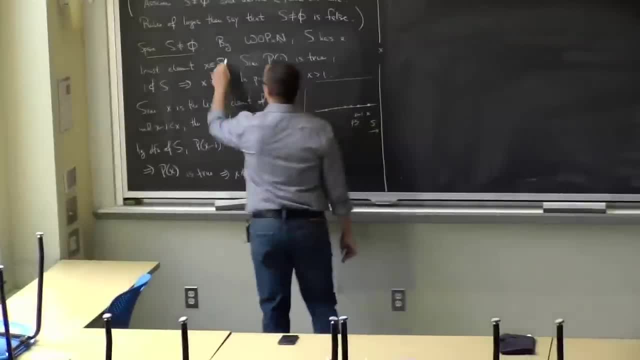 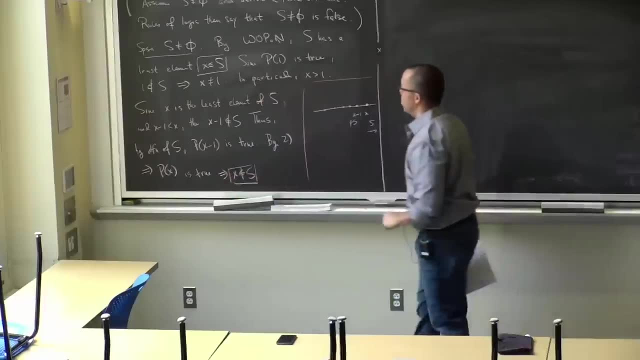 What did Y equal at And what will P lead to? Right, Yeah, Tell me about P, please. Yeah, iedz, I mean P. Nice idea, A move that actually does the same number of parameters with P. I agree with you. 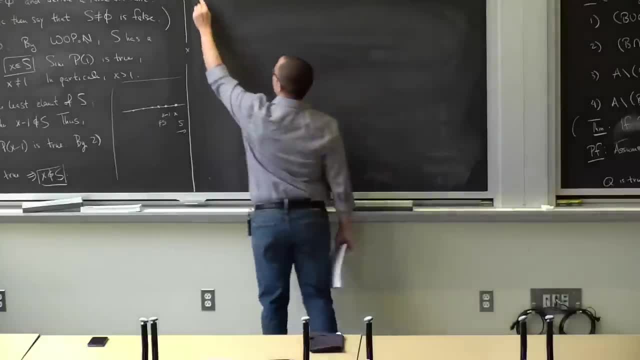 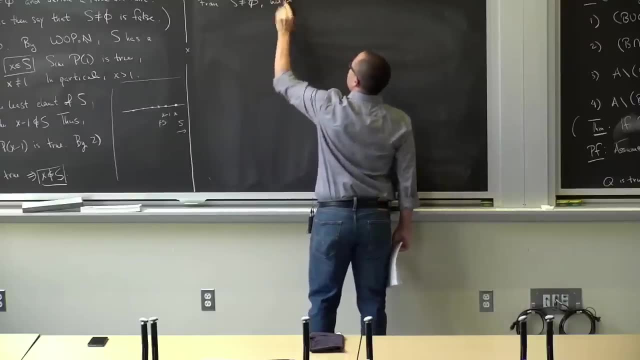 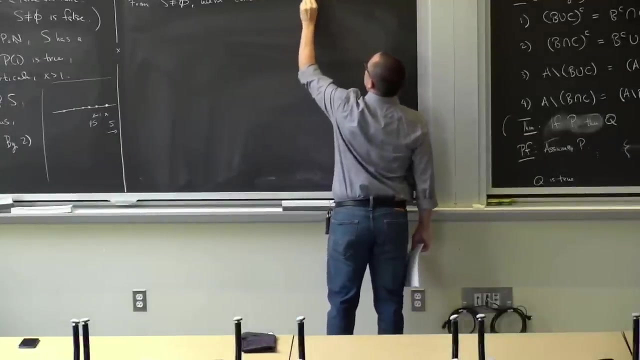 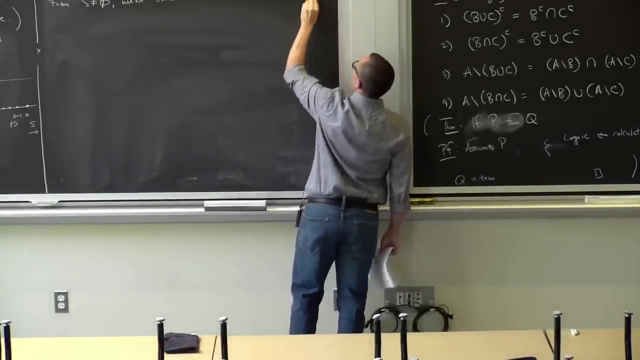 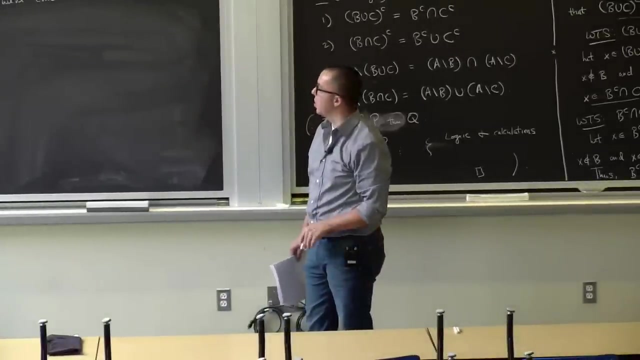 Okay, good Thanks, Okay, OK, Bye. See you next time, Bye, Bye, Bye. So written out. we've concluded there exists a natural number which is both ns and not ns, And this is a false statement. You cannot have an object, a member, that's both in the set. 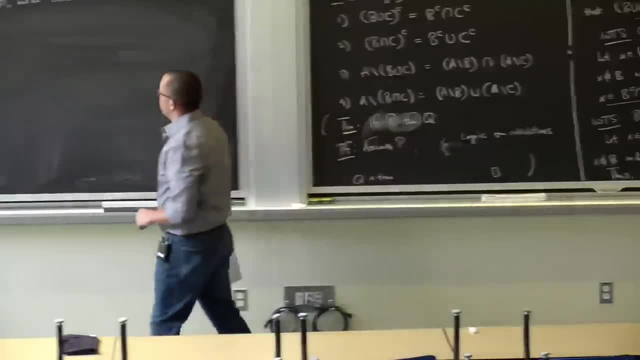 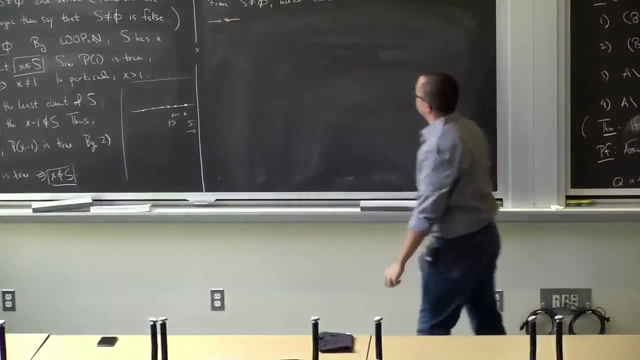 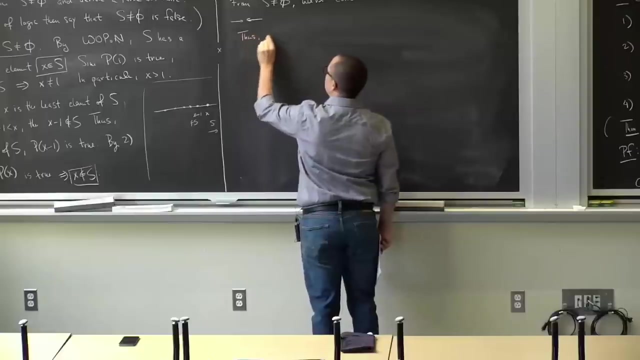 and not in the set. And at the end of contradiction arguments I'll usually put two arrows hitting each other. So that's a contradiction. Therefore, our initial assumption that s is non-empty has to be false And therefore s is the empty set. 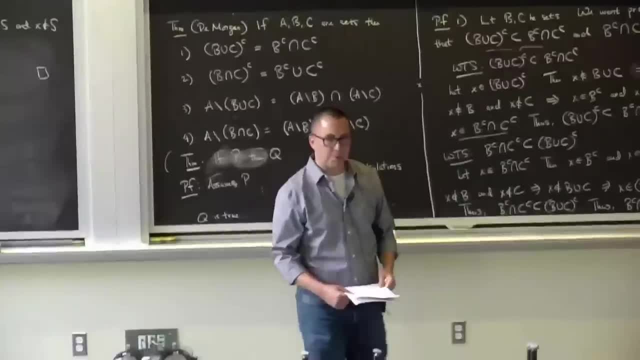 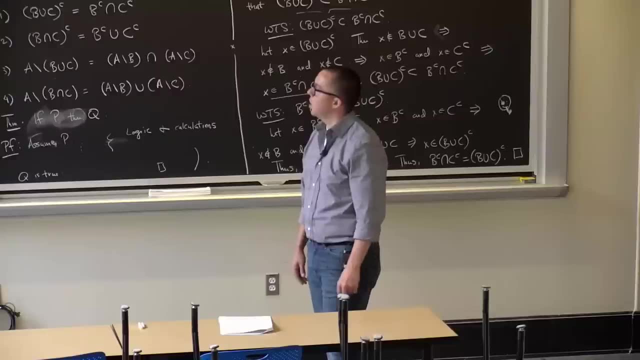 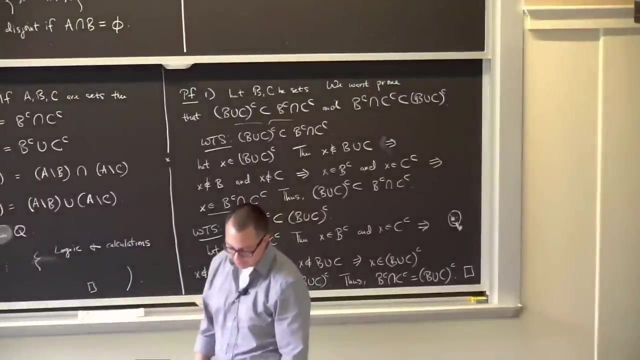 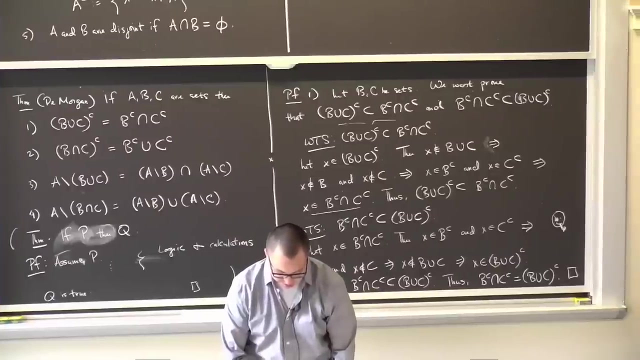 So I encourage you to go through that proof a little slowly, because maybe you got turned around by taking the complements or the general scheme of how a proof by contradiction works. But don't spend too much time on it because, as I've said, 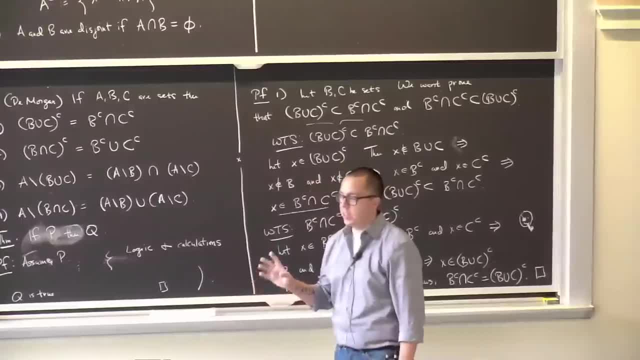 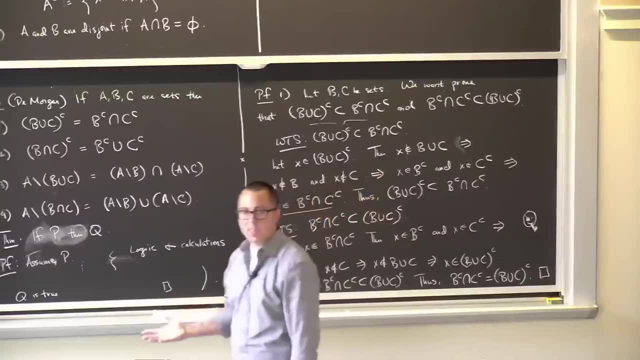 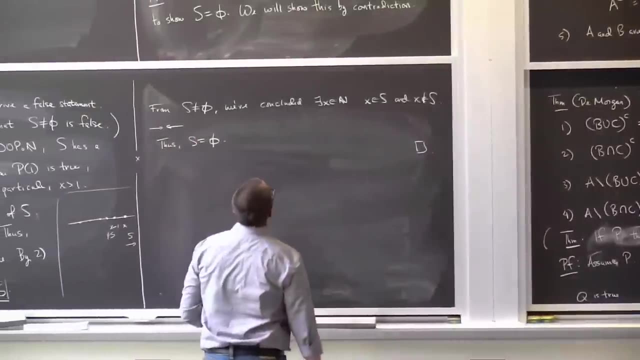 this theorem itself and its proof are not the thing we're really interested in, Or at least it's not the most interesting. It's more of a tool that we'll use to prove more interesting statements. So how do we actually use this theorem? induction: 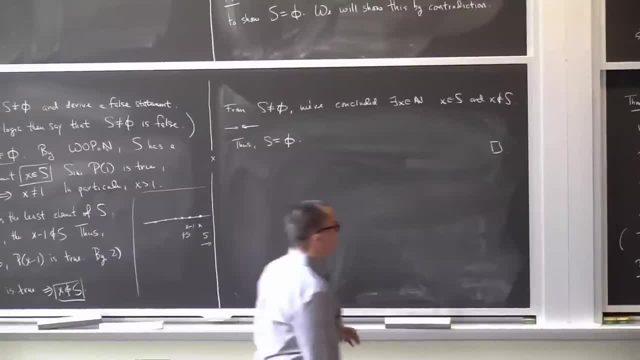 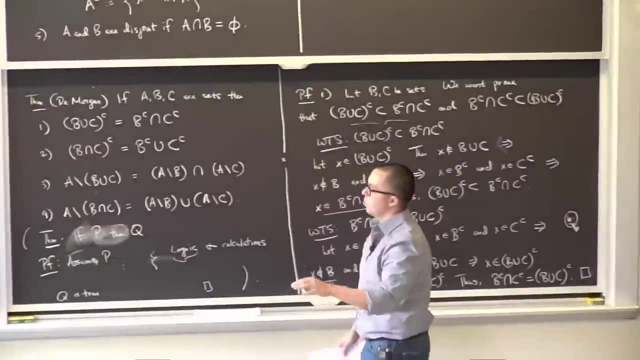 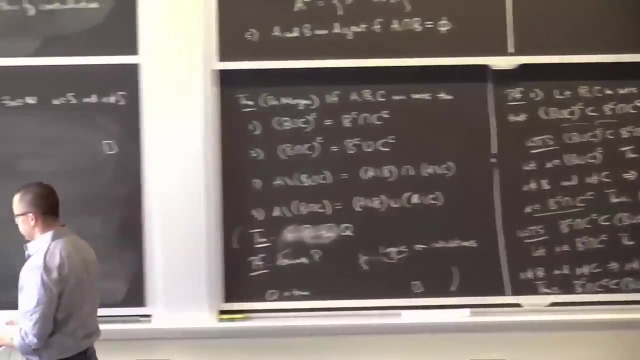 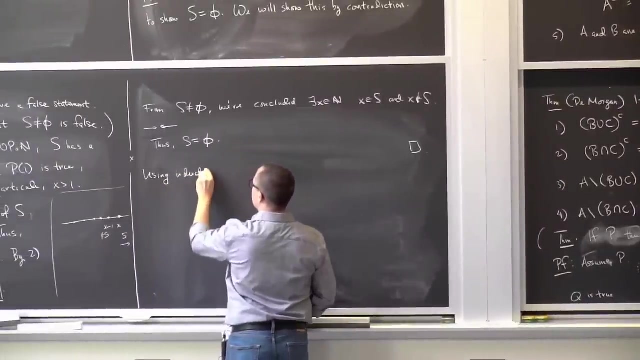 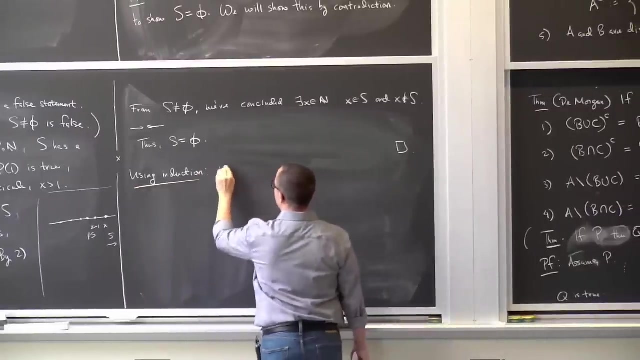 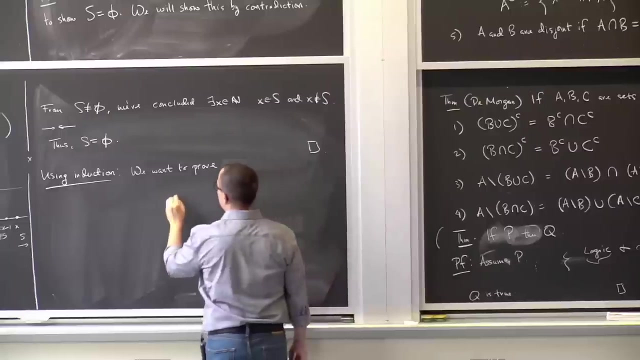 to prove other statements. So I guess I should include this here. This falls under the umbrella of logic, meaning we're going to use previous statements we've proven to prove new statements, But anyway. So how do we use induction in practice? So if we want to prove some statement for all, n pn is true. 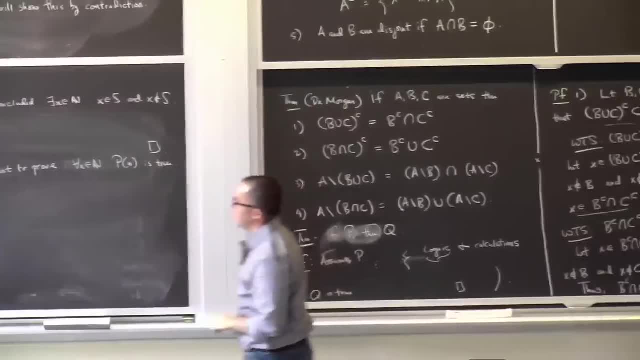 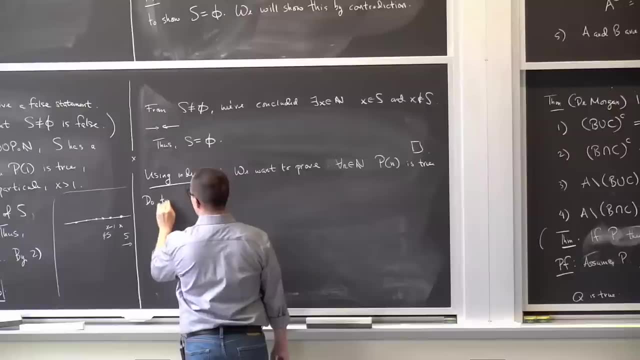 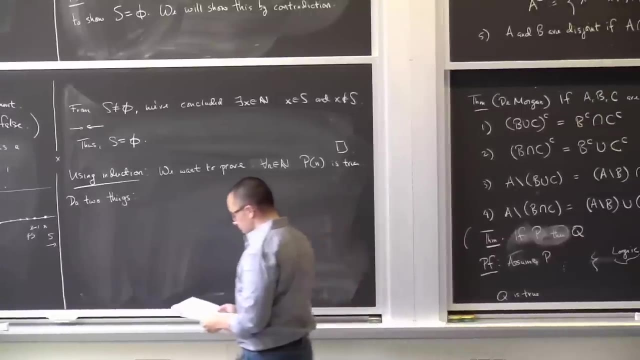 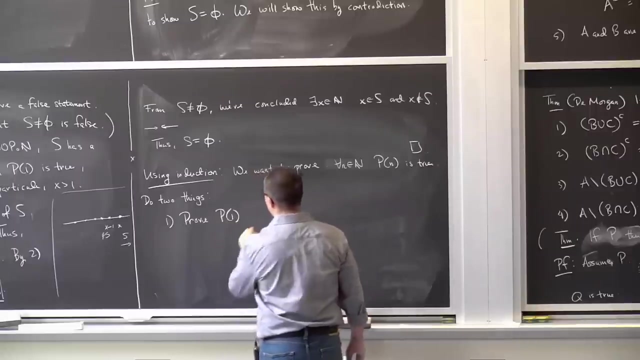 So if we want to prove some statement for all n pn is true, And then this theorem about induction, this theorem of induction tells us, we just have to do two things. We have to prove the base case, And this is usually easy. 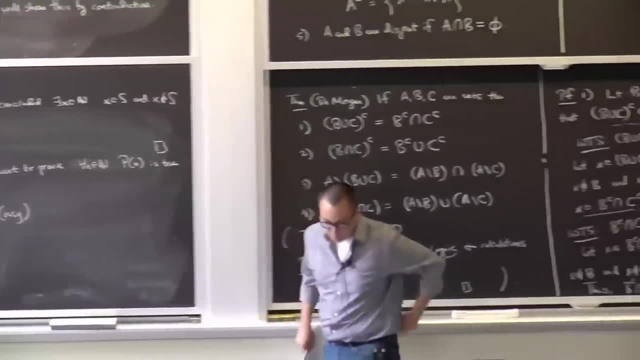 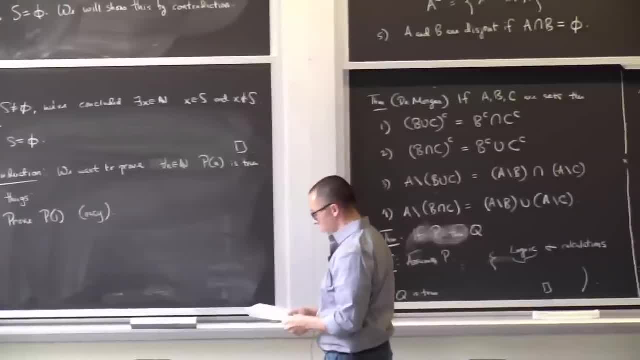 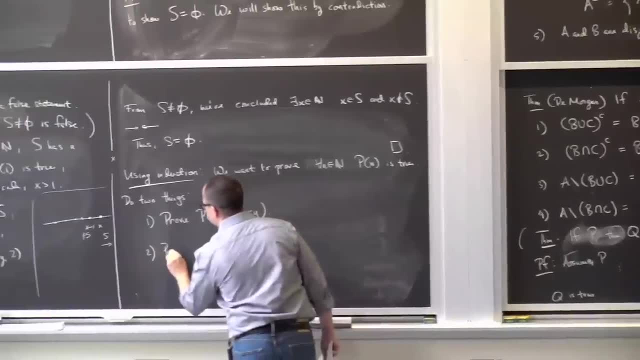 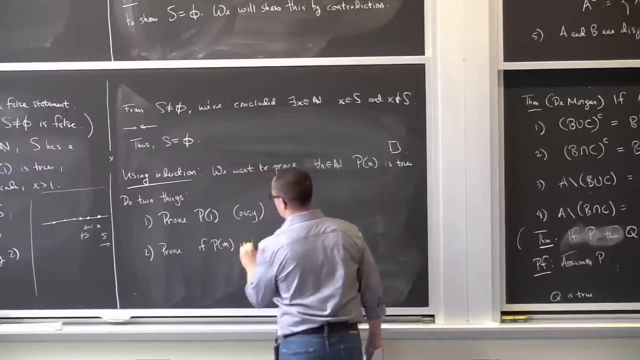 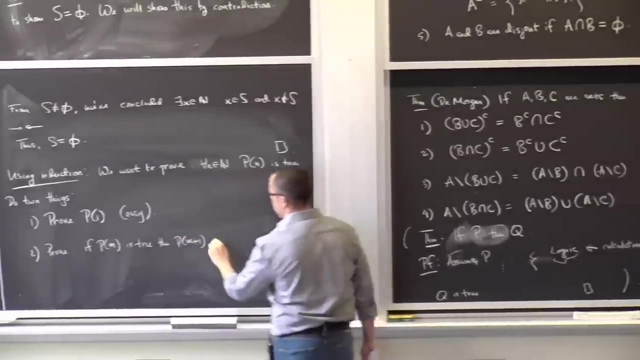 And the second step is usually, or the second thing we have to prove, is the more involved part, which is we have to prove that the statement that if pn is true, if pn is true, then p of n plus 1 is true, 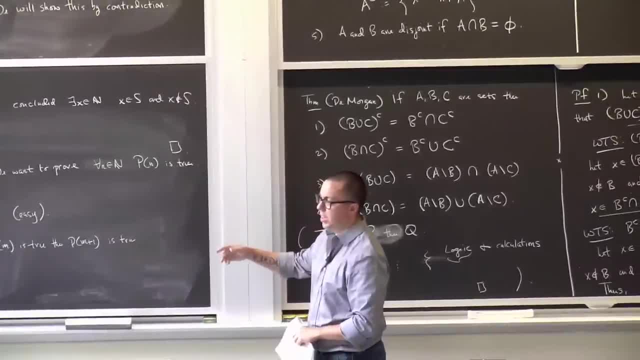 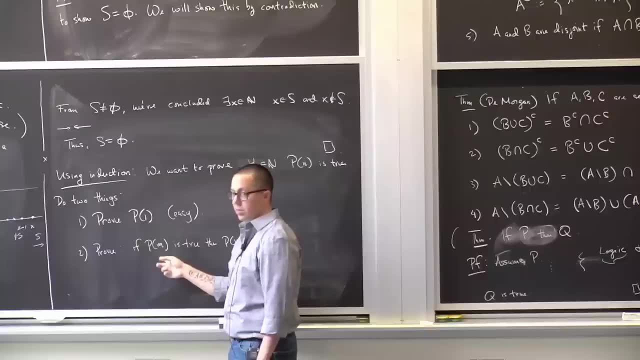 It's kind of, if we want to do a proof by induction, there's kind of two smaller proofs we have to do. First we have to prove p of 1 is true And then we have to prove this statement: If p of n, then p of n plus 1.. 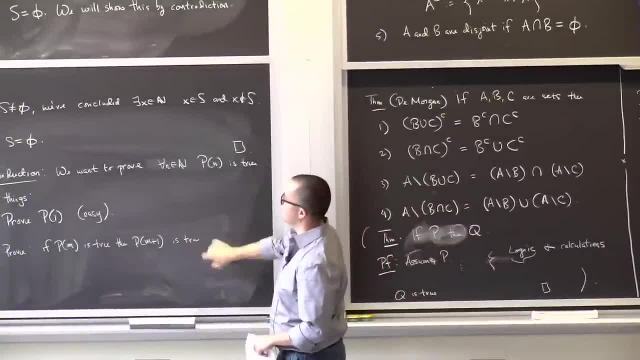 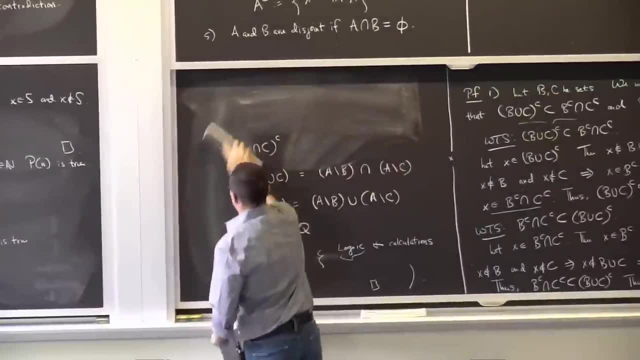 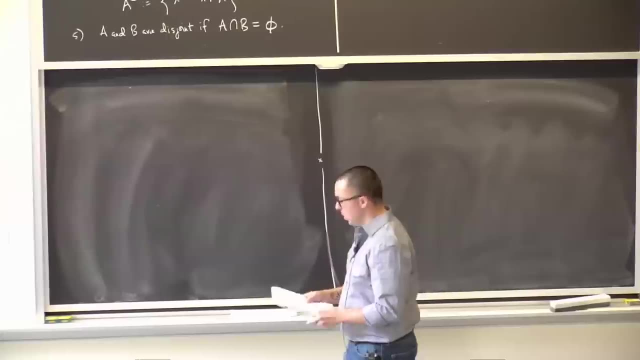 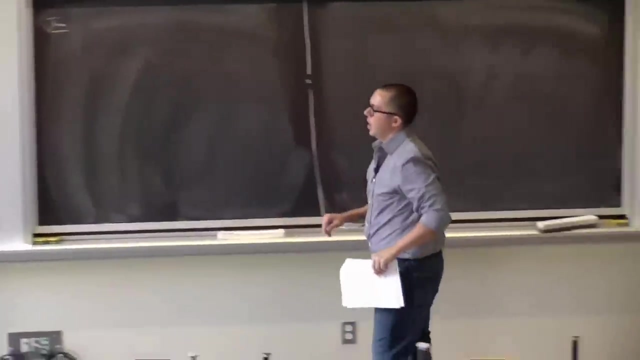 So again, This is usually referred to as p of n plus 1. This is usually referred to as the base case. This is the inductive step. So let's try and actually do this. All right, So another question I get at the beginning of a course. 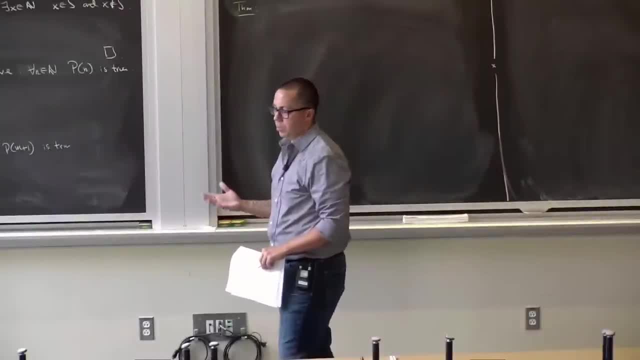 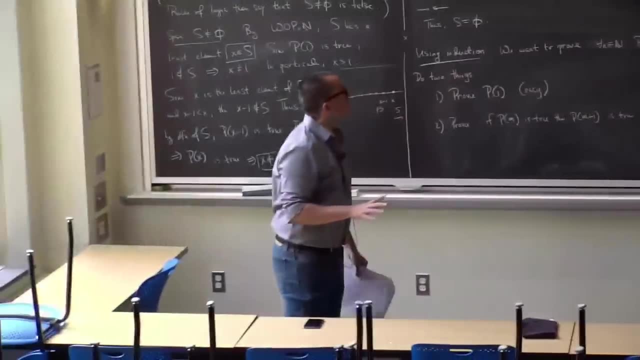 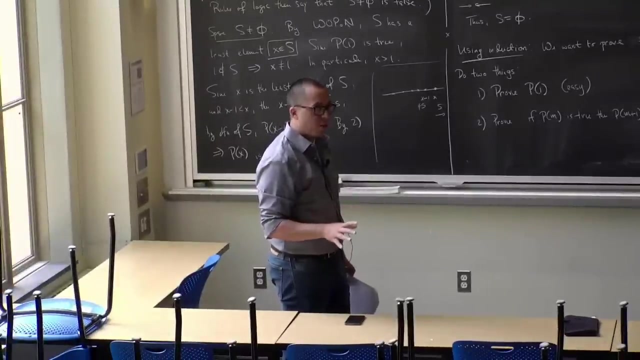 especially about proofs, because there's a lot of uncertainty about what you can assume is true. What can you use? What can you not use Right now? at this point, you can use whatever you know about any of the algebraic properties. you know about the real numbers, the rational numbers. 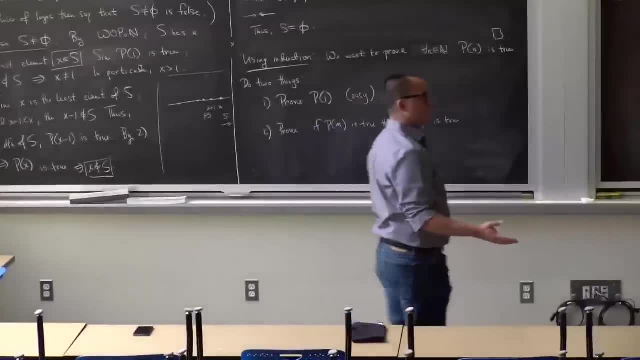 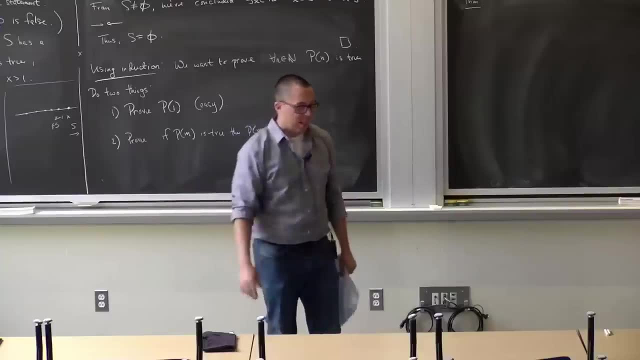 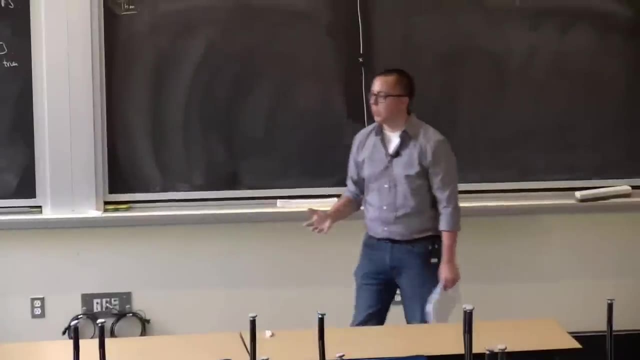 And by algebraic properties I mean if a plus b equals c, then a plus b times d equals c times d. OK, And what you know about inequalities. So we're going to go much more in depth into ordering, which is what inequality is a part of. 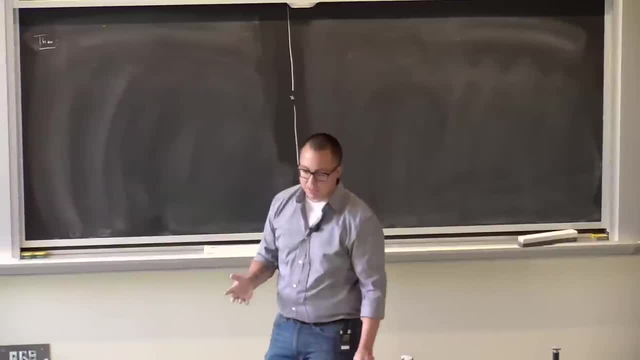 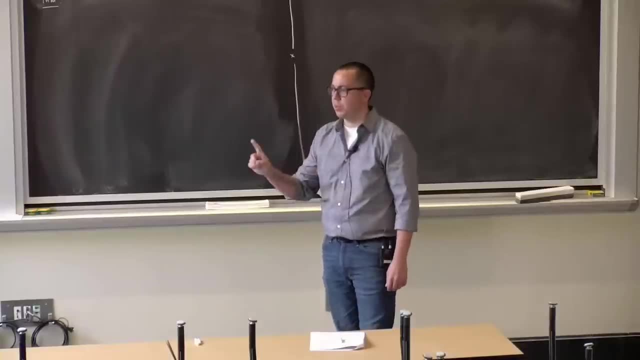 But you can use all the properties you know about solving inequalities or manipulating inequalities. Meaning if I have one number is less than or equal to another number, then when I multiply both sides by a positive number, that doesn't change the inequality. So you can use all of these algebraic properties. 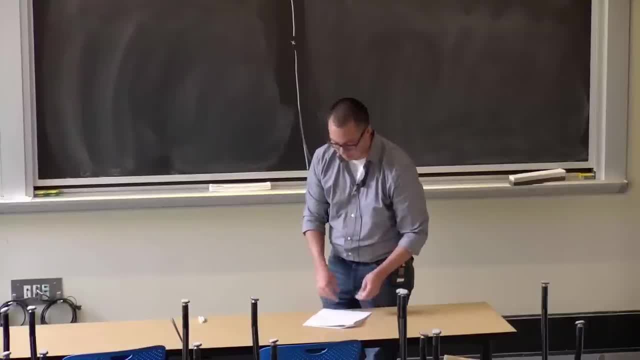 of rationals and real numbers. from here on out There will be at I mean so we're going to be proving things about calculus. So you certainly cannot use anything about continuity, differentiation or anything like that, But for now you can use all the algebraic properties you know. 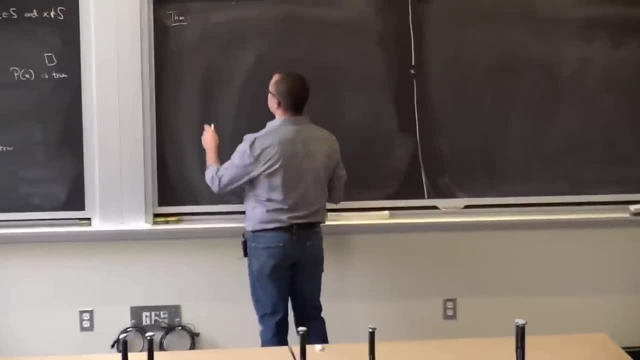 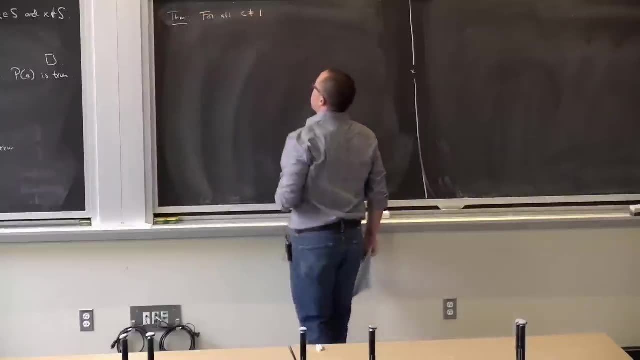 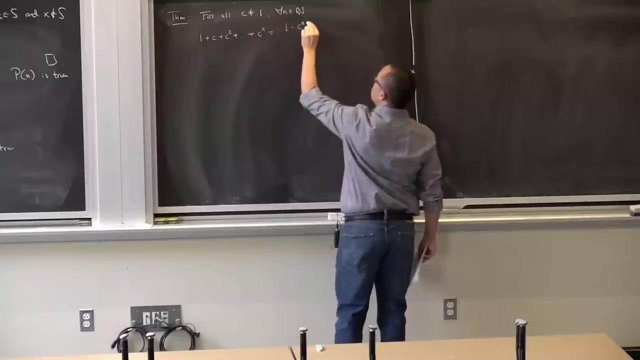 So the first one, The first statement we're going to try and prove using induction is the statement that for all c not equal to 1, we're all in a natural number: 1 plus c plus c. squared plus c to the n equals 1 minus c, to the n plus 1 over 1 minus c. 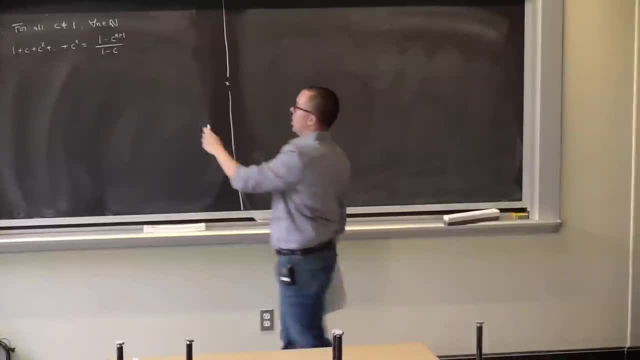 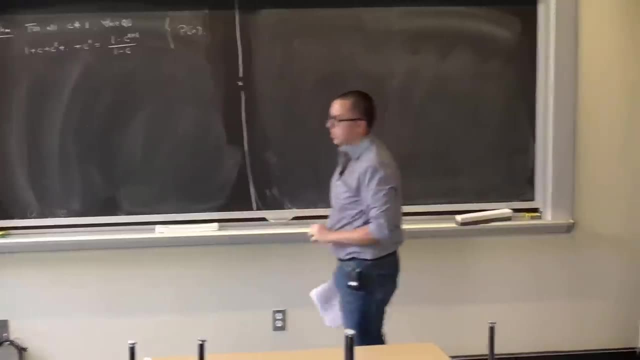 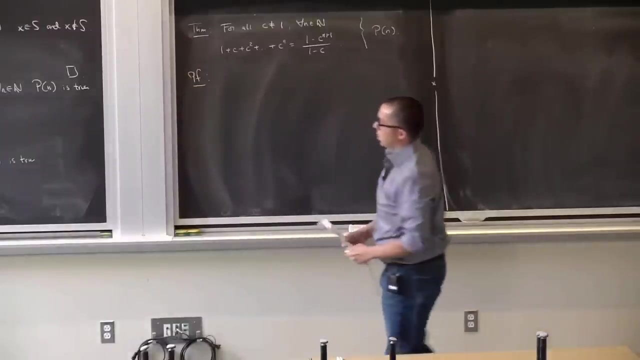 OK. So This here is our statement: p of n Depends on a natural number, n. OK, So we're going to do this by induction, which means we're going to do those two things. We're going to prove the base case, p of 1, which I said. 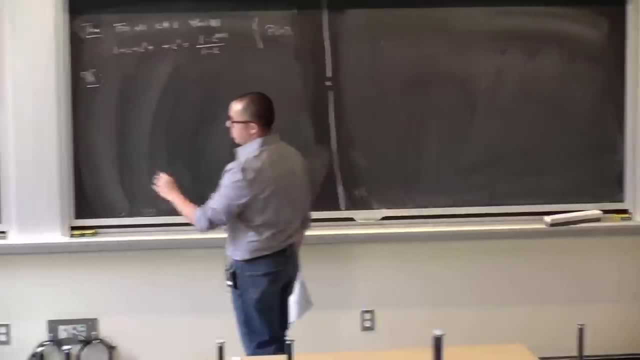 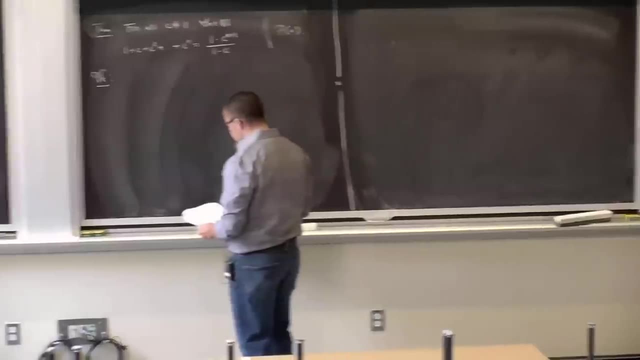 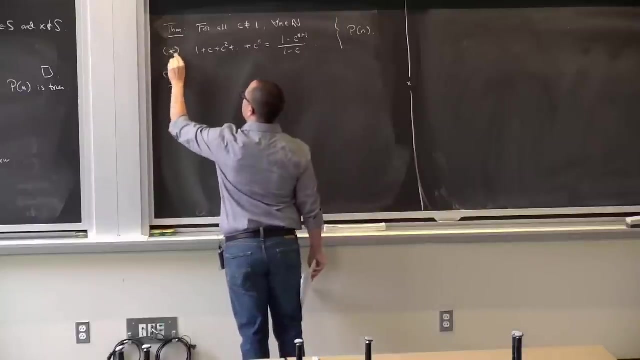 is easy. And then we're going to prove the second case, the second property, the inductive step, which is a little more involved, but not so much involved, at least in the beginning. So let me call this inequality star. 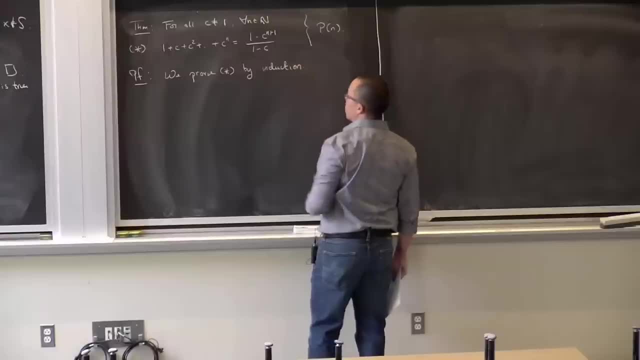 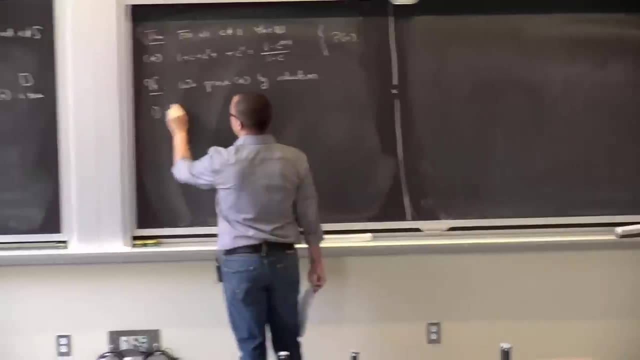 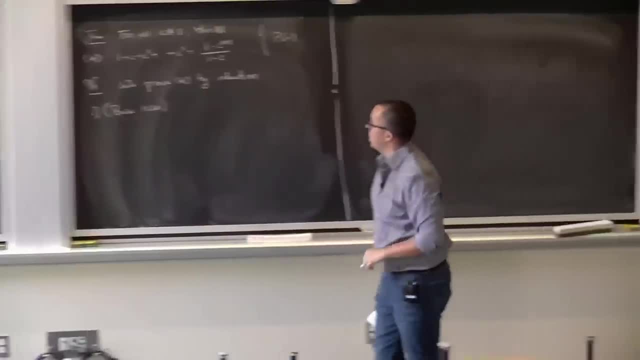 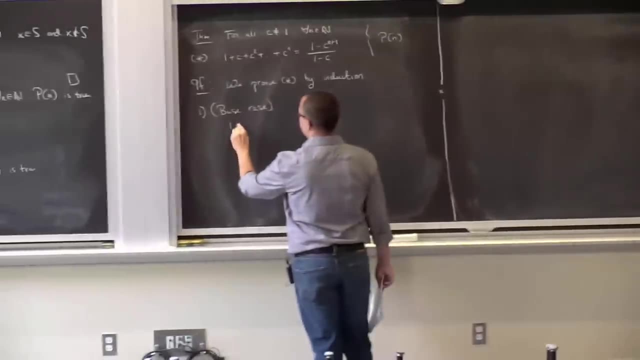 OK, Like I said, the base case is usually you just plug in n equals 1 and verify that p of n is true. And that's what we do: 1 plus c to the 1, which is the left-hand side. 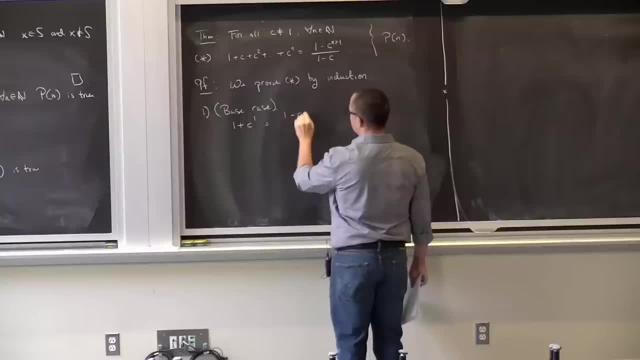 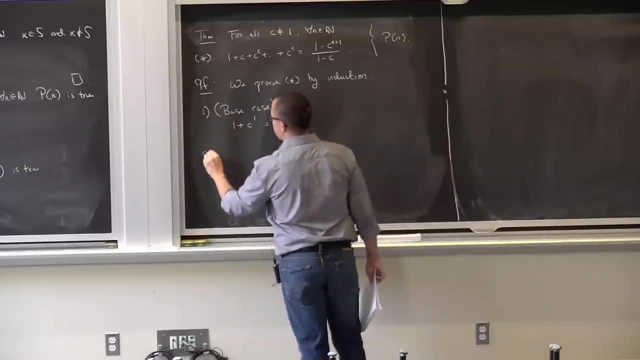 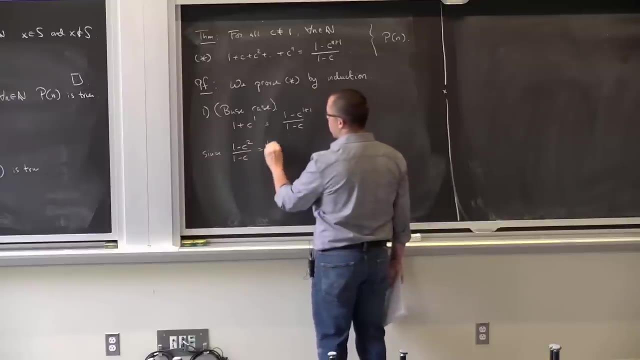 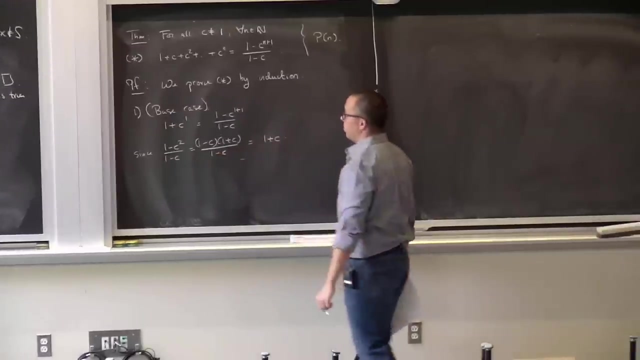 does in fact equal 1 minus c to the 1 plus 1 over 1 minus c, Because this right-hand side, 1 minus c, squared is 1 minus c times 1 plus c, The 1 minus c's cancel, and so the base case is proven. 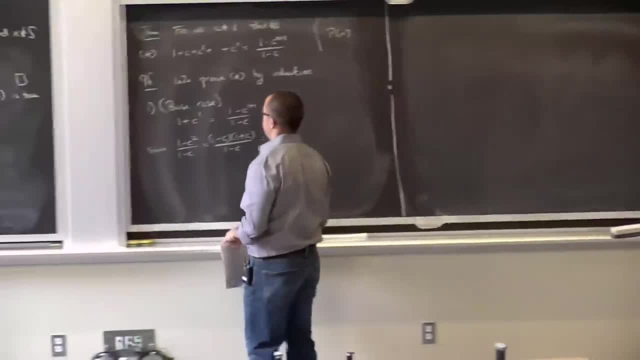 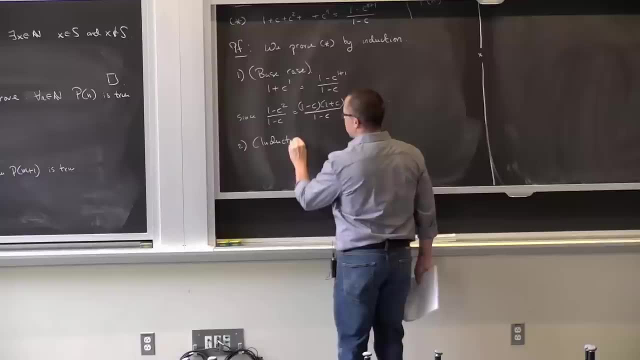 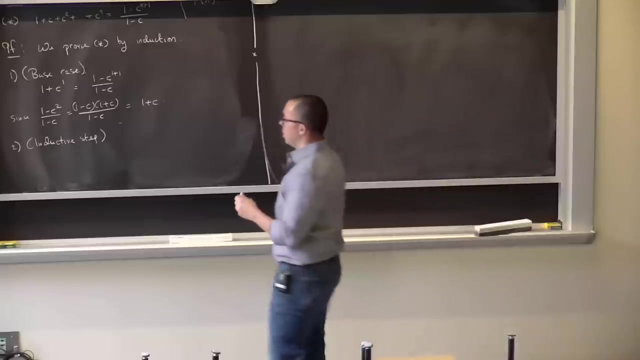 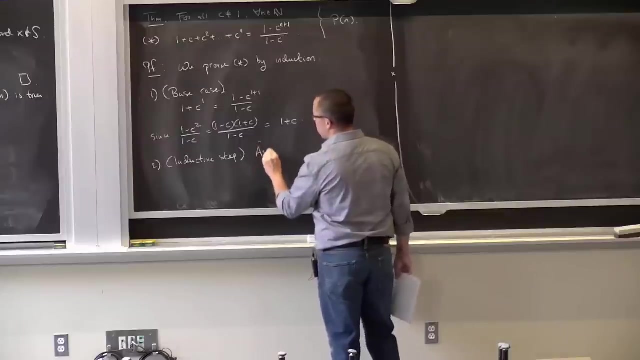 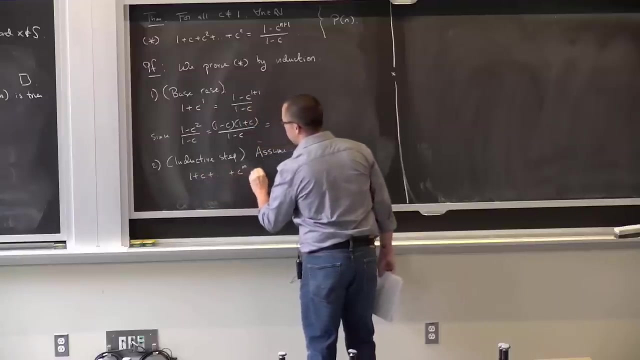 All right, Now we do the inductive step. OK, So we're going to assume that star holds for: n equals m. So we're going to assume p of m. So assume that 1 plus c plus c to the m equals 1 minus c over 1. 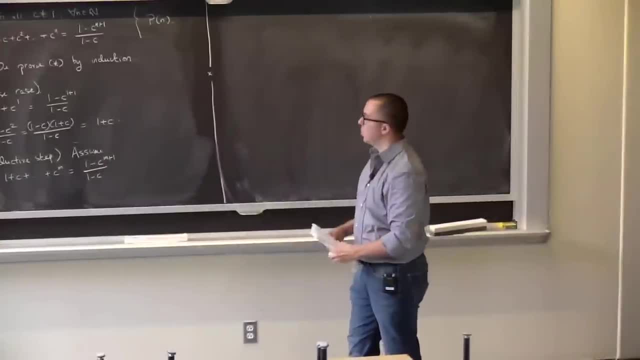 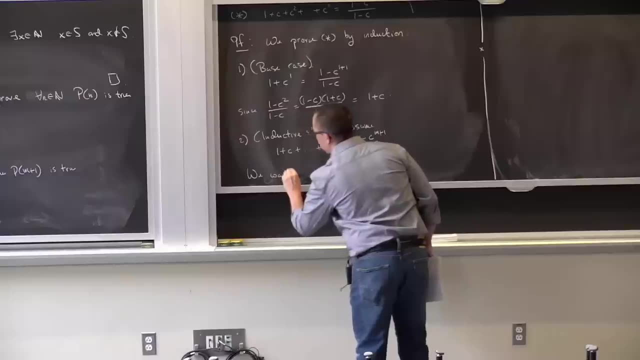 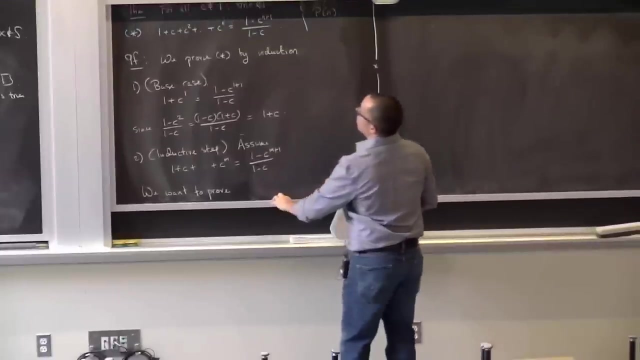 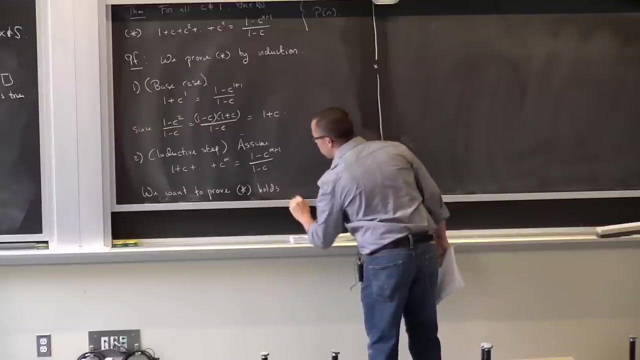 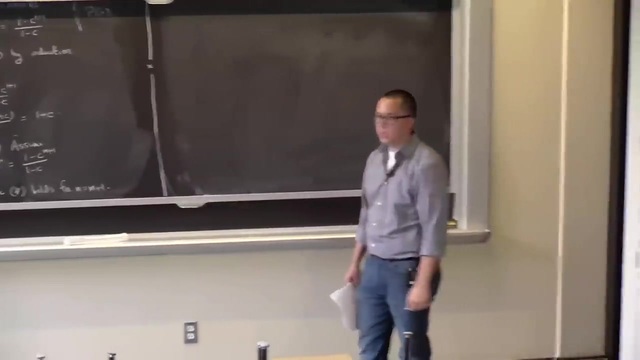 minus c. OK, Now we want to show again. let's write out what we want to do. What's our plan. We want to prove that this equality that this line star holds for n equals m plus 1.. OK, 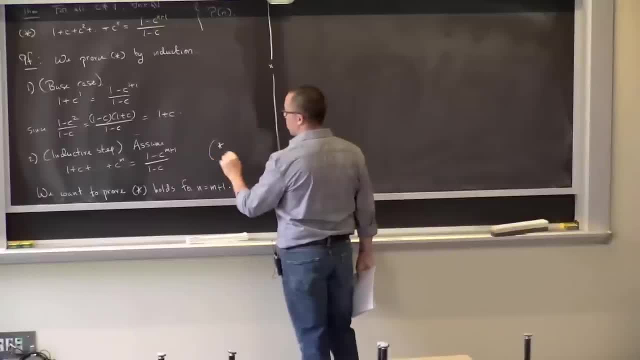 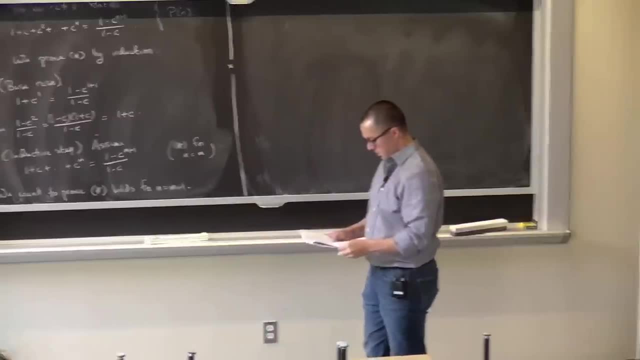 So again, this is what I wrote here. This is basically star for n equals m plus 1.. OK, So again, this is what I wrote here. This is basically star for n equals m plus 1.. OK, So this is our assumption. for n equals m. 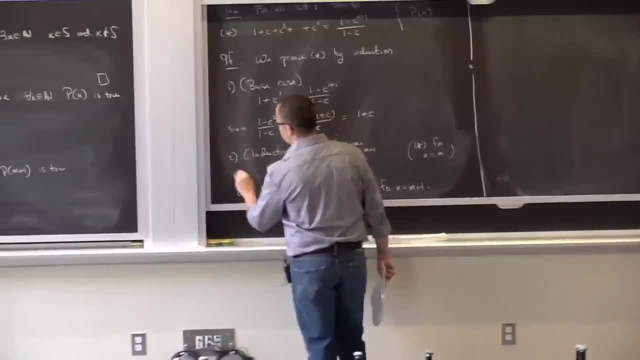 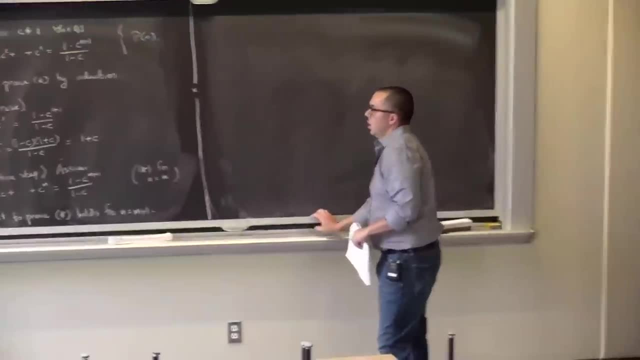 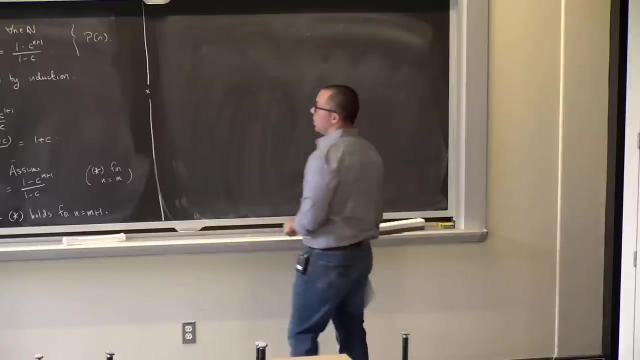 OK, And let me call this second equality 2 star. So this is my assumption. for m, n equals m. OK. So let's take the left side, for n equals m plus 1, and see if we cannot massage it to get, I guess, 2 stars. 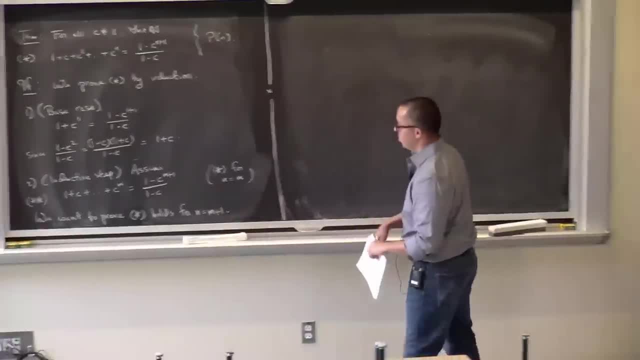 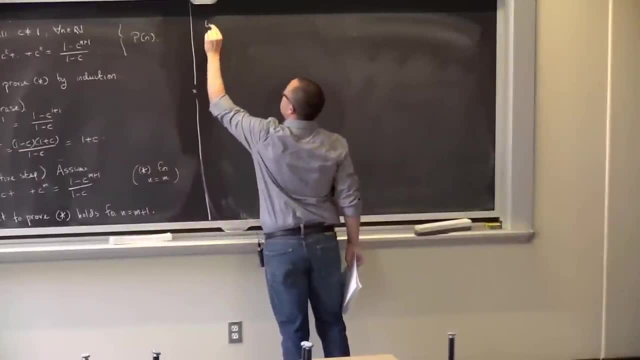 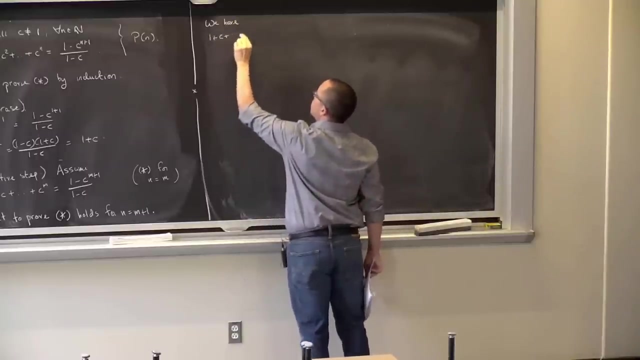 All right, All right, All right, the right-hand side for I should say the right-hand side for n equals n plus 1.. So here is the calculation part. So we have 1 plus c, plus c to the m, plus c to the m plus 1.. 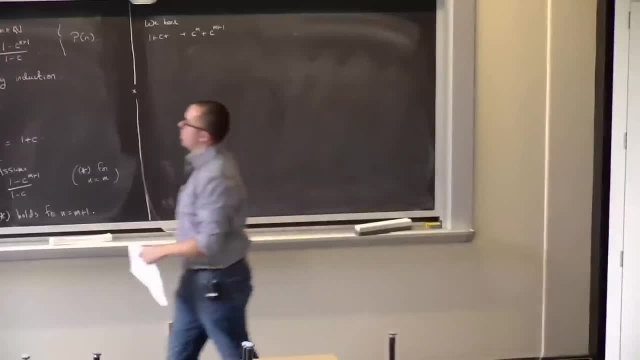 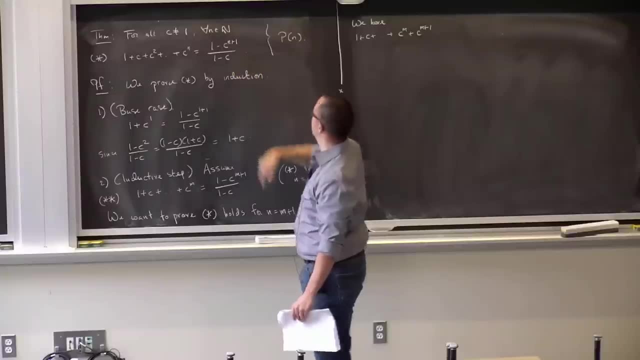 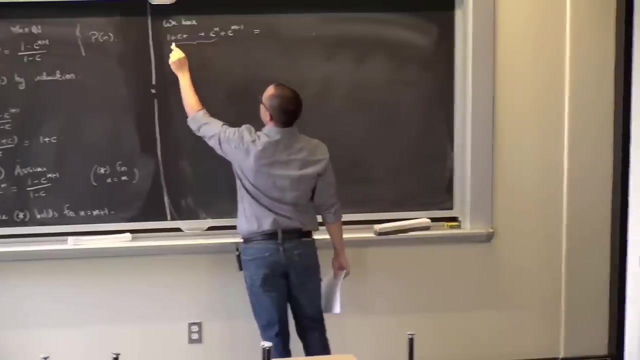 This is the m plus 1 case of the left-hand side of star, which we want to show is equal to the n equals n plus 1 case of the right-hand side. Now, this is equal to. now we already know what this is equal to by our assumption. 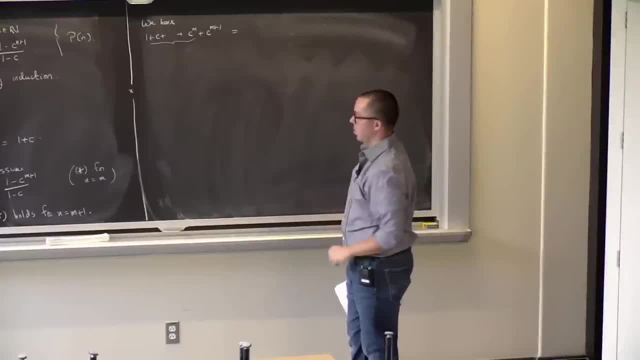 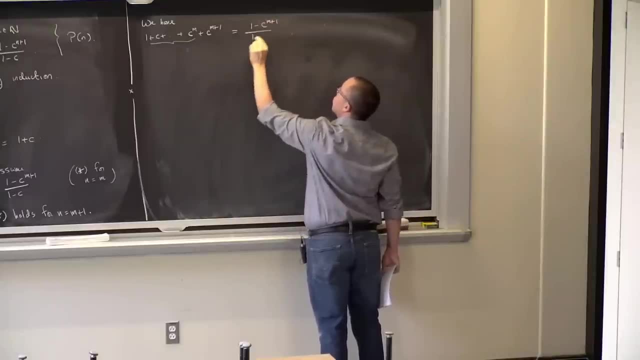 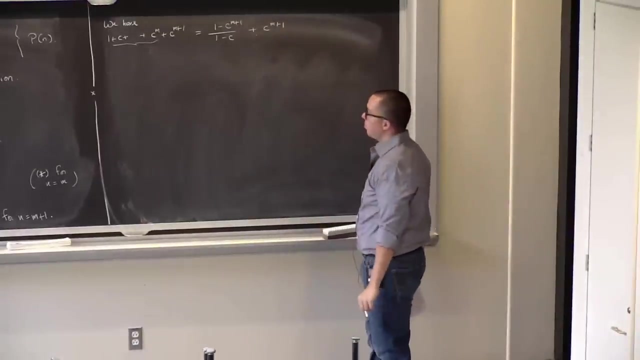 This is by the second star there, which is what we're assuming is true. This is equal to 1 minus c? n plus 1 over 1 minus c plus c, n plus 1.. And so now we just do a little bit of algebra. 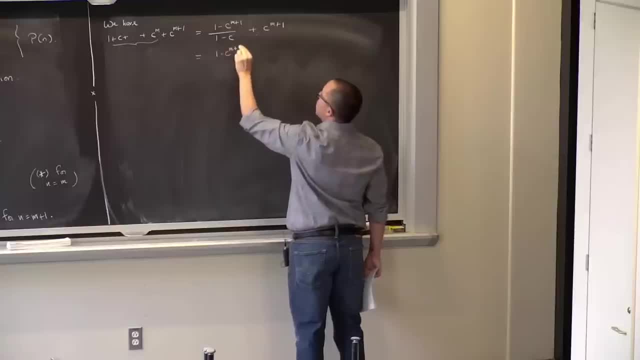 This is equal to 1 over 1 minus c, n plus 1 plus c, n plus 1 minus c, n plus 2 over 1 minus c. Those cancel and I'm left with 1 minus c to the m plus 2.. 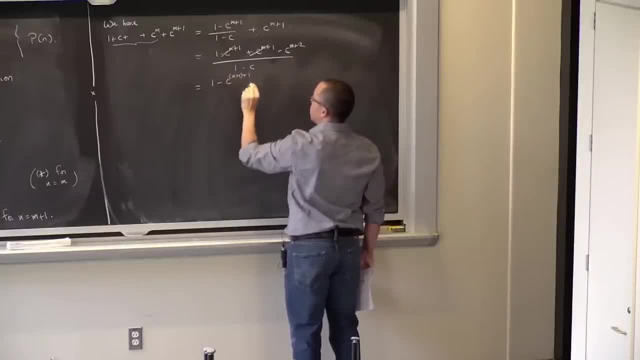 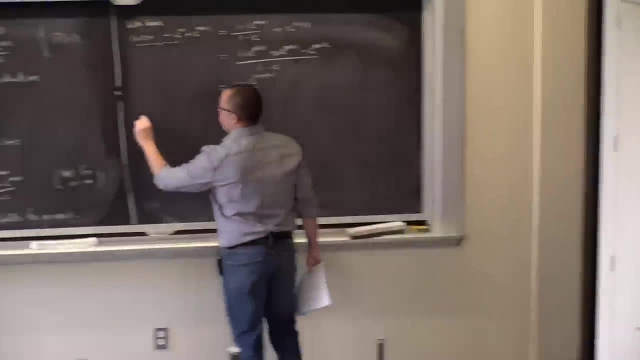 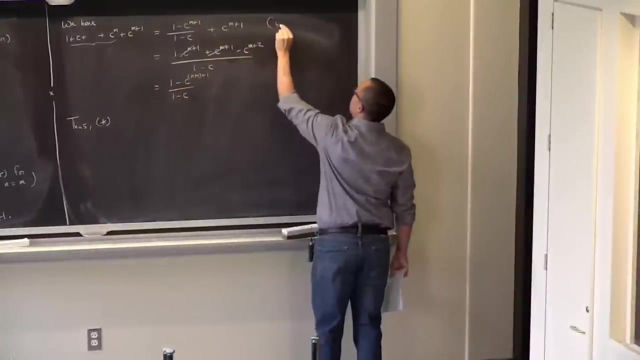 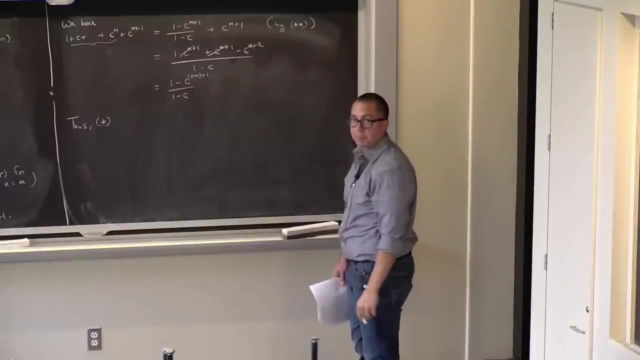 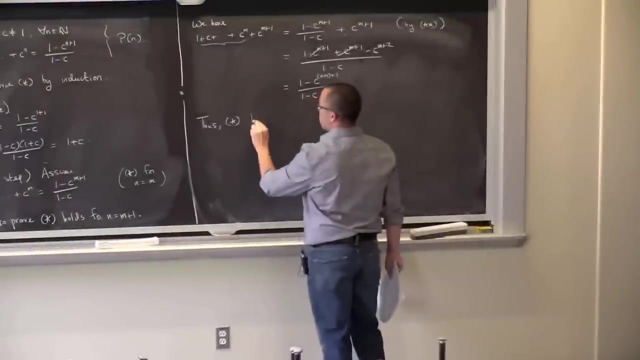 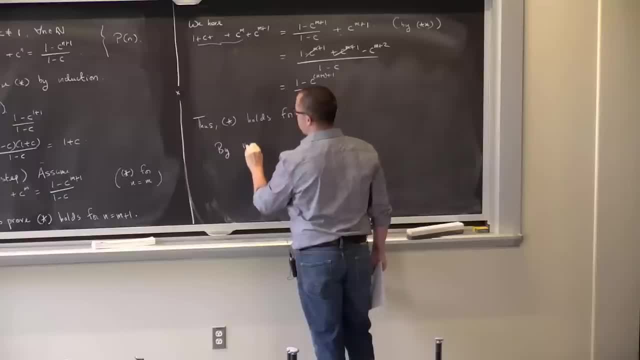 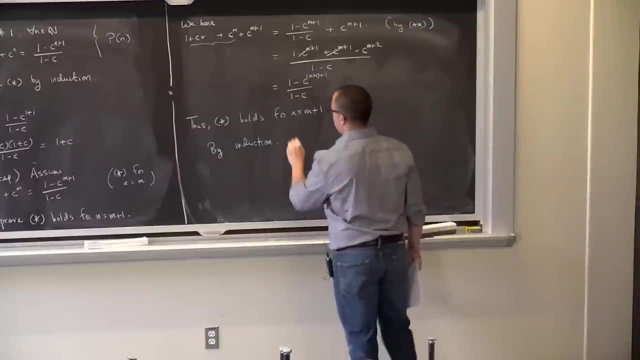 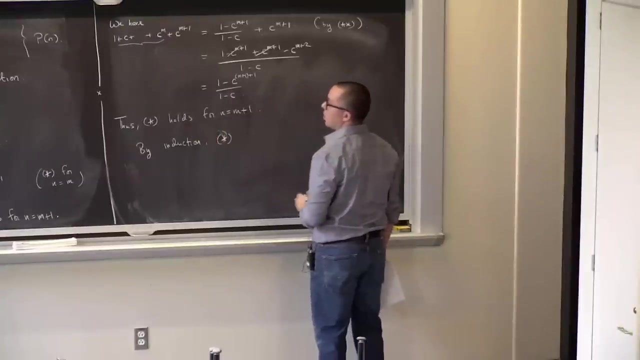 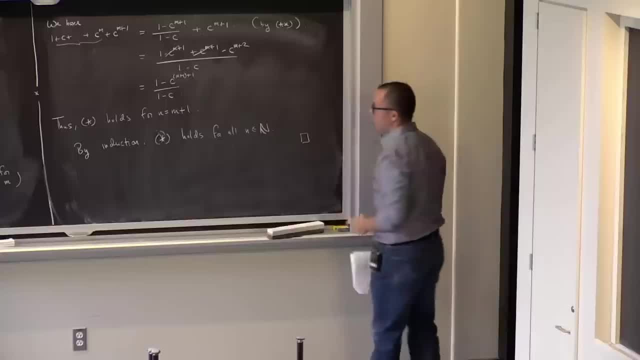 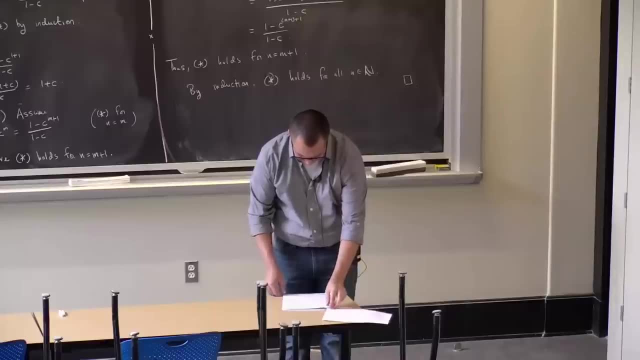 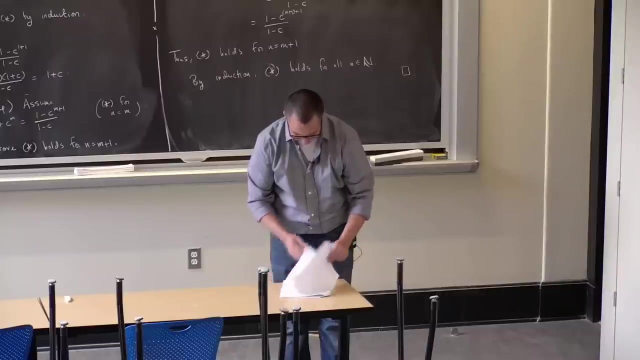 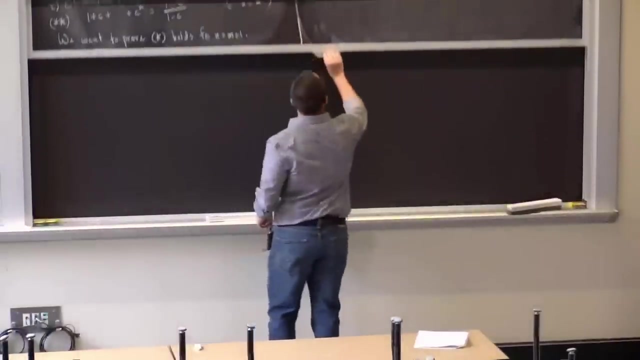 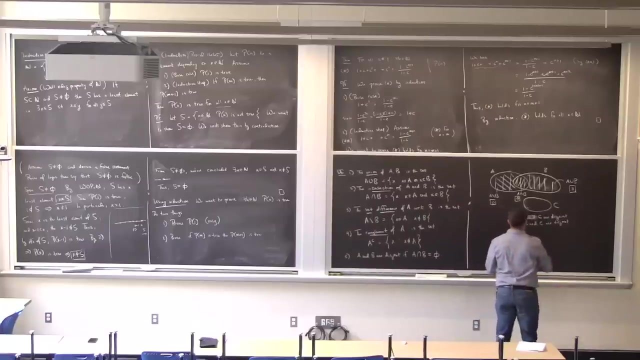 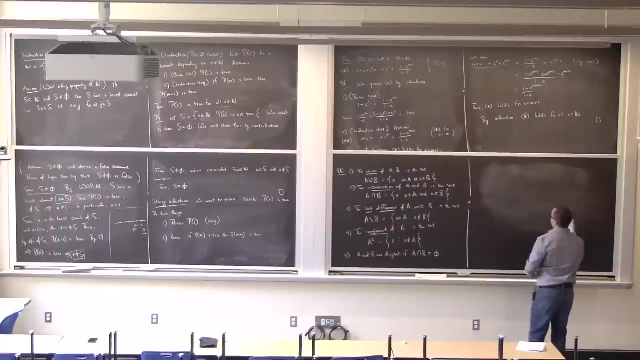 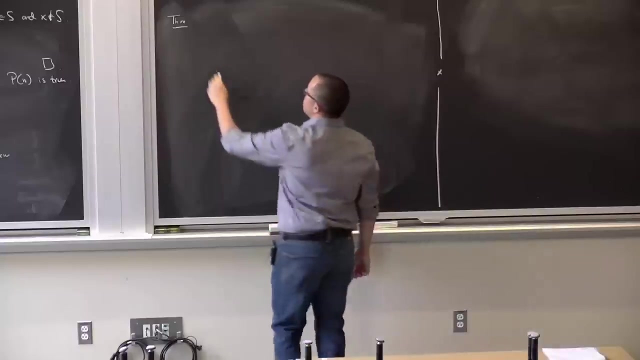 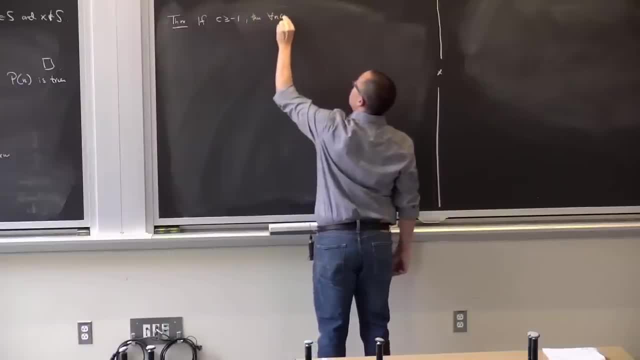 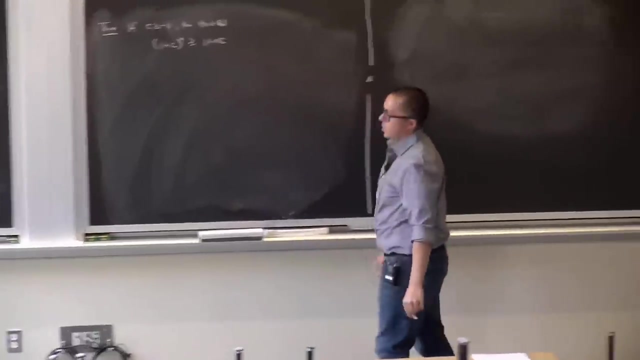 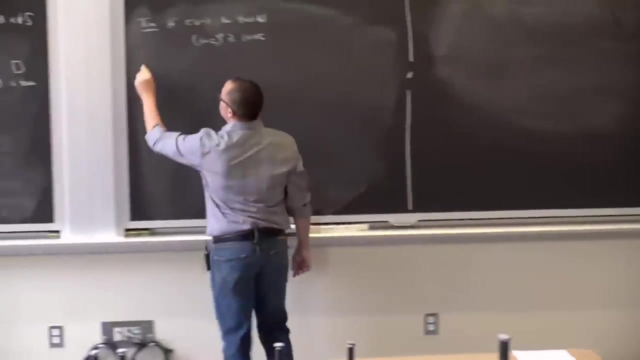 then for all n natural number, 1 plus C to the n is bigger than or equal to 1 plus n times C. Okay, All right, so we're going to do this by induction. again, That means we need to prove the base case. 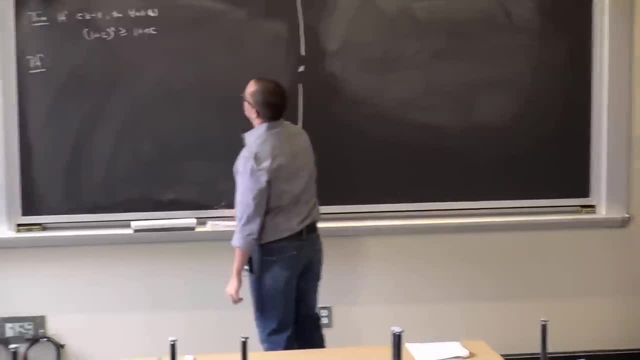 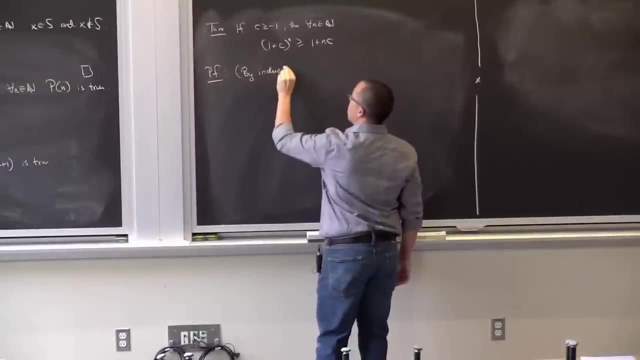 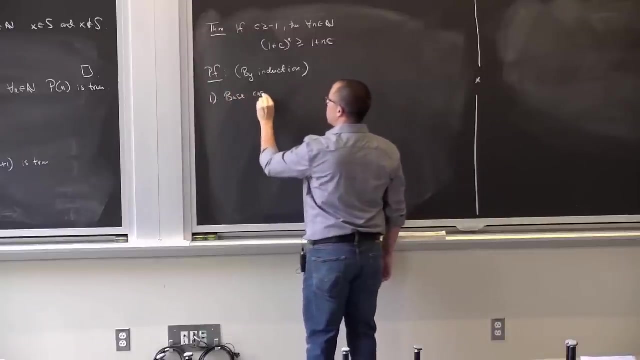 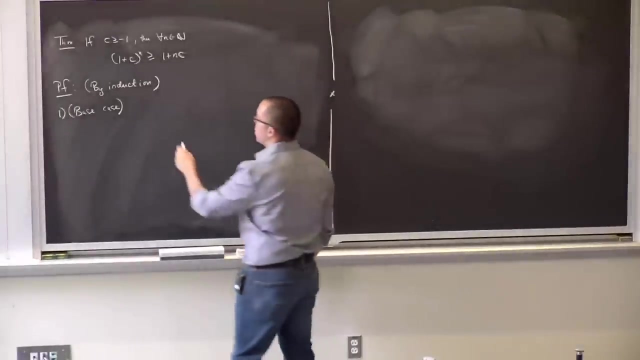 And we need to do the inductive step. So base case, as always will. So this is just right here: We're going to do this by induction. So, as you can see, the base case is again: n equals 1. is clear just by looking at it. 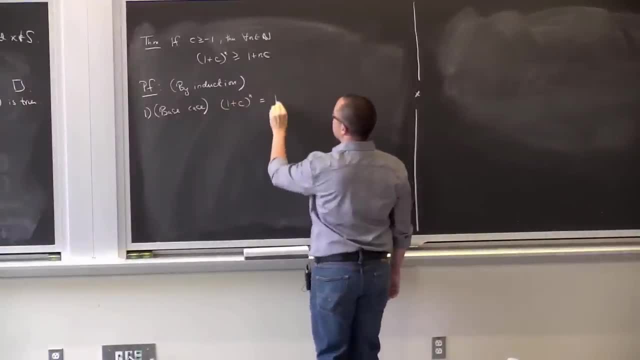 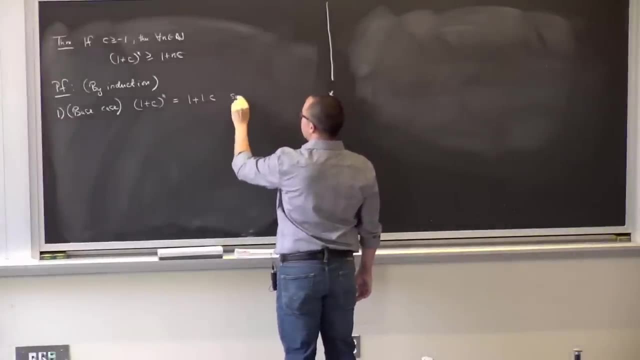 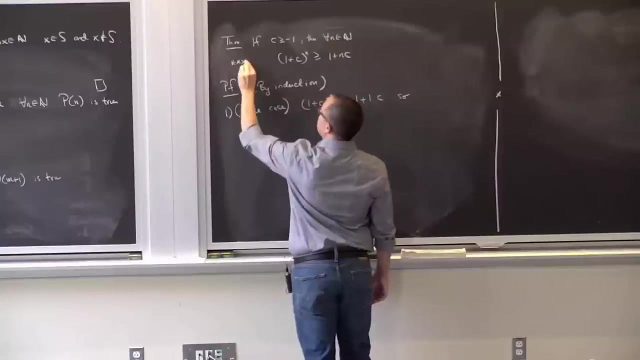 1 plus C to the 1, in fact equals 1 plus 1 times C. So it's certainly bigger than or equal to 1 plus n times C. So I think that's the last stars I'll use for this lecture. 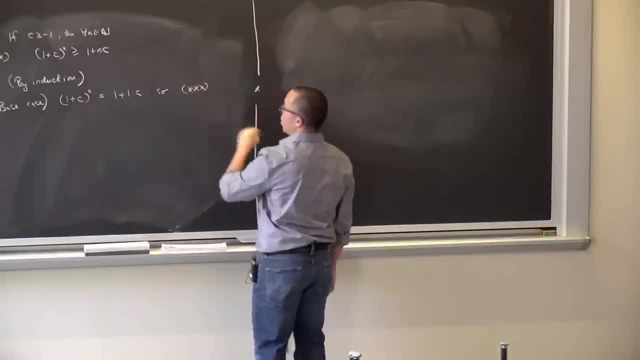 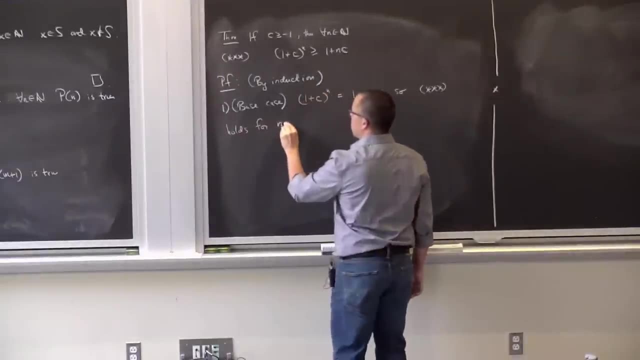 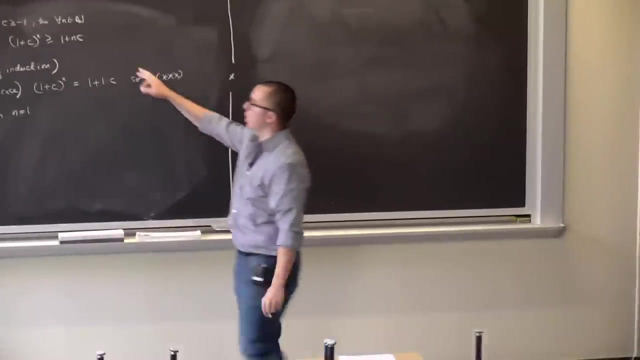 So our statement: our inequality, star, star, star star. holds for n equals 1.. All right, so that's our base case. Now we're going to assume that this inequality holds for n equals m, and try to prove that it holds for n equals m plus 1.. 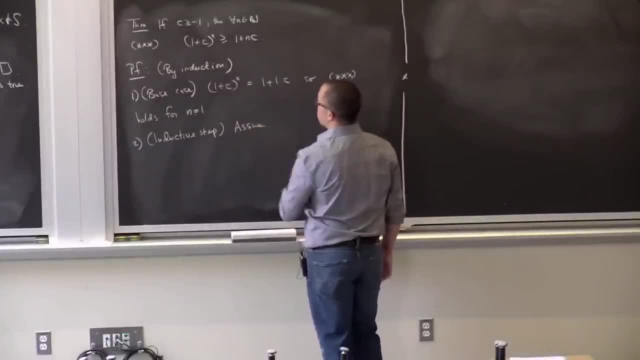 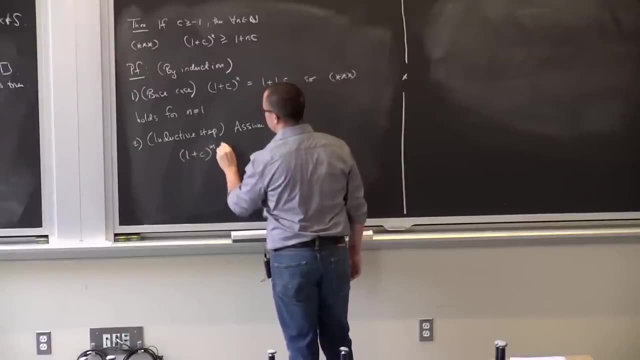 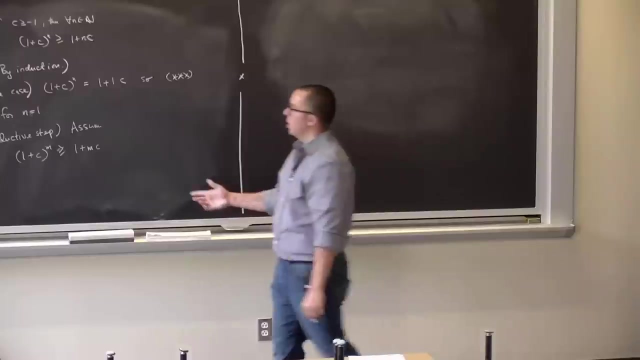 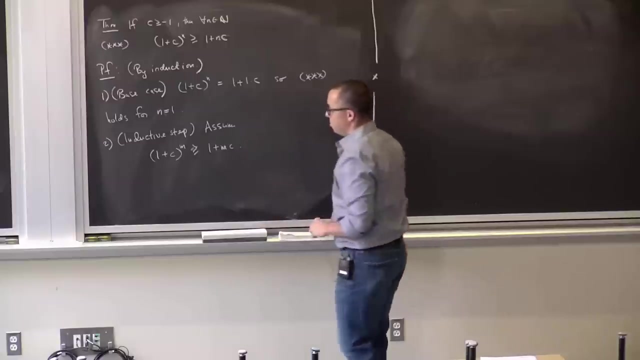 So we're assuming this when n equals m. So 1 plus C to the m is bigger than or equal to 1 plus m times C. And we want to prove this inequality with n equal to m plus 1.. And we're just assuming this guy. 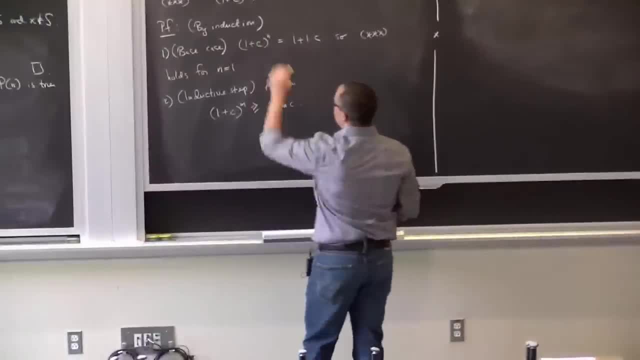 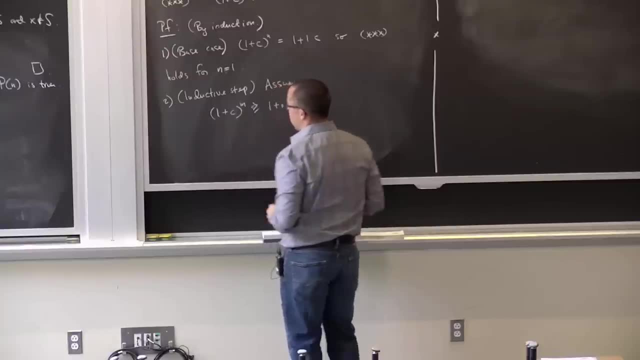 So I want to get the statement for: n equals m plus 1.. One way to do that is this left side I want to get: Let's look at the n equals m plus 1.. Let's look at the n equals m plus 1 side and see what we can do with it. 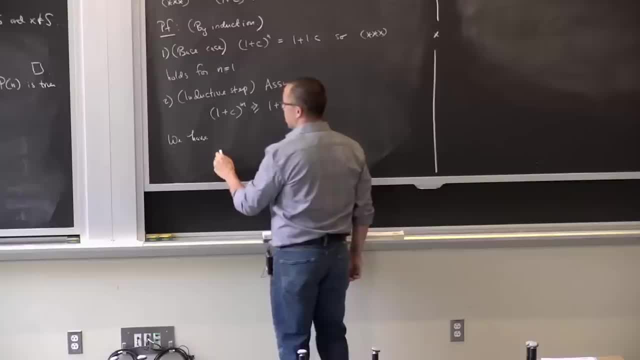 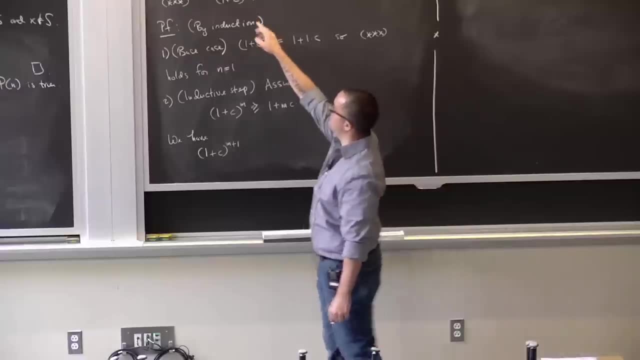 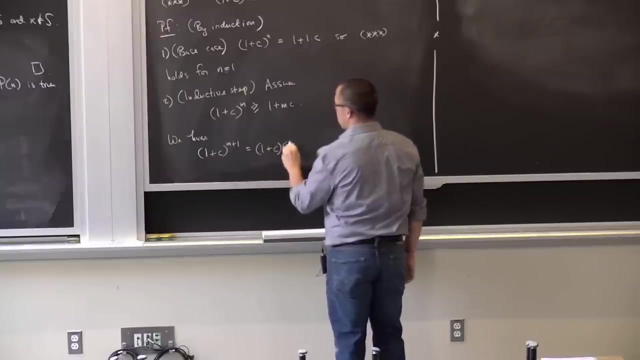 So again, this is a calculation part and logic. So we have 1 plus C to the m plus 1.. So that's the n equals m plus 1 side of this. This is equal to 1 plus C times 1 plus C to the m. 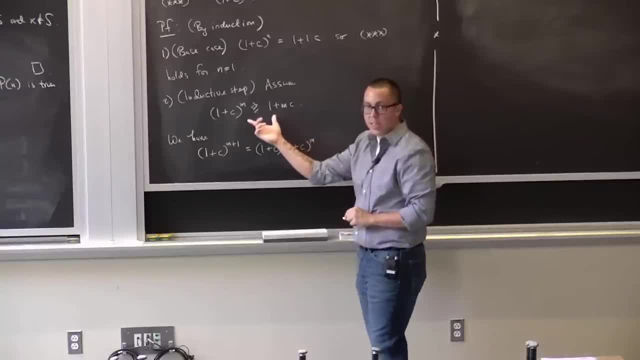 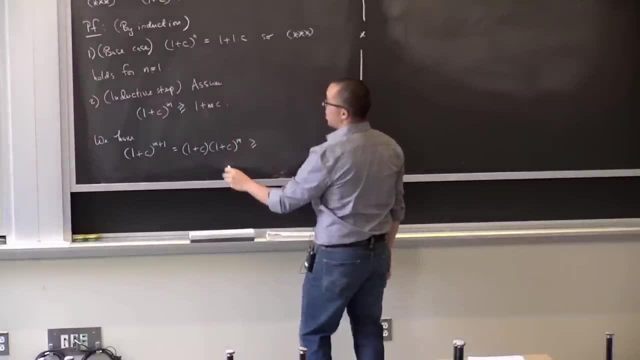 Now we're assuming again this inequality. This is the n equals m case, So we can use it. So we're assuming it. We use it This: And since C is bigger than or equal to minus 1,, 1 plus C is non-negative. 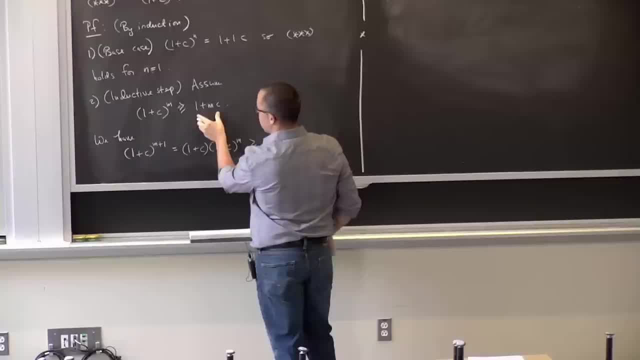 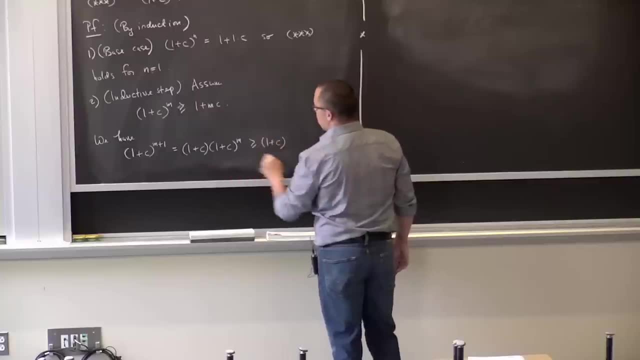 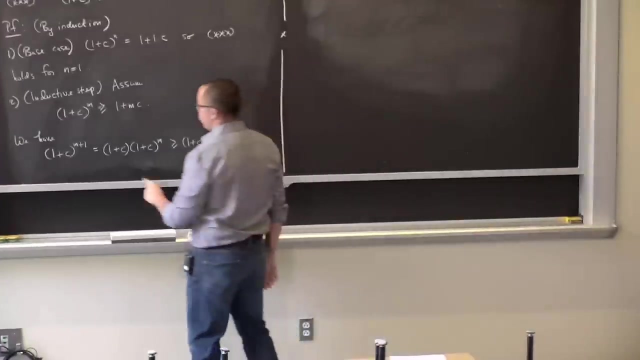 So this thing is bigger than or equal to this thing. So if I multiply both sides by 1 plus C, I preserve the inequality. So this is bigger than or equal to 1 plus mC. Okay, Again, this just follows. 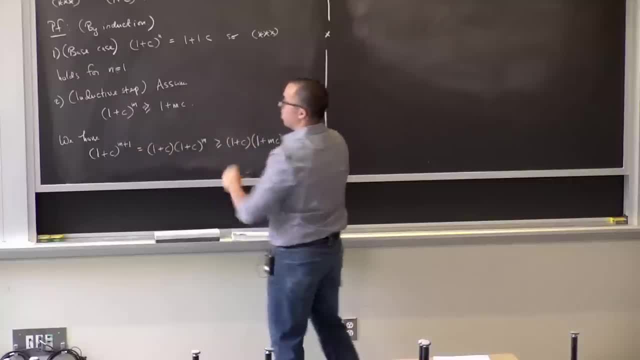 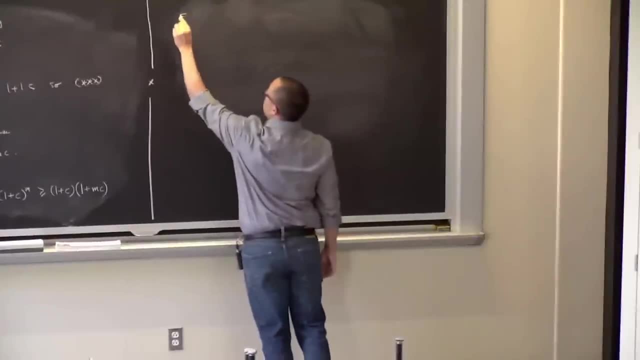 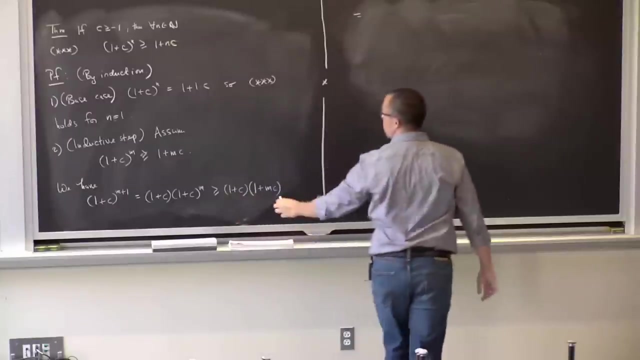 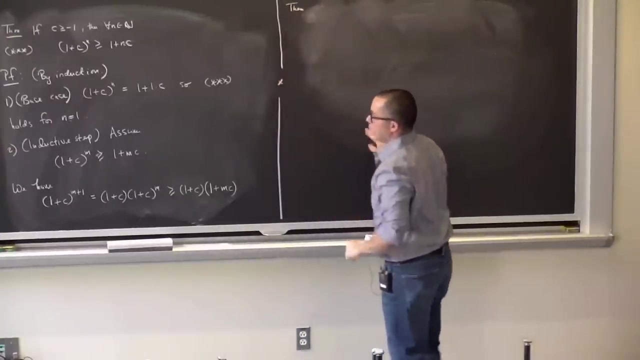 This follows from, essentially the assumption multiplied through by 1 plus C. Okay, And now? So now I'm going to finagle this, So let me just. I'm not doing anything different here, I'm just going to rewrite this over here so that I can. 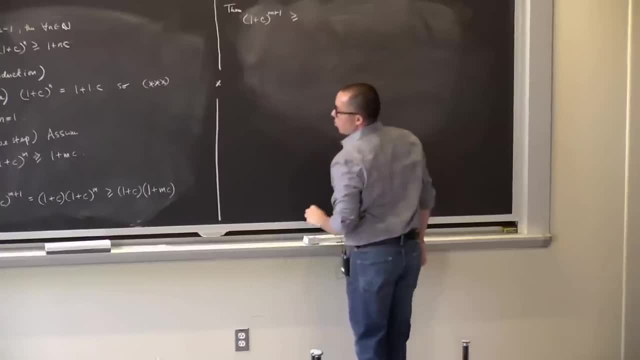 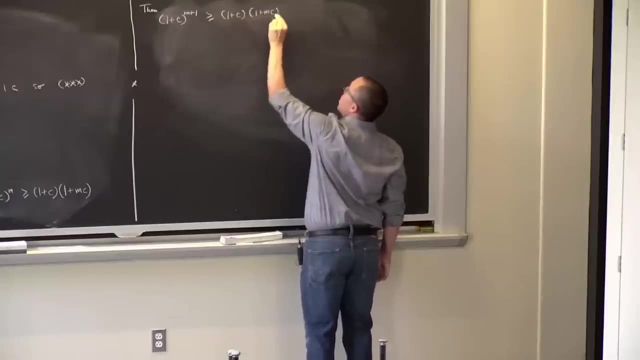 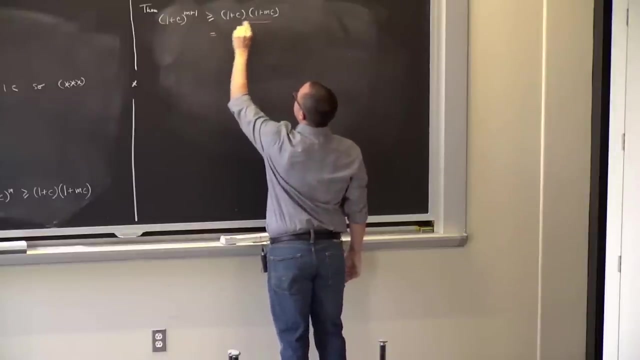 have a chain of inequalities. So I have 1 plus C to the m plus 1 is greater than or equal to 1 plus C, 1 plus mC. All right, So now this is bigger than or equal to this And this here. 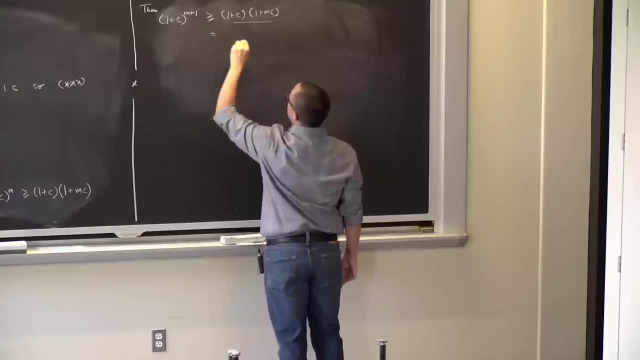 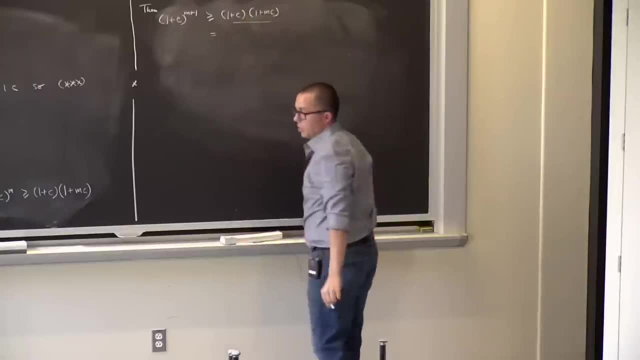 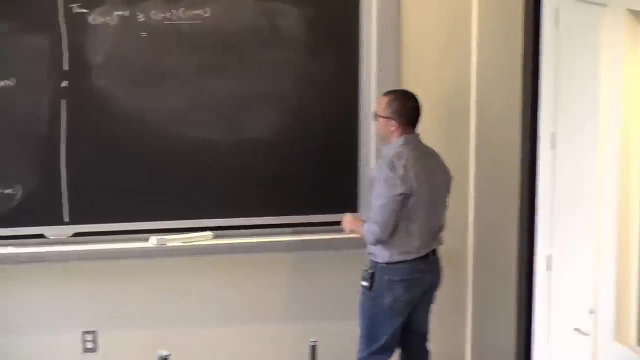 So when I write it equal, I do not mean that this left side is now equal to what I'm about to write here. That means the previous thing on here is equal to what I'm about to write here. Okay, This is a typical fashion in writing down inequalities, or, I guess, practice. 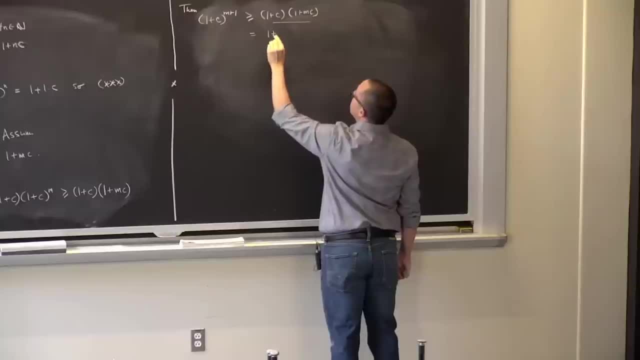 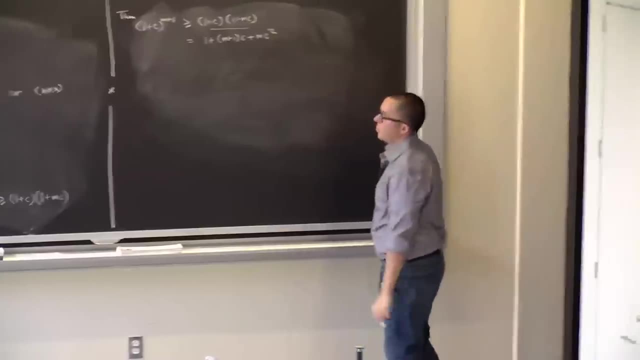 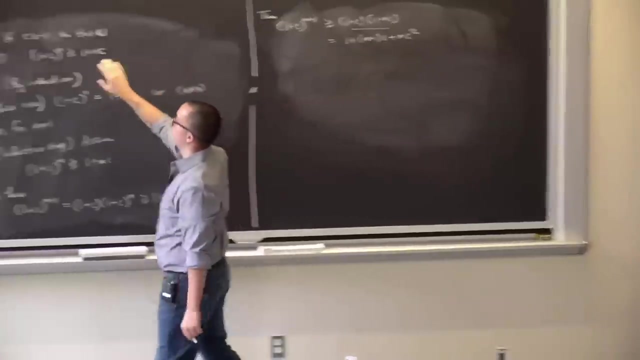 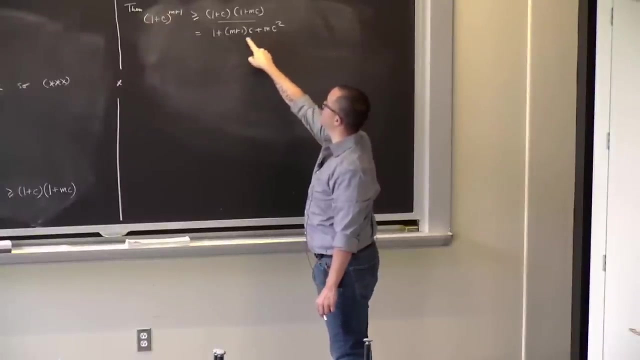 So this is equal to 1.. So just doing the algebra m plus 1 times C, plus m times C, squared, Okay, Now this part is exactly the n equals m plus 1 side of this, And I have a little room to give because now this is plus something that's non-negative. 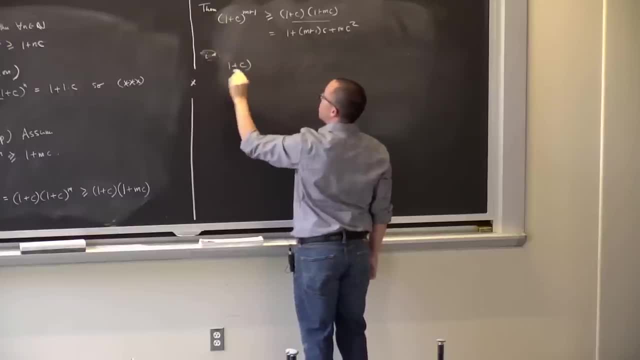 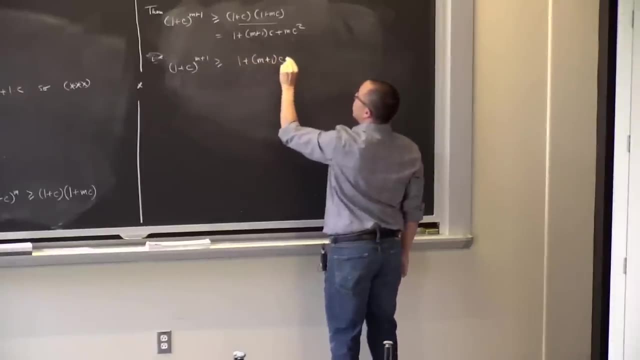 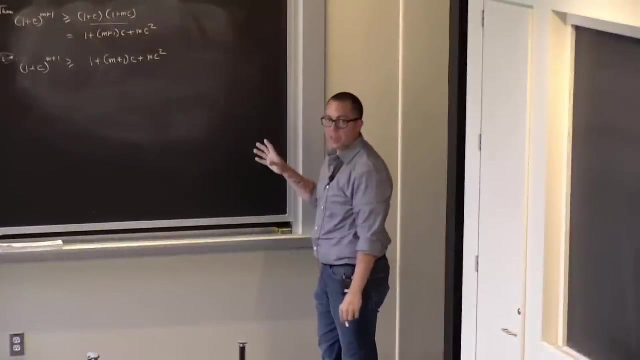 So let me just rewrite this again. This means that 1 plus C to the m plus 1 is greater than or equal to 1 plus. So again, I'm kind of writing a lot here. I will stop writing. I will stop writing as much as the course goes on. 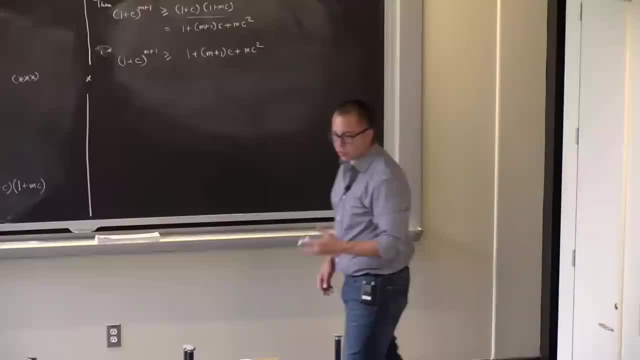 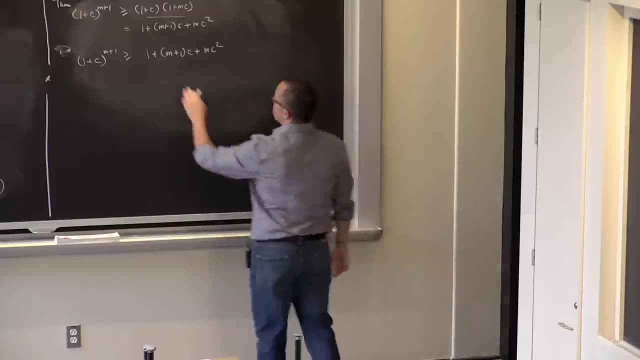 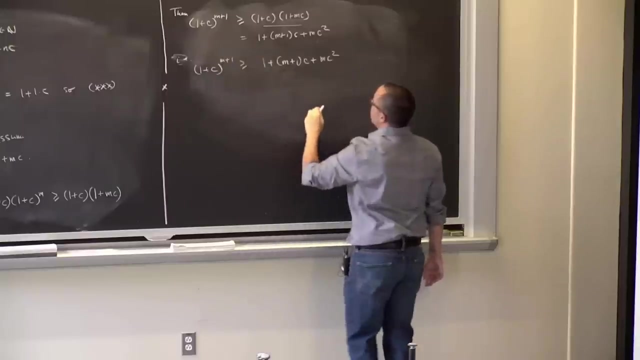 But I encourage you, especially in the beginning, to write all the steps in logic. Okay, So again, I'm not rewriting anything, I'm just summarizing what I've done here. Now, this right-hand side- So I have this- is bigger than or equal to this. 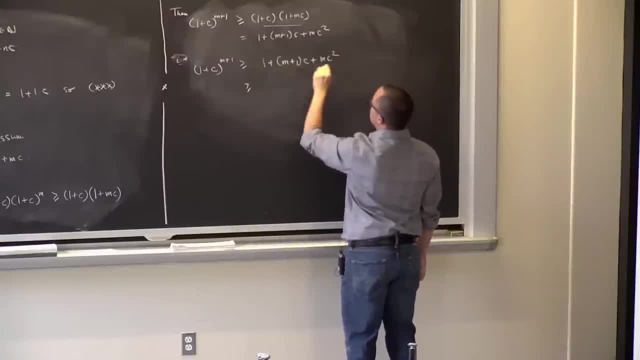 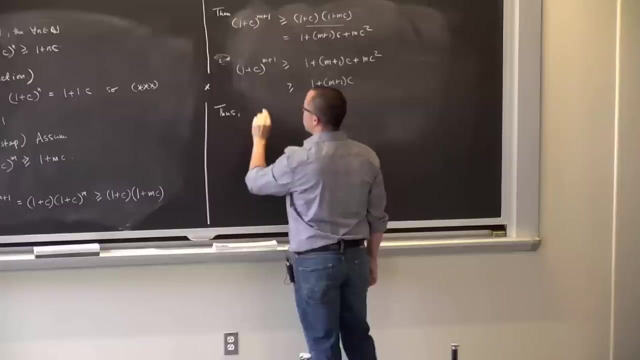 And this right-hand side. since I have a number plus something non-negative: m times C squared m is a natural number. This is bigger than, or equal to, 1 plus m plus 1 times C. Thus, 1 plus C to the m plus 1 is greater than or equal to. 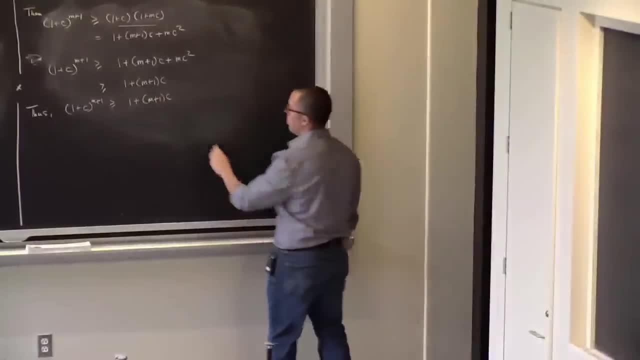 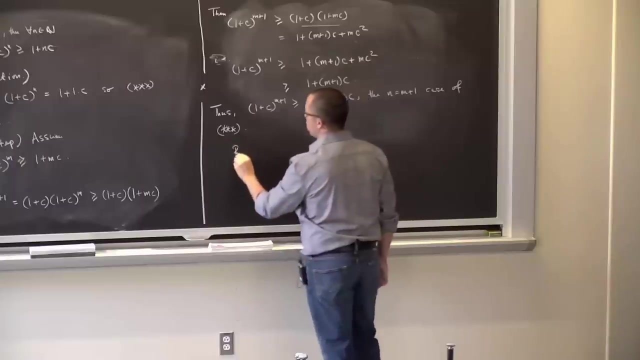 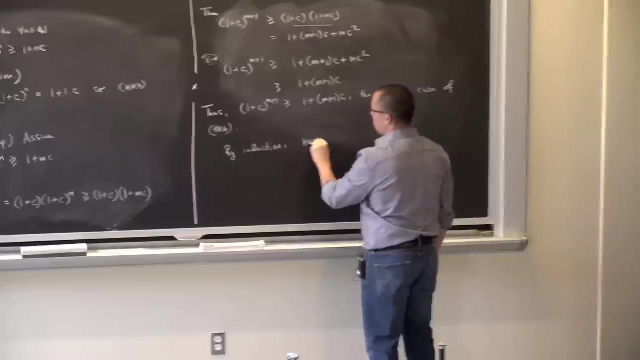 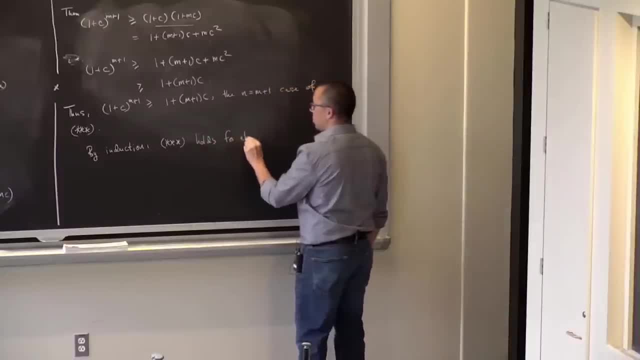 I'm going to write this again. I'm going to write this again, All right.